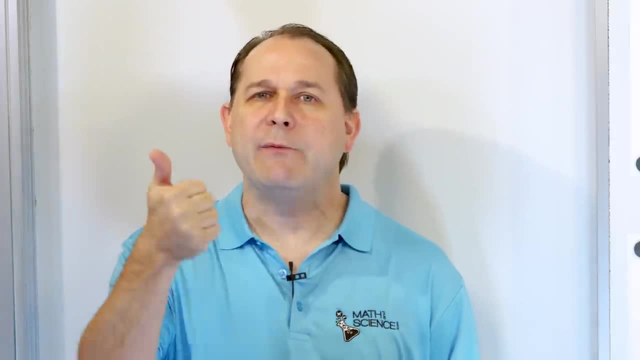 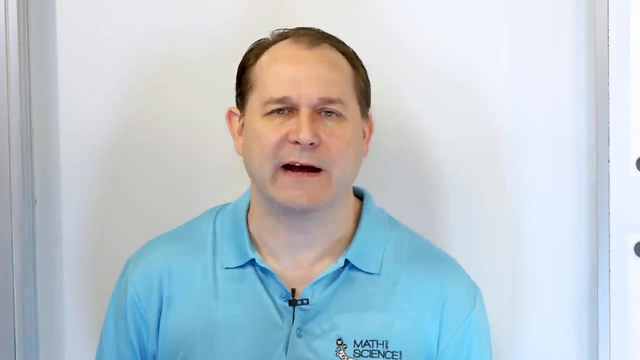 things that you have everyday experience with right. There's a couple of things Everybody is familiar with: flipping a coin, a two-sided coin. Everyone is familiar with a deck of cards, grabbing cards out of a deck of cards. We're going to talk about that. 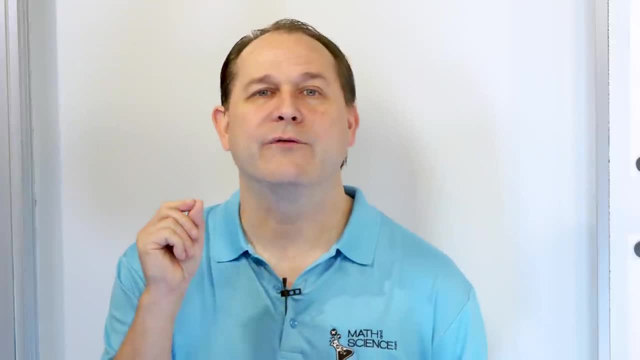 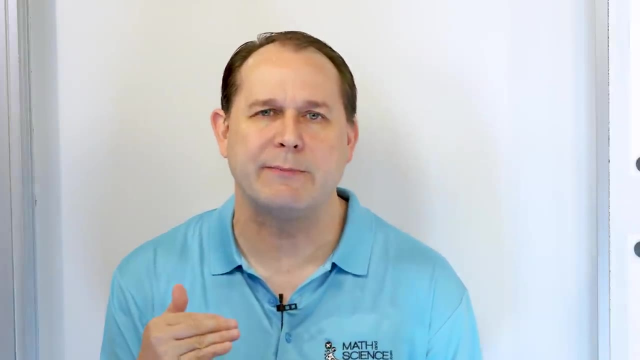 And everybody is familiar with the forecast of the weather. okay, So let's talk about the forecast of the weather for just a minute. We're going to talk about lots of things before we get into calculating probability, But for now let's just get an idea of what it means. So if the weather 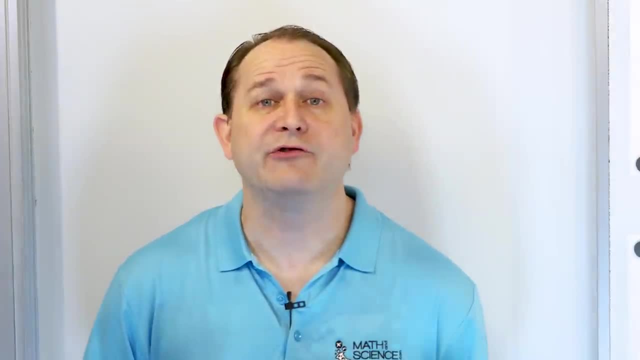 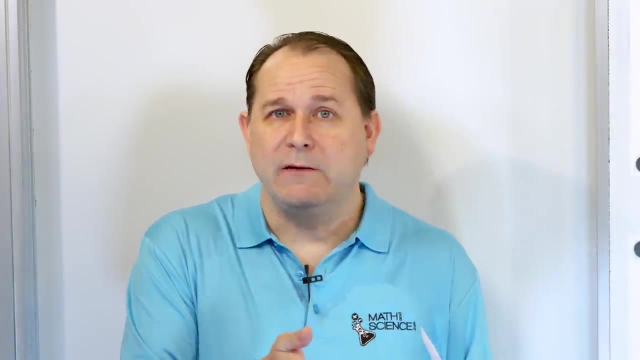 person comes on and says there is a 50% chance of rain tomorrow. right, Then, what do you interpret that to mean? Well, it means tomorrow it might rain or it might not rain. You're not totally sure, because the percentage is 50%, which means it's not going to rain tomorrow. So you're not. 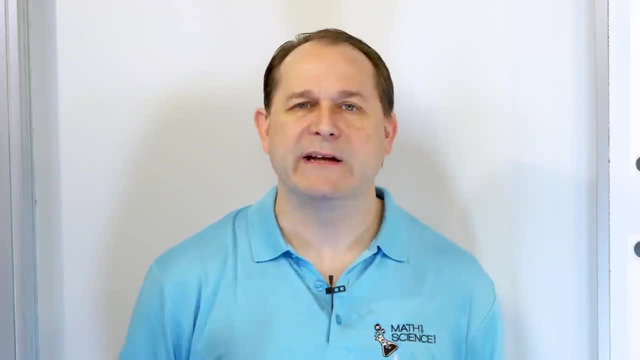 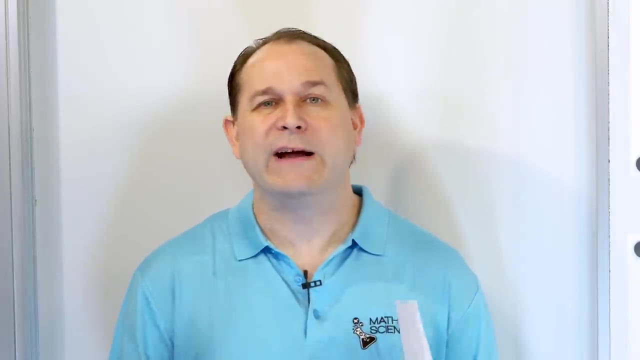 sure It means it's right in the middle. But if you instead hear that the probability of rain is 100%, then you know that it will definitely, totally, absolutely rain tomorrow. But if the chance of rain is 0%, then it will definitely not rain tomorrow. If we're right in the middle at 50%. 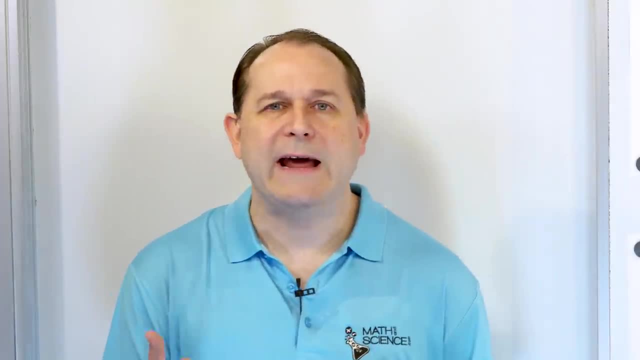 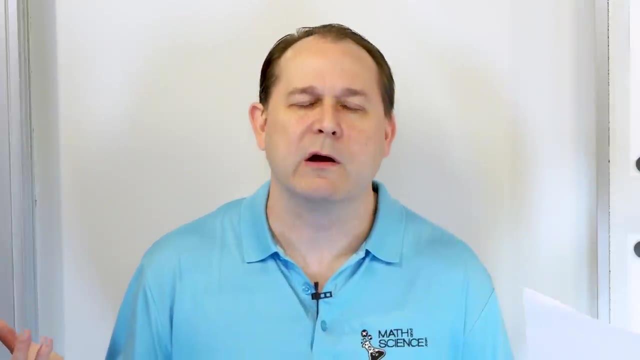 then it might rain or it might not rain, right. So of course, some days when the weather person says 50% chance of rain, some days you go outside it doesn't rain all day. You say, oh, the weather was wrong, That person was wrong. Or you go outside and a 50% chance of rain day. 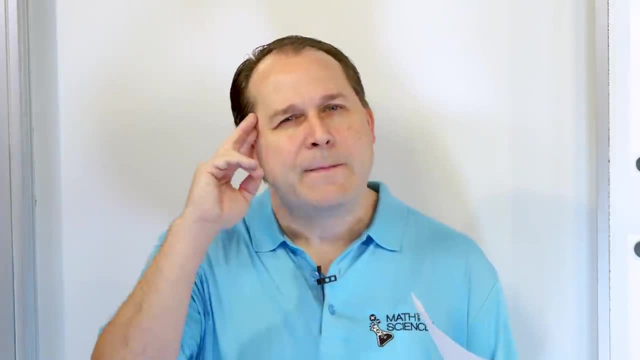 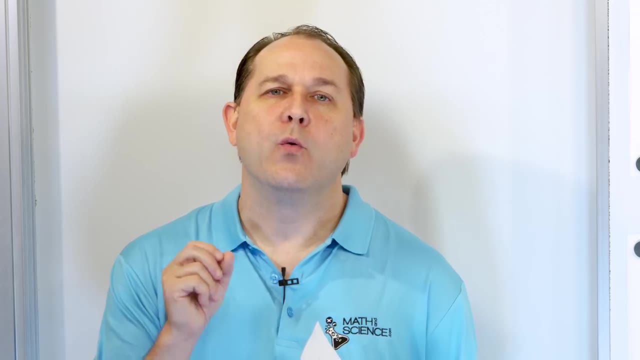 and it does rain And you say, oh, I guess they were right. We have our ideas in our mind about what it means. Let's talk more specifically about what actually a 50% chance of rain means. What it means is- if I can make a copy of that day- of all the atmospheric dynamics. 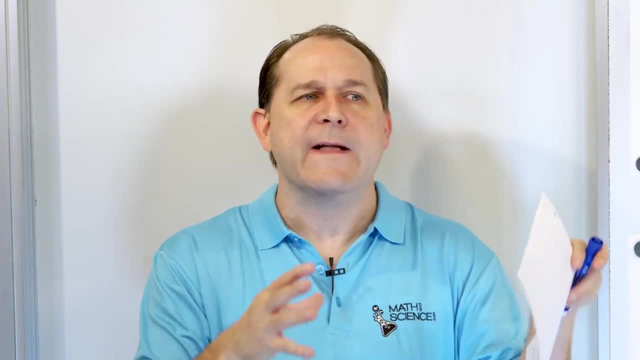 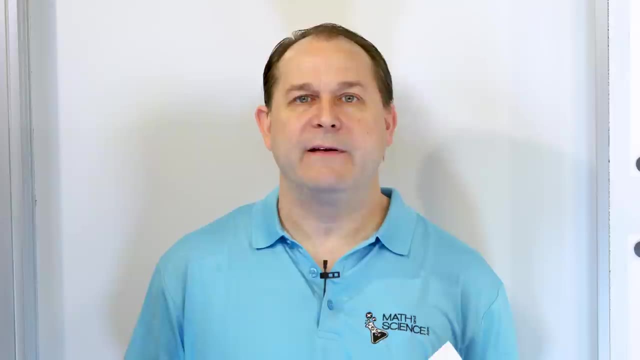 the weather patterns, the pressure, the clouds, the moisture content. if I could just, like in a computer, make a copy of tomorrow's weather situation and make a thousand copies or a million copies, And if I ran a computer simulation a million times with the exact 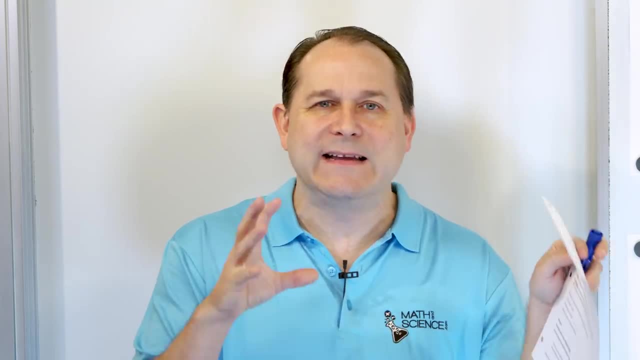 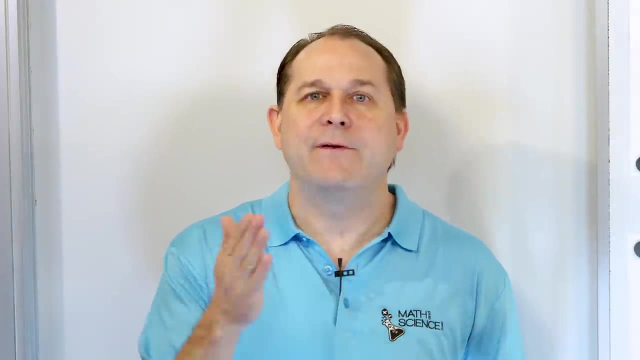 same weather. if I could repeat the day, exactly the same orientation of the atoms and the water in the clouds, then on average, about half of those days would rain And the other half of the days it wouldn't rain. So clearly, some of those days it would not rain And some of those days 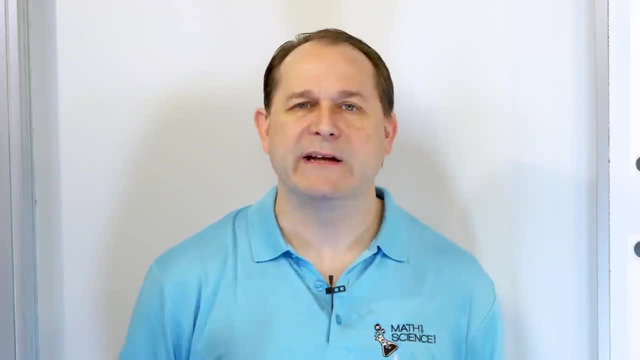 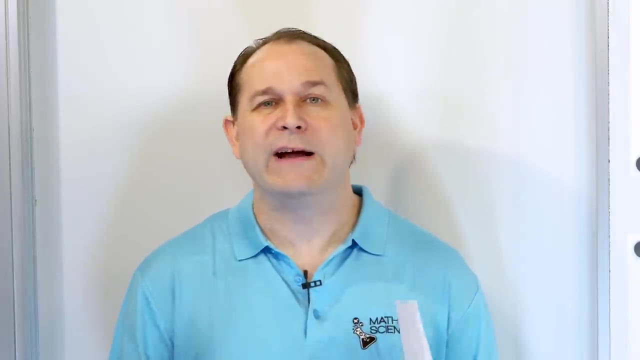 sure It means it's right in the middle. But if you instead hear that the probability of rain is 100%, then you know that it will definitely, totally, absolutely rain tomorrow. But if the chance of rain is 0%, then it will definitely not rain tomorrow. If we're right in the middle at 50%. 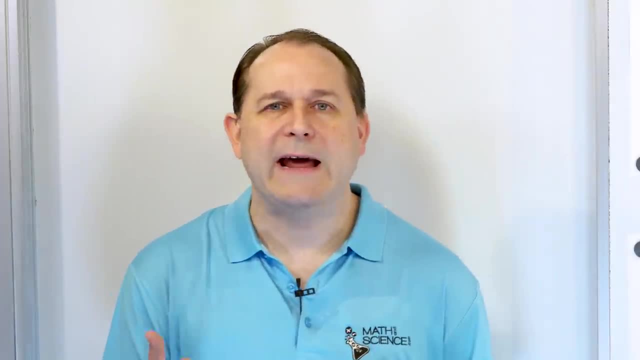 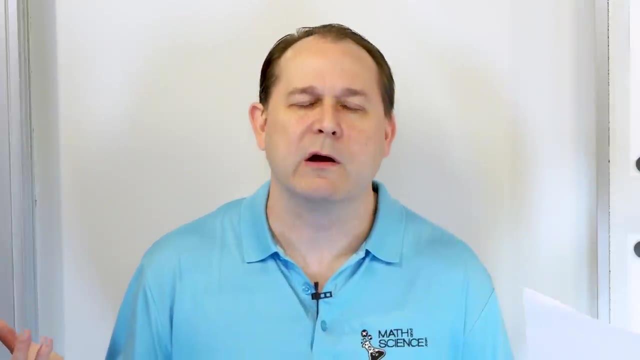 then it might rain or it might not rain, right. So of course, some days when the weather person says 50% chance of rain, some days you go outside it doesn't rain all day. You say, oh, the weather was wrong, That person was wrong. Or you go outside and a 50% chance of rain day. 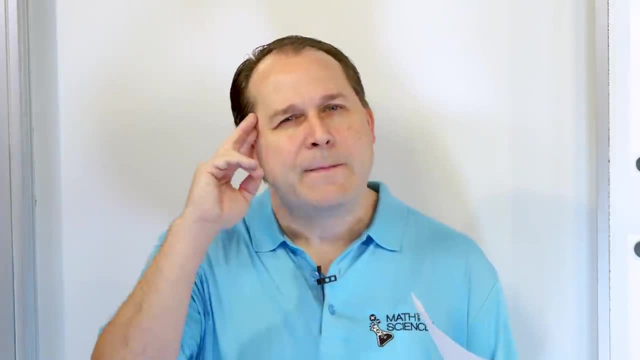 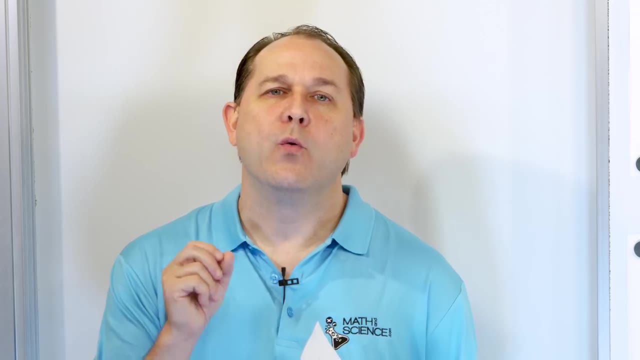 and it does rain And you say, oh, I guess they were right. We have our ideas in our mind about what it means. Let's talk more specifically about what actually a 50% chance of rain means. What it means is- if I can make a copy of that day- of all the atmospheric dynamics. 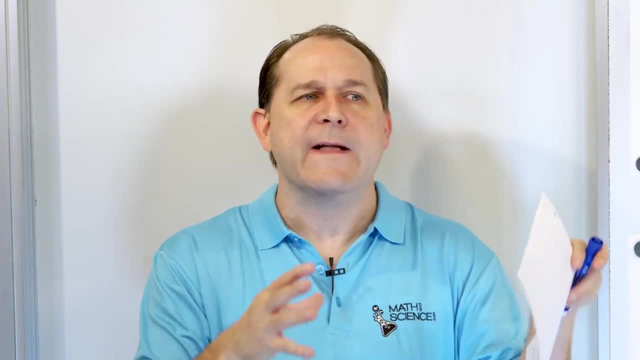 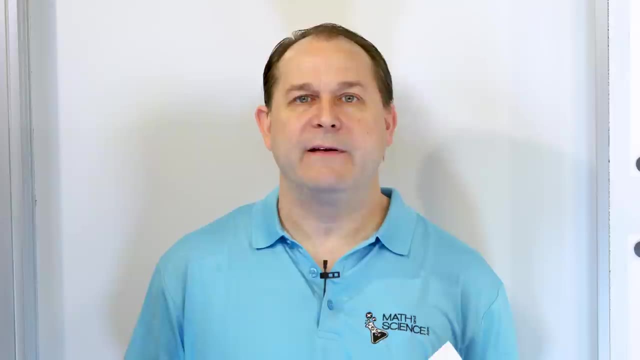 the weather patterns, the pressure, the clouds, the moisture content. if I could just, like in a computer, make a copy of tomorrow's weather situation and make a thousand copies or a million copies, And if I ran a computer simulation a million times with the exact 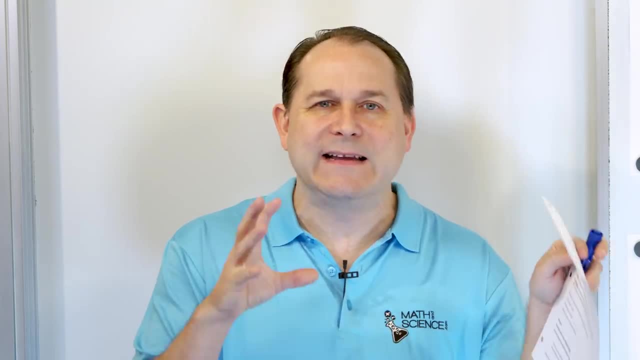 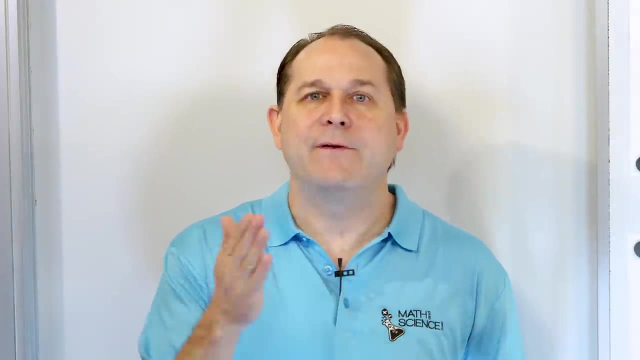 same weather. if I could repeat the day, exactly the same orientation of the atoms and the water in the clouds, then on average, about half of those days would rain And the other half of the days it wouldn't rain. So clearly, some of those days it would not rain And some of those days 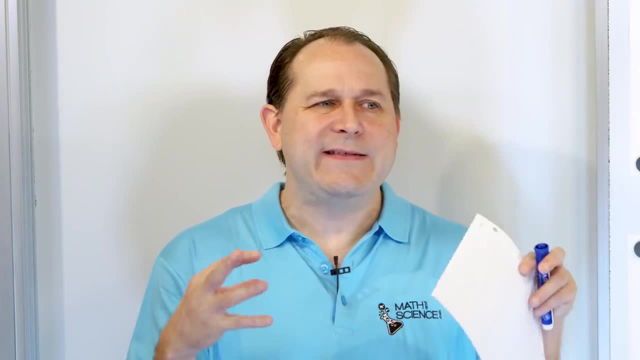 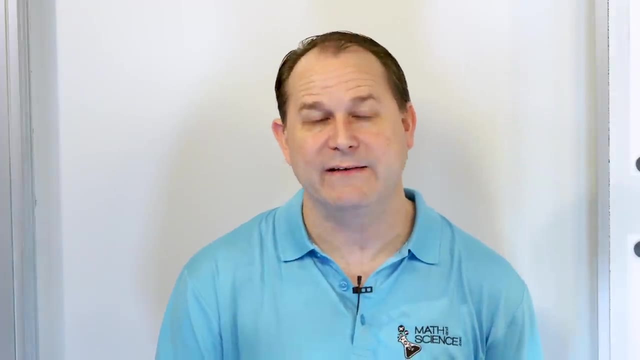 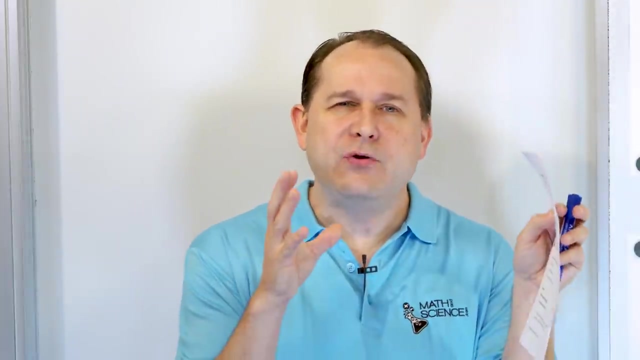 it would rain because weather is chaotic. The interactions, because we can't model every single molecule in the atmosphere. all we can look is the aggregate And we can predict, with some sort of percentage probability, What's going to happen. So the definition of probability is: if you understand what the 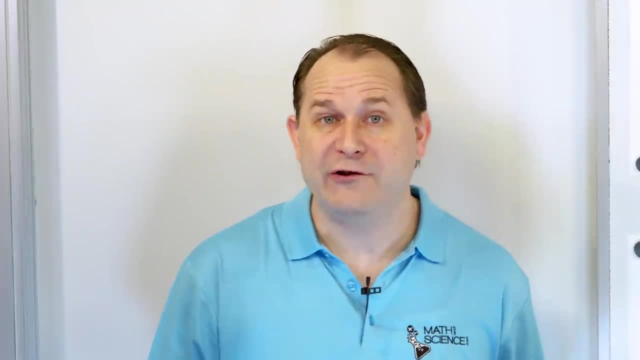 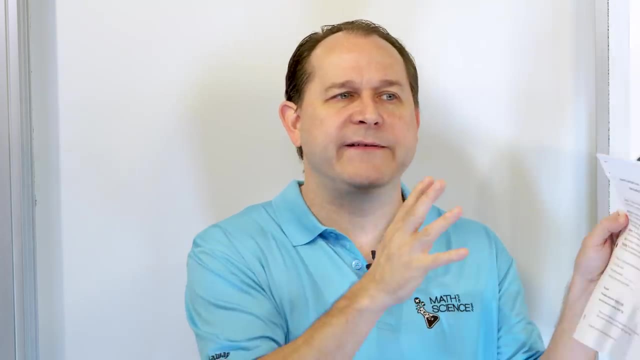 probability is as a number. if you could run that situation- we're going to call it an experiment here, in just a second We're going to define that word- But if you could think of it as an experiment where you run the days, the day, over and over and over and over again, and you ran it. 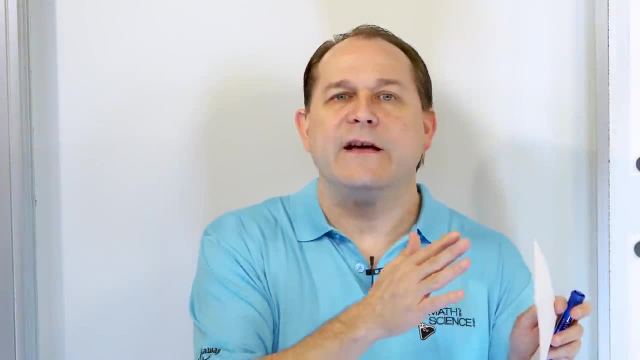 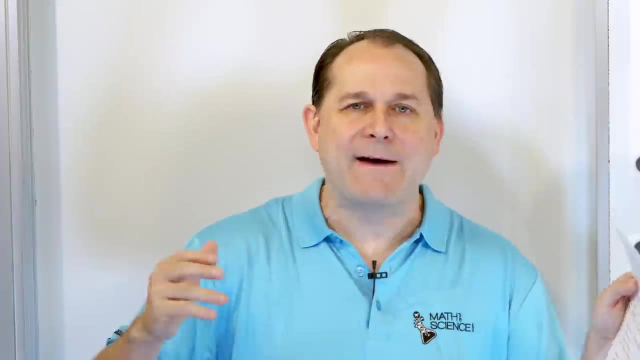 for a large number of times. then, as you run it longer and longer- number of times, approaching a million or a billion times- we run the day over and over again. then half of those days we're going to rain and the other half will not. That's what 50% chance of rain means, Of course. 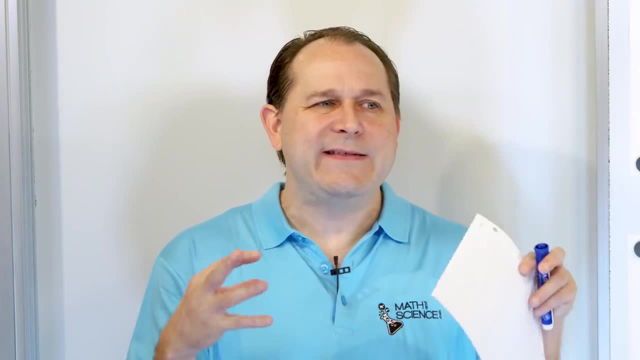 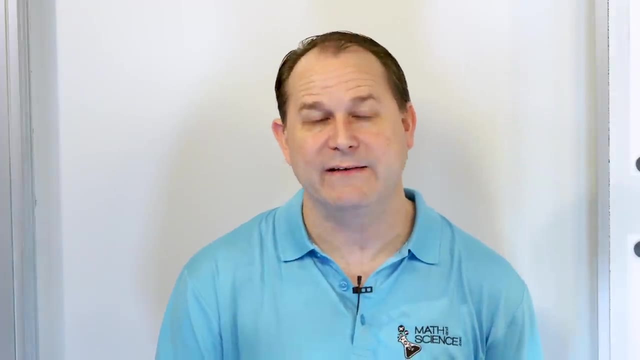 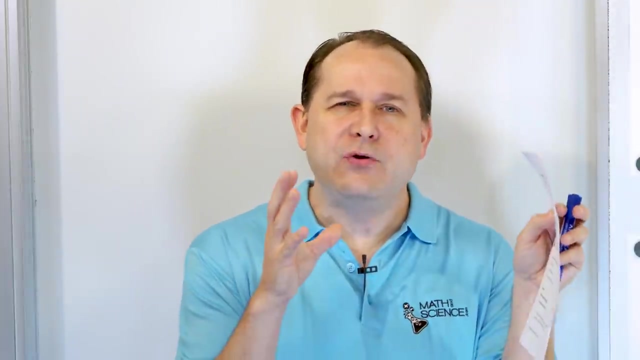 it would rain because weather is chaotic. The interactions, because we can't model every single molecule in the atmosphere. all we can look is the aggregate And we can predict, with some sort of percentage probability, What's going to happen. So the definition of probability is: if you understand what the 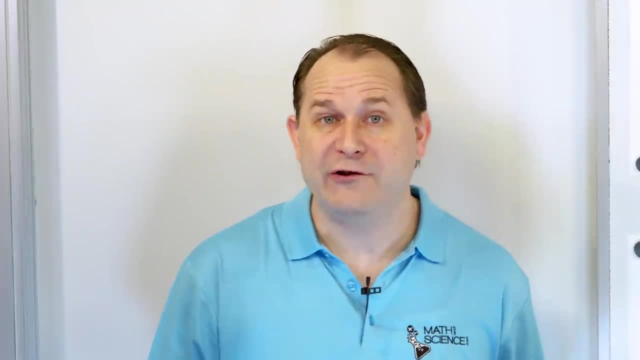 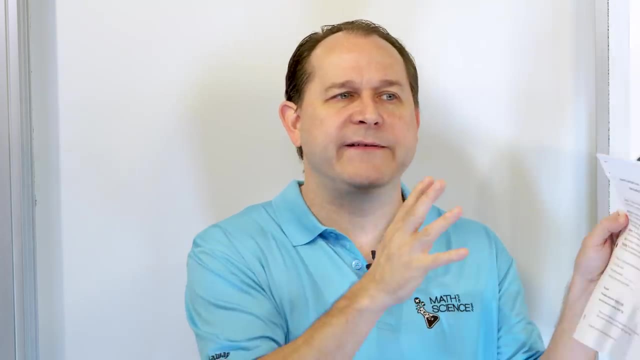 probability is as a number. if you could run that situation- we're going to call it an experiment here, in just a second we're going to define that word- But if you could think of it as an experiment where you run the days, the day, over and over and over and over again, and you ran it. 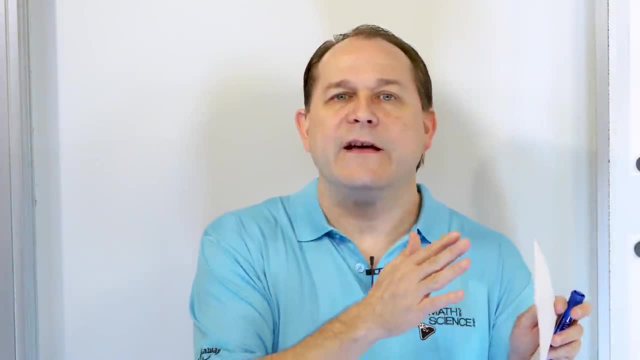 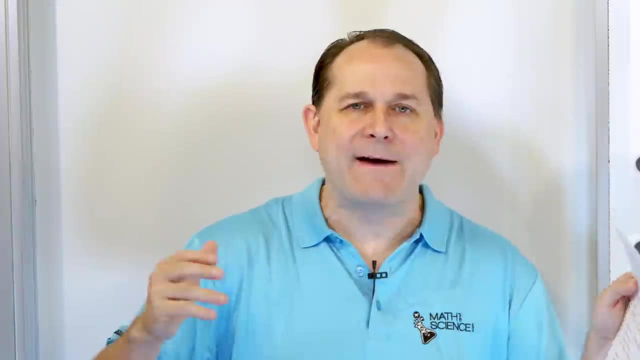 for a large number of times. then as you run it longer and longer- number of times, approaching a million or a billion times, we run the day over and over again. then half of those days, those days are going to rain and the other half will not. That's what 50% chance of rain means. 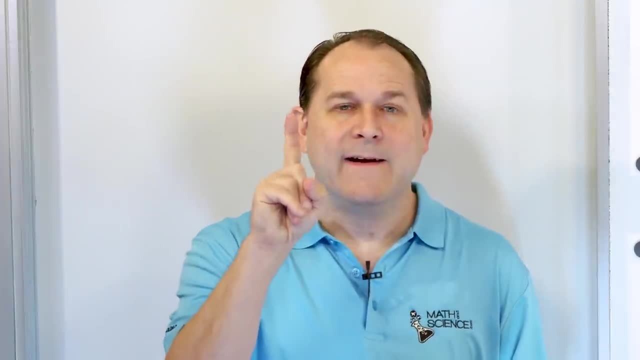 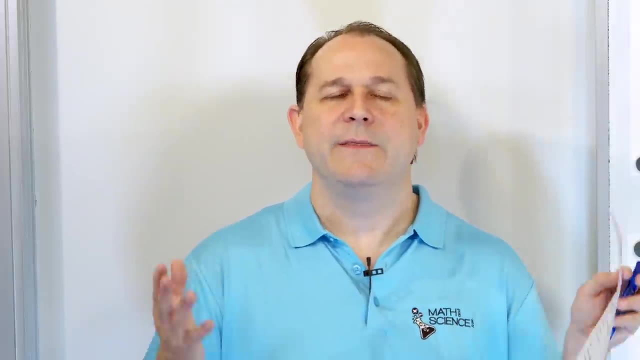 Of course, when you go out the next day and you just run one day of that weather, then of course some days it'll rain and some days it won't. But if you could run the situation a million times then it would rain half the time. If the percentage rain chance is 100%, then that would mean if I ran. 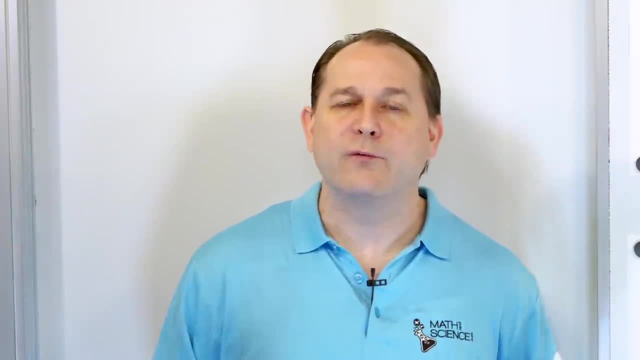 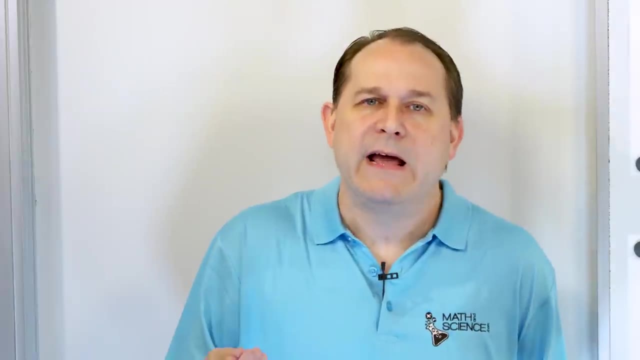 the simulation a million times. it would rain every one of those times. So that is what percentage means I want you to, uh, probability means I want you to start thinking about probability as what would happen if I could run this experiment over and over and over again for a large number of. 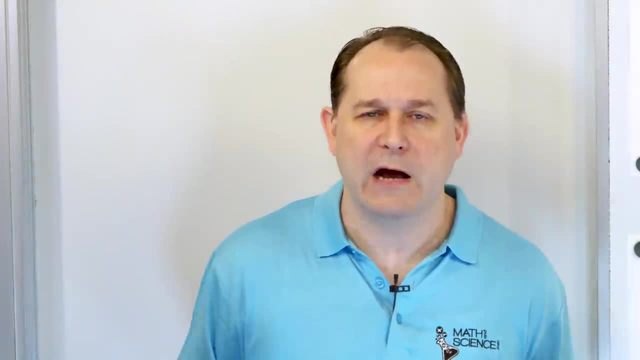 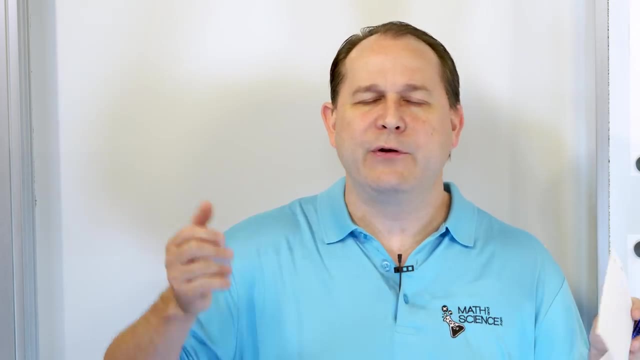 times The probability is telling you how, uh, what fraction of the time then you will get that outcome. In this case, we're talking about rain. So now we're starting to talk about experiments and what's going to happen if we do things over and over again. we need to define some terms in 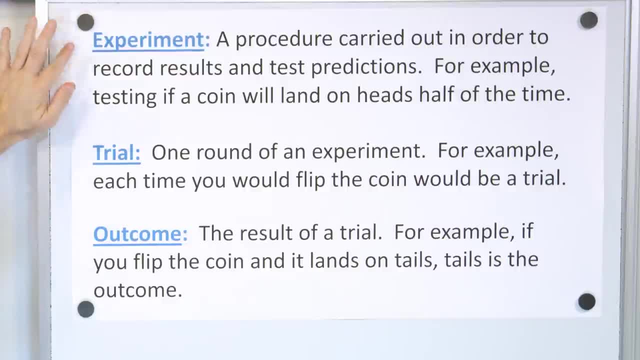 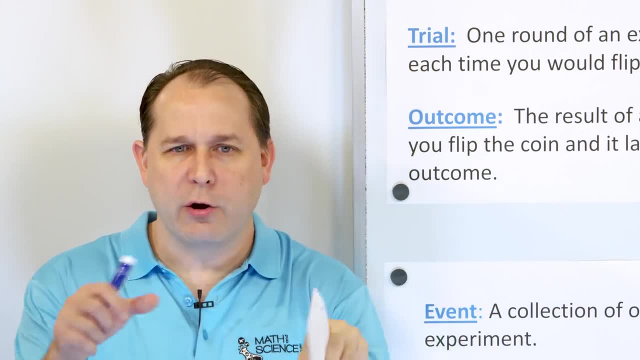 order to understand probability. So let's take a look at our first term In probability. we talk about the idea of an experiment. An experiment in science is when you go and you run the day over and you pour things in the test tube or you run, you know a generator or whatever it is you're. 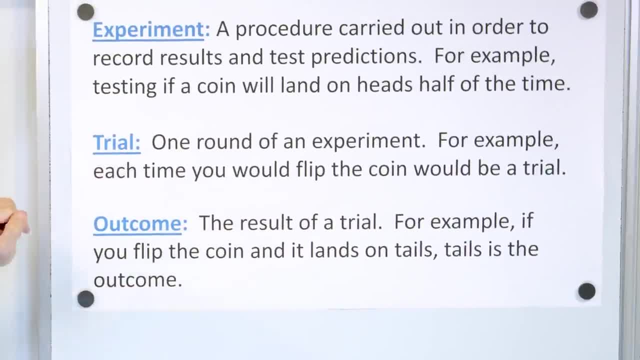 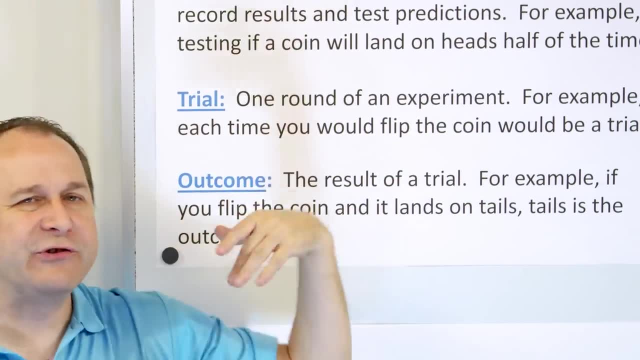 studying and you see and see what the outcome is In probability and statistics. an experiment is just a procedure carried out in order to record the results and test predictions. That's a bunch of words. It just means it's, it's, it's, uh, something that we do to see what's going to. 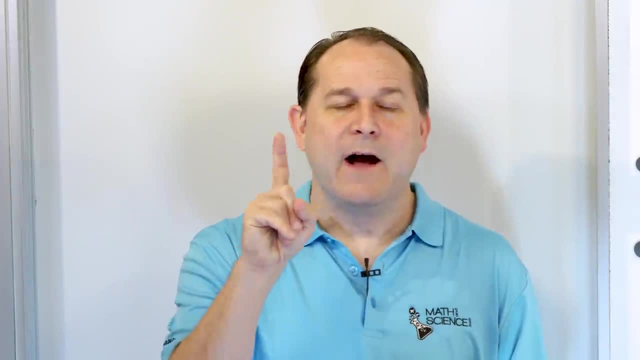 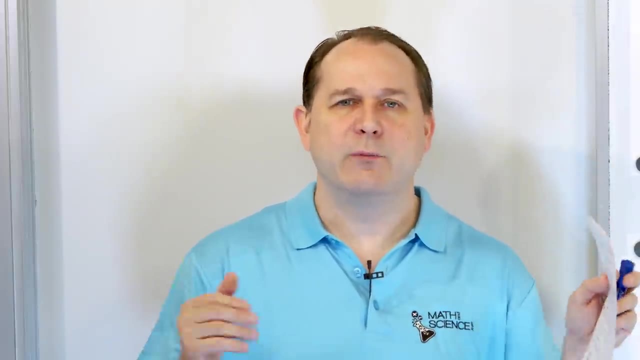 when you go out the next day and you just run one day of that weather, then of course some days it will rain and some days it won't. But if you could run the situation a million times then it would rain half the time. If the percentage rain chance is 100%, then that would mean if I ran the 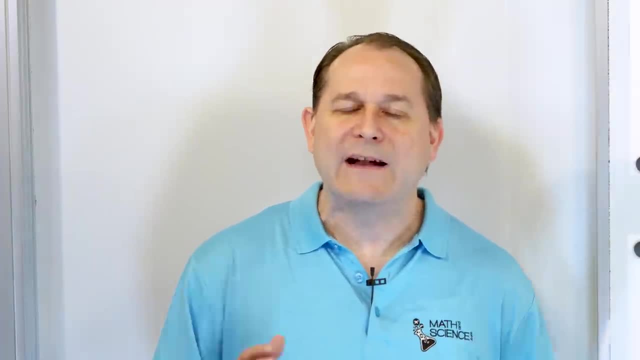 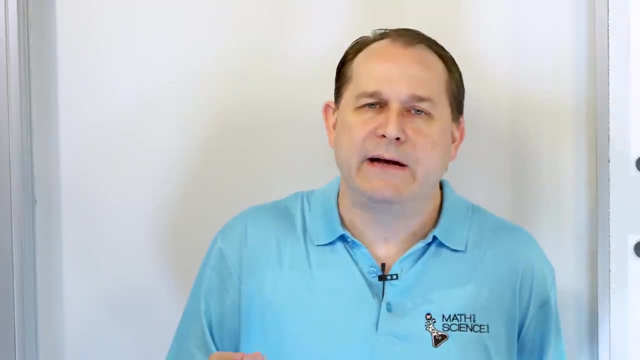 simulation a million times. it would rain every one of those times. So that is what percentage means I want you to. probability means I want you to start thinking about probability as a number. what would happen if I could run this experiment over and over and over again for a large number of? 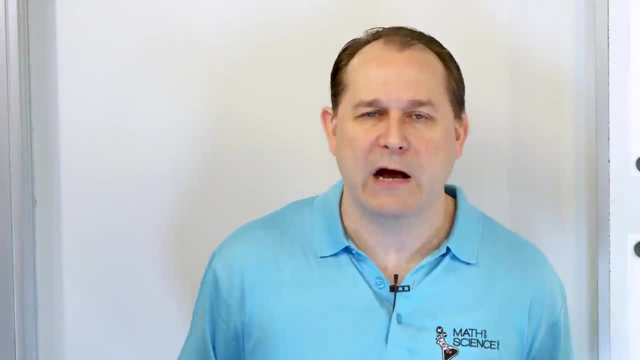 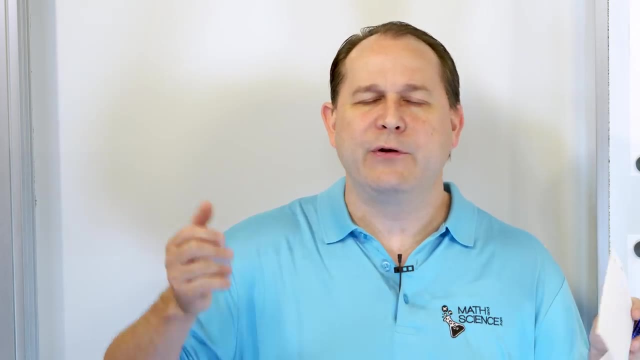 times. The probability is telling you how, what fraction of the time then you will get that outcome. In this case, we're talking about rain. So now we're starting to talk about experiments and what's going to happen if we do things over and over again. We need to define some terms in 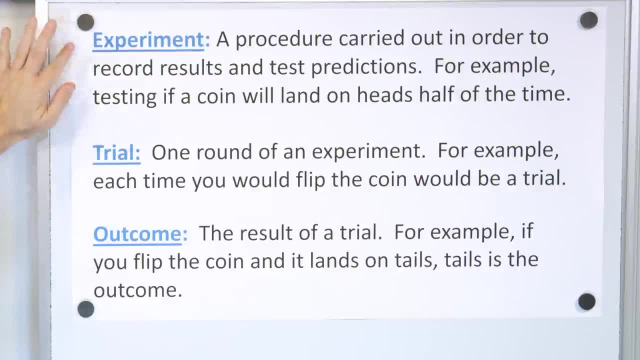 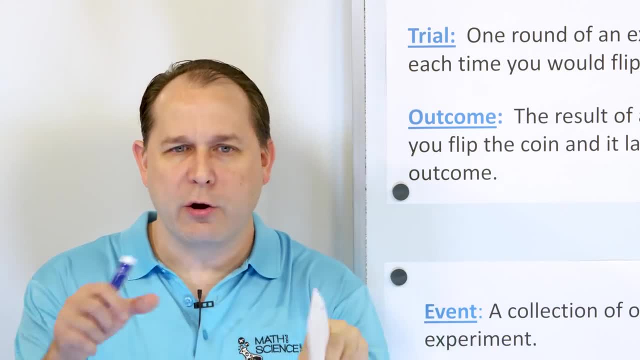 order to understand probability. So let's take a look at our first term. In probability, we talk about the idea of an experiment. An experiment in science is when you go and you run the day over and you go and you pour things in the test tube or you run a generator or whatever it is you're studying. 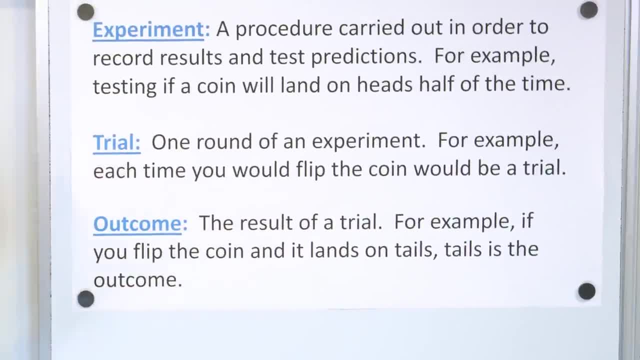 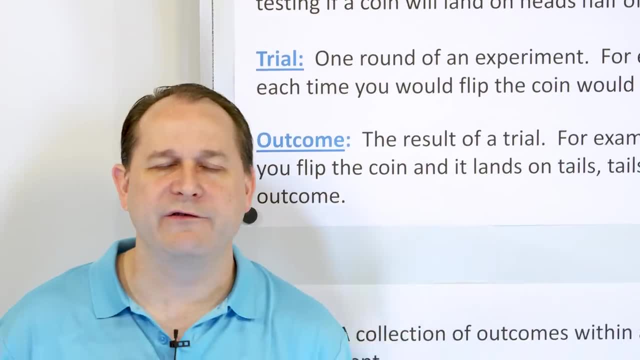 and you see what the outcome is. In probability and statistics. an experiment is just a procedure carried out in order to record the results and test predictions. That's a bunch of words. It just means it's something that we do to see what's going to happen, like flipping a coin. 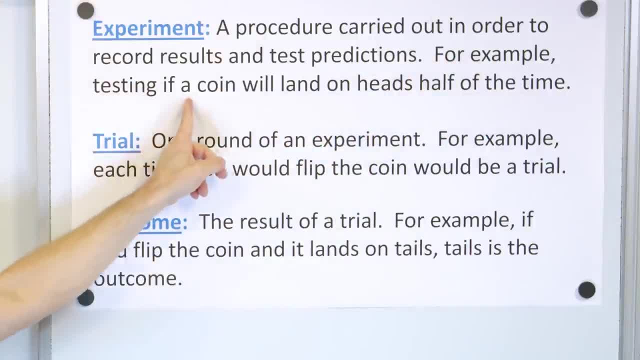 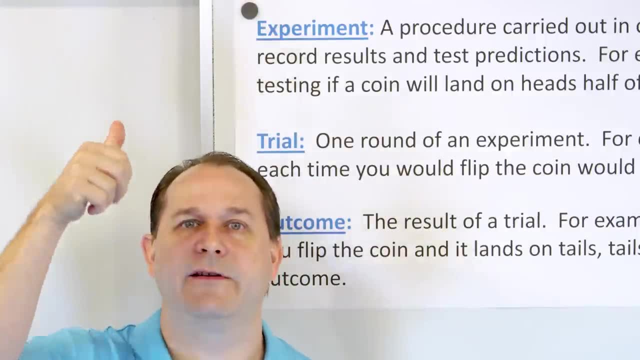 or drawing cards, For example, testing if a coin will land on heads or tails. So an experiment is when I would flip one of these coins. That's an experiment. Here's another one. That's an experiment Here, flipping it again. That's an experiment Every time you do it. 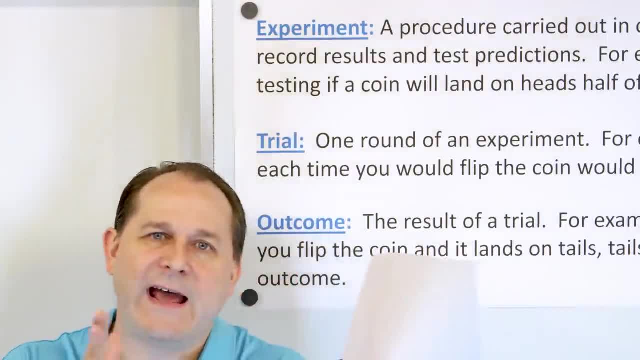 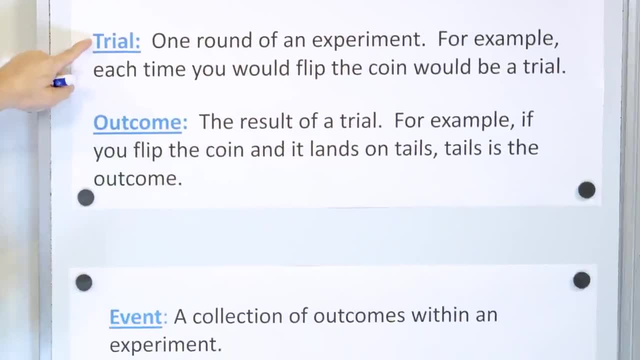 that's an experiment In our weather example, every time we run the day. if we could run the day over and over again- which we couldn't, but if we could every day- would be an experiment. Now, the trial is just one round of an experiment, So basically an experiment. I guess a better way. 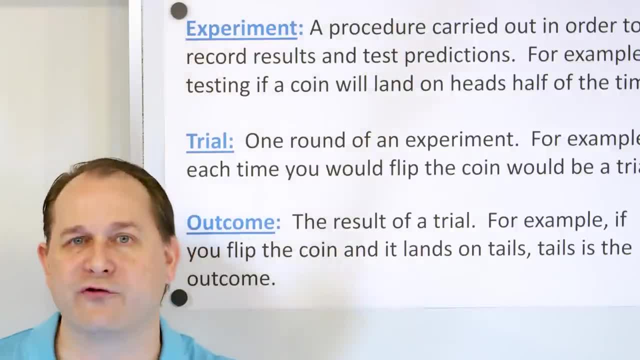 of saying it is an experiment is how many times you're going to run the trial. I should say An experiment is, let's say, I'm going to flip a coin 10 times. That's a better example. A trial is 10 times, That's a better example. A trial is 10 times, That's a better example. A trial is 10. 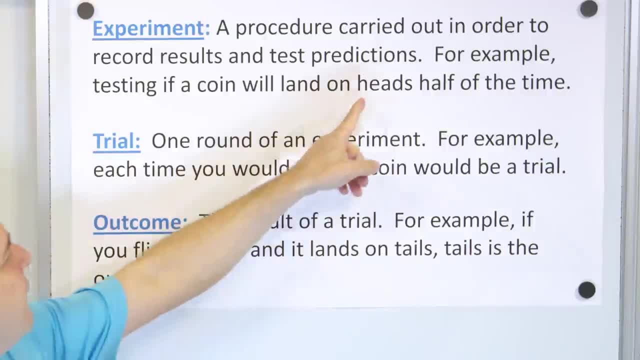 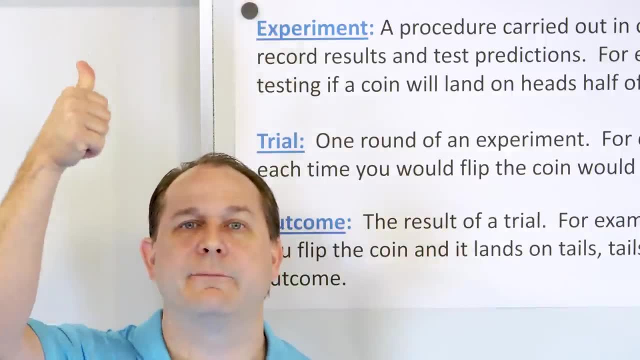 happen at, like flipping a coin or drawing cards, For example, testing if a coin will land on heads or tails. So an experiment is when I would flip one of these coins. That's an experiment. Here's another one. That's an experiment. here I'm flipping it again. That's an experiment Every time you do it. 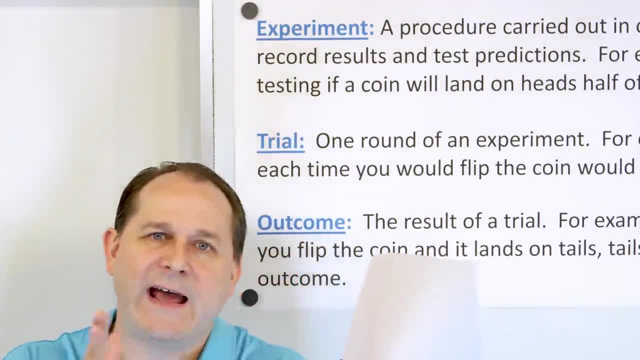 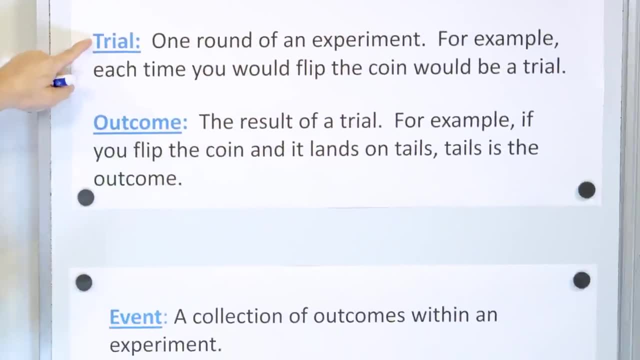 that's an experiment in our weather example, Every time we run the day. if we could run the day over and over again- which we couldn't, but if we could every day- would be an experiment. Now, the trial is just one round of an experiment. So so, basically an experiment, I guess a better way of. 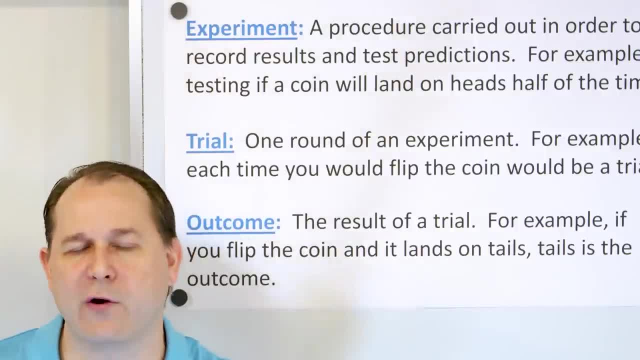 saying it is an experiment is how many times you're you're going to run the trial. I should say an experiment is, let's say, I'm going to flip a coin 10 times. That's a better example. A trial is every single time I flip the coin and the entire experiment is all of the times that I flip. 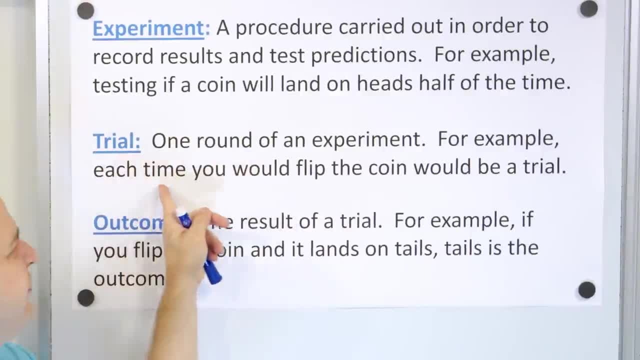 the coin. uh, together there, All right. So, for example, each time I would flip the coin would be a trial. So I guess a better way of saying it is: when I flip the coin, that's a trial, that's a trial, that's a trial. But my entire experiment might be what would happen if I flip. 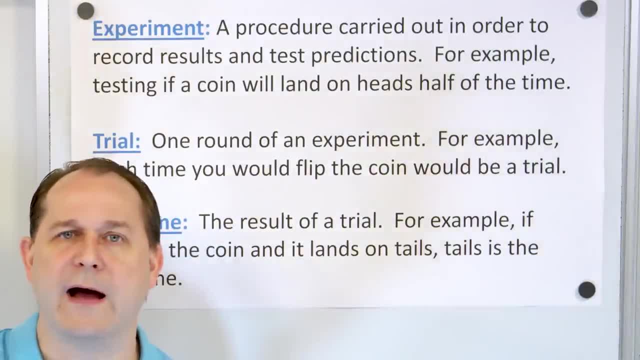 a coin 10 times. I have 10 trials: one, two, three, four, five, six, seven, eight, nine, 10 and so on. Now the outcome is the result of a trial. So every time I flip that coin and it lands. 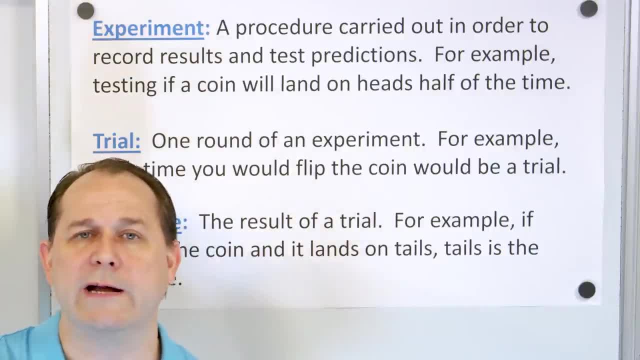 tails, tails is the outcome. So here we go. Trial number one: I flip it: heads, heads is the outcome. right, Outcome is the result of a trial. Trial number two: I flip it again: Heads, heads comes out. Trial number three: heads, heads comes out. Trial number four: tails. That's the outcome. 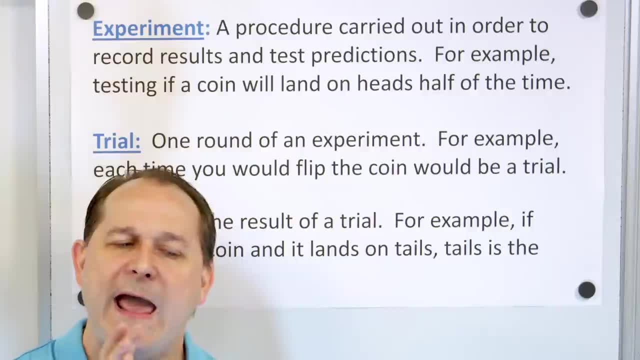 outcome for trial number four. So every time I flip it that's a trial And whatever I see that happens at the outcome of that trial is called the outcome. And when you put all the trials together you know maybe I'm going to flip the coin 20 times. I'm going to flip the coin 20. 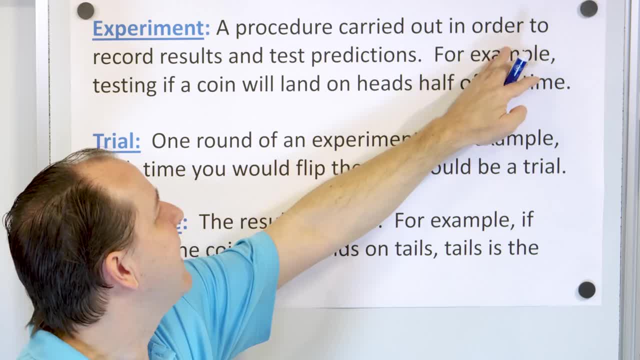 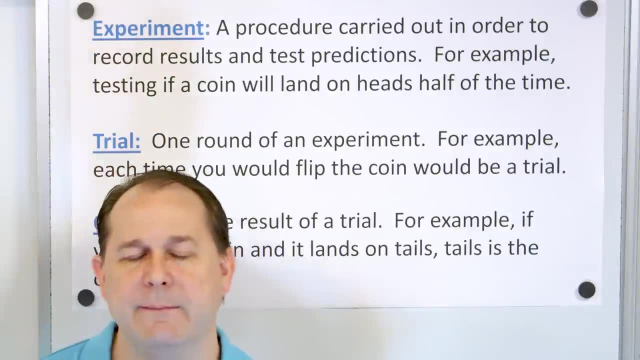 times. The entire thing is called an experiment, a procedure carried out in order to record results and test predictions, For example, testing if a coin will land heads or tails half of the time. So maybe I test it by flipping the thing 10 times and see what would happen. I generally expect it. 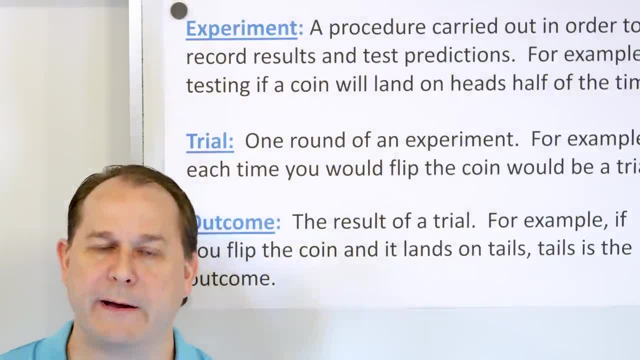 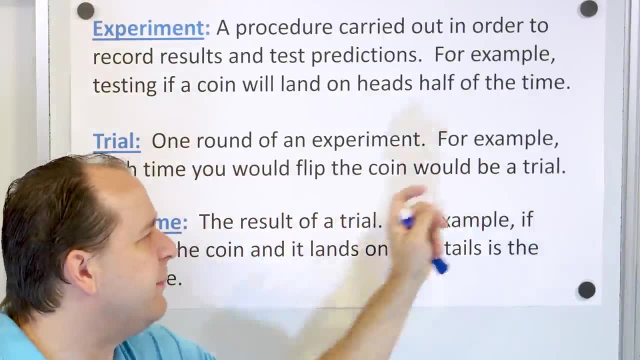 times, Every single time I flip the coin, and the entire experiment is all of the times that I flip the coin together there. So, for example, each time I would flip the coin would be a trial. So I guess a better way of saying it is: when I flip the coin, that's a trial, That's a trial, That's a trial. 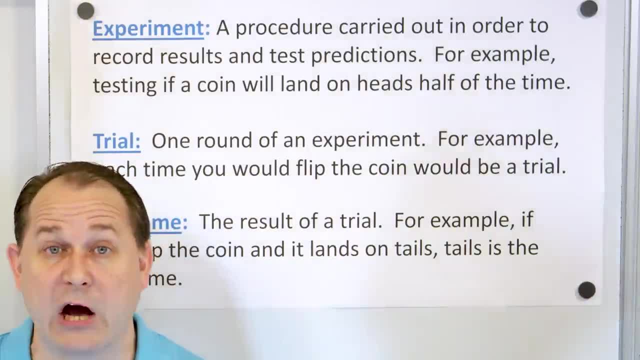 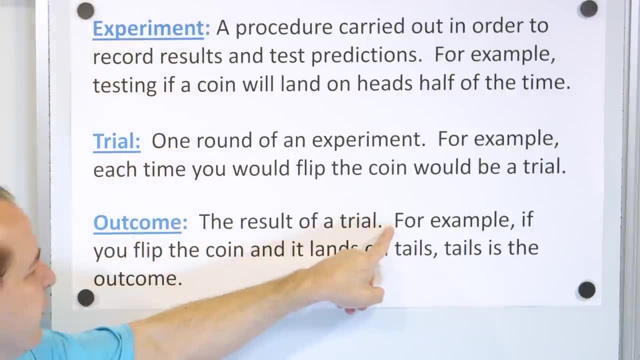 But my entire experiment might be what would happen if I flip a coin 10 times. I have 10 trials: 1,, 2,, 3, 4,, 5,, 6,, 7,, 8,, 9,, 10, and so on. Now the outcome is the result of a trial, So 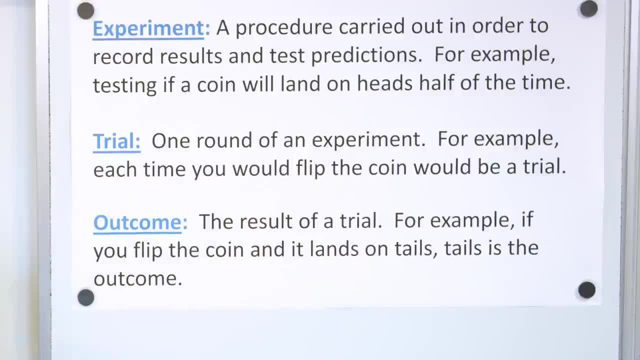 every time I flip that coin and it lands on tails is the outcome. So here we go. Trial number one: I flip it heads. Heads is the outcome. right Outcome is the result of a trial. Trial number two: I flip it again. heads comes out. 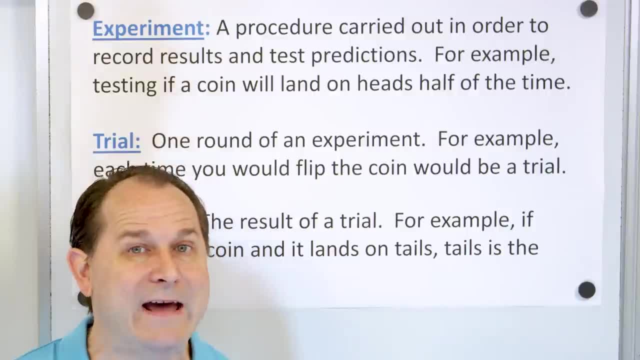 Trial number three: heads- Heads comes out. Trial number four: tails. That's the outcome for trial number four. So every time I flip it that's a trial And whatever I see that happens at the outcome of that trial is called the outcome. And when you put all the trials together, 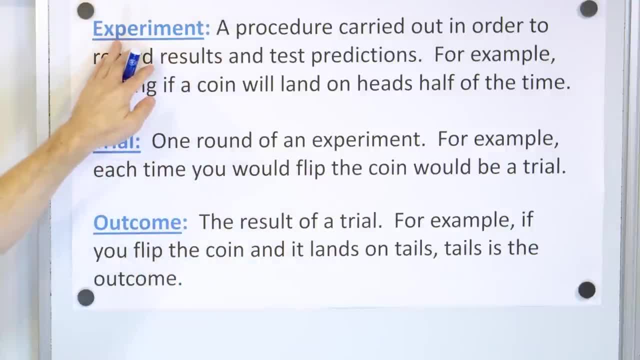 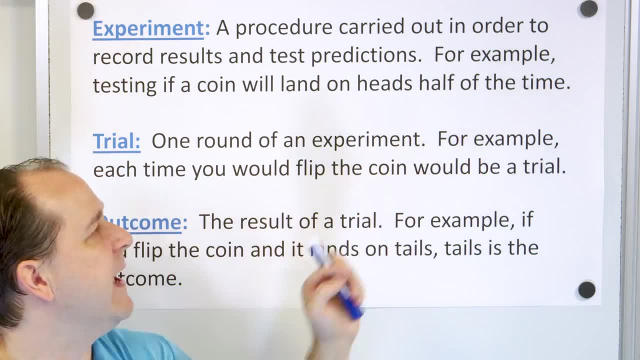 you know, maybe I'm going to flip the coin 20 times. the entire thing is called an experiment, a procedure carried out in order to record results and test predictions, For example, testing if a coin will land, heads or tails half of the. 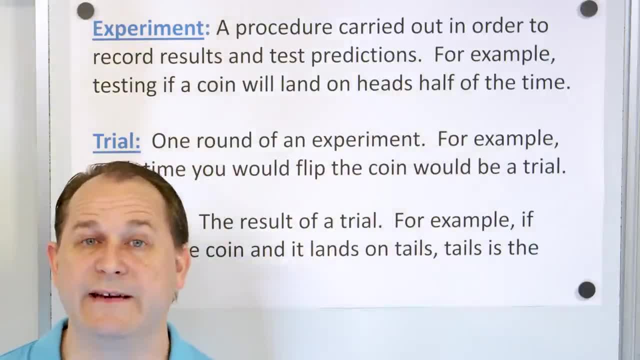 time, So maybe I test it by flipping the thing 10 times and see what would happen. I generally expect it to land half the time on heads and half the time on tails. We're going to talk about a lot more why that is the case later. All right, Now let's talk about the idea of an event. 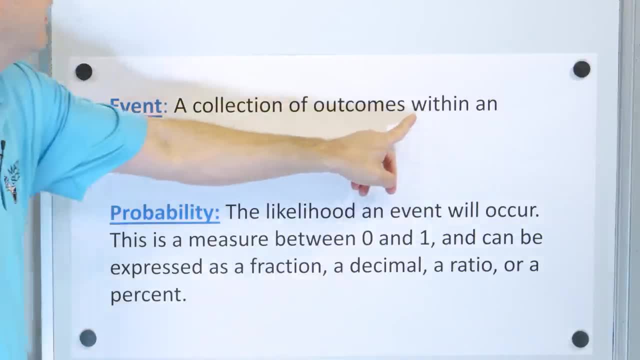 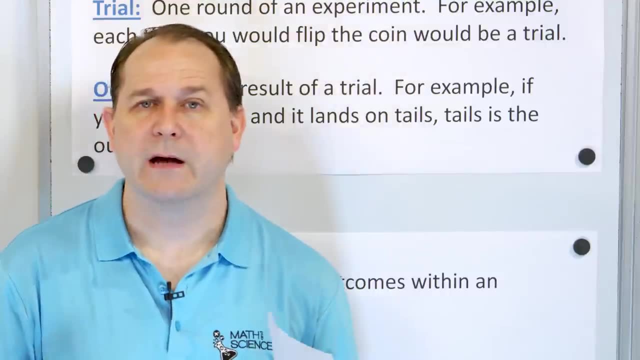 This one can seem a little bit confusing at first. An event is a collection of outcomes within an experiment. All right, So let's say I flip, you know, the first three times, I flip the coin. I'm going to flip them 10 times. That's the entire experiment And the event is a collection. 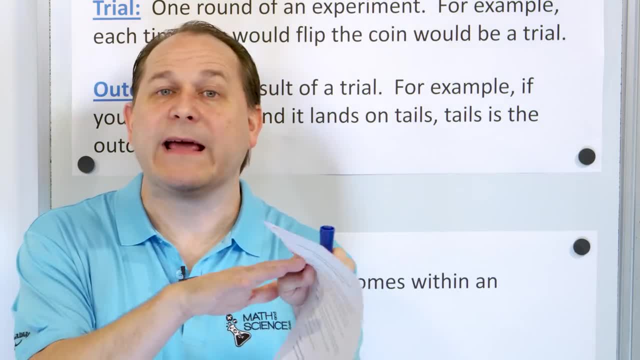 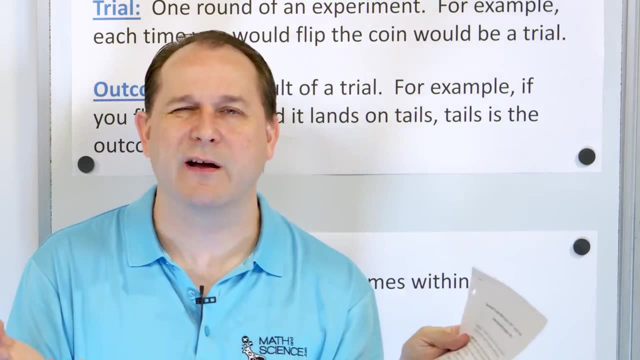 of outcomes. So maybe I could say an event would be: I get five heads in a row, or I could get six heads in a row, or I get three heads and two tails. Any collection of outcomes is just called an event. We just have a word for that. If you talk about the entire experiment and I come and I tell you, 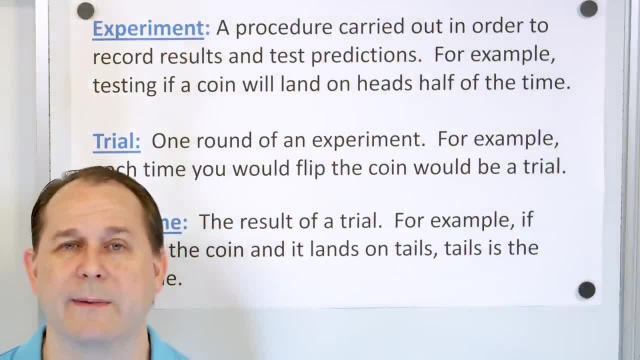 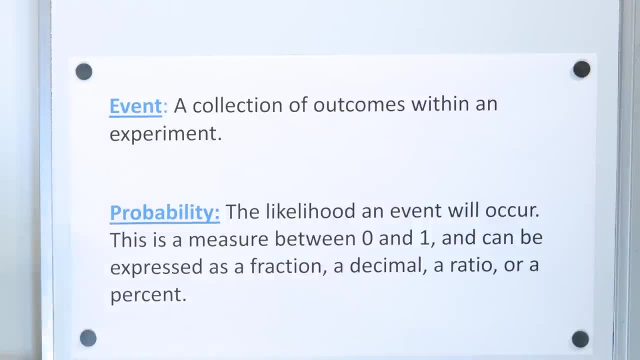 to land half the time on heads and half the time on tails. We're going to talk about a lot more why that is the case later. All right, Now let's talk about the idea of an event. This one can seem a little bit confusing at first. An event is a collection of outcomes. 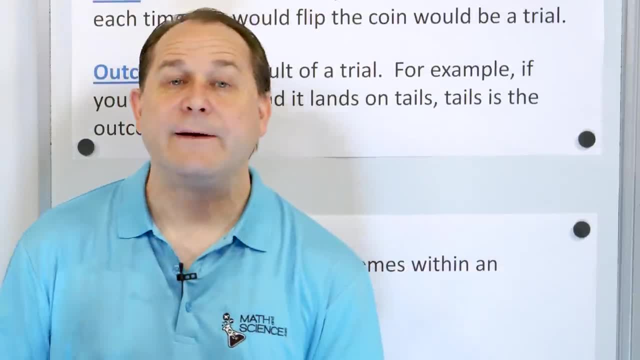 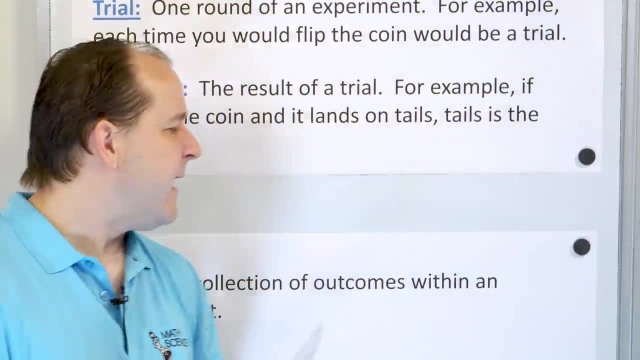 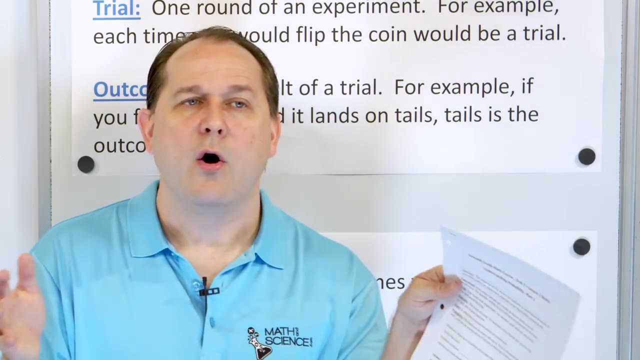 Within an experiment. All right, So let's say, I flip, you know, the first three times I flip the coin. I'm going to flip them 10 times. That's the entire experiment And the event is a collection of outcomes. So maybe I could say an event would be: I get five heads in a row, or I could get six. 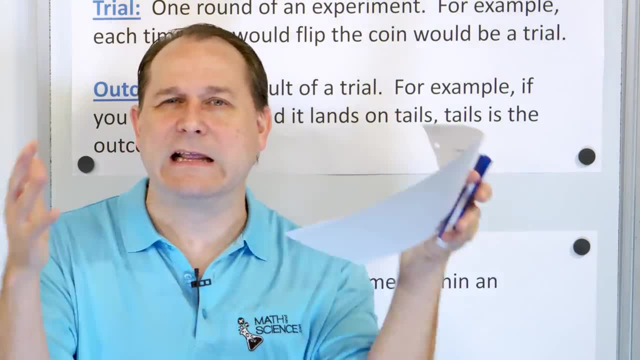 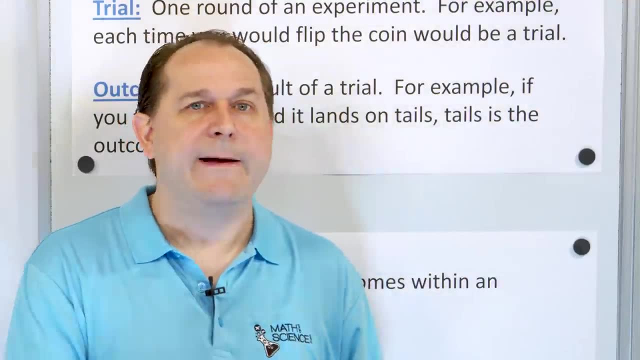 heads in a row, or I get three, three heads and two tails. Any collection of outcomes is just called an event. We just have a word for that. If you talk about the entire experiment and I come and I tell you: Hey, I actually got 10 heads in a row, I'm going to flip the coin 10 times, That's. 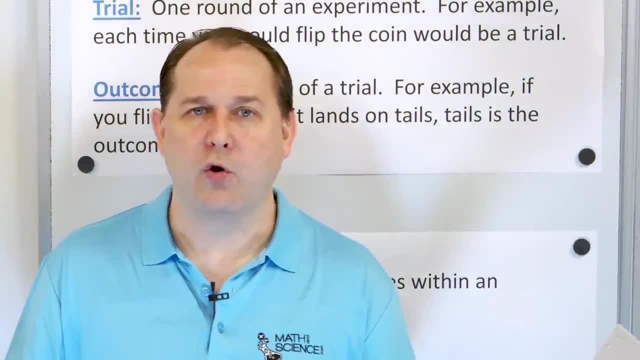 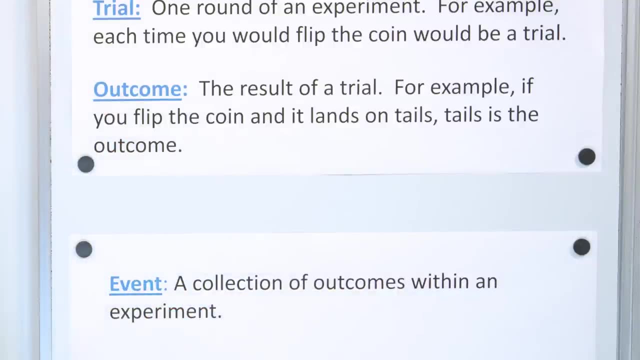 going to be 10 heads in a row. The entire experiment is flipping all the coins to see what's going to happen, And the event is the collection of outcomes that I got: 10, 10 in a row, basically All right. Now, here is where we make our money. here, Probability is the likelihood. 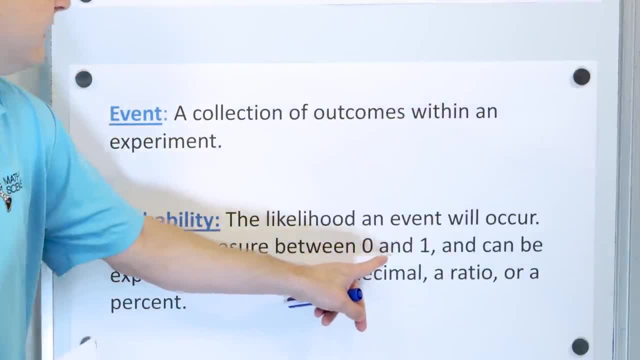 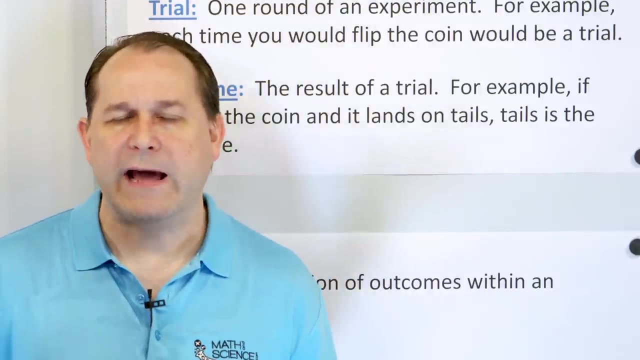 an event will occur. This is a measure between zero and one- We'll talk about that in a minute- and can be expressed as a fraction, a decimal, a ratio or a percent Probability. That is the. that is what we really have to understand here. So when you're looking at the weather forecast, 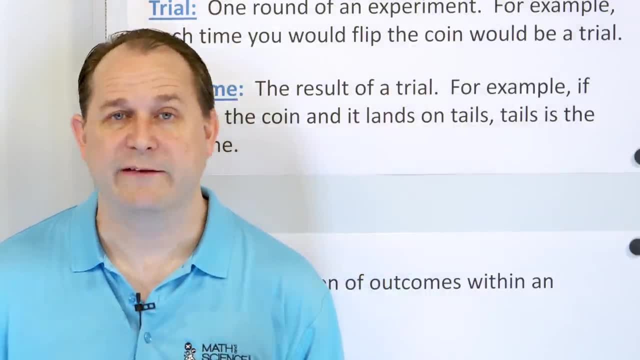 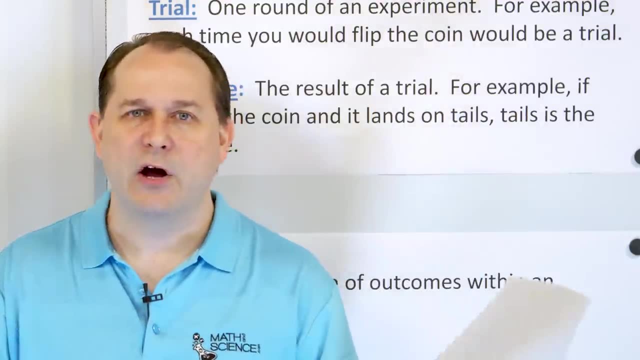 they always tell you in percentages, it's going to rain, 10% chance of rain tomorrow. You know that that means 10 out of a hundred times, because that's what a percent is: 10%, 10 out of a hundred. 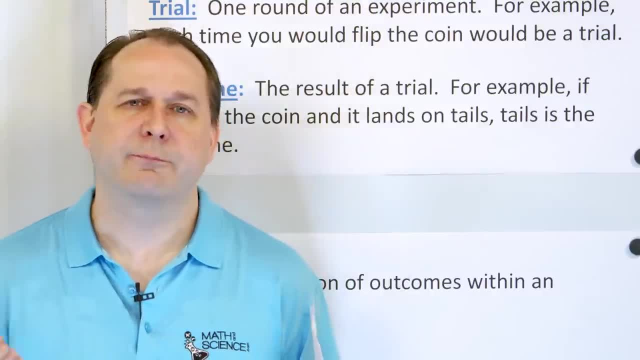 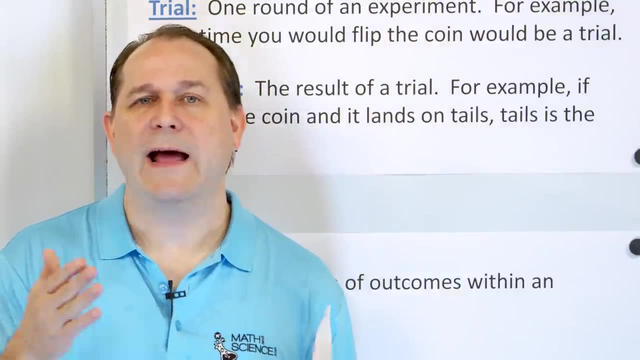 That's what that means, right? But in probability, usually we express the probability as a fraction right- 10 out of a hundred, That's a fraction right. Or we express it as a decimal, and the decimal is really going to go between zero and one. So we're going to express the probability as a 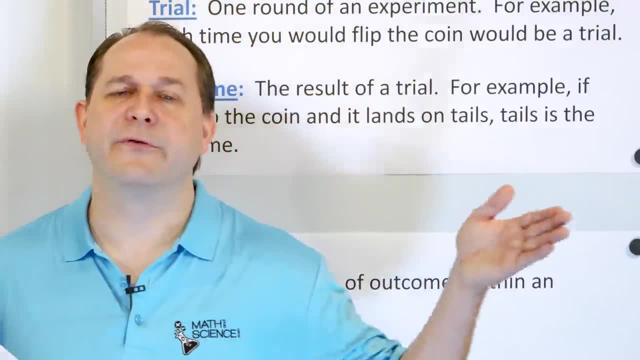 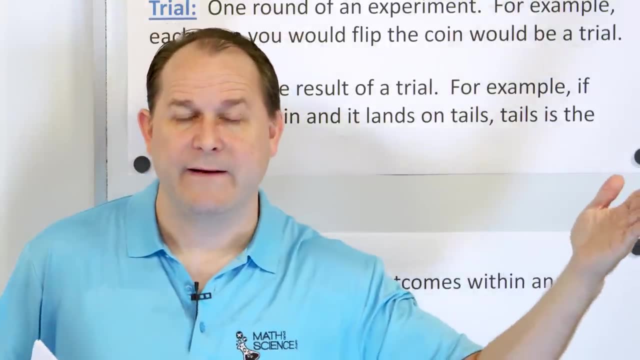 fraction. So instead of saying 50%, I might give you the decimal 0.5.. Zero is the, the no probability at all, And one is like a hundred percent, and 0.5 is right in the middle at 50%. So I can express. 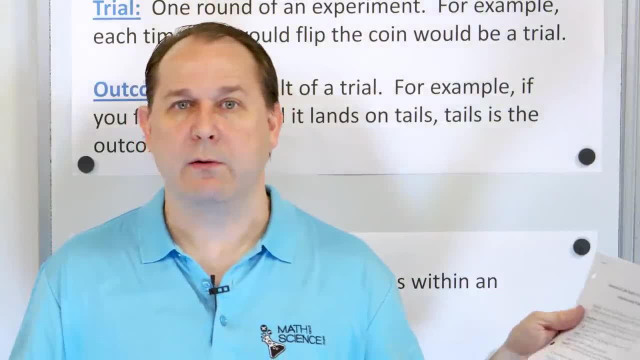 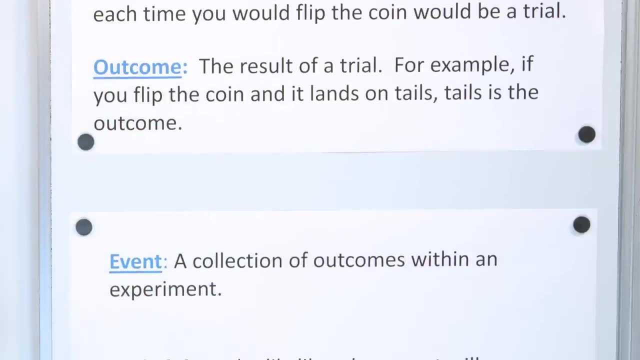 I got five heads in a row. the entire experiment is flipping all the coins to see what's going to happen, And the event is the collection of outcomes that I got 10, 10 in a row. basically All right. Now here is where we make our money here, Probability is the likelihood an event will. 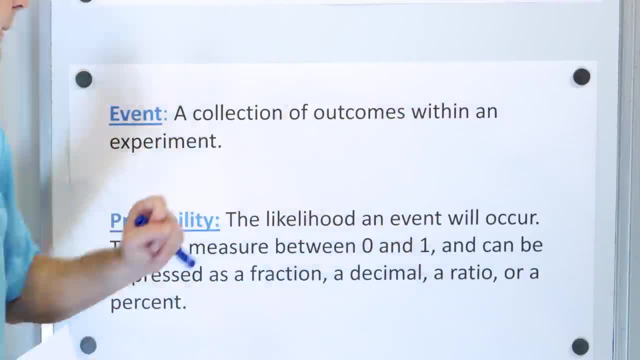 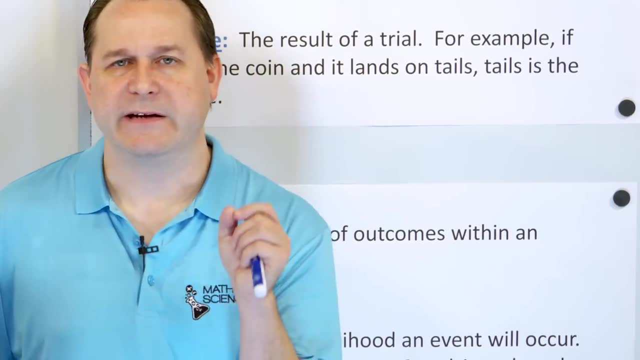 occur. This is a measure between zero and one- We'll talk about that in a minute- and can be expressed as a fraction, a decimal, a ratio or a percent Probability. That is the. that is what we really have to understand here. 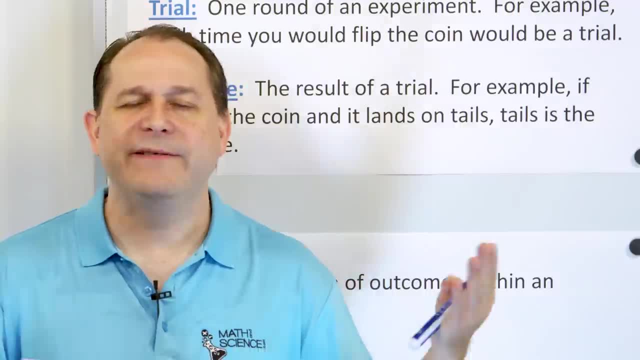 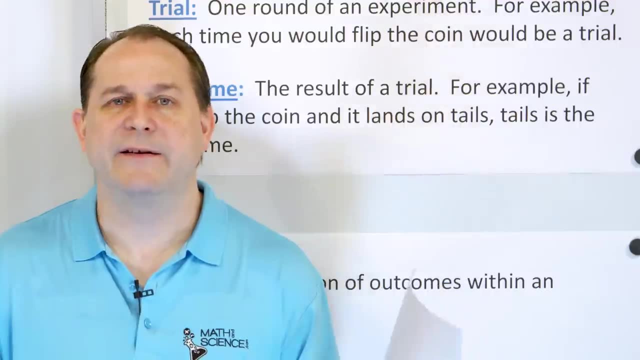 So when you're looking at the weather forecast, they always tell you in percentages: it's going to rain: 10% chance of rain tomorrow. You know that that means 10 out of a hundred times, because that's what a percent is: 10%, 10 out of a hundred. That's what that means. right, But in probability. 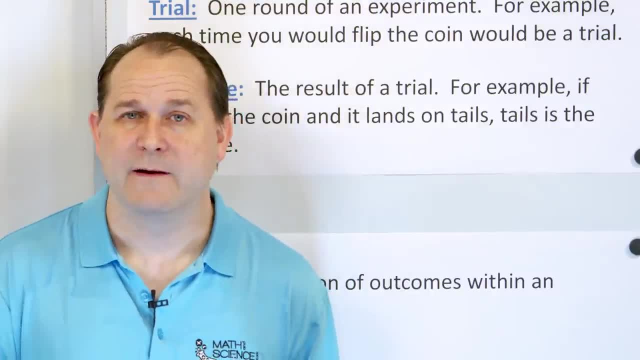 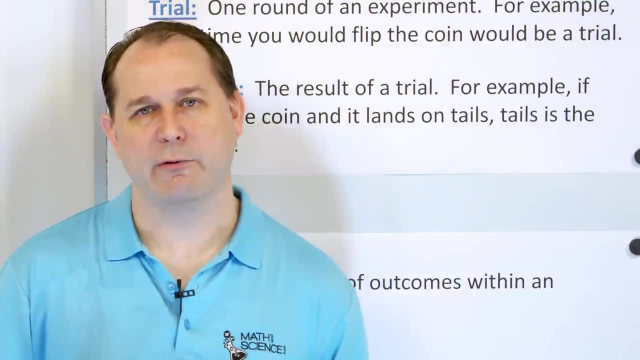 usually we express the probability as a fraction right- 10 out of a hundred, that's a fraction right. Or we express it as a decimal, and the decimal is really going to go between zero and one. So instead of saying 50%. 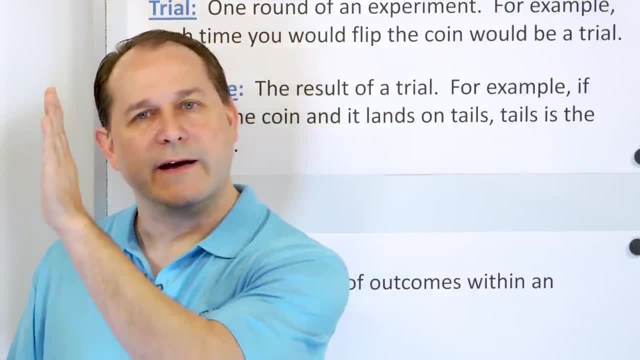 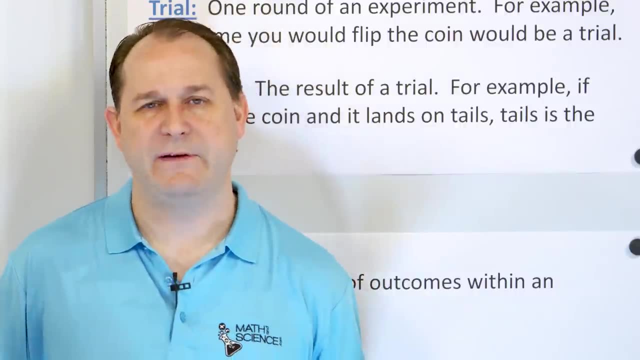 I might give you the decimal 0.5.. Zero is the, the no probability at all, And one is like a hundred percent and 0.5 is right in the middle at 50%. So I can express any percentage as a decimal. I just 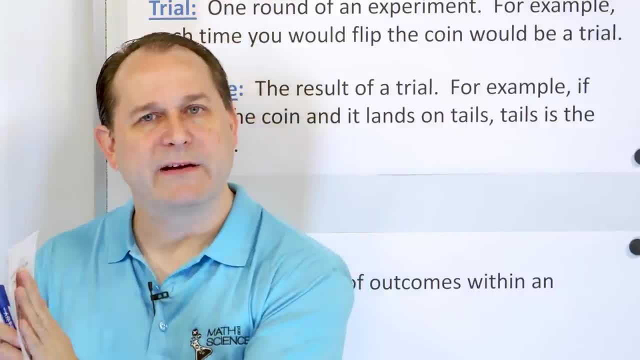 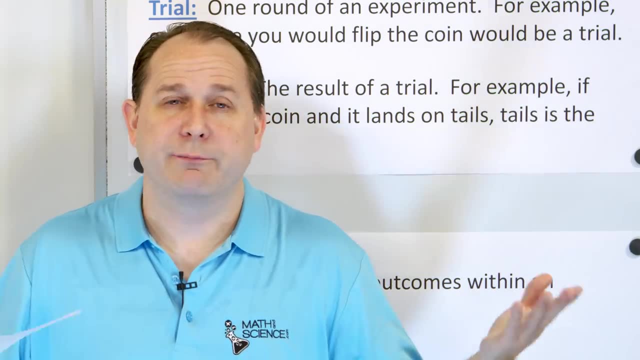 move the decimal point back, And so that the range of probability will be between zero and one, And the probability in terms of a percent will be between zero and a hundred percent. So, or you can express it as a fraction: One half is the same as 0.5, but that's also the same as 50%. So that's. 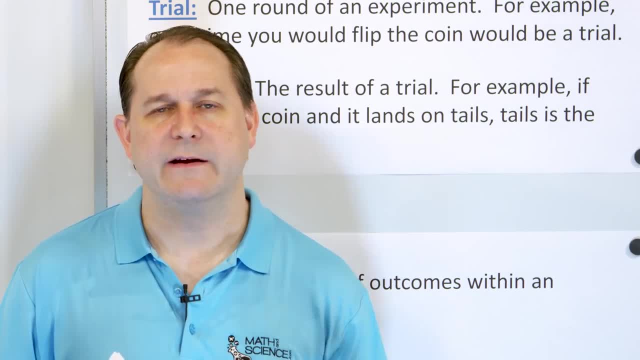 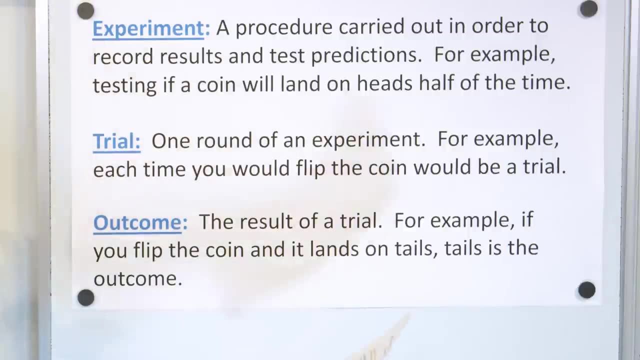 50%, So you can express these probabilities in different ways. So, from the top, an experiment is just something I'm going to test, where I'm going to basically perform multiple trials of an experiment to see what happens. For instance, I have a sock drawer, I have some blue socks and 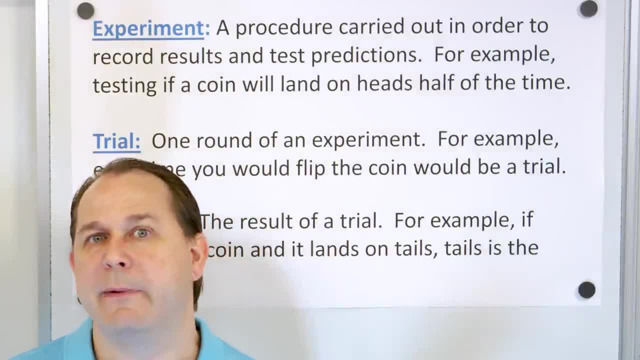 some orange socks and I know how many of each I have And the experiment might be- I'm going to pull, you know 50 socks out of the drawer. How many do I expect to get? And so I'm going to test. 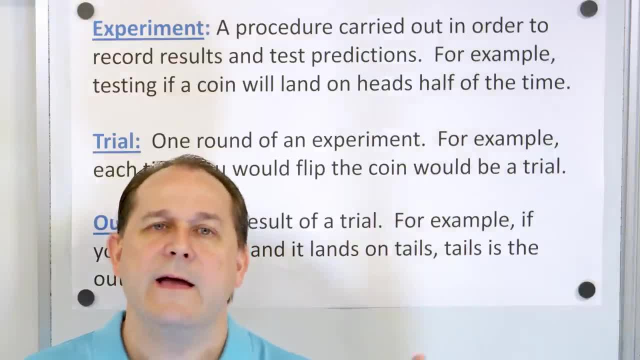 that experiment by performing trials of an experiment. And by trials I mean I do something and then measure the outcome. So the trial could be that I take one sock out of the drawer and see what I get, And I take another sock out of the drawer and 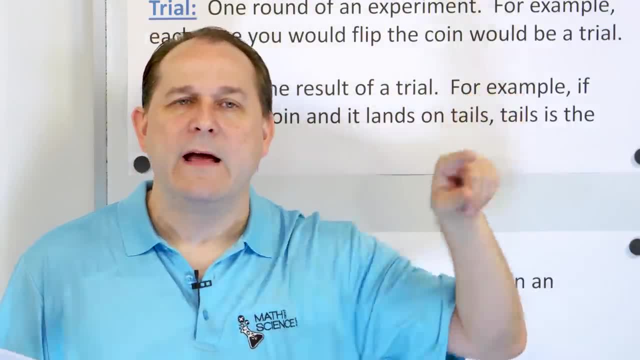 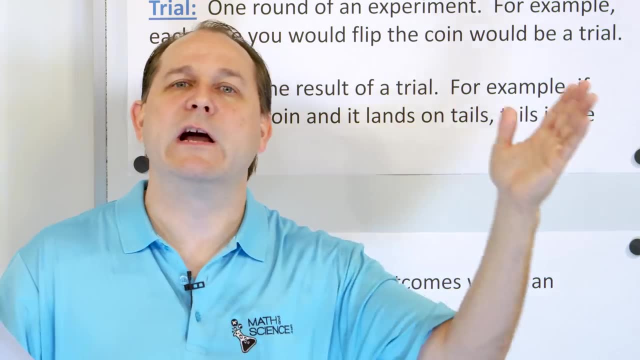 any percentage as a decimal. I just move the decimal point back And so that the range of probability will be between zero and one, And the probability in terms of a percent will be between zero and a hundred percent. So or you can express it as a fraction: One half is the same as zero. 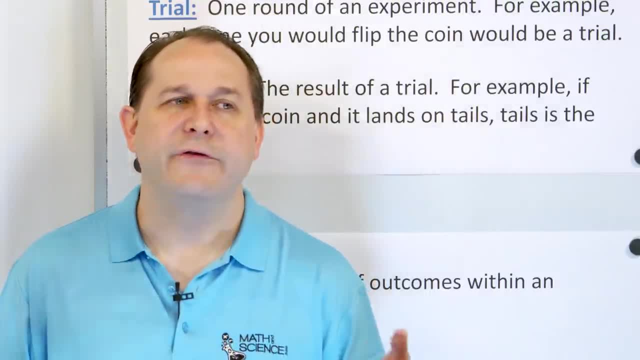 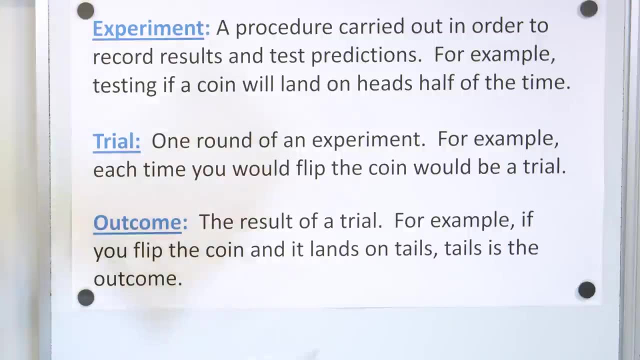 point five, but that's also the same as 50%, So you can express these probabilities in different ways. So, from the top, an experiment is just something I'm going to test, where I'm going to basically perform multiple trials of an experiment to see what happens. For instance, I have a sock. 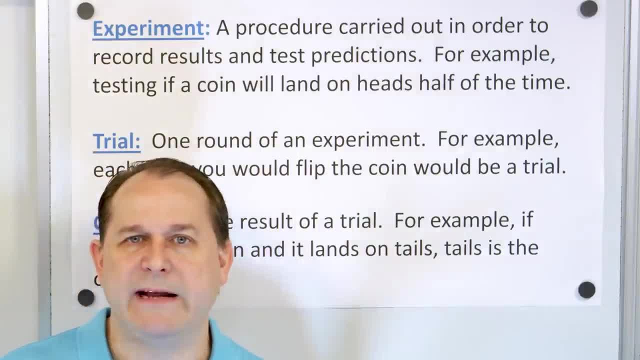 drawer. I have some blue socks and some orange socks, and I know how many of each I have And the experiment might be: I'm going to pull, you know, 50 socks out of the drawer. How many do I expect to get? And so I'm going to test that experiment by performing trials. 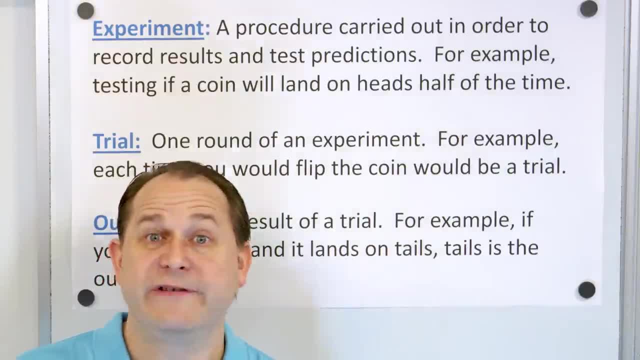 of an experiment, And by trials I mean I do something and then measure the outcome. So the trial could be that I take one sock out of the drawer and see what I get, And I take another sock out of the drawer and see what I get. In every single trial I get an outcome, So I do a. 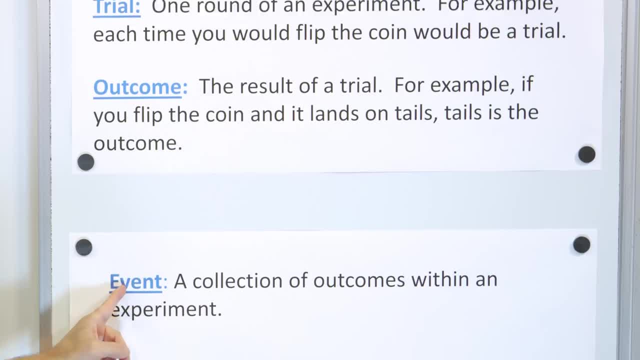 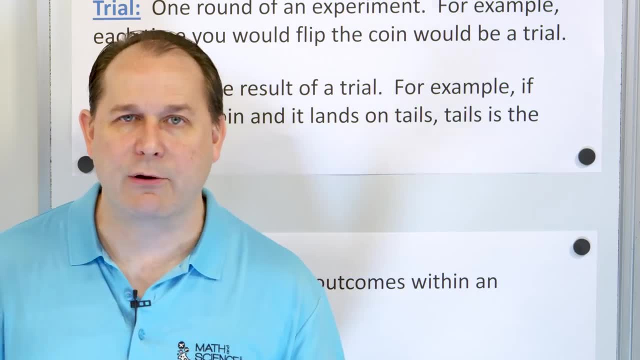 trial of an experiment and I get an outcome, And an event is a collection of outcomes. So maybe I observe that I get five red socks in a row. That could be an event, right, It's a collection of outcomes. that are trials of an experiment, right? And from all of that information I can then 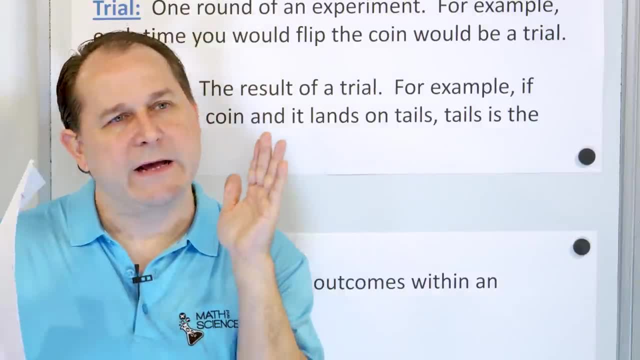 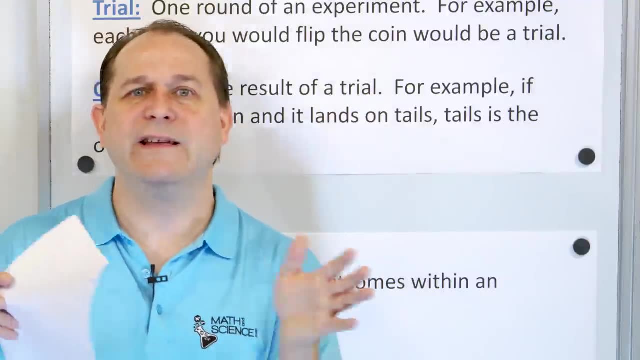 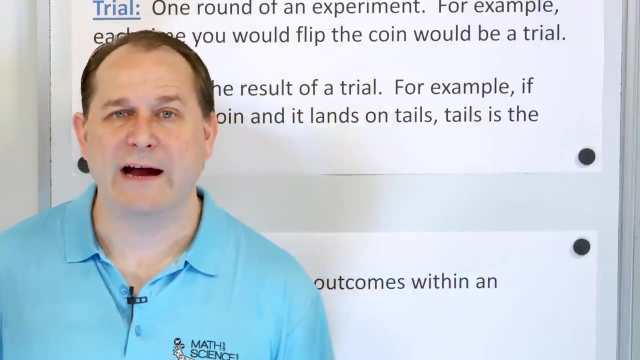 calculate a probability. I can either calculate a probability ahead of time and then check my experiment against the probability, or I could use the data I get to calculate the probability. You get the idea. So I might say that in my sock drawer there's a 35% chance of getting a red sock. 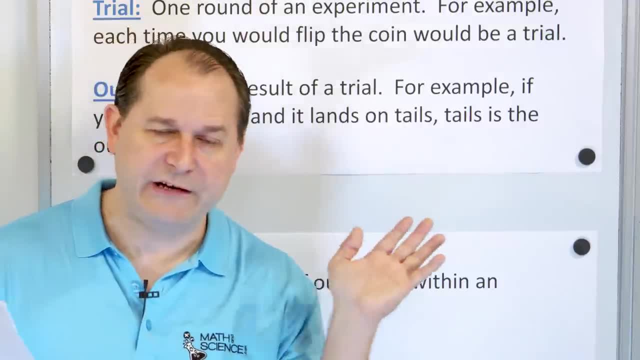 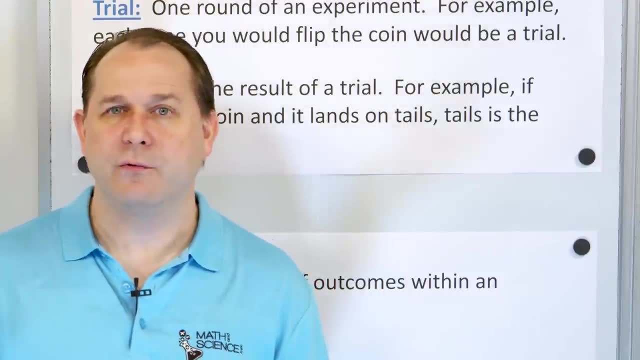 on any given draw, because I'm going to teach you how to calculate the probability and what that means. Thirty-five percent means that less than half of the time then I should pull a red sock out and then I might do an experiment to test and see if that is the case. So probability again. 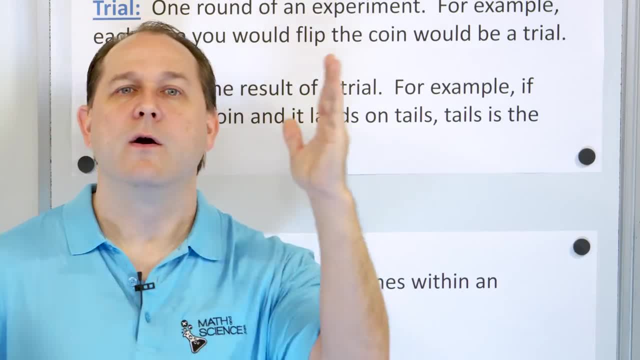 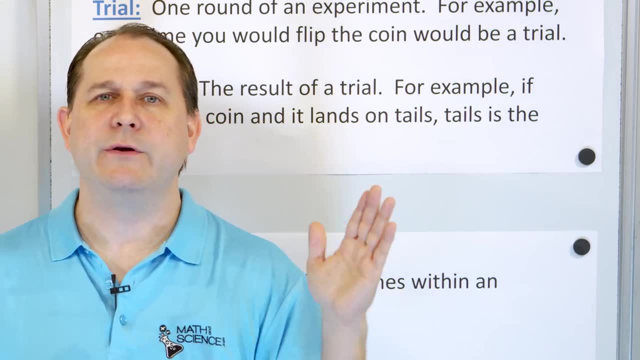 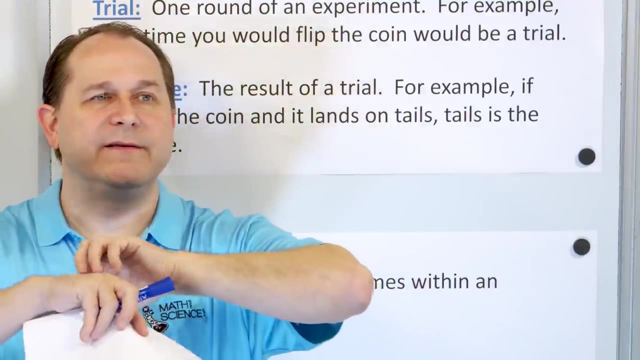 a number expressed between zero, for zero chance of happening. One means definitely will happen. That corresponds to 0% and 100%. But in general in probability we use decimals instead of percentages And we also can use fractions quite a bit. So the entire topic of probability is: 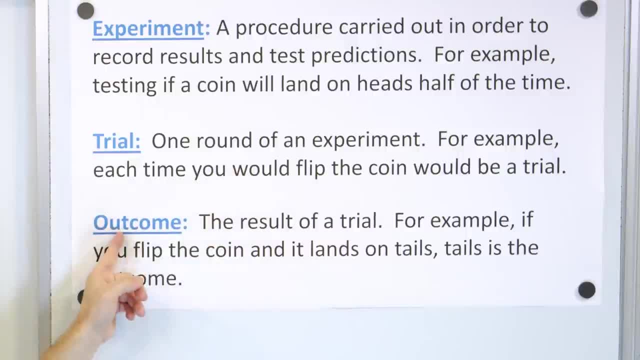 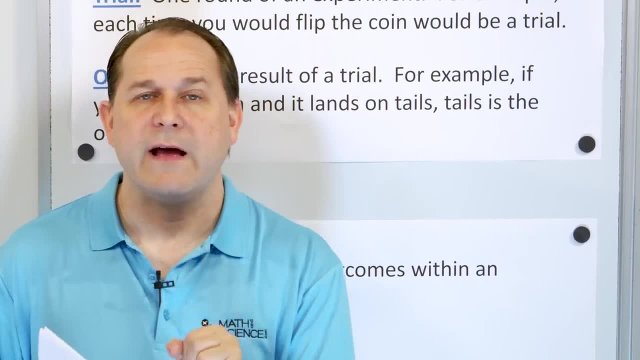 see what I get. In every single trial I get an outcome. So I do a trial of an experiment and I get an outcome. And an event is a collection of outcomes. So maybe I observe that I get five red socks in a row. That could be an event. right, It's a collection of outcomes that are trials of. 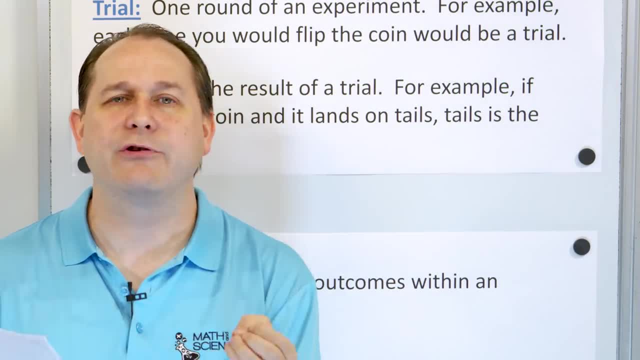 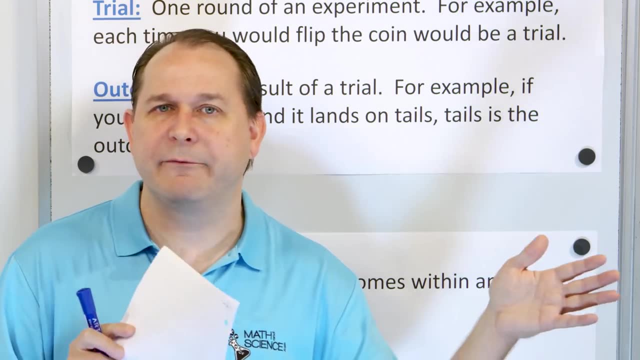 an experiment right, And from all of that information I can then calculate a probability. I can make a. I can either calculate a probability ahead of time and then check my experiment against the probability, or I could use the data I get to calculate the probability. You get the. 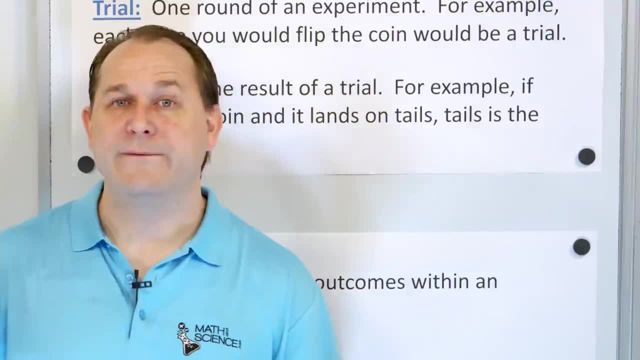 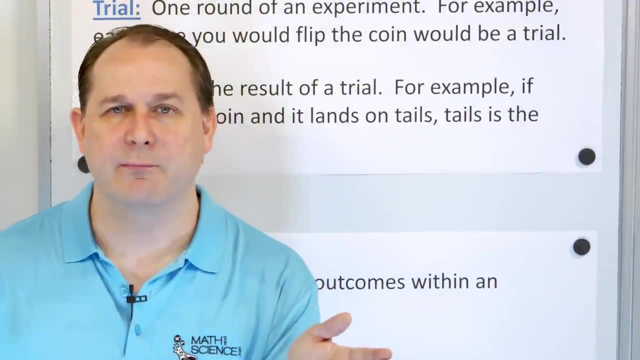 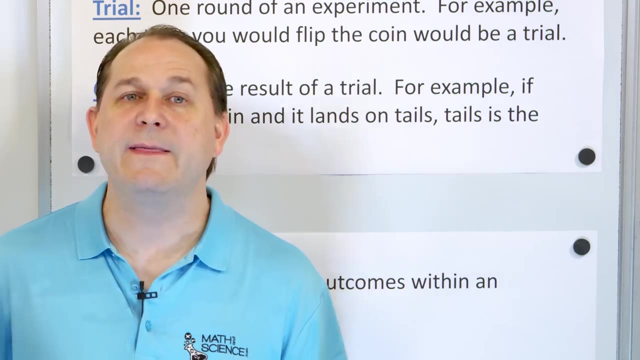 idea. So I might say that in my sock drawer there's a 35% chance of getting a red sock on any given draw. because I can, I'm going to teach you how to calculate the probability and what that means. 35% means that less than half of the time then I should pull a red sock out And then 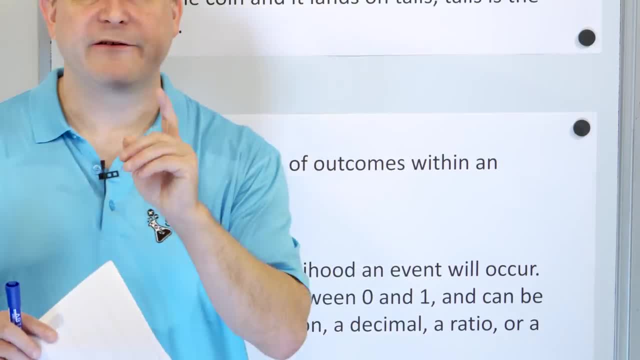 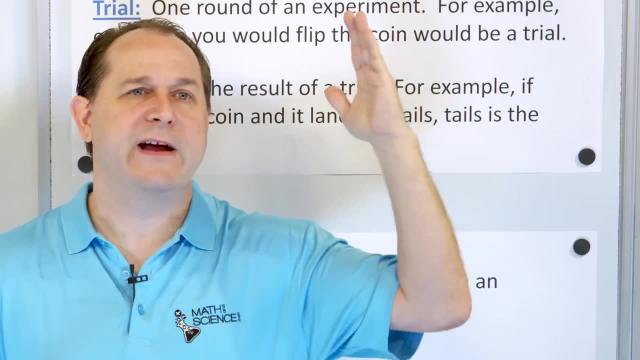 see if that is the case. So probability again: a number expressed between zero for zero, chance of happening. One means definitely will happen. That corresponds to 0% and 100%. But in general in probability we use decimals instead of percentages And we also can use fractions. 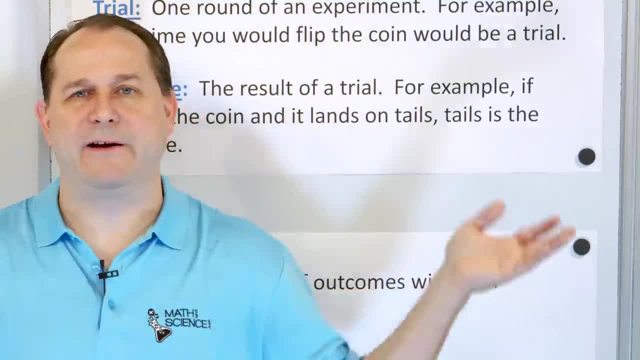 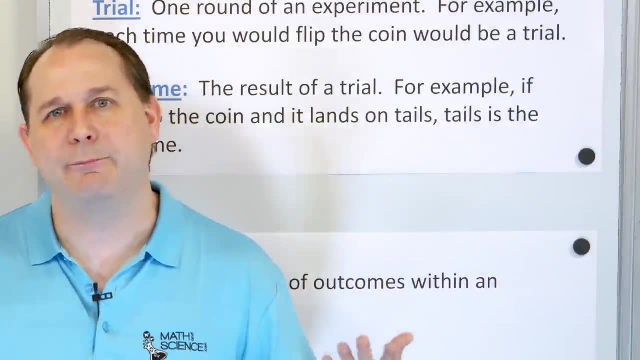 quite a bit. So the entire topic of probability is basically fractions. It's an application of fractions. That's why we learn fractions first, And you can think of probability as being essentially an application of what you have learned in fractions. All right, so let's start. 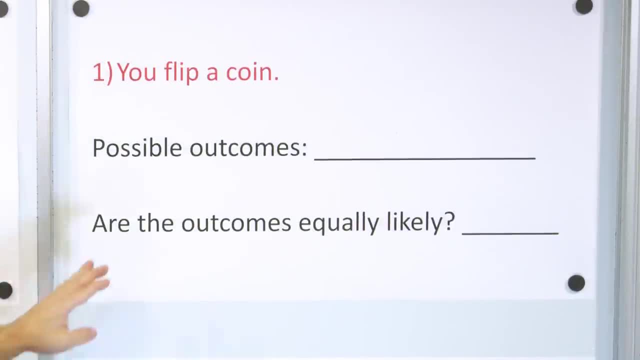 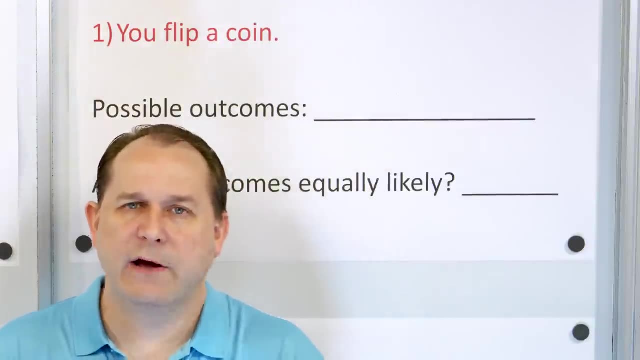 to talk about some different scenarios. So let's say I'm going to flip a coin. We're not going to really calculate anything right here. I'll do a little bit of teaching along the way to kind of help us understand what probability is. But these are just very basic problems. We flip a coin And 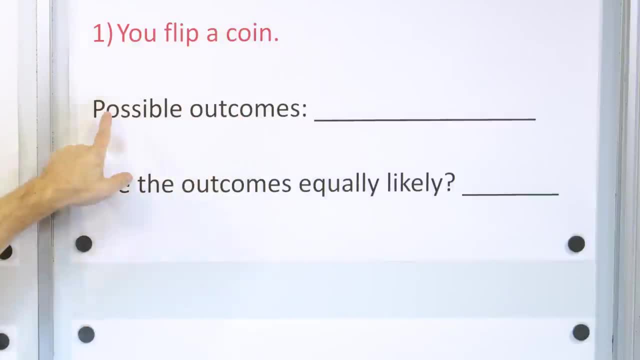 of course, you have to know that a coin has two sides, heads or tails. What are the possible outcomes? In other words, when you look at the possible outcomes, what could happen? What are the choices of what could happen? Well, the coin only has two sides. It has a side with a head on it. 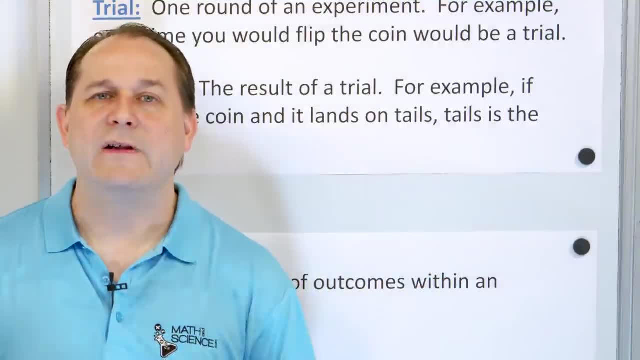 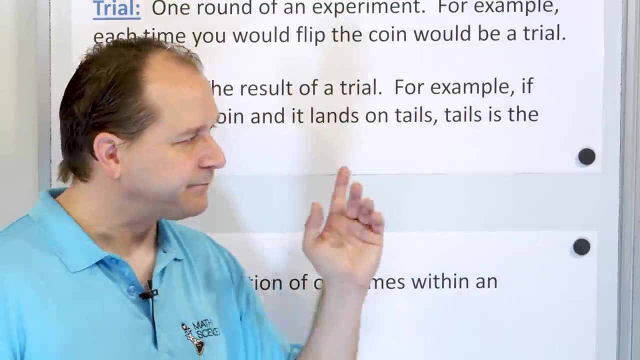 basically fractions. It's an application of fractions. That's why we learn fractions first, And you can think of probability as being essentially an application of what you have learned in fractions. All right, so let's start to talk about some different scenarios. 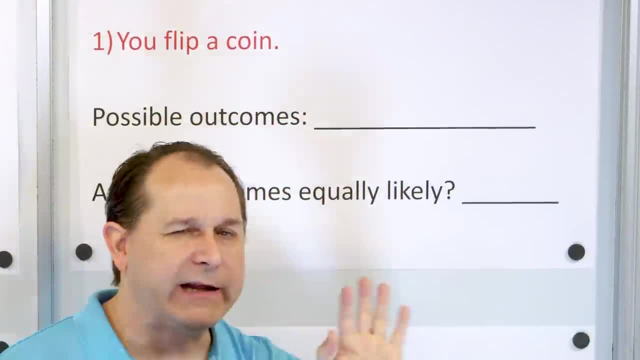 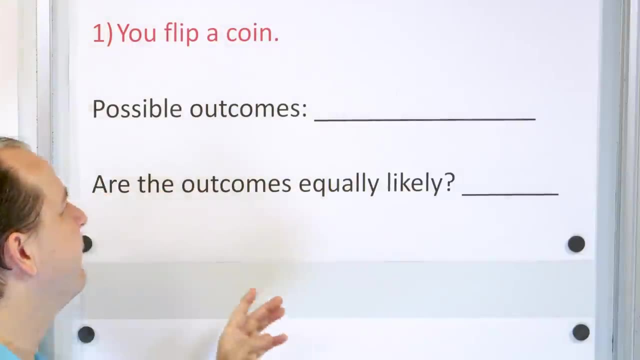 So let's say I'm going to flip a coin, We're not going to really calculate anything right here. I'll do a little bit of teaching along the way to kind of help us understand what probability is. but these are just very basic problems. 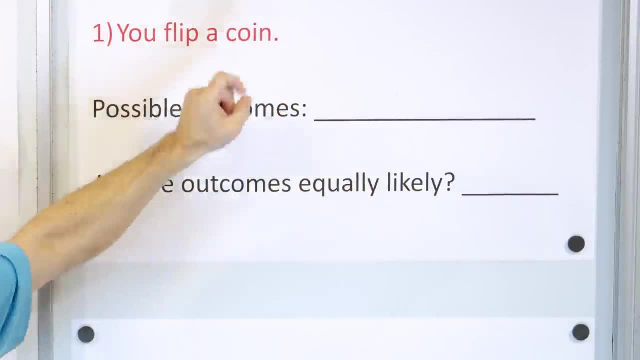 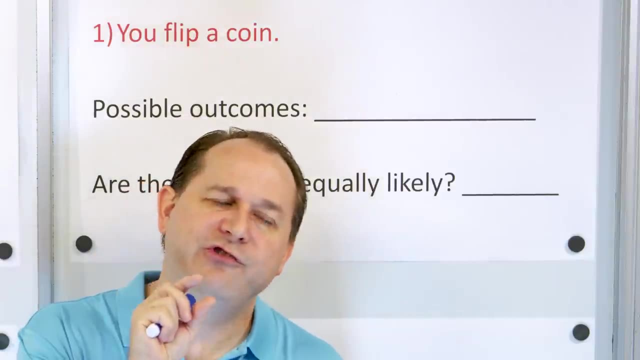 We flip a coin and of course, you have to know that a coin has two sides, heads or tails. What are the possible outcomes? In other words, when you look at the possible outcomes, what could happen, What are the choices of what could happen? 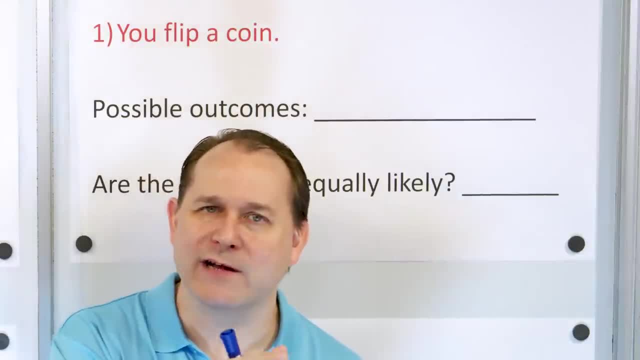 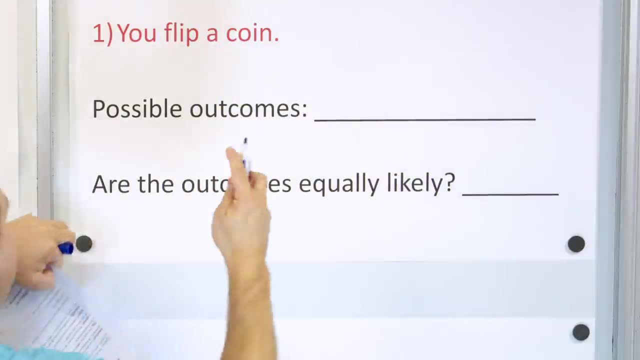 Well, the coin only has two sides. It has a side with a head on it and there's a side that's not the head. We call it the tail side. There's only two possible ways that thing can land. So, basically, the possible outcomes are going to be H for heads and T for tails. 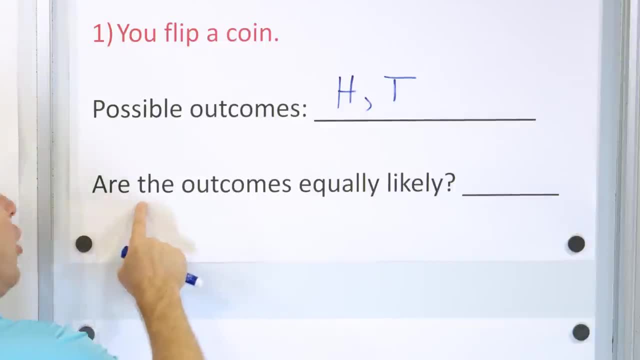 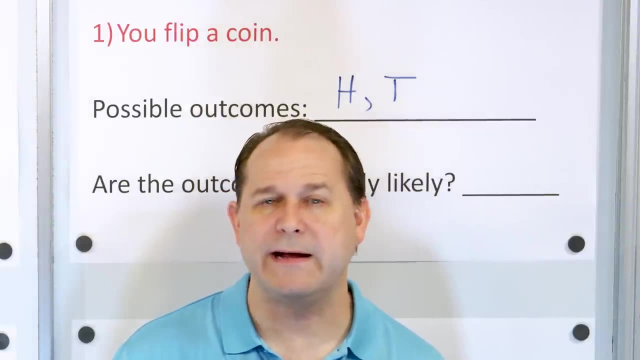 I'm going to use H for head and T for tails And I'm going to ask you: are the outcomes equally likely? Now we haven't talked about how to calculate the probability of something yet. We're going to talk about it in just a minute and then we're going to have entire lessons on it later. 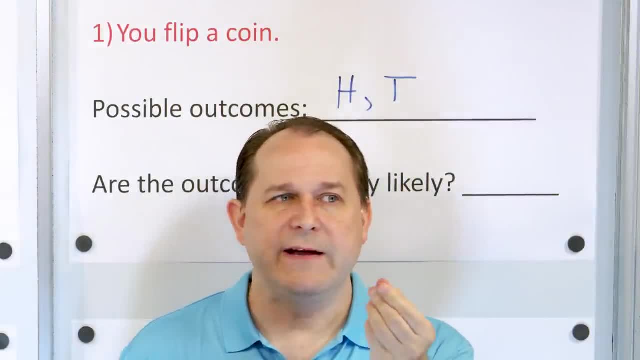 But just think about it: If there's only two ways to get the outcome, there's two outcomes, basically heads or tails, And the coin is equally balanced. In other words, it's not like lopsided or weighted funny or anything like that. 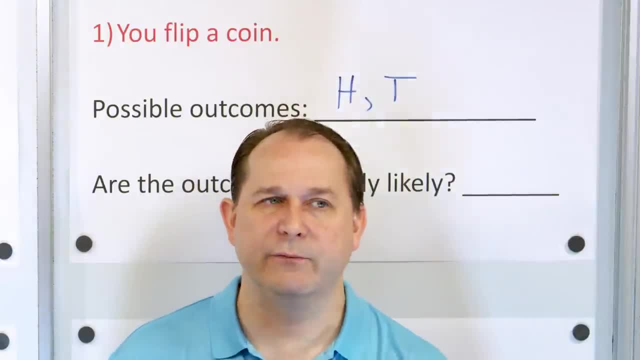 And it's called a fair coin, where it can land on either side without having something influencing the way it lands. It's just totally random And there's only two choices. right, And because there's only two choices and we only have one of each of the two choices, 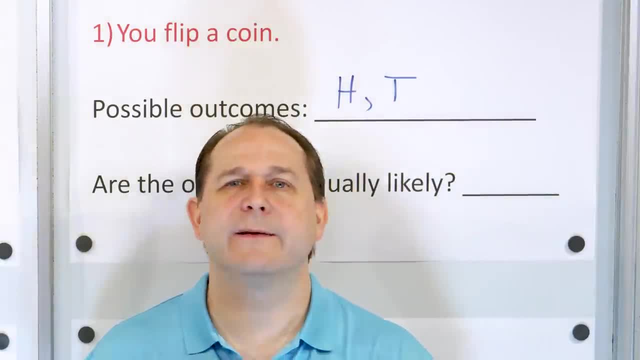 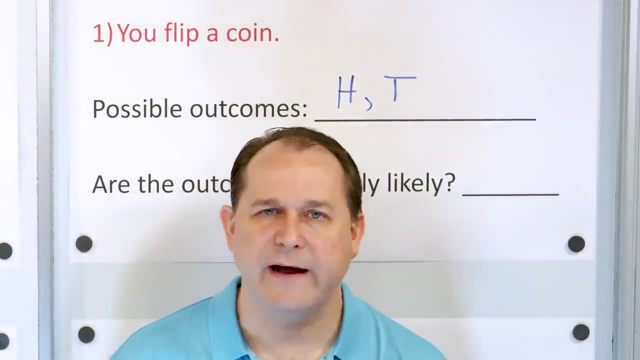 we expect that half the time will be heads and half the time will be tails. That's something you get when you just play with coins as a kid and kind of from your intuitive experience. There's only two choices, and there's heads or tails. 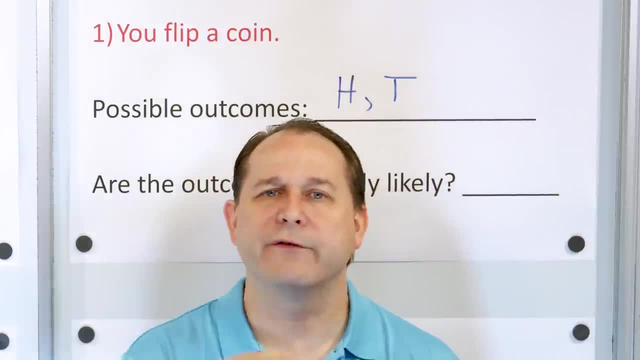 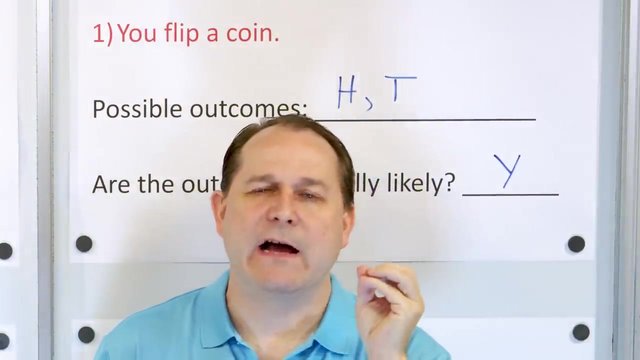 And we only have one of each of those choices: one head or one tail. So we expect that the outcomes are equally likely. We expect that half the time we will get heads and half the time we will get the tails. Now the rest of these problems. we're not yet studying all the details of how to. 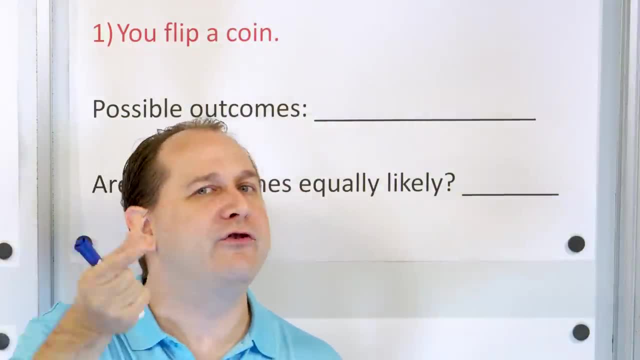 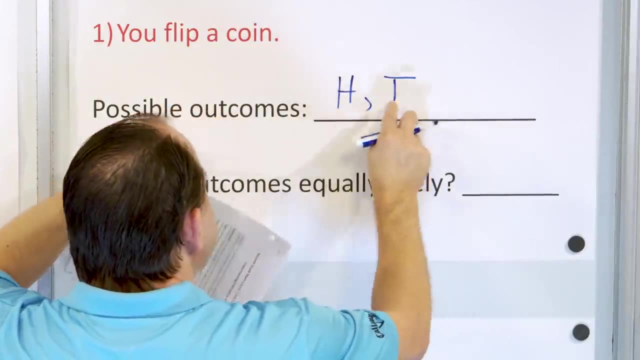 and there's a side that's not the head, We call it the tail side. There's only two possible ways that thing can land. So, basically, the possible outcomes are going to be H for heads and T for tails. I'm going to use H for head and T for tails And I'm going to ask you: are the outcomes? 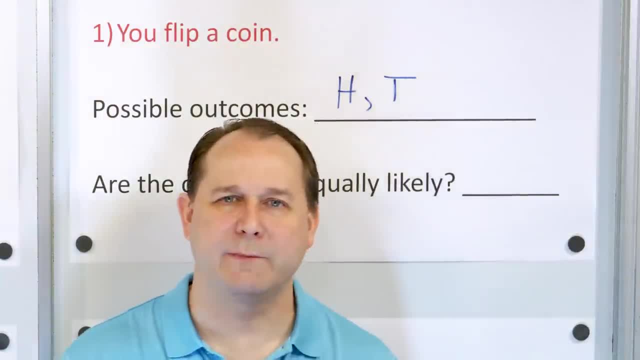 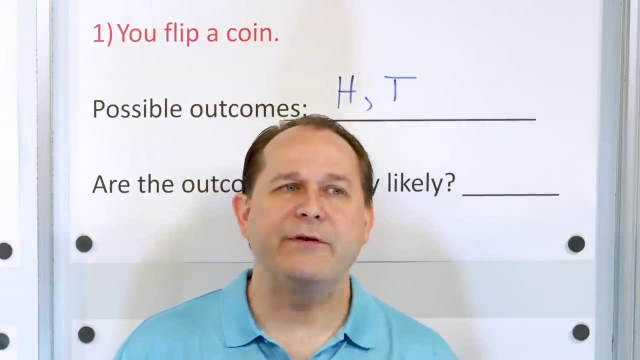 equally likely. Now we haven't talked about how to calculate the probability of something yet. We're going to talk about it in just a minute And then we're going to have entire lessons on it. to think about it. If there's only two ways to get the outcome, there's two outcomes, basically. 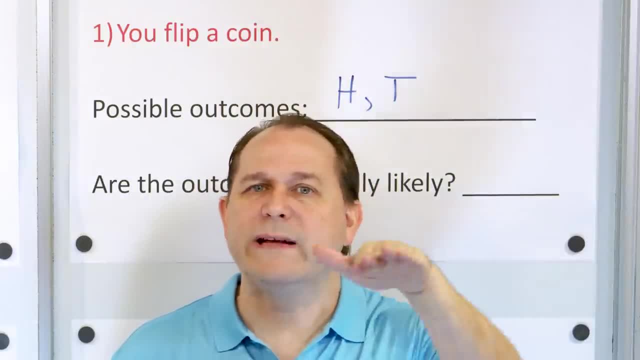 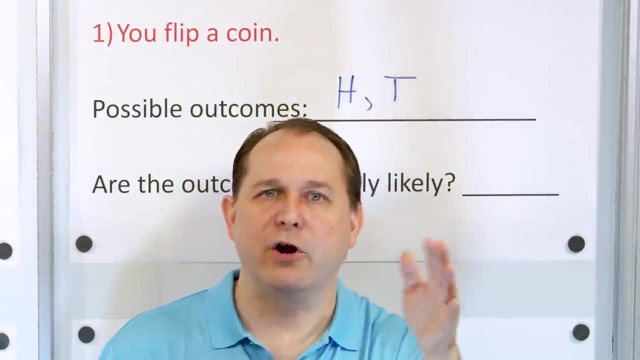 heads or tails And the coin is equally balanced. In other words, it's not like lopsided or weighted funny or anything like that, And it's called a fair coin, where it can land on either side without having something influencing the way it lands. It's just totally random And there's only 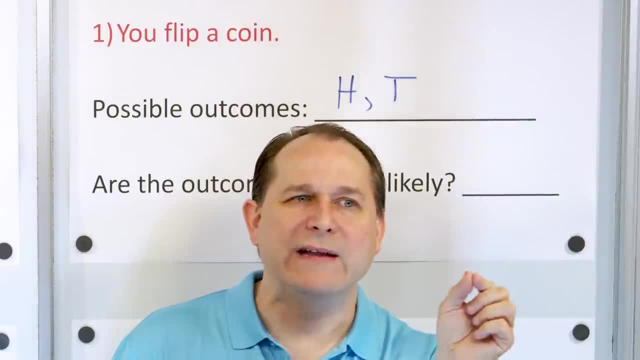 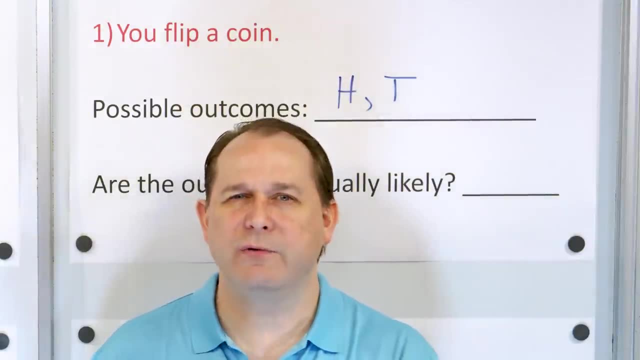 two choices- right, Because there's only two choices and we only have one of each of the two choices. then we expect that half the time will be heads and half the time will be tails. That's something you get when you just play with coins as a kid and kind of from your intuitive experience. 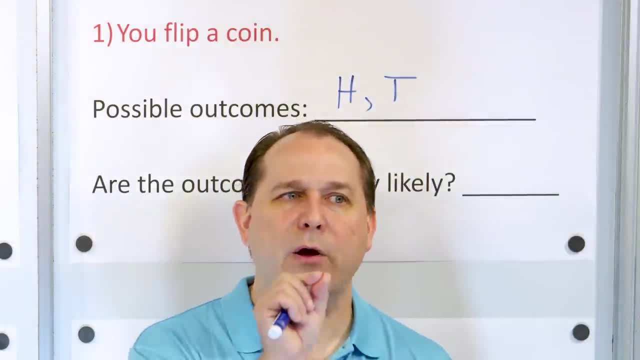 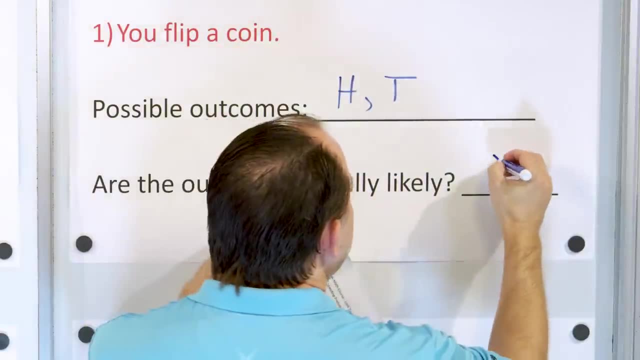 There's only two choices, and there's heads or tails, And we only have one of each of those choices, one head or one tail. So we expect that the outcomes are equally likely. We expect that half the time we will get heads and half the time we will get the tails. Now, the rest of 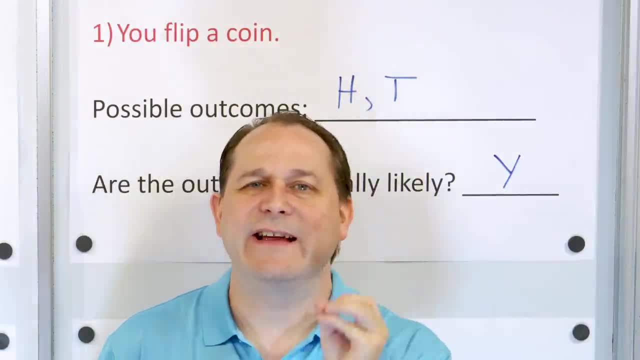 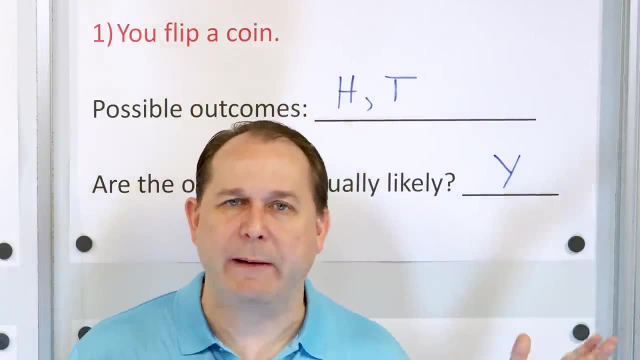 these problems. we're not yet studying all of them. We're not yet studying all of them. We're not all the details of how to calculate probability, but I just can't resist showing you, as we learn, these basic ideas, how to generally calculate a probability. So we're going to do it for some. 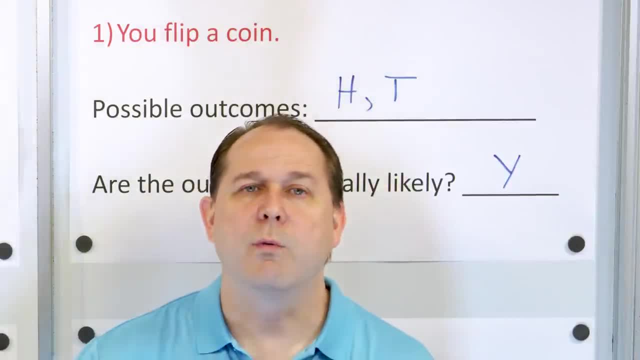 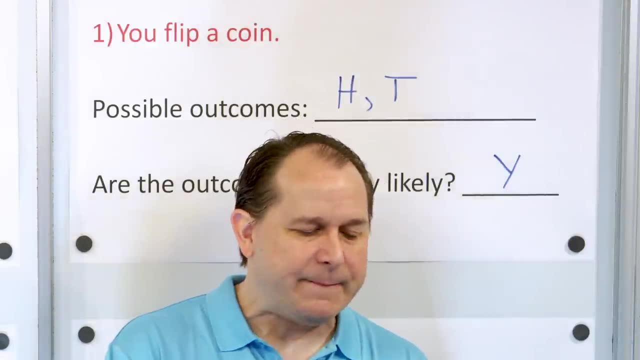 basic problems. but just keep in mind that we have entire lessons coming up where we're going to study lots of different situations with probability. So, in general, the way we write a probability is: it's the outcome that you're looking for in the numerator of the fraction. 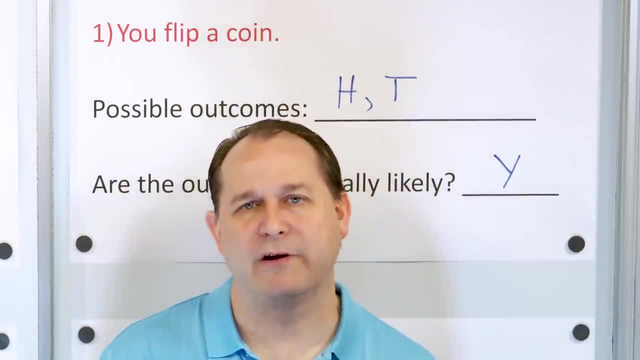 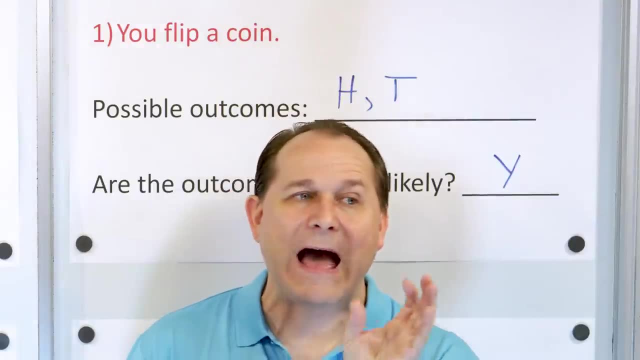 and on the denominator of the fraction, it's the total possible number. So basically, when you look at calculating the probability, you have to know how many outcomes you have, how many different ways in which the coin could land. The coin can only land in two. 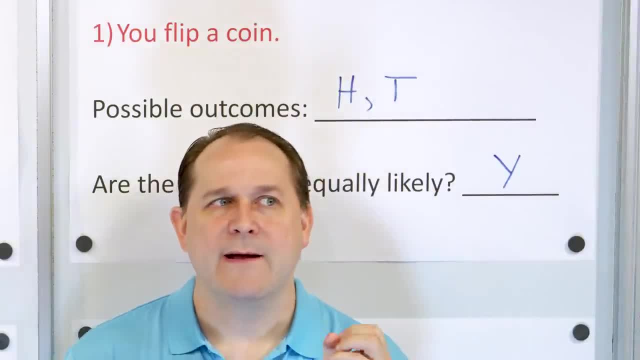 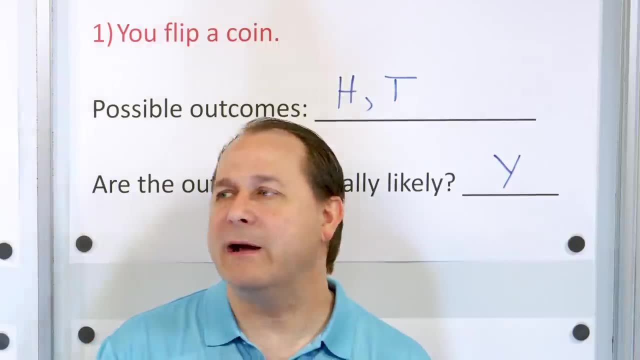 calculate probability, but I just can't resist showing you, as we learn, these basic ideas, how to generally calculate a probability. So we're going to do it for some basic problems, but just keep in mind that we have entire lessons coming up where we're going to study lots of different situations with probability. 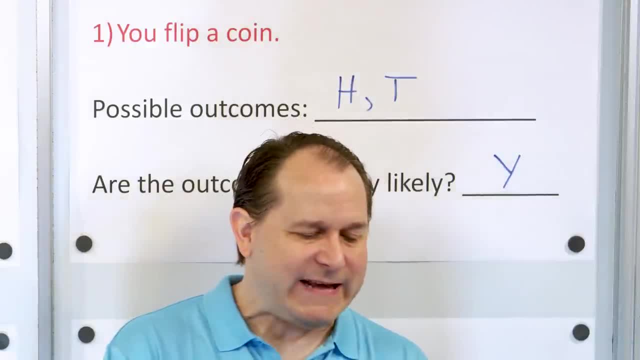 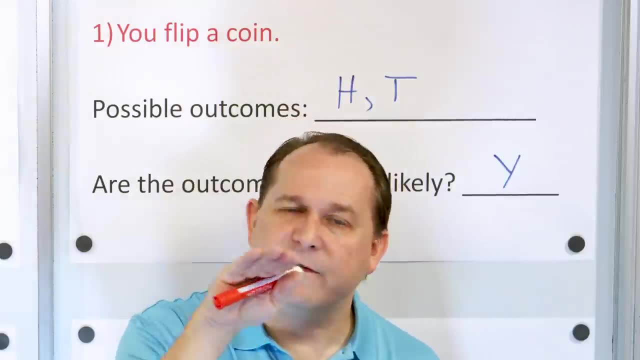 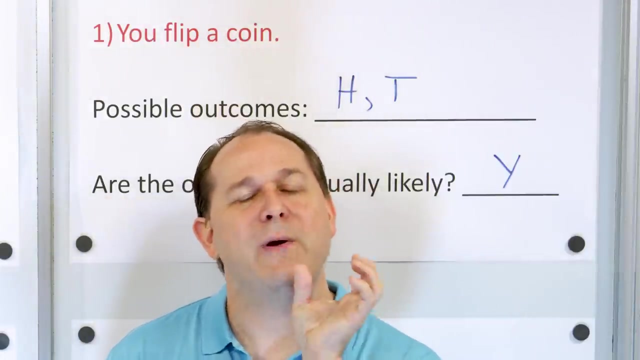 So, in general, the way we write a probability is: it's the outcome that you're looking for in the numerator of the fraction and on the denominator of the fraction it's the total possible number of outcomes. So, basically, when you look at calculating the probability, you have to know how many outcomes you have. 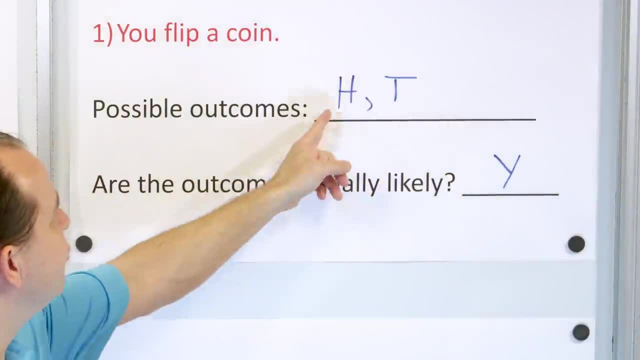 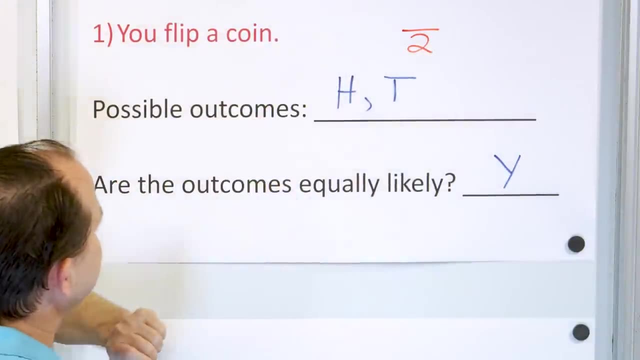 how many different ways in which the coin could land. The coin can only land in two positions, So the denominator of this fraction is two. If I'm going to try to find the probability of heads happening, for instance, then first I have to know how many different ways the coin can land. 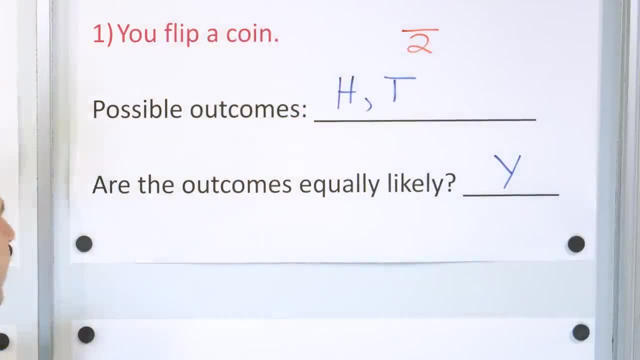 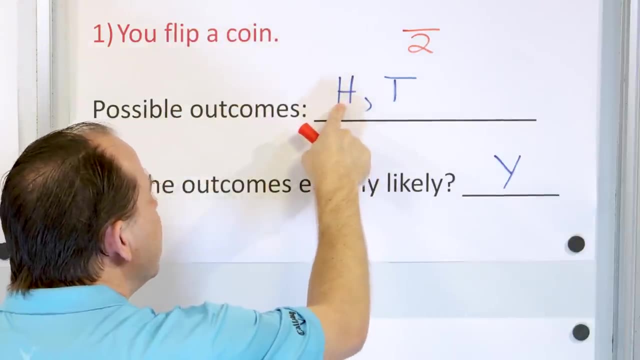 It can land two ways, which means the denominator of the fraction of the probability of landing on heads is two. Now, how many ways in which I can get a heads? I only have one way. I have one heads here, So there's only one heads that I can get out of a total of two possible ways in which the thing could land. 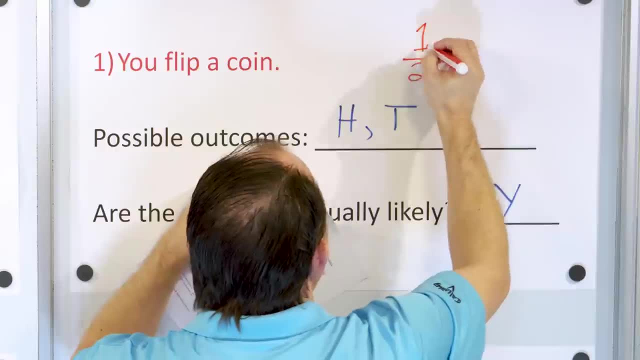 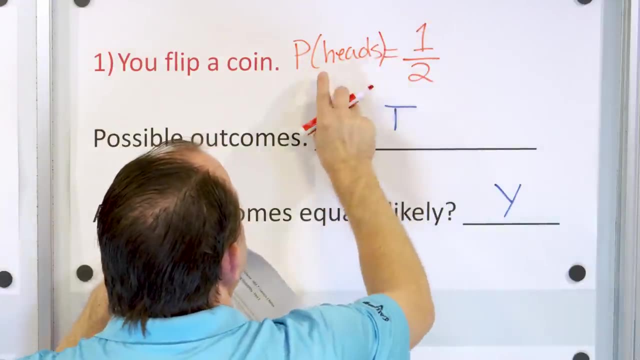 So this is starting to smell like a fraction, right, And so the probability of landing of heads. I'll put: probability of heads is one half, And the parentheses it doesn't mean multiplication, It means probability of landing on heads is one half. 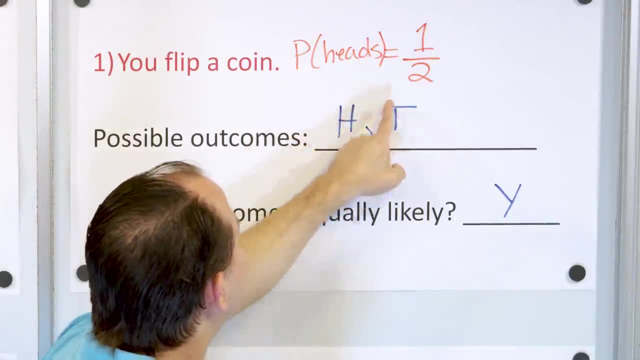 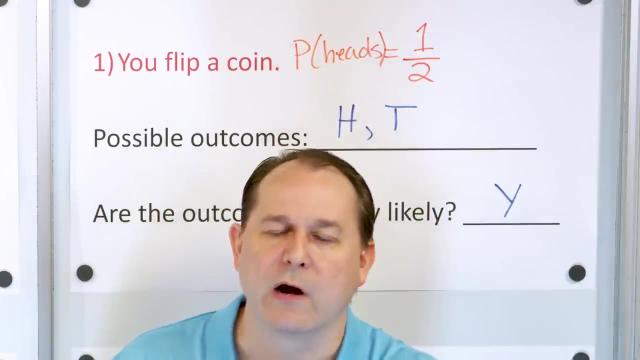 Why is it one half? Because there's only one heads that can happen and there's two possible outcomes. That's how you find a probability. First you have to identify the outcome. you're looking for how many ways that that can happen. only one heads. 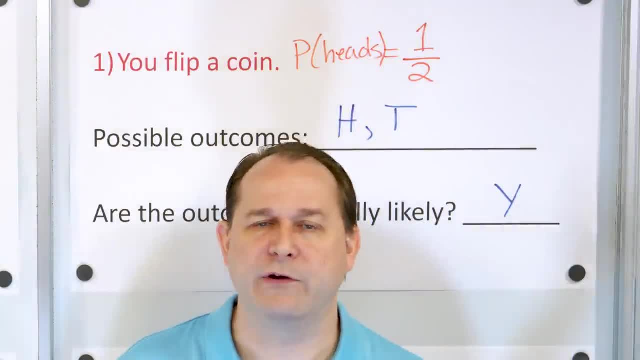 And then you have to look at the total number of outcomes in all of the ways in which the thing can land. So there's only two outcomes: heads or tails. So because I'm looking for heads, that's only one outcome. But the thing can only land two ways, that's two outcomes. 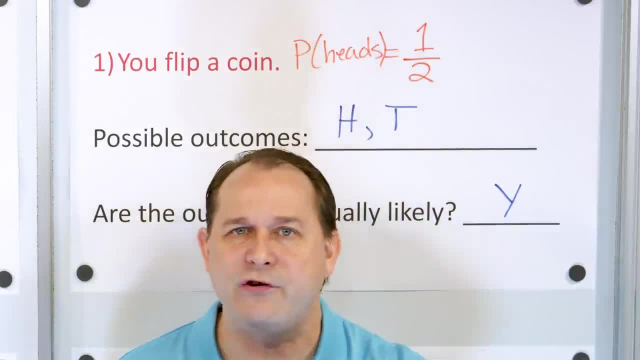 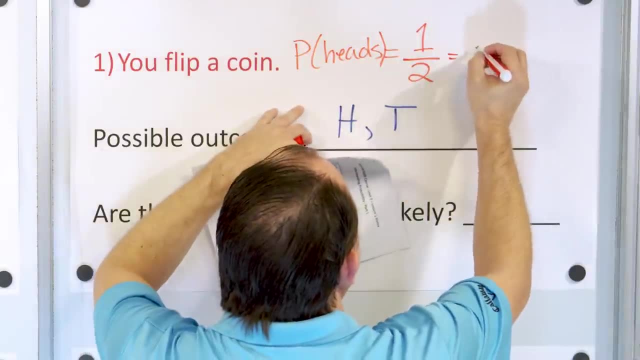 The probability, the fraction of time it'll land on heads is one out of two. one out of two times Now. this means one half. Now you all know that one half as a fraction is equal to zero, 0.5.. 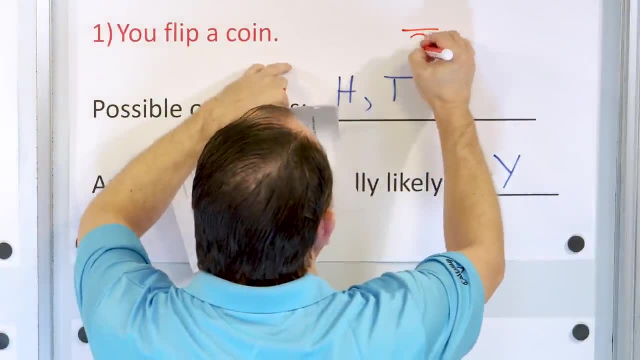 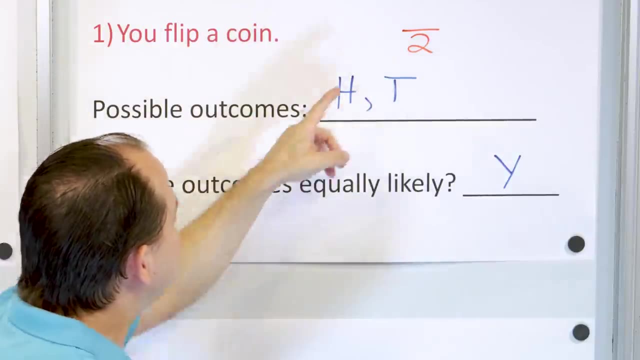 positions. So the denominator of this fraction is two. If I'm going to try to find the probability of heads happening, for instance, then first I have to know how many different ways the coin can land. It can land two ways, which means the denominator of the fraction of the probability 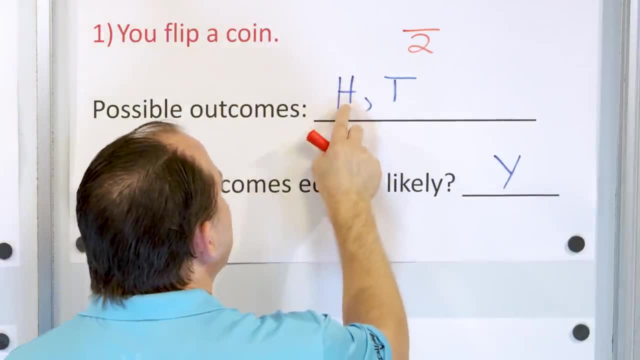 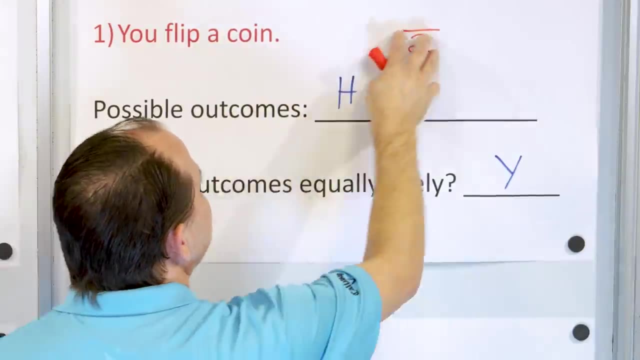 of landing on heads is two. Now, how many ways in which the coin can land is two. Now, how many ways in which the probability of price ends up falling is a six. The probability of price starts remaining multiple ways. So let's say I can get a head and I only have one heads here. 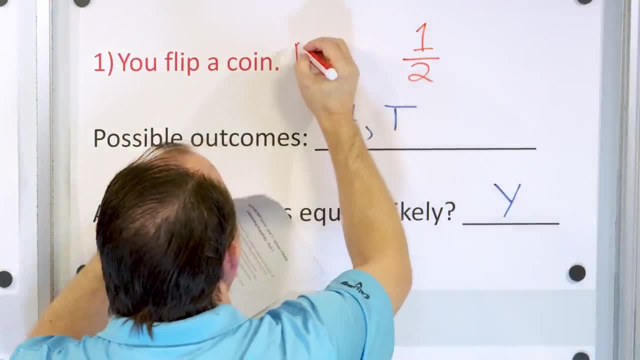 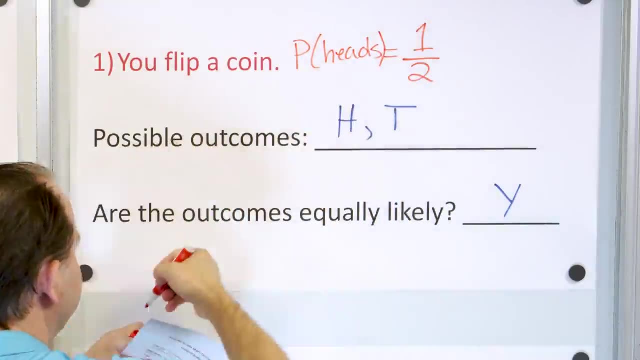 So there's only one heads that I can get out of a total of two possible ways in which the thing can land. So this is starting to smell like a fraction Right, And so the probability of landing of heads- I'll put probability of heads- is 1. 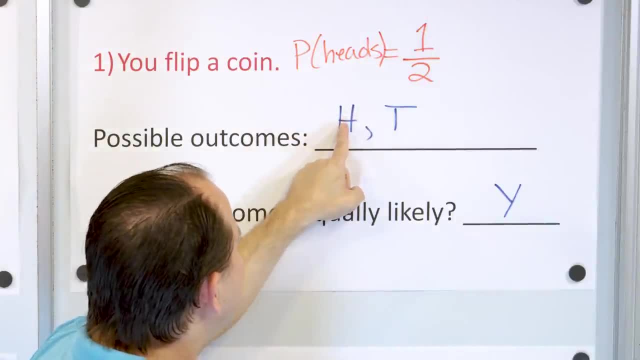 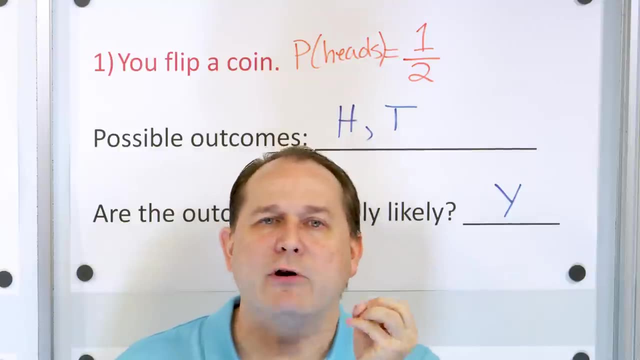 1⁄2.. And the parentheses. it doesn't mean multiplication. It means probability of landing on heads is 1⁄2.. Why is 1⁄2?? First you have to identify the outcome you're looking for. 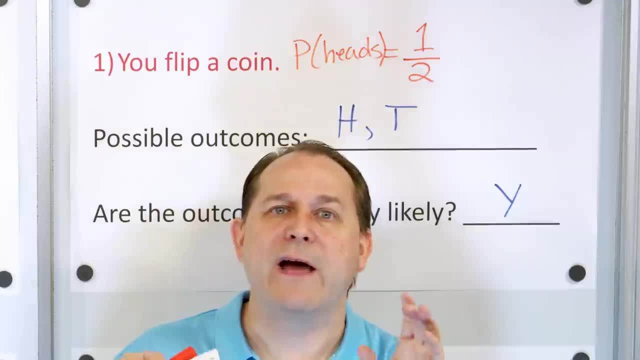 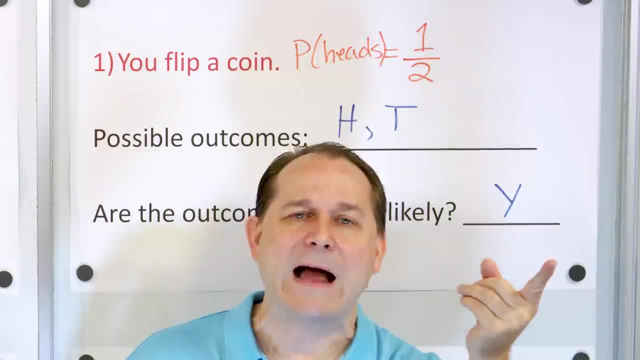 how many ways that that can happen. only one: heads. And then you have to look at the total number of outcomes and all of the ways in which the thing can land. So there's only two outcomes: heads or tails. So because I'm looking for heads, that's only one outcome. 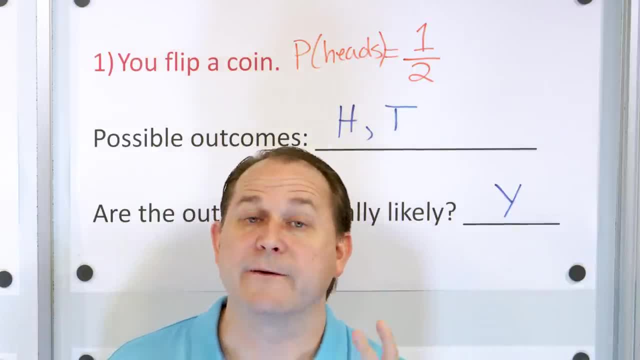 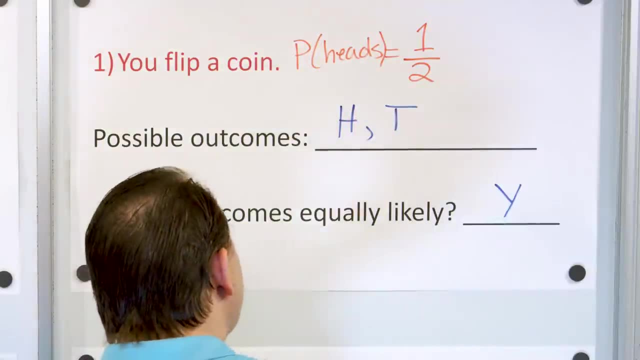 but the thing can only land two ways, that's two outcomes. The probability, the fraction of time it'll land on heads is one out of two. one out of two times Now, this means one half. Now. you all know that one half as a fraction is equal to 0.5.. 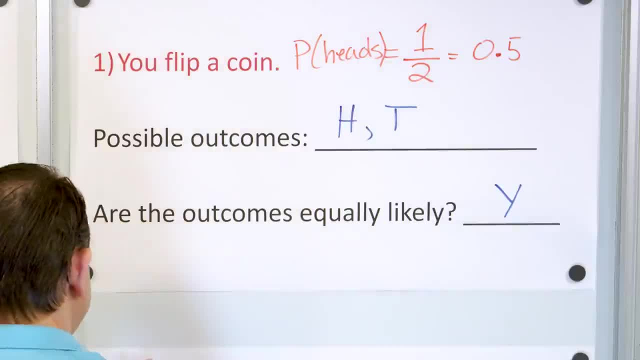 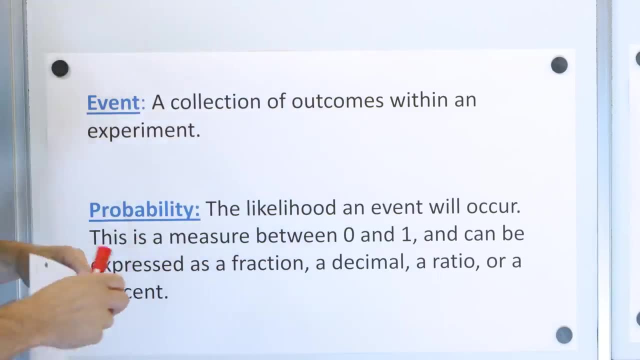 So we can express the probability as the fraction one half right And we can also express it as the decimal 0.5.. Remember, over here in our definition we said that probability is the likelihood an event will occur. It's a measure between zero and one. 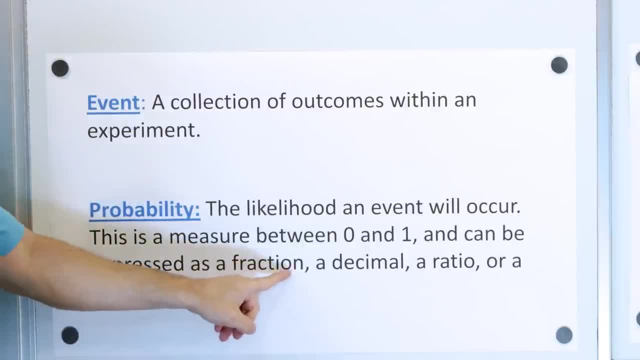 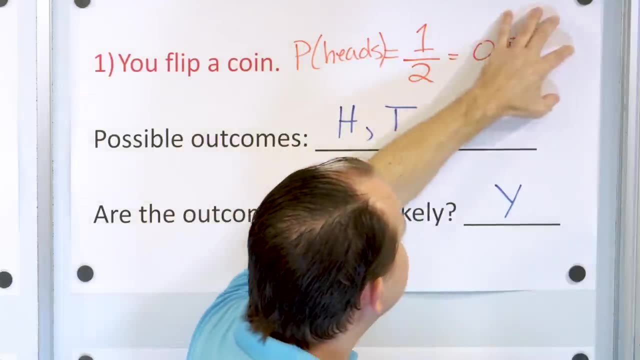 We got a decimal of 0.5 and can be expressed as a fraction, a decimal, a ratio or a percent. So we can express this probability in two ways, Or more than two ways. really, We can say the probability is 0.5.. 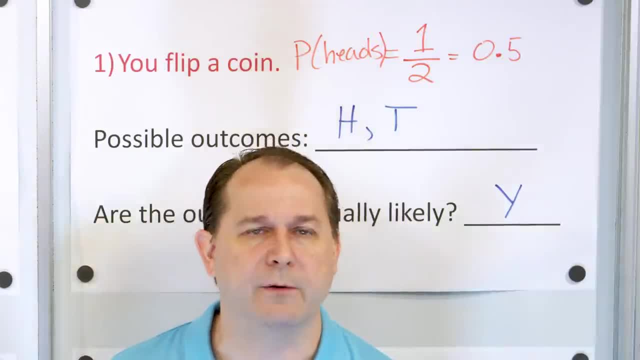 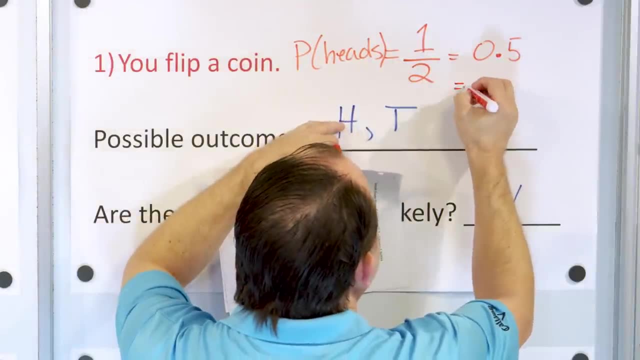 Remember, the scale is 0 to 1.. 0.5, right in the middle. We can also express it as the fraction one half. That's okay too. And then if you were looking at the weather or something, what you would do is you would convert this to a percent. 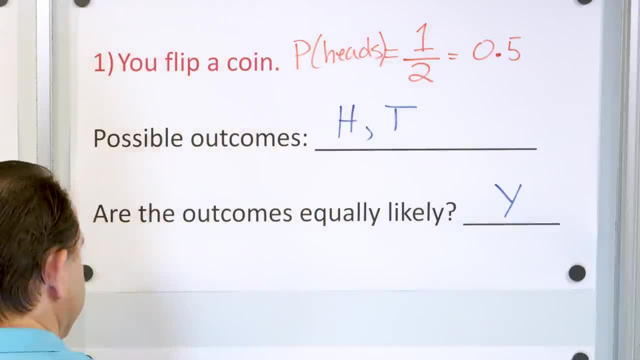 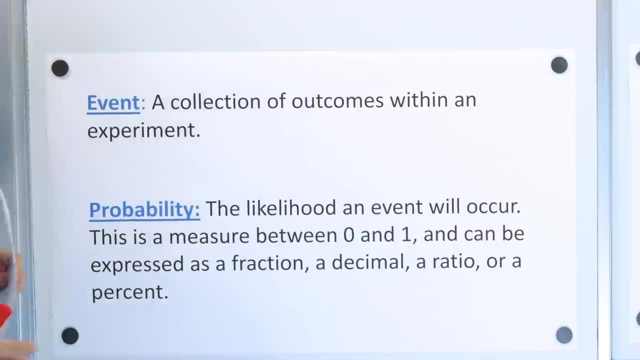 So we can express the probability as the fraction one half right And we can also express it express it as the decimal 0.5.. Remember, over here in our definition, we said that probability is the likelihood an event will occur. It's a measure between 0 and 1.. 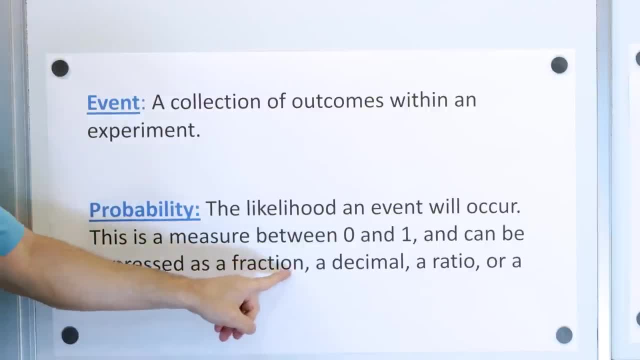 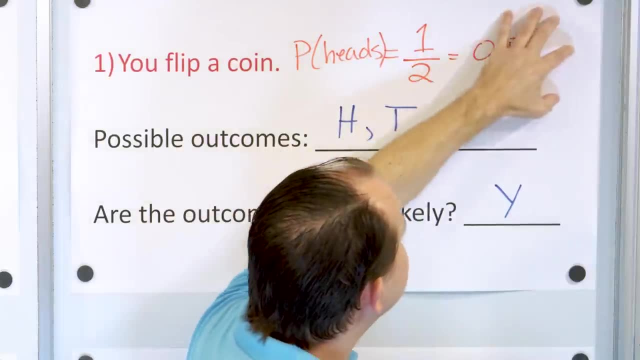 We got a decimal of 0.5 and can be expressed as a fraction, a decimal, a ratio or a percent. So we can express this probability in two ways, or more than two ways. really, We can say the probability is 0.5.. 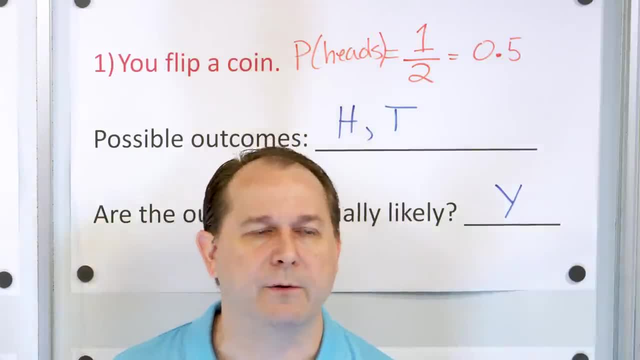 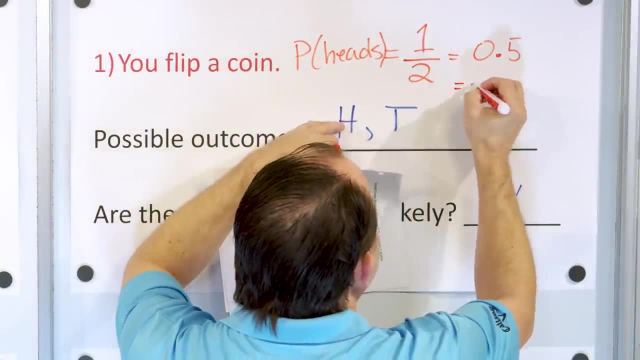 Remember, the tail is 0 to 1,, 0.5, right in the middle. We can also express it as the fraction one half. That's okay too. And then if you were looking at the weather or something, what you would do is you would convert this to a percent by multiplying by 100, move the decimal two spots, and so it would be 50%. 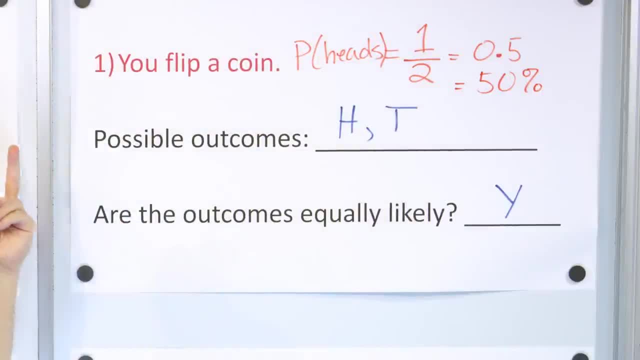 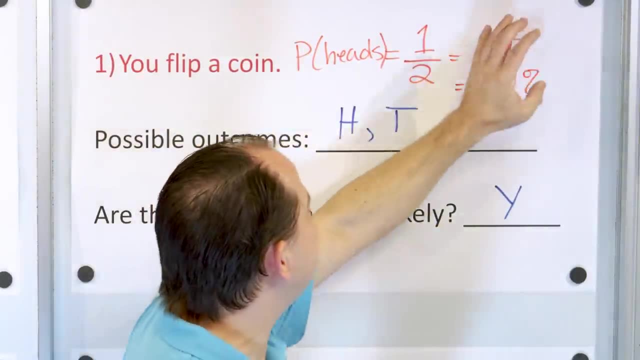 So what we have figured out is that if we flip a coin, a coin has two ways in which it can land. The possible outcomes are heads and tails: only two ways in which the thing can land. Are they equally likely? Yes, they are. 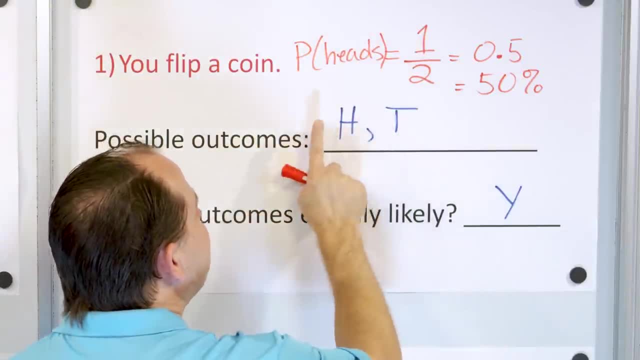 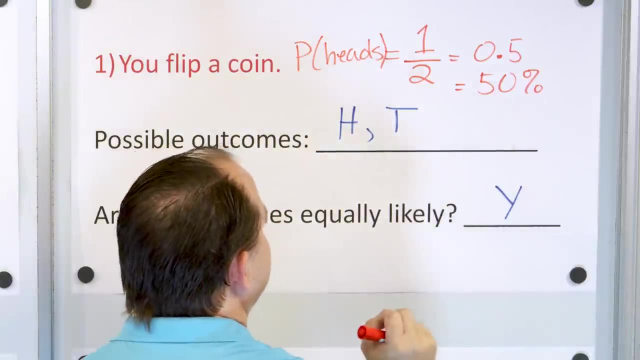 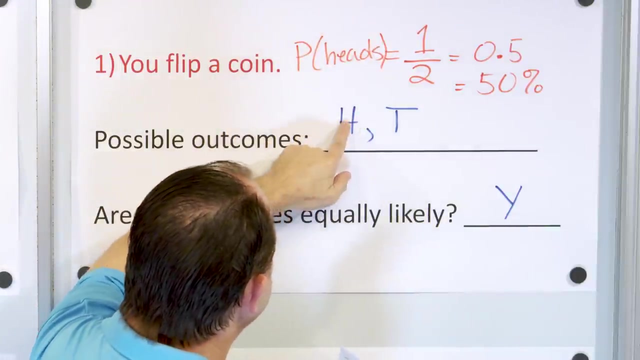 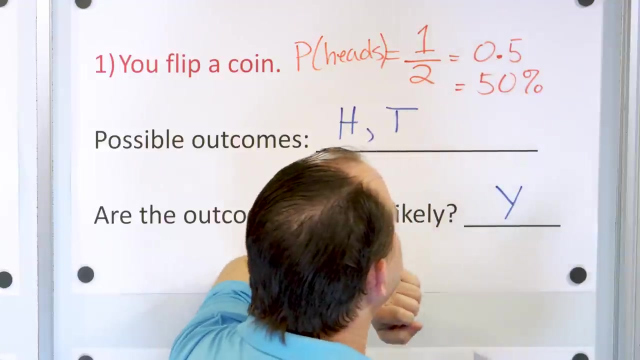 Because we only have two ways in which it can land, And each way it can land only happens one time, So we expect that the number of ways it can land is equally likely. So we put a yes right there And then, just for giggles, even though we haven't gotten to it yet, we calculated the probability of landing on heads as being one possible outcome out of a total of two possible ways it can land, which is a probability of one half, which is the same as a probability of 0.5, which is the same as 50% probability that you would see, maybe on TV in terms of a percentage. 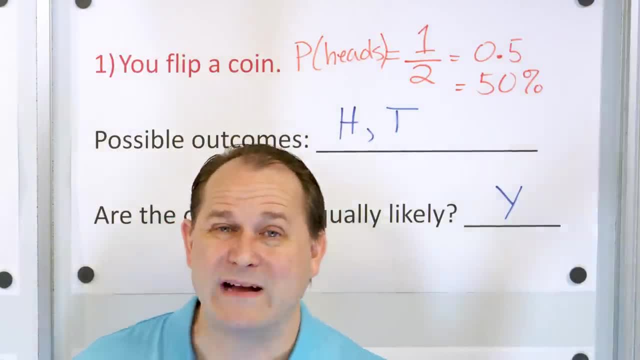 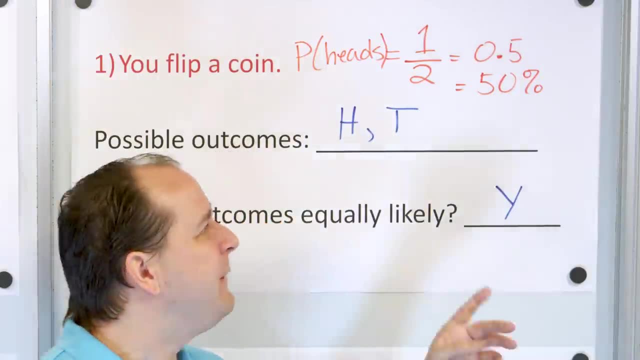 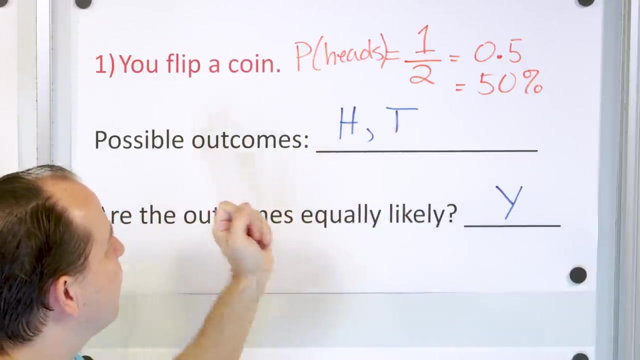 Now let me ask you another question. The probability of heads is one half 0.5.. What's the probability of landing on tails? Probability of tails? It's the same probability, Because if you land on tails, there's only one way in which you can get on tails, but there's two possible ways of two possible outcomes: total. 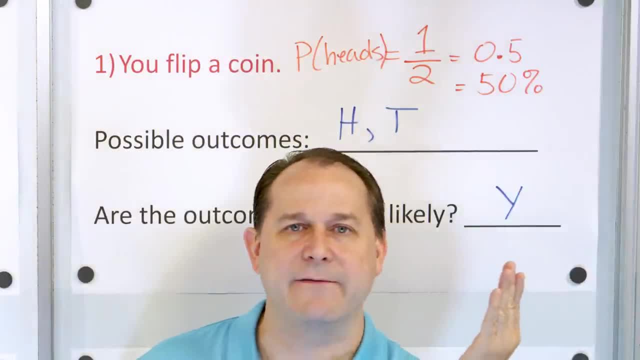 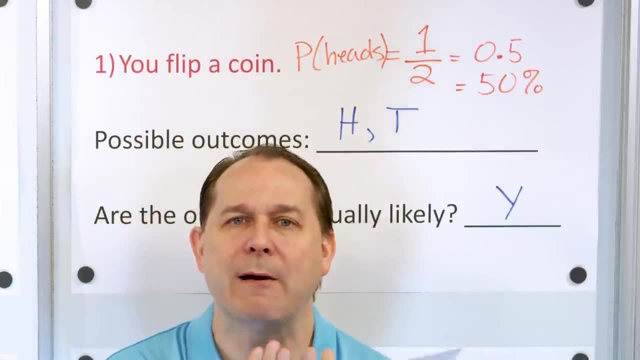 So again, it's one out of two. So the probability of heads is half and the probability of tails is also half, And when you put them together, what's one half plus one half- The probability of getting on tails. So either thing- heads or tails- is one half plus one half, which is one, which means that when you flip the coin, you're guaranteed to get either heads or tails. 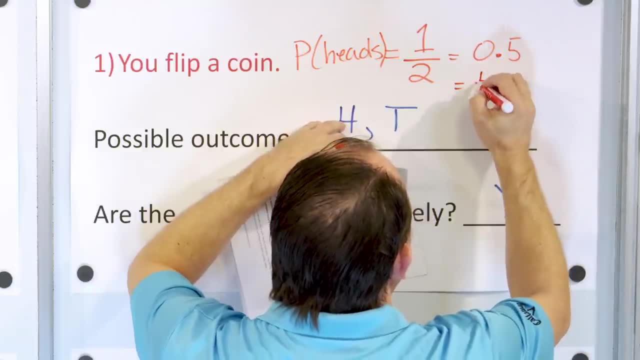 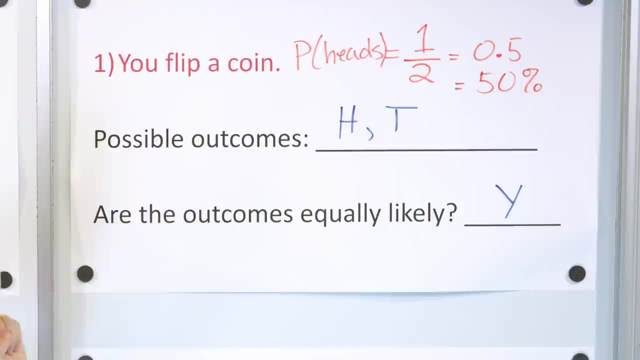 by multiplying by 100, move the decimal two spots, and so it would be 50%. So what we have figured out is that if we flip a coin, a coin has two ways in which it can land. The possible outcomes are heads and tails. 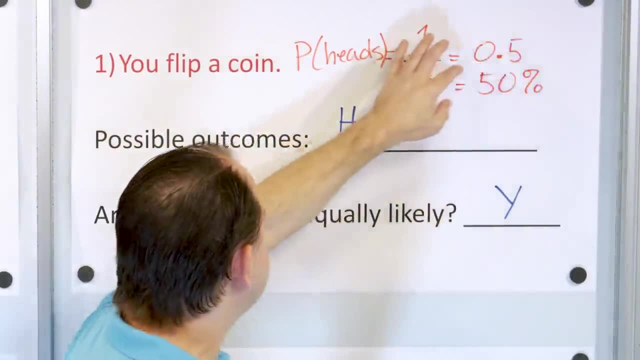 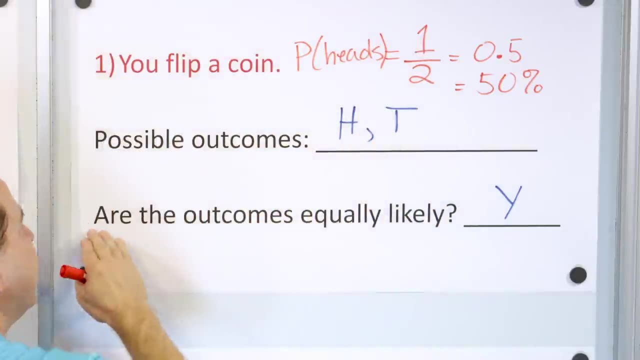 only two ways in which the thing can land, Are they equally likely? Yes, they are, because we only have two ways in which it can land and each way it can land only happens one time, So we expect that the number of ways it can land 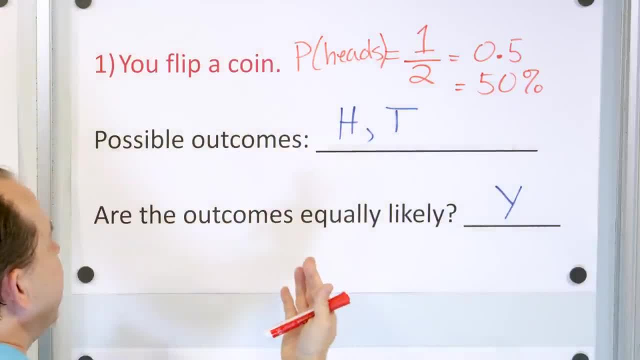 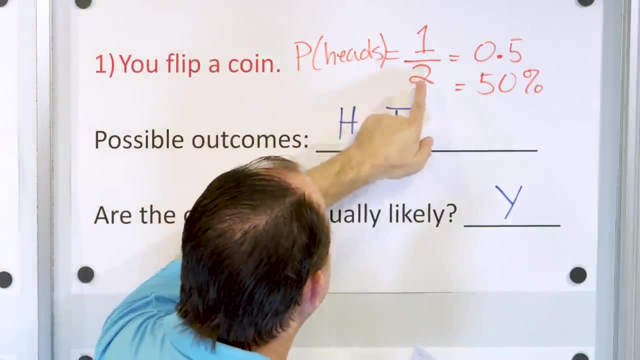 is equally likely. So we put a yes right there. And then, just for giggles, even though we haven't gotten to it yet, we calculated the probability of landing on heads as being one possible outcome out of a total of two possible ways it can land. 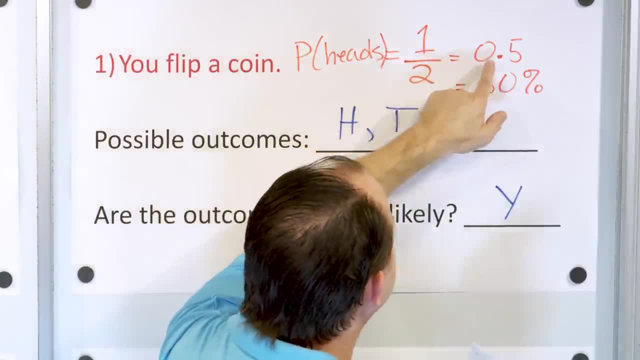 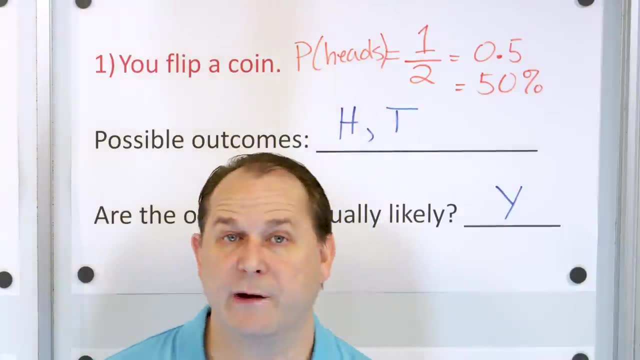 which is a probability of one half, which is the same as a probability of 0.5, which is the same as 50% Probability that you would see maybe on TV in terms of a percentage. Now let me ask you another question. 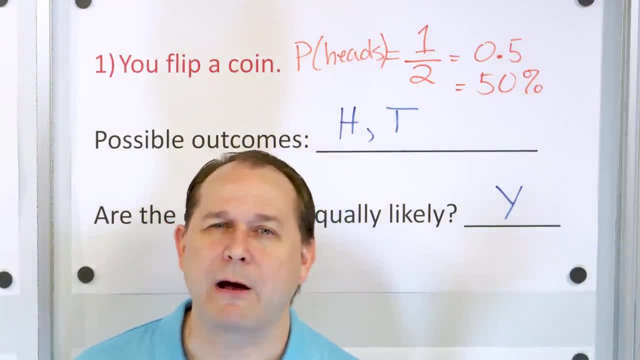 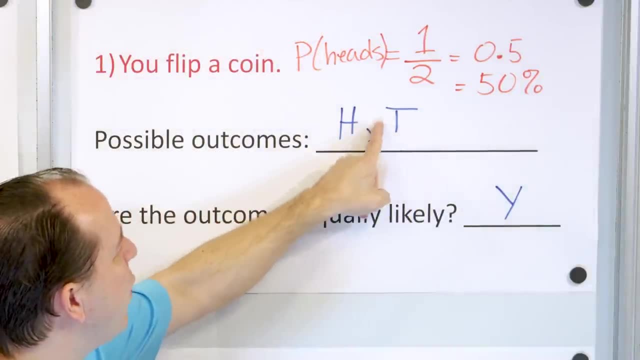 The probability of heads is one half 0.5.. What's the probability of landing on tails? Probability of tails: It's the same probability, because if you land on tails, there's only one way in which you can get on tails. 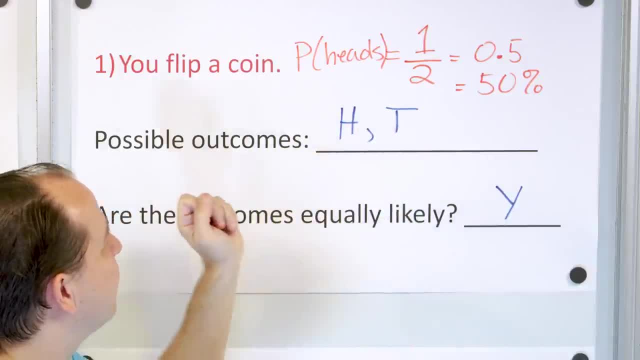 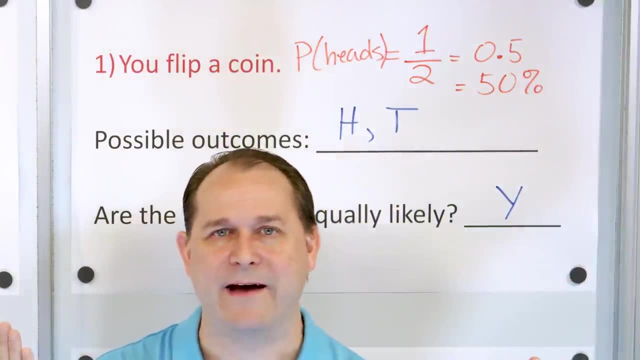 but there's two possible ways of two possible outcomes total. So again, it's one out of two. So the probability of heads is half and the probability of tails is also half, And when you put them together, what's one half? 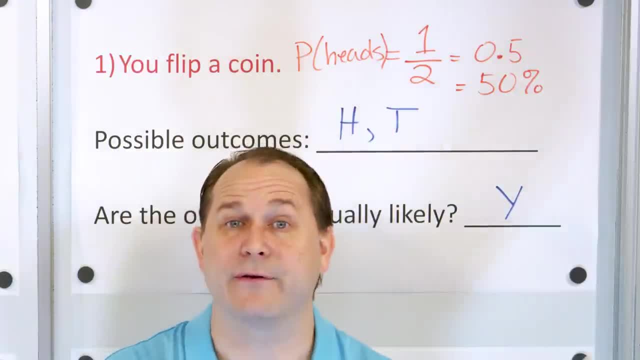 Plus one half, The probability of getting either thing- heads or tails- is one half plus one half, which is one, Which means that when you flip the coin, you're guaranteed to get either heads or tails Because, remember, the probability is a number. 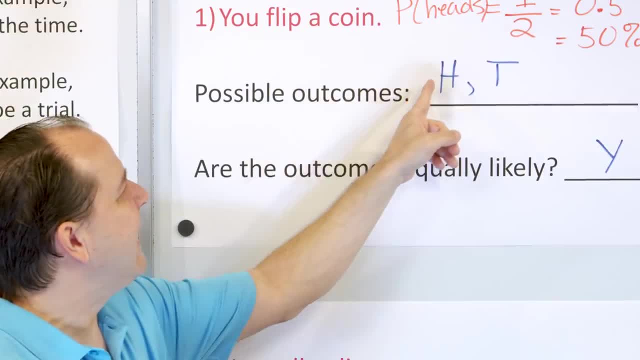 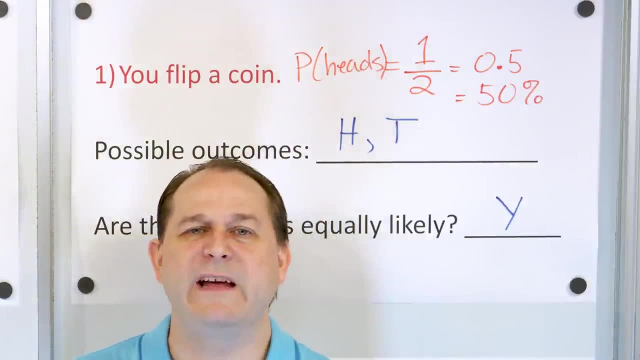 between zero and one. The probability of getting heads is one half. The probability of getting tails is also one half, And if you add those together you get one, which means the probability of getting either one of those things is one, which means you will always get one of those answers. 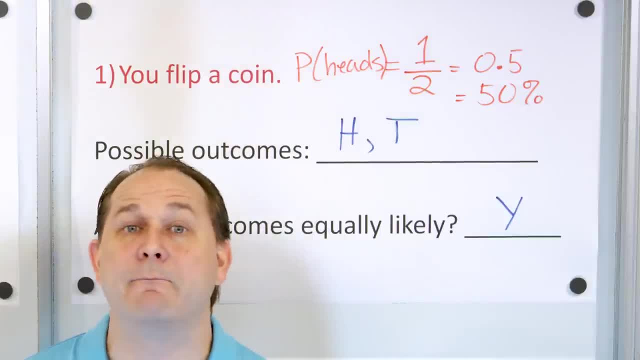 Now, Before we go on, what does probability of one half mean in this context? Obviously, I can flip a coin. Sometimes I'll get heads and sometimes I'll get tails. So what does it really mean to get one half? All it means is, if I flip a coin a large number of times, 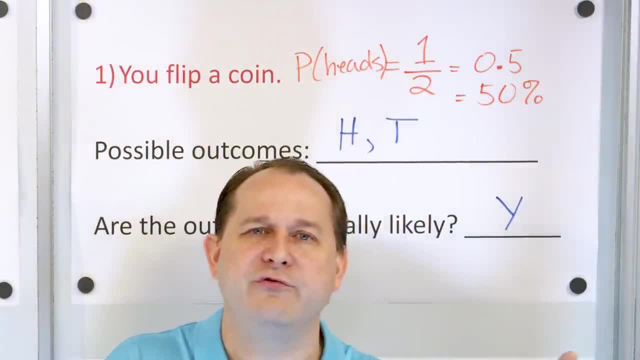 because probability theory says that the more trials that you do, the more times in which you flip that coin, then the closer and closer the actual observation of heads and tails approach one half. So in other words, if I flip a coin ten times, 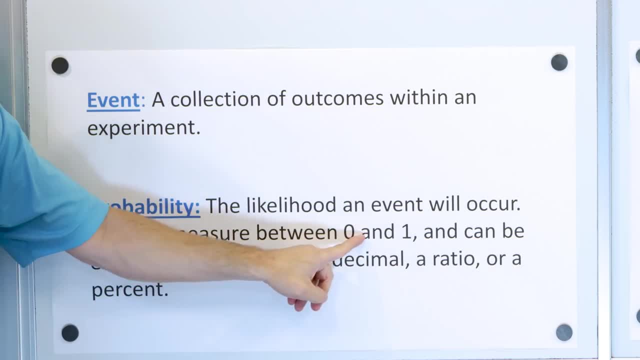 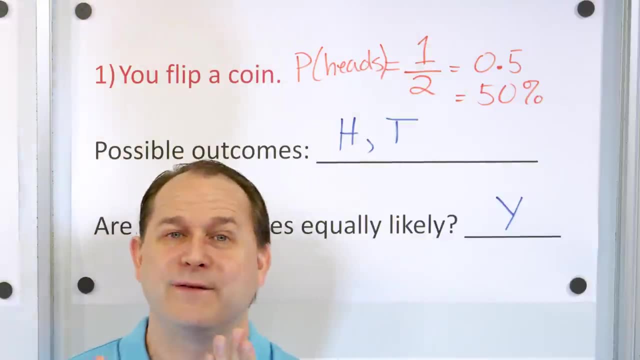 Because, remember, the probability is a number between zero and one. The probability of getting heads is one half, The probability of getting tails is also one half And if you add those together you get one, which means the probability of getting either one of those things is one, which means you will always get one of those answers. 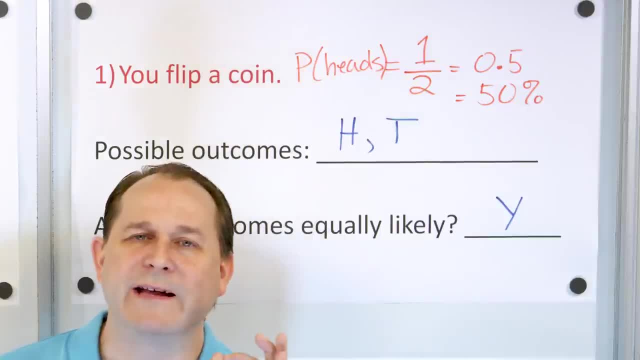 Now, before we go on, what does probability of one half mean In this context? obviously I can flip a coin. Sometimes I'll get heads and sometimes I'll get tails. So what does it really mean to get one half? All it means is if I flip a coin a large number of times, because probability theory says that the more trials that you do, the more times in which you flip that coin. 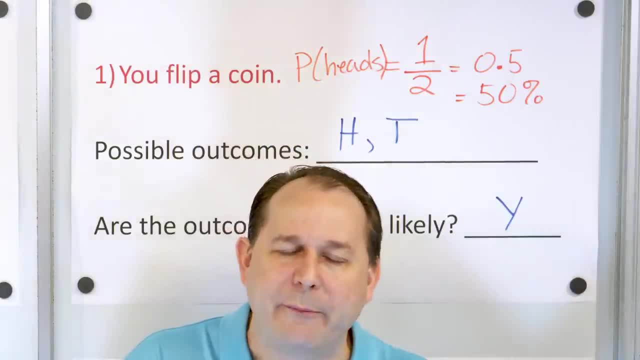 then the closer and closer, the actual observation of heads and tails approach one half. So in other words, if I flip a coin ten times, the probability would tell me that half of those times I should get heads and half of those times I should get tails. five and five. 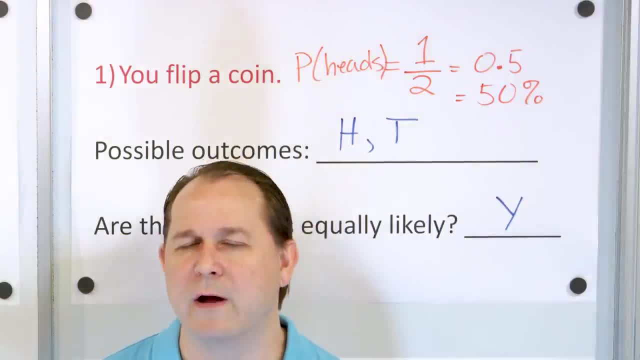 If I flip a coin ten times I should get five heads and five tails. But we all know that if you actually do that, you might not get five and five, You might get like seven and three or you might get six and four. 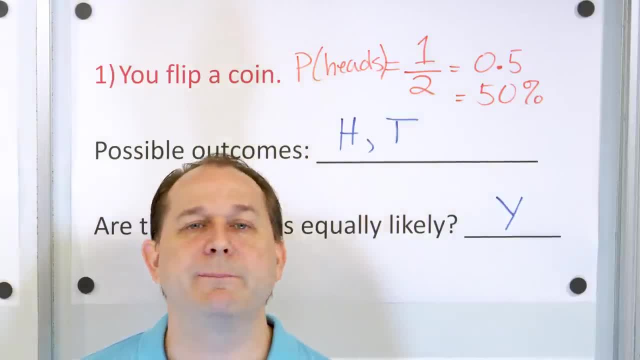 It's not going to be exactly five and five for only ten trials, But if you flip the coin 20 times, you would expect five heads and five tails. It might happen, but you might get maybe 11 heads and nine tails. They still have to add to 20, right? 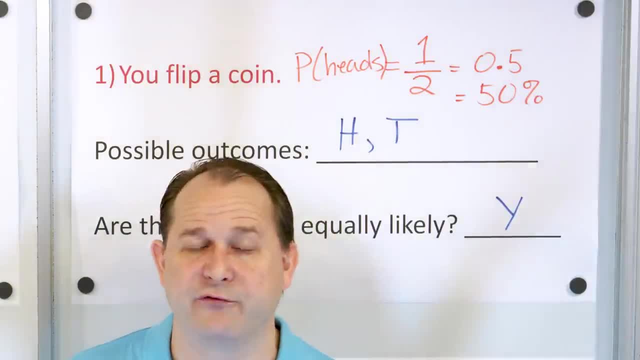 But as I increase the number of trials. if I go to a thousand trials then I should expect 500 heads and 500 tails, half and half, That's what the probability is telling me, But I might actually get more like 499 heads and 501 tails. 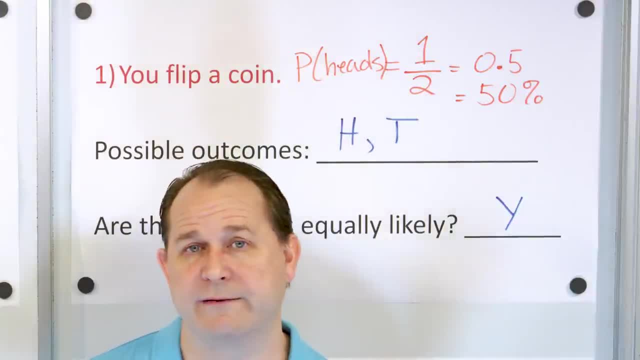 But you see, it's getting closer to half and half. If I run this experiment a trillion times, a trillion times, if I approach infinity number of trials, the more and more and more and more trials I do, the closer and closer I actually expect. 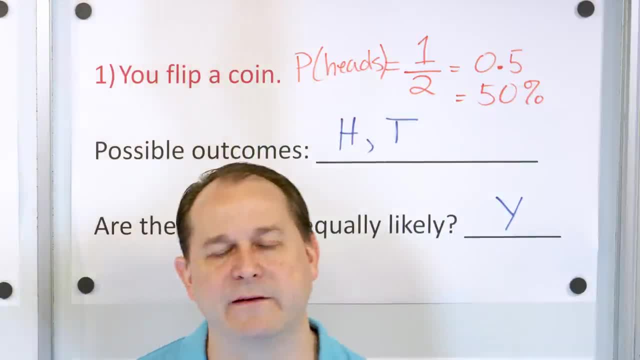 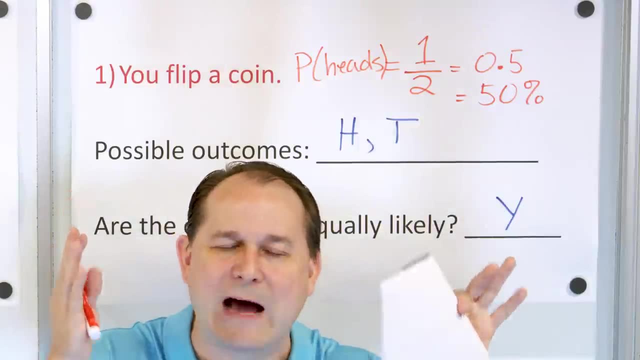 to see the observation of heads coming up half the time and tails coming up half the time. It's the same with the weather. If I take my day of weather, if the percent chance of rain is 50%, if I could somehow copy the day and run it over and over again for a million times. 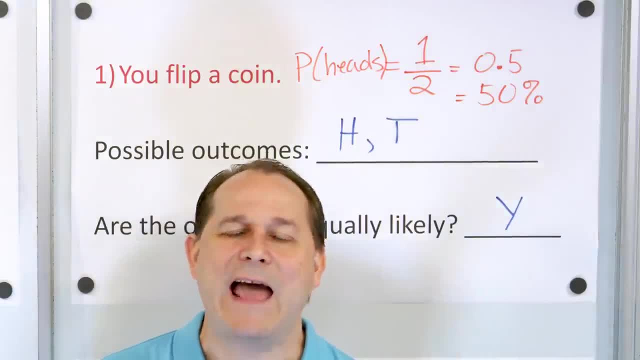 the probability would tell me that half of those times I should get heads and half of those times I should get tails, Five and five. If I flip a coin ten times, I should get five heads and five tails. But we all know that if you actually do that, 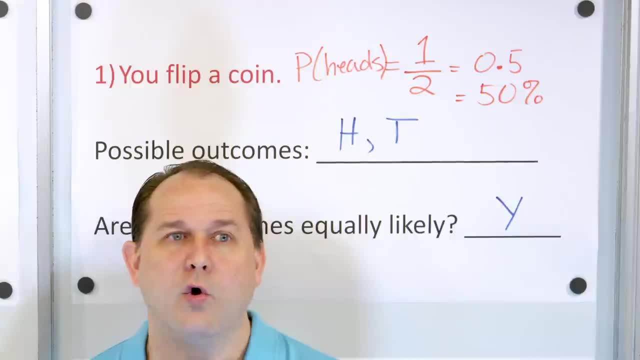 you might not get five and five. You might get like seven and three, or you might get six and four. It's not going to be exactly five and five for only ten trials, But if you flip the coin twenty times, you would expect five heads and five tails. 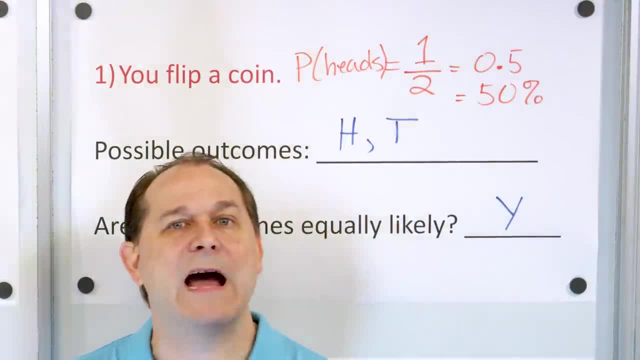 It might happen. but you might get maybe eleven heads and nine tails. They still have to add to twenty, right? But as I increase the number of trials, if I go to a thousand trials, right, then I should expect five hundred heads and five hundred tails, half and half. 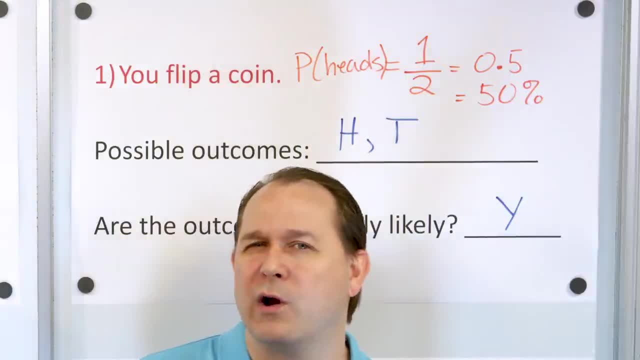 That's what the probability is telling me, But I might actually get more, like four hundred and ninety nine heads and five hundred and one tails. But you see, it's getting closer to half and half. If I run this experiment a trillion times, a trillion times, 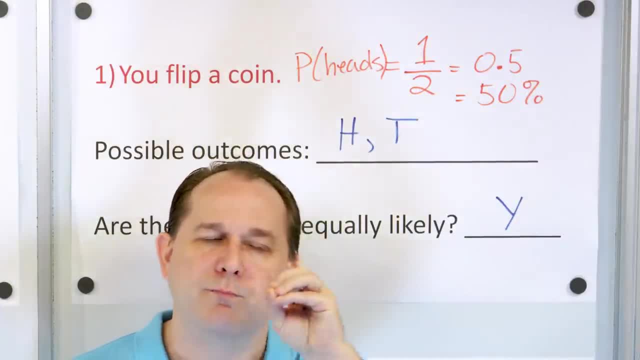 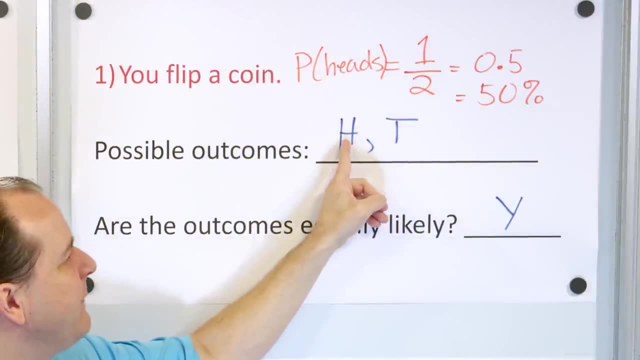 if I approach infinity number of trials. the more and more and more and more trials I do, the closer and closer I actually expect to see the observation of heads coming up half the time and tails coming up half the time. It's the same with the weather. 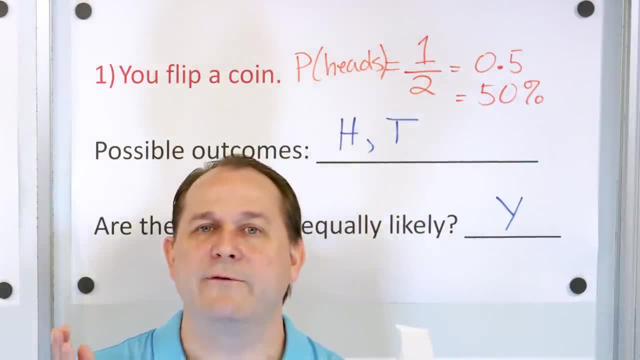 If I take my day of weather, if the percent chance of rain is 50 percent, if I could somehow copy the day and run it over and over again for a million times, I would expect half of those days to be raining and half of those days to not. 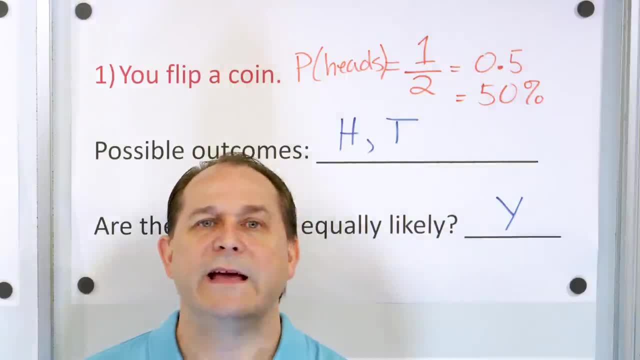 I would expect half heads and half tails for this probability. if I run it many, many times, do a thousand or a million trials, And the more trials I do, the closer I expect the probability to match reality. that I'm harping about it because a lot of students can calculate. 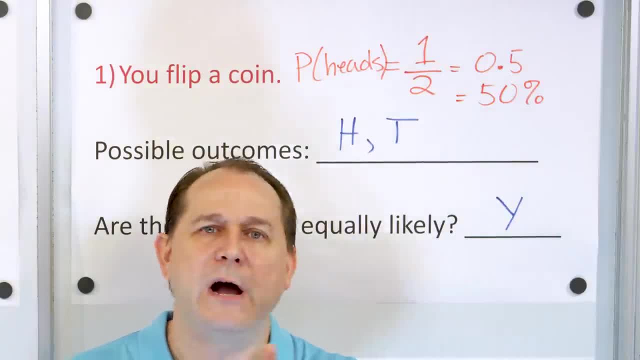 probability, but they don't know what it means. And that's what it means. It means do it a bunch of times, And the more times you do it, the closer what you observe will match what you have calculated. That's what probability is. 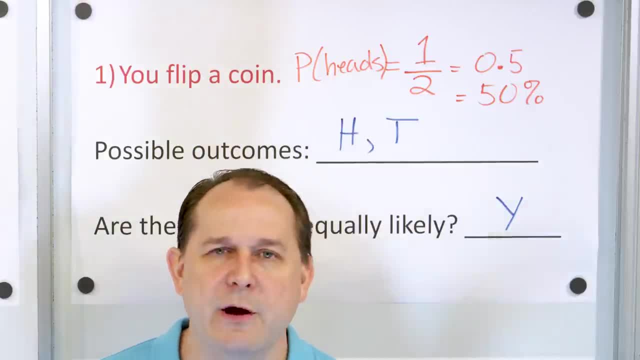 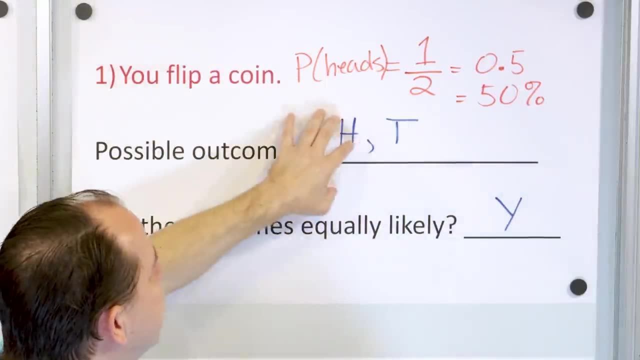 If I flip the coin three times, it doesn't tell me much at all, It's just a number. If I do it a thousand or a million times, it tells me a lot. All right, So let's put this one aside and move on, and 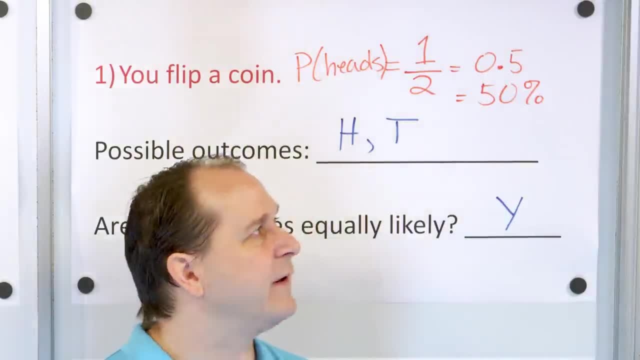 I would expect half of those days to be raining and half of those days to not. I would expect half heads and half tails for this probability. if I run it many, many times, do a thousand or a million trials, And the more trials I do, the closer I expect the probability to match reality. 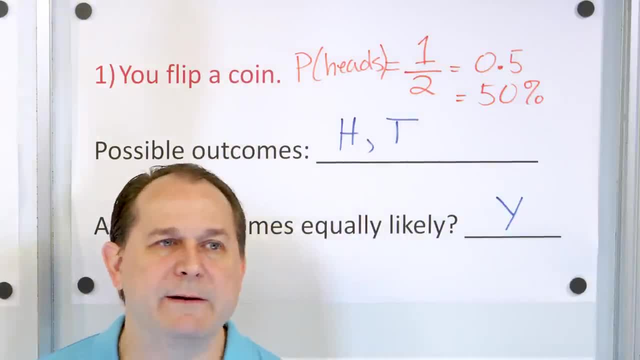 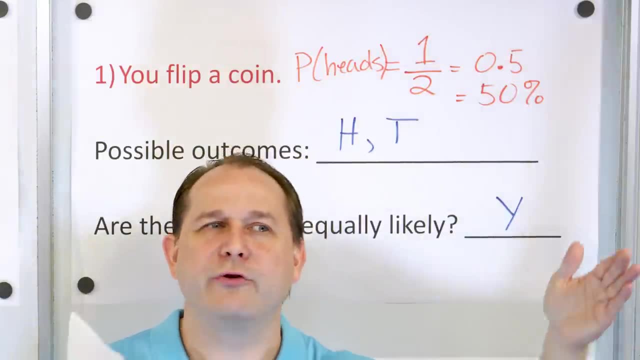 I'm harping about it because a lot of students can calculate probability, but they don't know what it means. And that's what it means. It means: do it a bunch of times, And the more times you do it, the closer what you observe will match what you have calculated. 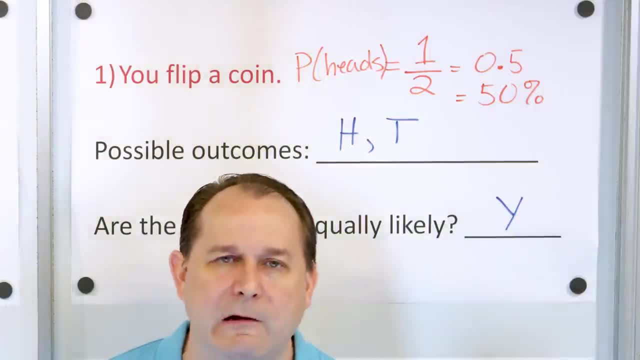 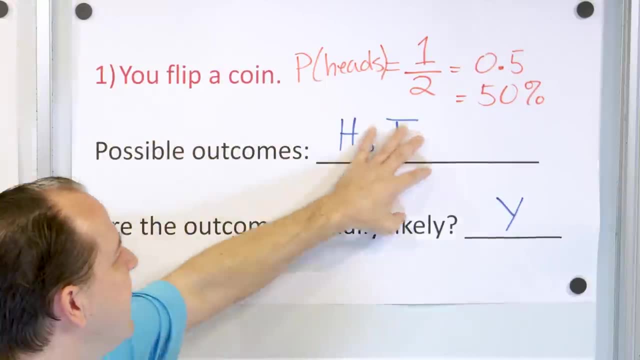 That's what probability is. If I flip the coin three times, it doesn't tell me much at all, It's just a number. If I do it a thousand or a million times, it tells me a lot, All right, So let's put this one aside and move on and continue on down the line. 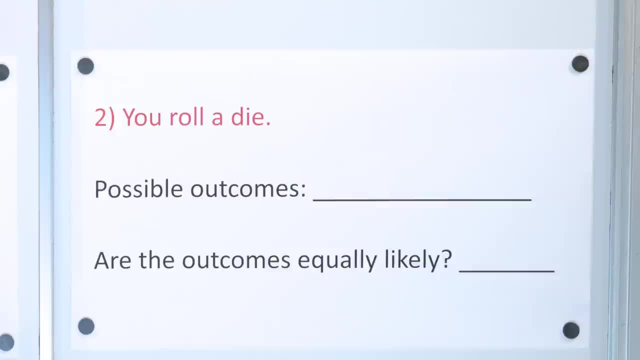 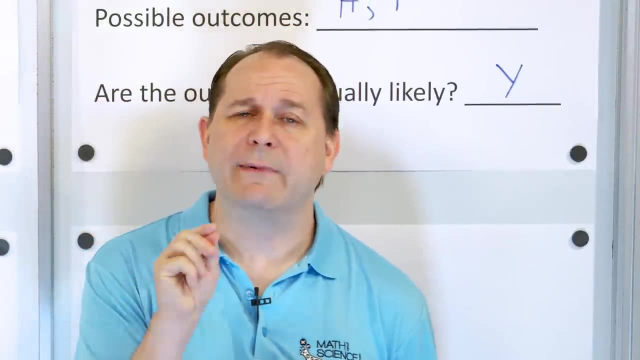 and learn about some other situations. Let's take a look at problem number two. Let's say I roll a die. Now, a die- I'm talking about a die- is like for a board game. it's a six-sided die. 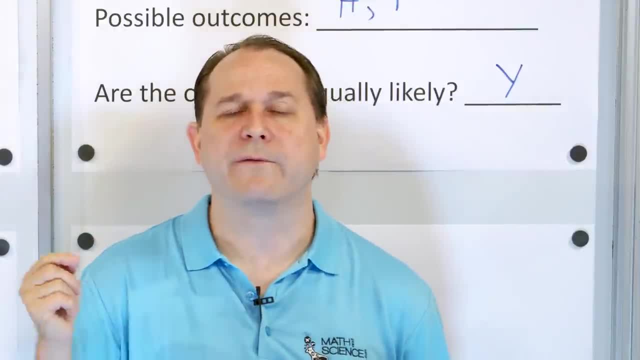 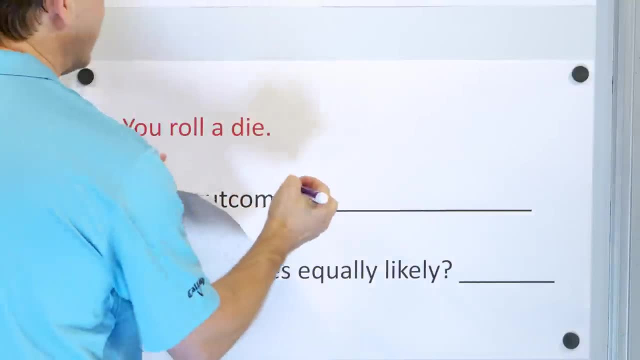 On the sides of the die have the little dots: one, two, three, four, five and six. All right. So I roll a die only one time. What are the possible outcomes if you roll that die? Well, there is no zero on the die, but there is a one, there is a two, 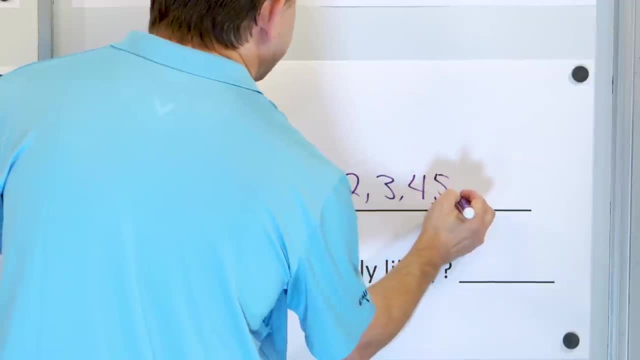 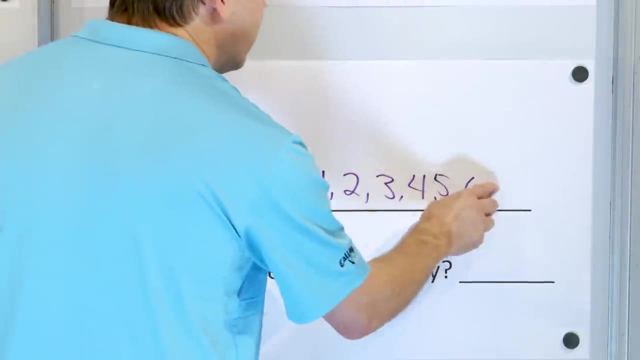 there is a three, there is a four, there is a five and there is a six. There's only one: two, three, four, five, six ways in which that thing can land, Each of these numbers, but there is no zero. 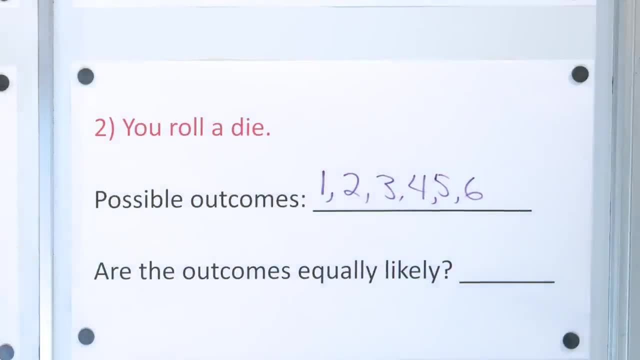 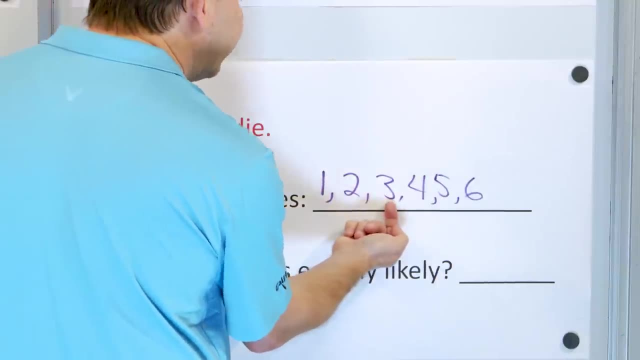 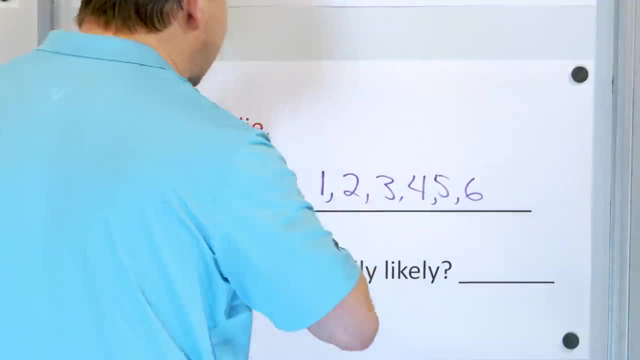 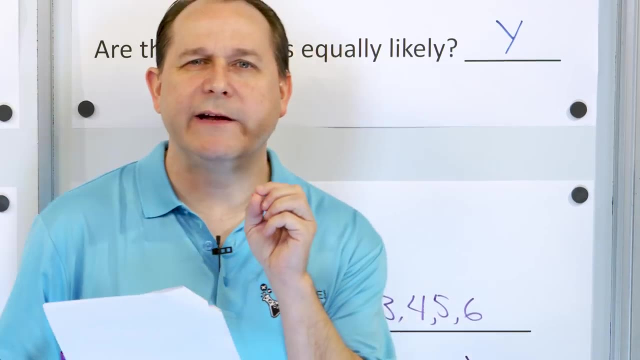 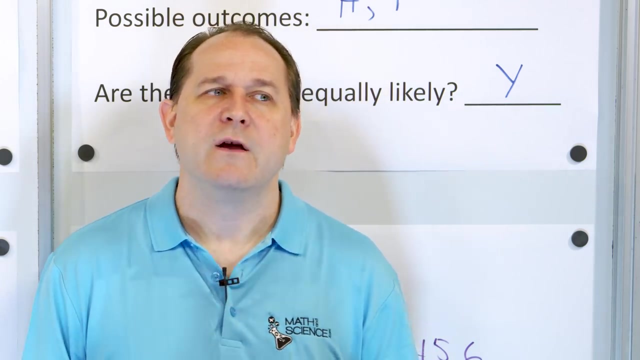 I only have one of these. So, because all of my outcomes only occur one time, are the outcomes equally likely? Yes, Let me ask you a question. If I constructed a new kind of die- let's say I constructed a new kind of die or I chiseled, I actually modified the die, okay? 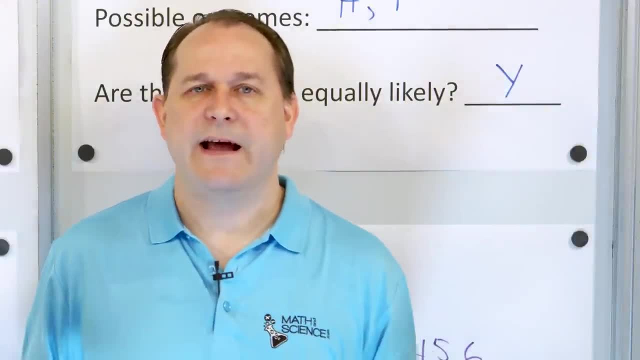 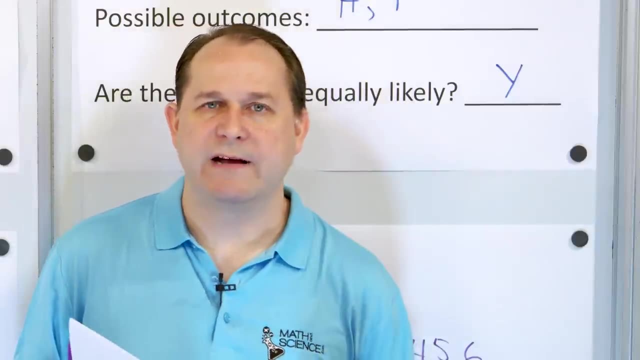 So normal die has one, two, three, four, five, six on there. Now let's say that I change it where I put. let's say I change it where I put: a one on one side, another one on another side. 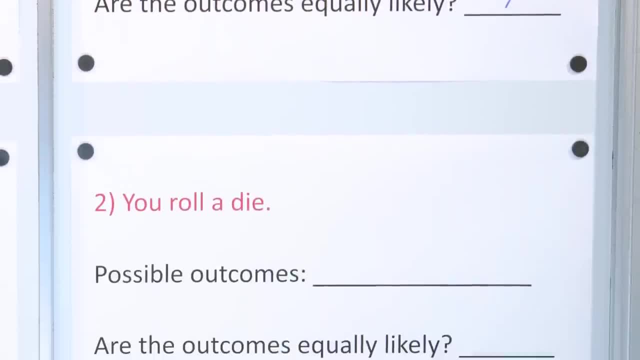 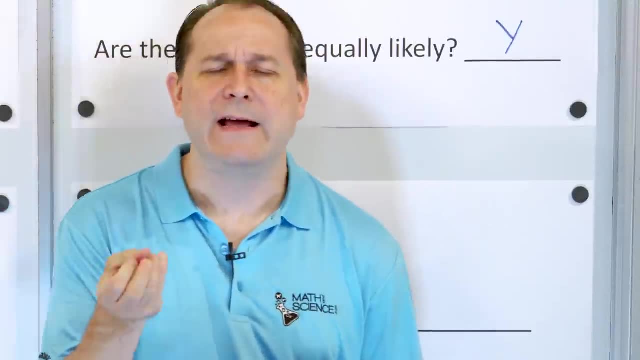 continue on down the line and and learn to have other situations. Let's take a look at problem number two. Let's say I roll a die, Now a die I'm talking about a die is like for a board game. It's a six sided die on the sides of the die. 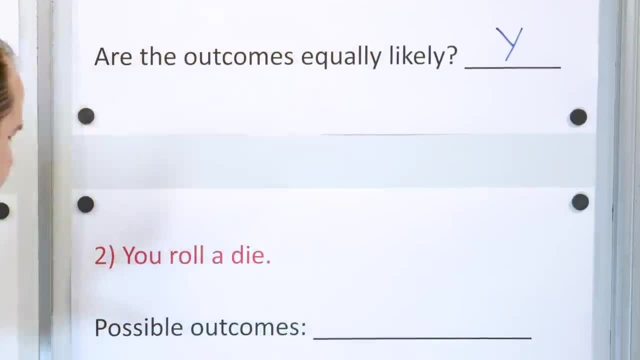 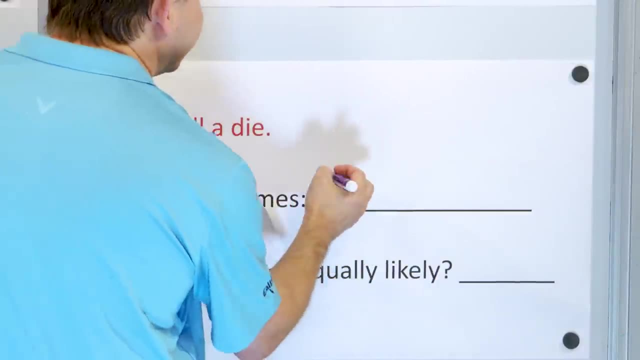 Have the little dots: one, two, three, four, five and six. All right, So I roll a die only one time. What are the possible outcomes if you roll that die? Well, there is no zero on the die, but there is a one. 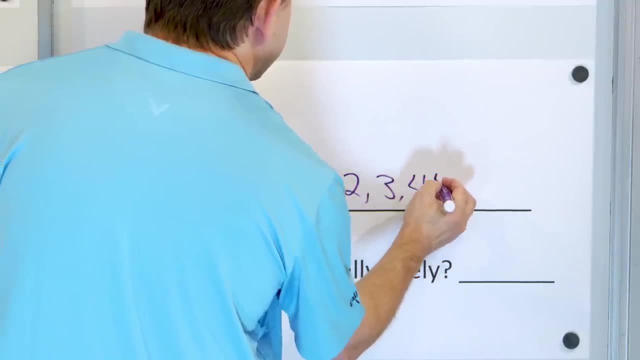 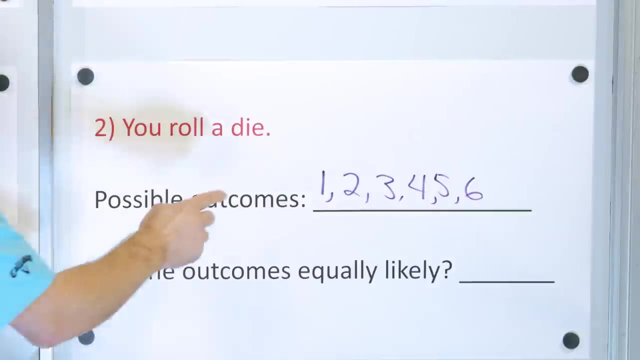 There is a two, There is a three, There is a four, There is a five and there is a six. There's only one: two, three, four, five, six ways in which that thing can land, each of these numbers, But there is no zero and there is nothing bigger than six. 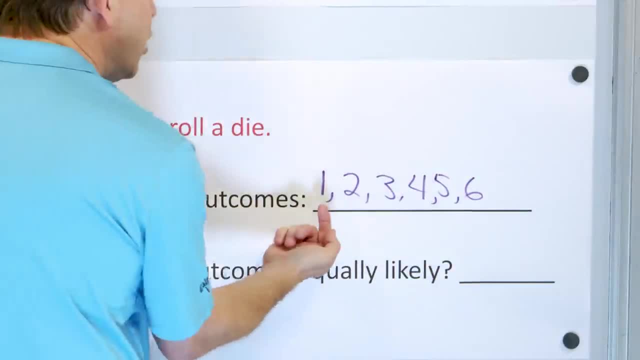 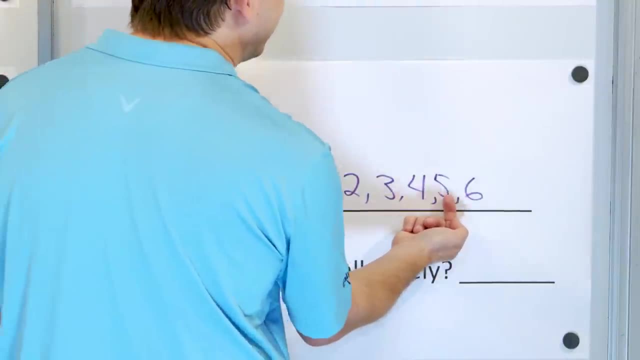 There's only six sides, Are the outcomes equally likely? Well, I only have one of the number ones. I only have one of these. I'll have one of these. I only have one of these. I only have one of these. I only have one of these. 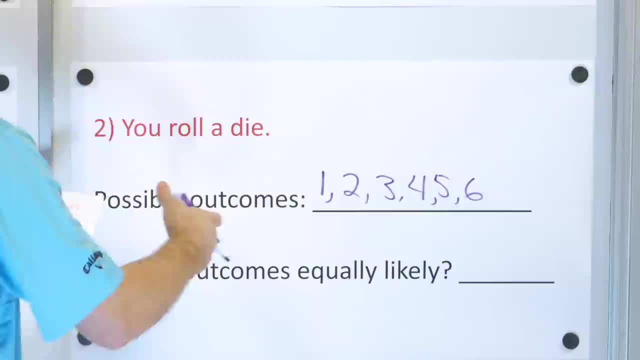 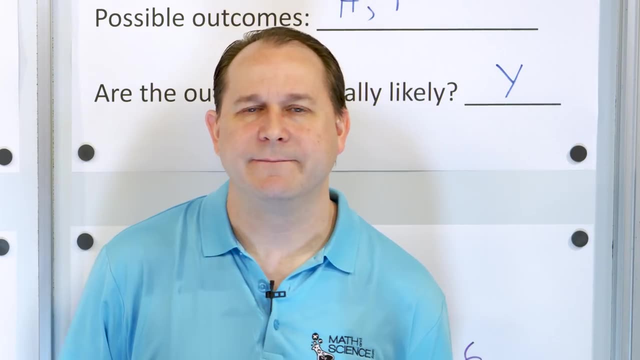 So, because all of my outcomes only occur one time, are the outcomes equally likely? Yes, Let me ask you a question. If I constructed a new kind of die, let's say I constructed a new kind of die or I chiseled, I actually modified the die. 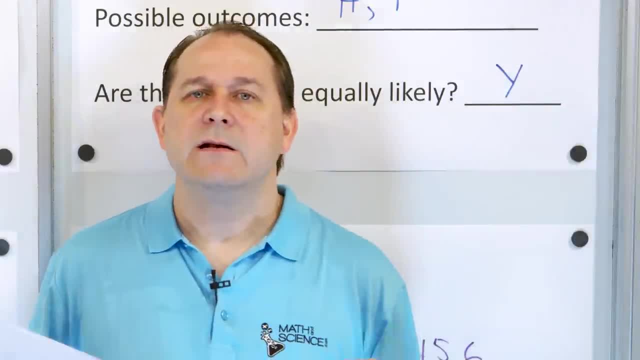 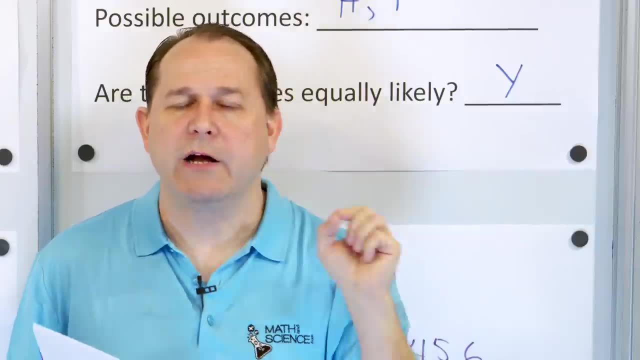 OK, so normal die, have one, two, three, four, five, six on there. Now let's say that I change it where I put. let's say I change it where I put a one on one side, another one on another side. 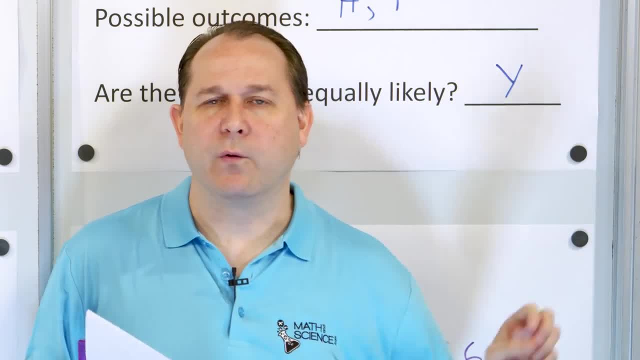 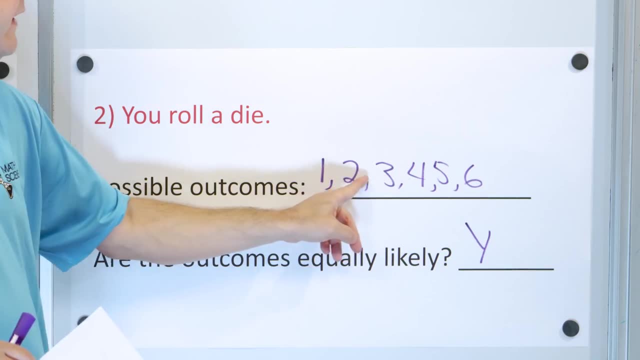 another one on another side, and then two, three and four. So in other words, I kind of erase some of the sides. So instead of, instead of having six unique independent outcomes, one for each side, instead of that I have a one, and then on another face. 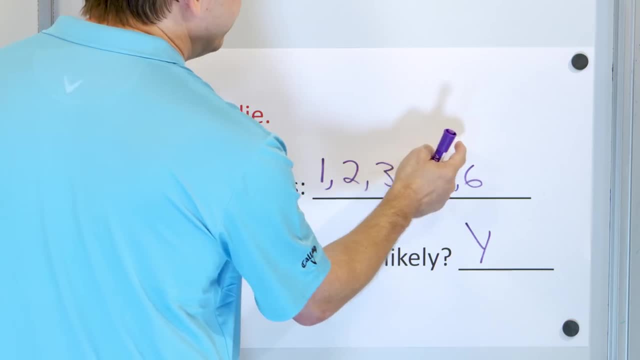 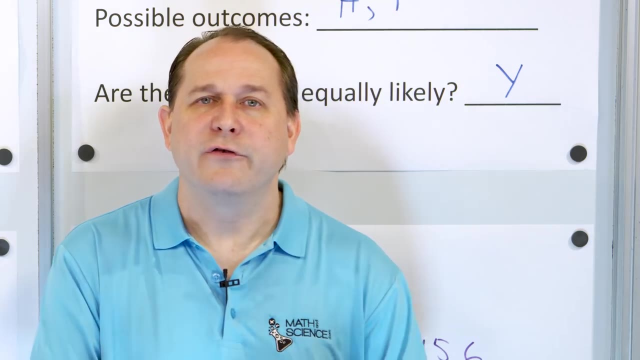 I have another one, and then, on another face, I have another one, And then I have two, three and four. Are those outcomes equally likely? Well, I have, you see, three sides with the same number. So if I roll that dice, 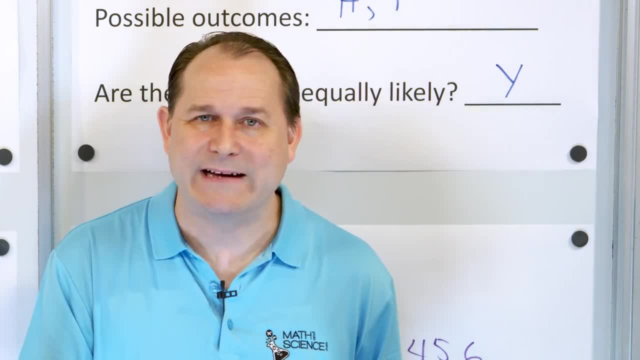 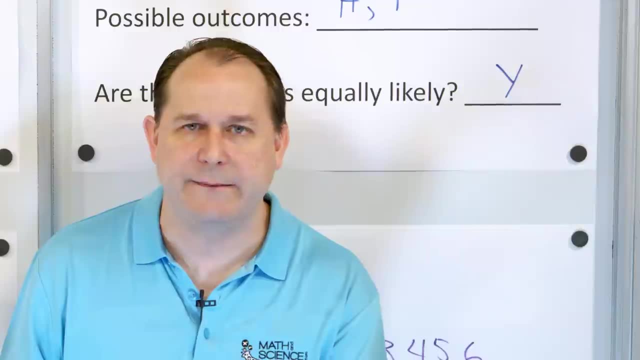 I'm going to expect to get the number one more often because there's more sides. So you see, in this case the outcomes are equally likely because all of the outcomes, they all occur the same number of times. The same thing is here. 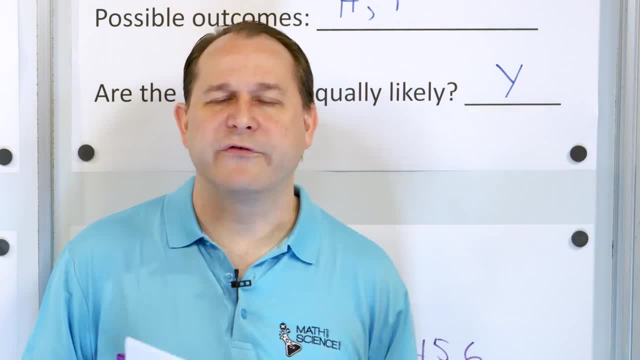 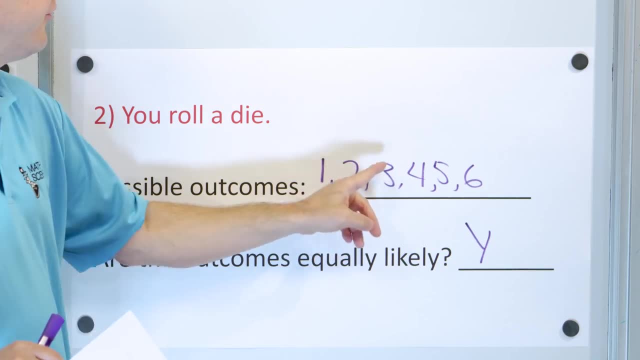 another one on another side, and then two, three and four. So in other words, I kind of erase some of the sides. So instead of having six unique independent outcomes, one for each side, instead of that I have a one, and then on another face I have another one. 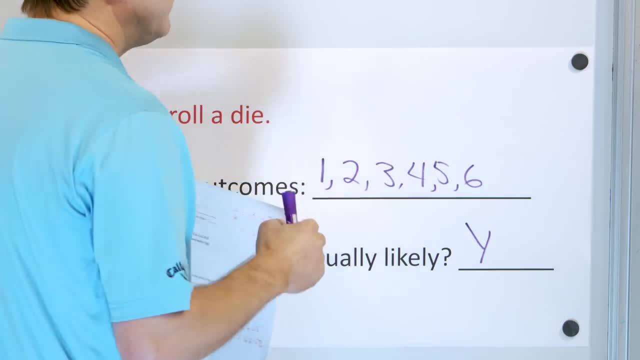 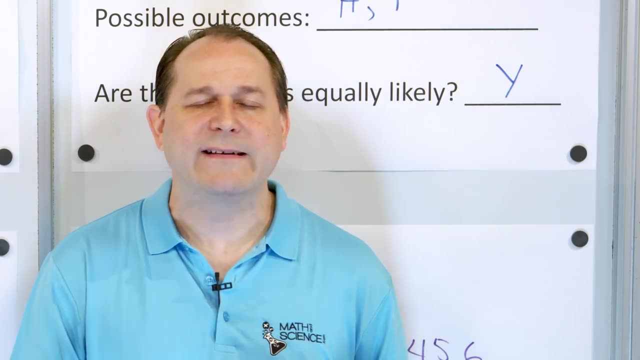 and then, on another face, I have another one, and then I have two, three and four. Are those outcomes equally likely? Well, I have, you see, three sides with the same number. So if I roll that dice, I'm going to expect to get the number one more often. 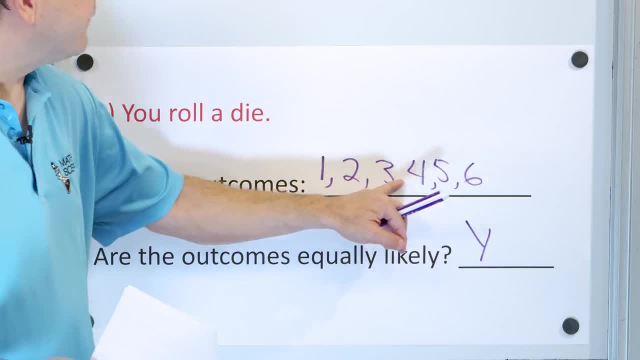 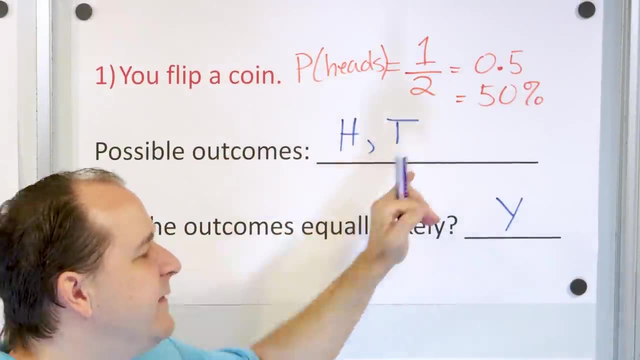 because there's more sides. So you see, in this case the outcomes are equally likely because all of the outcomes, they all occur the same number of times. The same thing is here: The outcomes, heads and tails. they only occurred one time each. 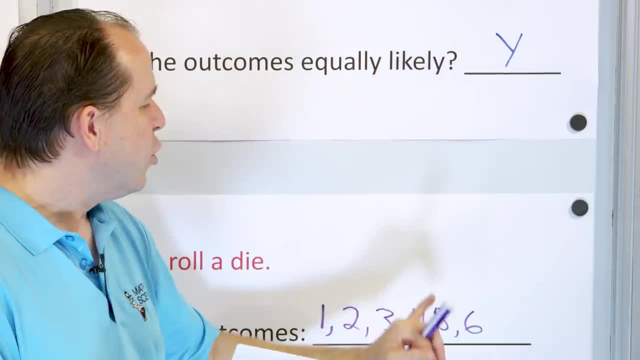 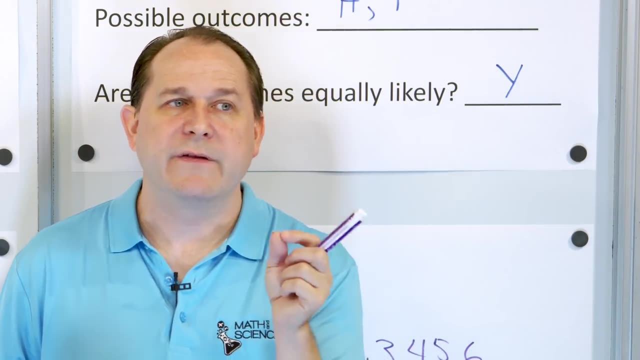 so we expected the outcomes to occur the same number of times, So we expect the outcomes to be equally likely. We expect the outcomes to be equally likely here because all of the outcomes only occurred one time. But if I modify the die so that I actually make three different faces, 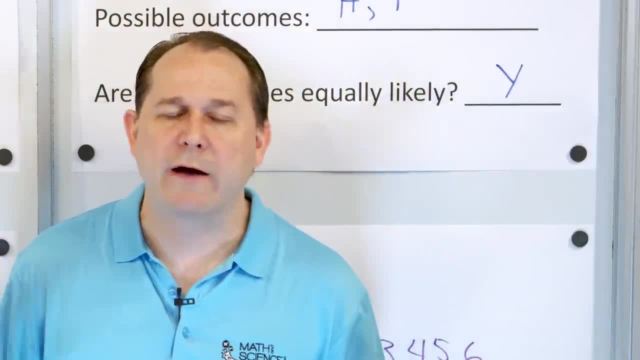 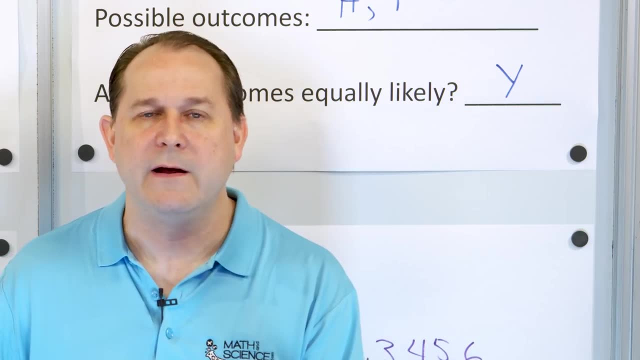 have the same number, then of course I'm going to expect to get that number more often and the outcomes will not be equally likely. They will not be equally likely because I would expect to get a three more often, I'm sorry, a one more often, if I, you know, put three faces of the die. 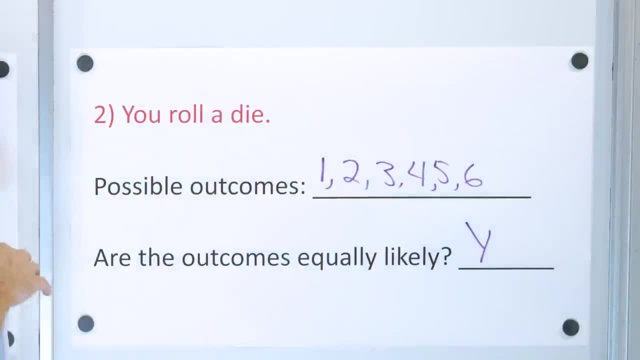 with the number one on there. So that is what I'm talking about. by equally likely, You get equal likeliness when all of the outcomes occur the same number of times and none of them is occurring more often. All right, Now just for giggles again. we're not teaching this yet. 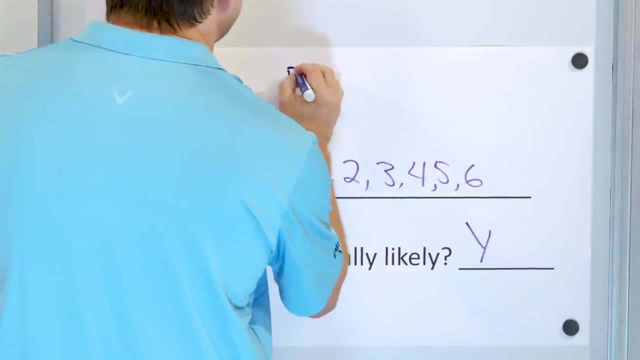 but let's see if we can figure out what the probability of rolling the number one is. What is the probability of rolling number one? Well, what you do is the same as we did up here For the probability of heads. we first had to identify how many ways in which heads can come up. 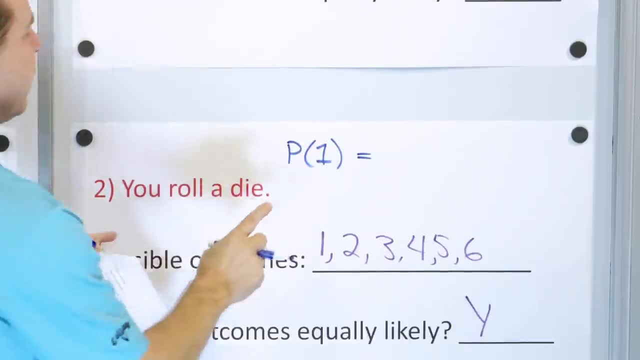 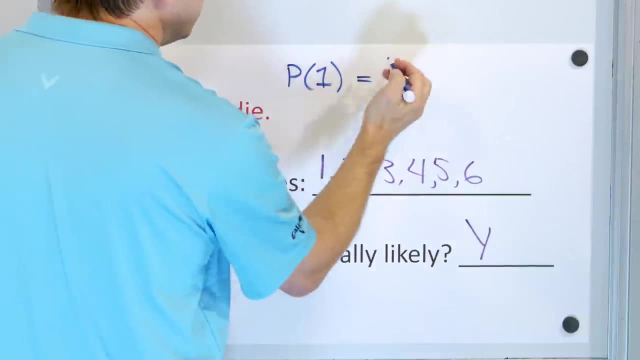 and then how many total outcomes are there for a trial. So we're going to do the same thing here. How many ways can the number one come up? Well, there's only one side with the number one, So there's only one way in which I can get a number one. 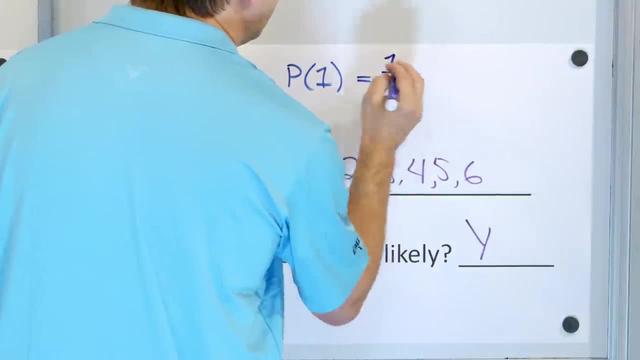 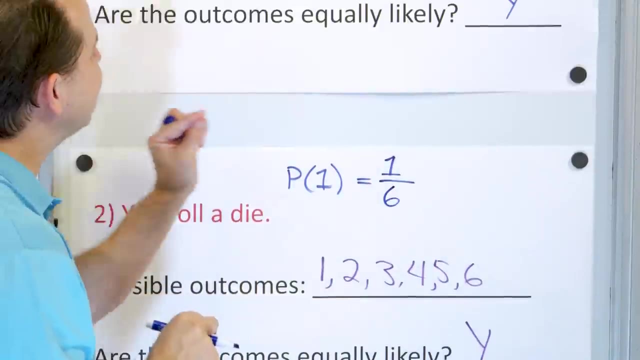 because all the other sides are different numbers right Now. how many total outcomes do I have? I have six total outcomes, So it's out of a total of six. It's exactly the same thing we did here. Probability of heads was one half because it was one way of getting a head out of a possible of two total outcomes. 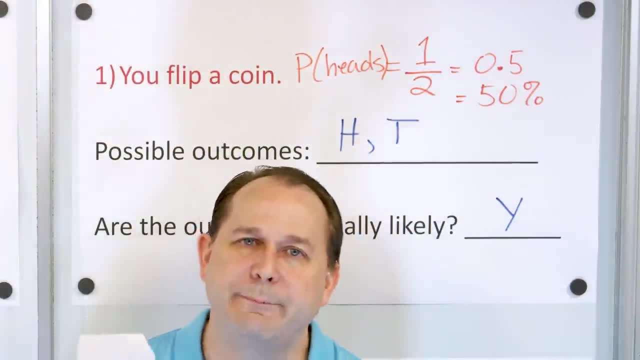 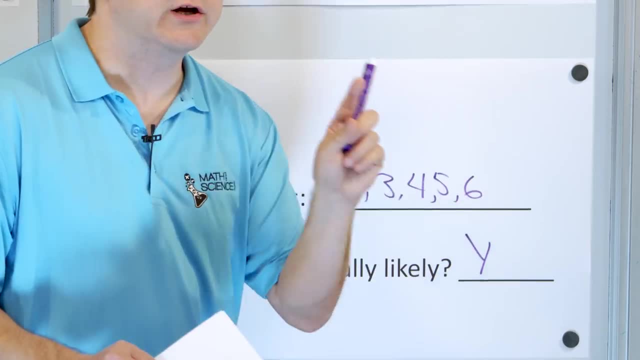 The outcomes heads and tails. They only occurred one time each, So we expected the outcomes to be equally likely. We expect the outcomes to be equally likely here because all of the outcomes only occurred one time. But if I modify the die so that I actually make three different faces, have 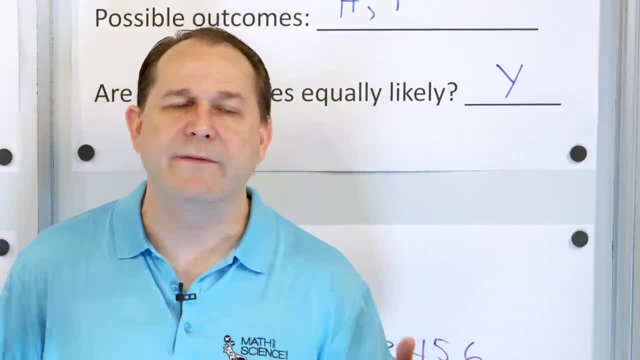 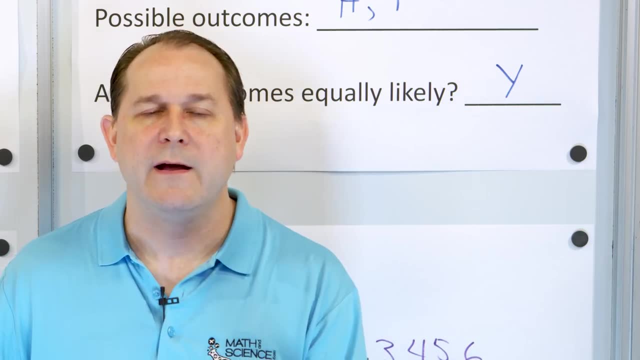 the same number, then of course I'm going to expect to get that number more often and the outcomes will not be equally likely. They will not be equally likely because I would expect to get a three more often, I'm sorry, a one more often. 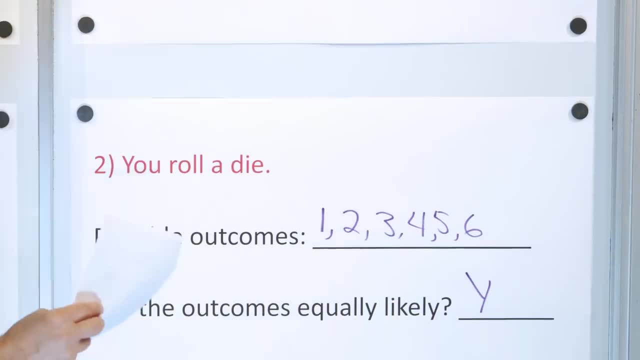 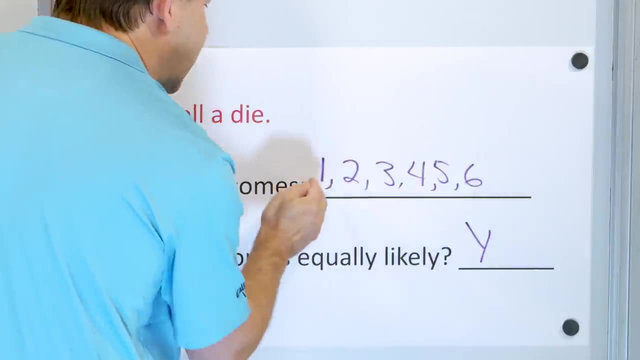 If I, you know, put three faces of the die to get the number one on there. So that is what I'm talking about. by equally likely, You get equally equal likeliness when all of the outcomes occur the same number of times and none of them is more. 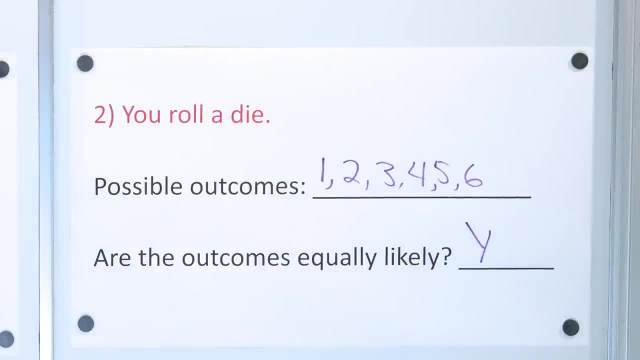 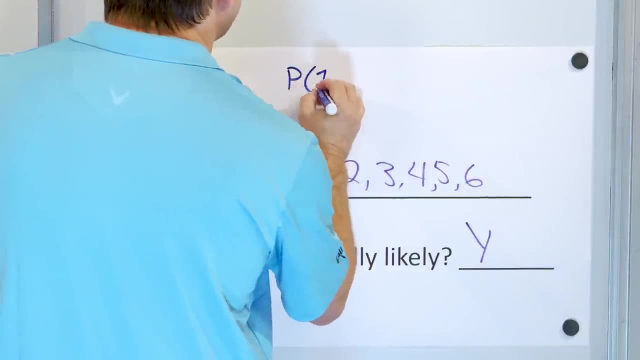 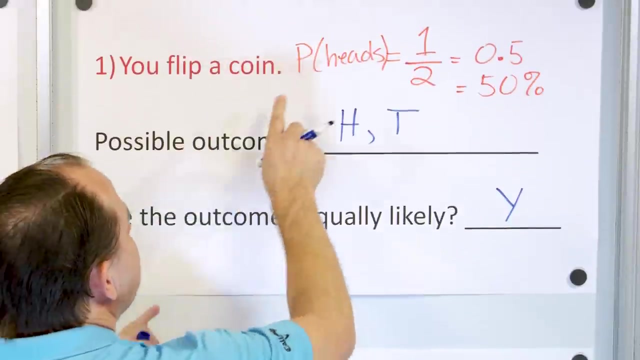 occurring more often. All right, Now just for giggles again, we're not teaching this yet, but let's see if we can figure out what the probability of rolling the number one is. What is the probability of rolling number one? Well, what you do is the same as we did up here for the probability of heads. 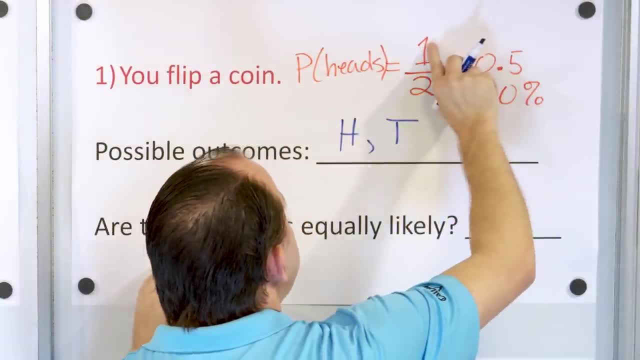 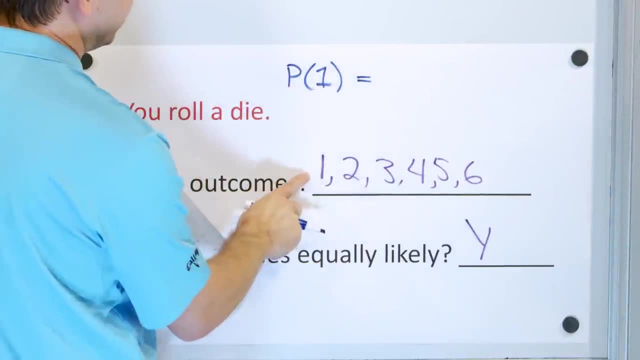 We first had to identify how many ways in which heads can come up, and then how many total outcomes are there for a trial. So we're going to do the same thing here. How many ways can the number one come up? Well, there's only one side with the number one. 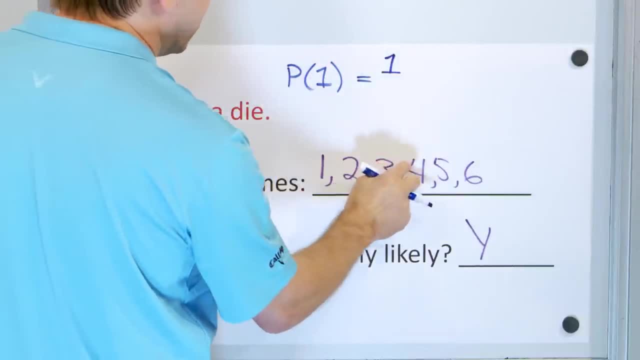 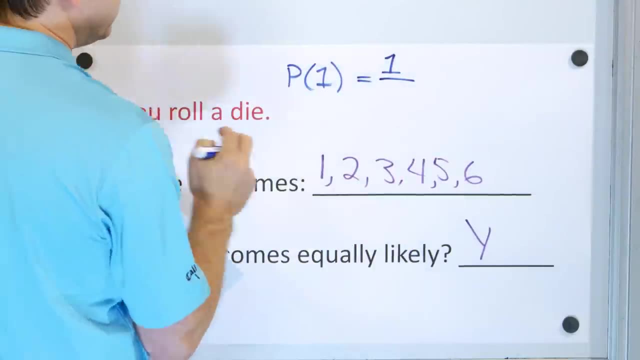 So there's only one way in which I can get a number one, because all the other sides are different numbers Right now. how many total outcomes do I have? I have six total outcomes, So it's out of a total of six. It's exactly the same thing we did here. 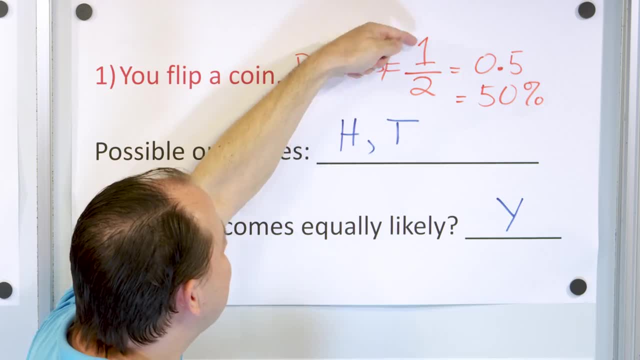 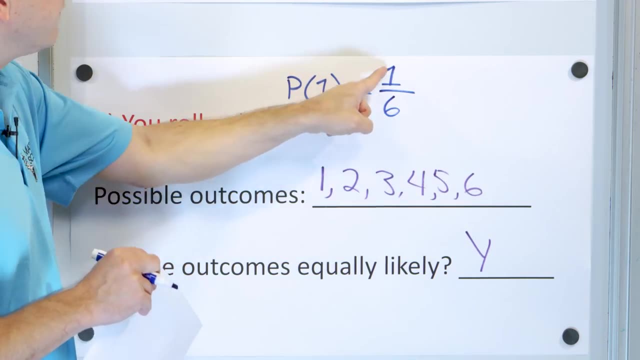 Probability of heads was one half because it was one way of getting a head out of a possible of two total outcomes. Here it's one way of getting a six out of a total possible six outcomes. So the probability of rolling a number one is six is one sixth. 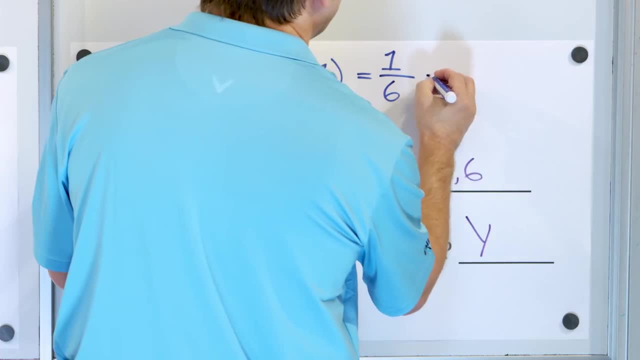 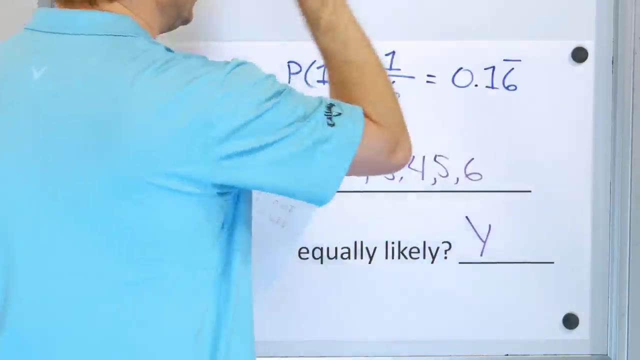 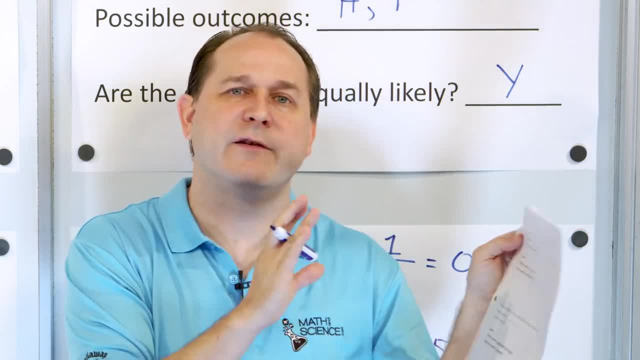 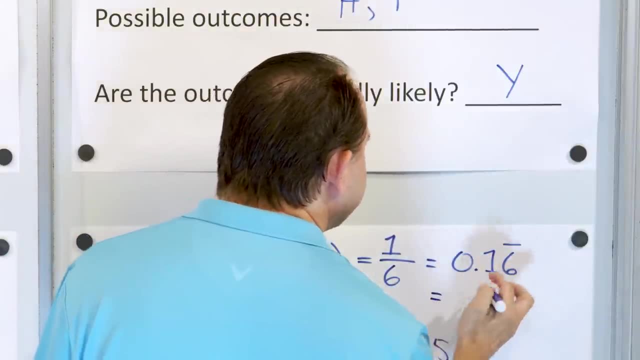 remember. we can express it as a decimal between zero and one is zero point one, six, repeating. Or you can express it as a fraction, one sixth. Or if you really want to express it as a percentage, multiply by one hundred and you'll get sixteen point six, repeating. 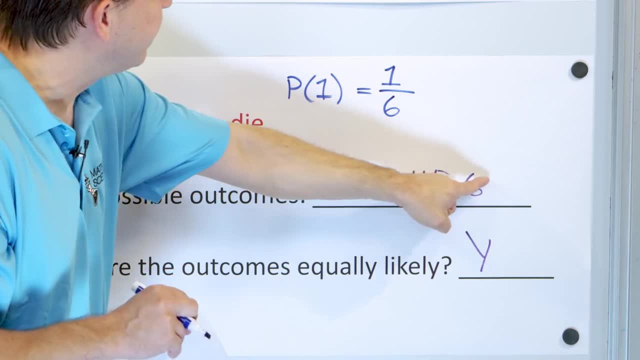 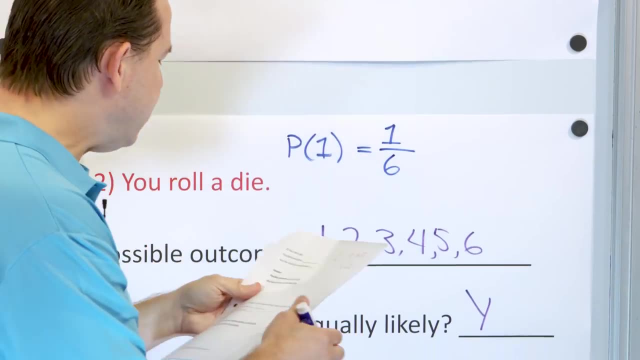 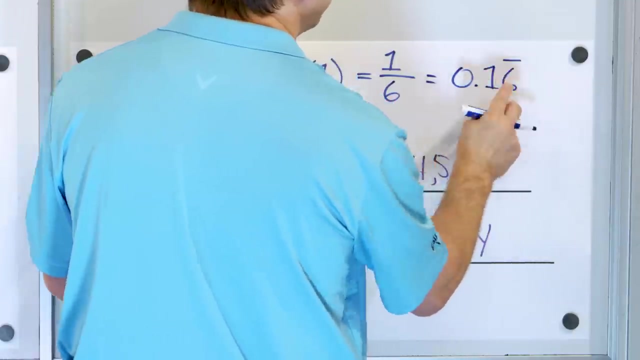 Here it's one way of getting a six out of a total possible six outcomes. So the probability of rolling a number one is six is one sixth. right Now, if you take one and you divide by six, you're going to get 0.16, with a repeating bar on the six: 0.16666666.. 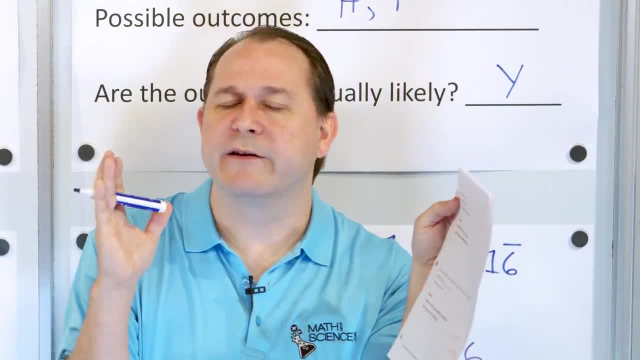 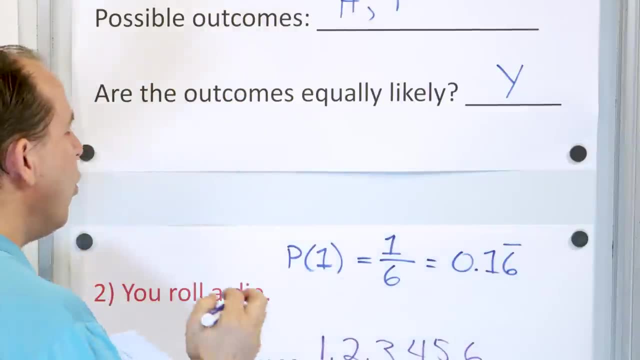 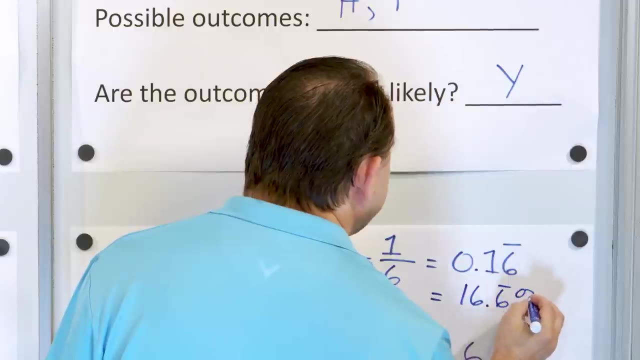 So the probability between zero and one- remember we can express it as a decimal- between zero and one- is 0.16 repeating. or you can express it as a fraction, one sixth. Or if you really want to express it as a percentage, multiply by a hundred and you'll get 16.6 repeating percent. 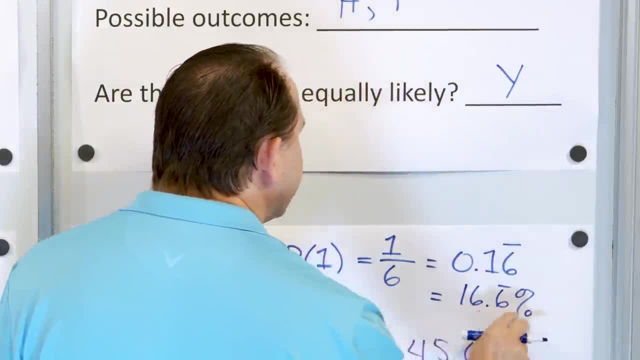 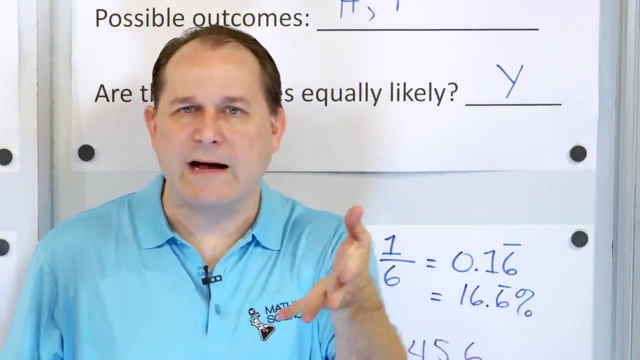 Because, don't forget, the sixes are going on. So if you move the decimal two spots, you'll get 16.6%. So what it means is, when you're going to a casino or just playing cards or whatever, if you roll a die, you expect to get a number one 16.6% of the time, right? 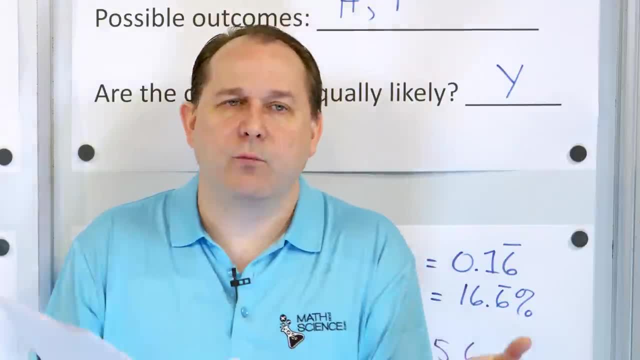 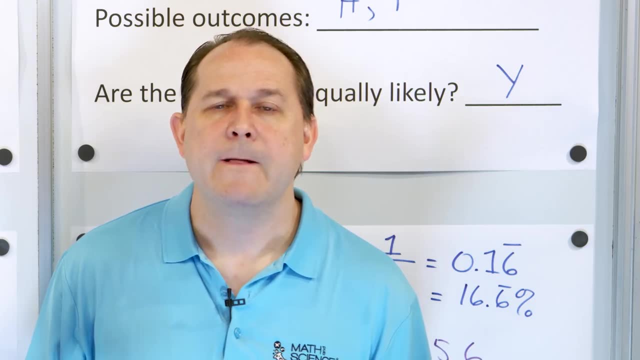 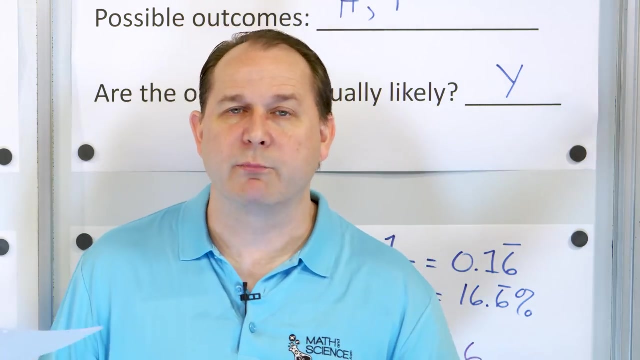 So what does that mean? right? What that means is that when I roll the die, I could get whatever I'm going to get. The percentage, or the probability is really telling you that if I roll that die a million times, then I would expect, with very high accuracy, to actually have 16 point, whatever percent of the number of rolls that I roll. 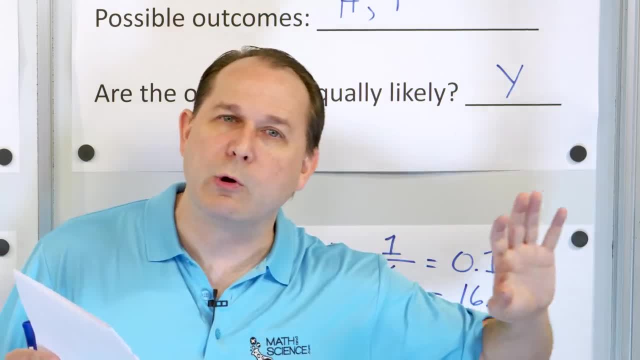 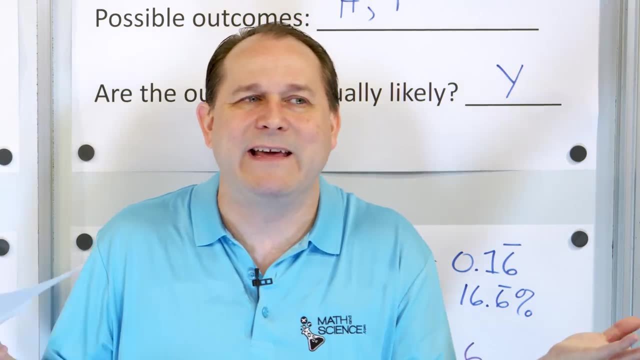 like a million rolls to actually be landing on the number one, And the more rolls that I roll the die, the more closely my observations will match with what I'm calculating here. If I only roll the die one time, I can get anything. 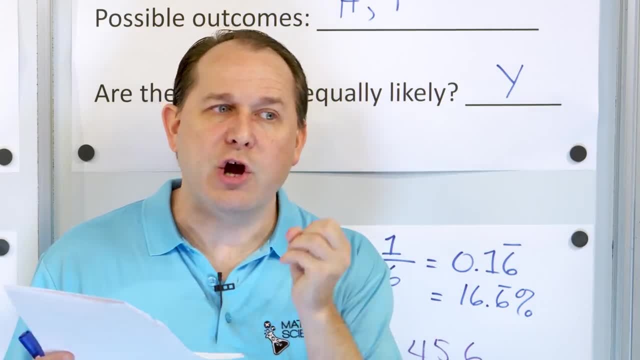 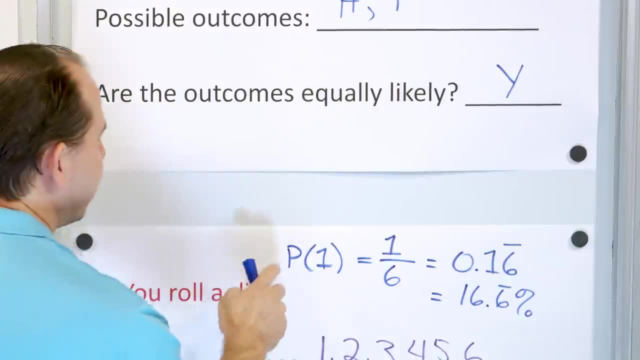 I can get a five or a four, or one, you know. But I know that as I increase the number one, the number of trials, what I observe is going to match what I calculate. Now let me ask you another question: What's the probability of getting a number three? 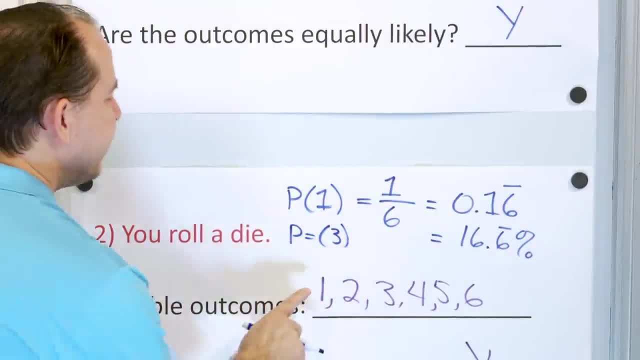 Well, it's the same thing. There's only one way of getting a three, but there's six total ways in which the die could fall. So the probability is one sixth. What's the probability of getting a four? It's also one sixth. 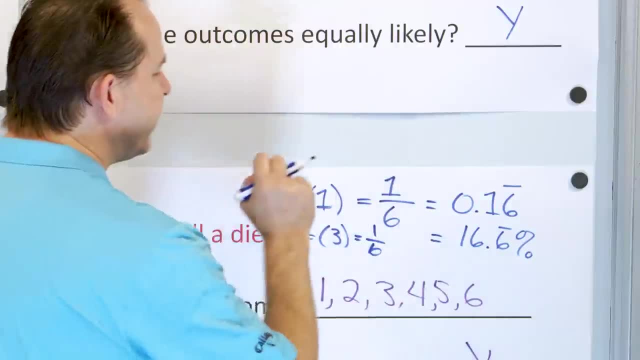 What's the probability of getting a five? It's also one sixth. What's the probability of getting a six? It's also one sixth Because, again, for all of them, there's only one way in which you can get the number, and there's six outcomes. 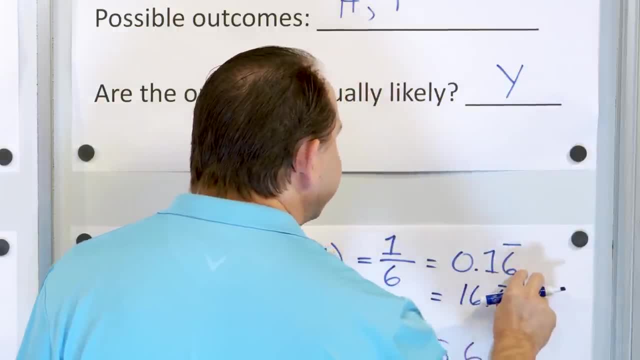 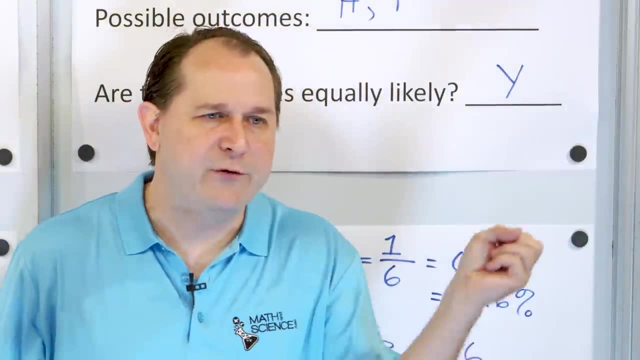 percent because, don't forget, the sixes are going on. So if you move the decimal two spots, you'll get sixteen point six percent. So what it means is when you're going to a casino or just playing cards or whatever, if you roll a die, you expect to get a number one, sixteen point six percent of the time. 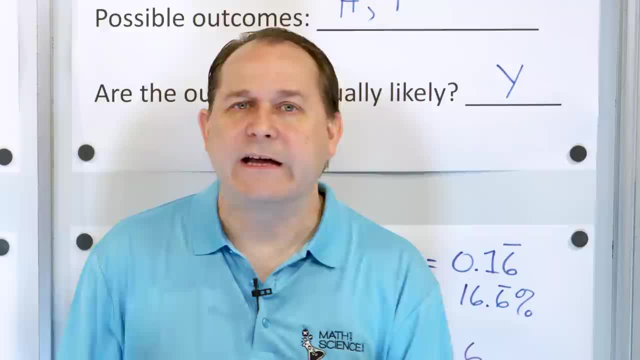 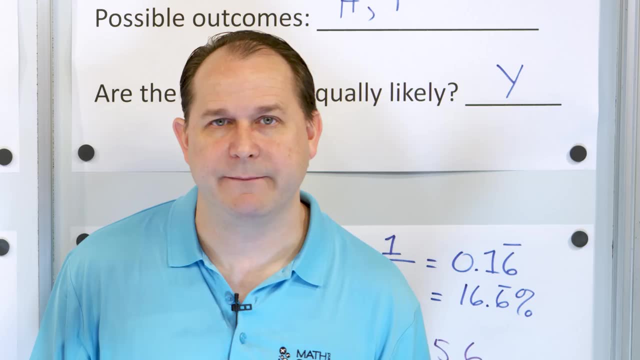 Right. So what does that mean, Right? What that means is that when I roll the die, I could get whatever I'm going to get, But the percentage or the probability is really telling you that if I roll that die a million times, then I would expect with very high accuracy. 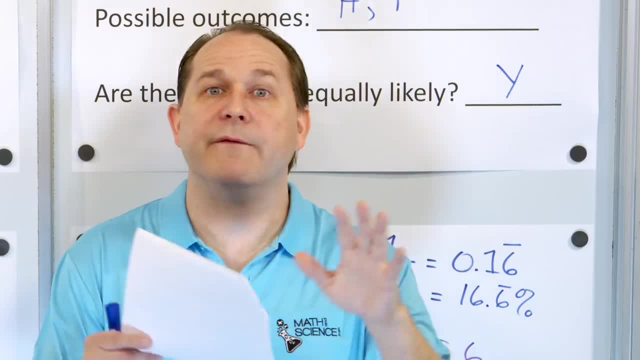 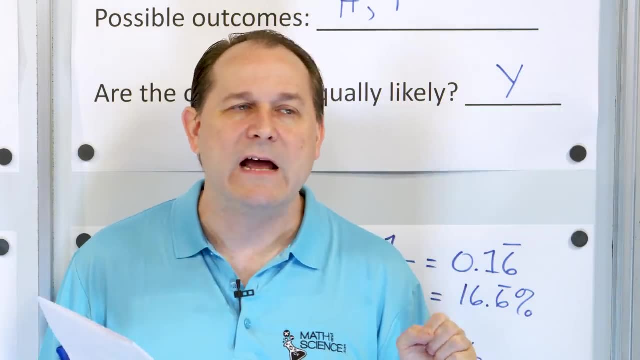 to actually have sixteen point, whatever percent of the number of rolls that I roll, like a million rolls, to actually be landing on the number one, And the more rolls that I roll the die, the more closely my observations will match with what I'm calculating here. 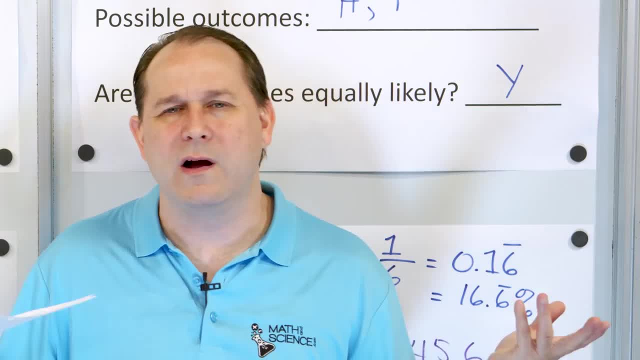 If I only roll the die one time, I can get anything. I can get a five or four or one, you know. but I know that As I increase the number of trials, what I observe is going to match what I calculate. 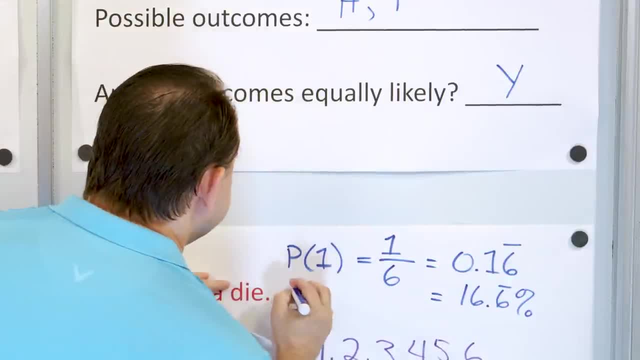 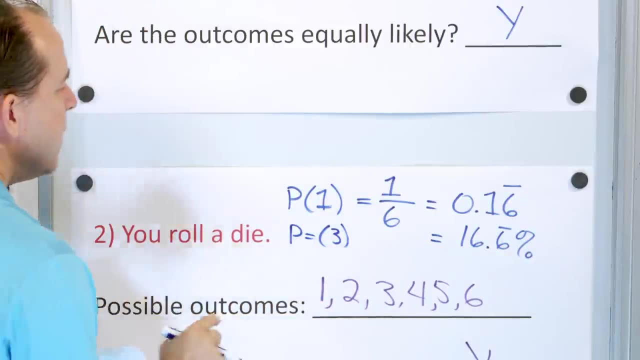 Now let me ask you another question: What's the probability of getting a number three? Well, it's the same thing. There's only one way of getting a three, but there's six total ways in which the die could fall. So the probability is one sixth. 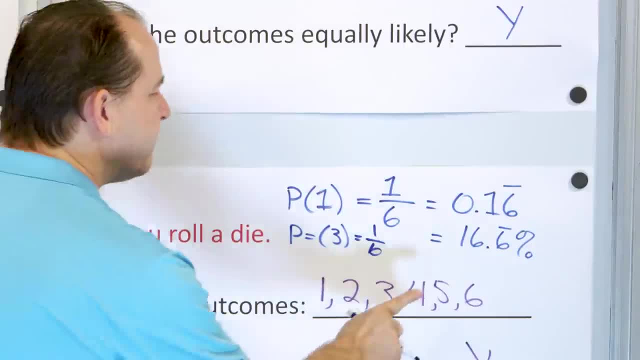 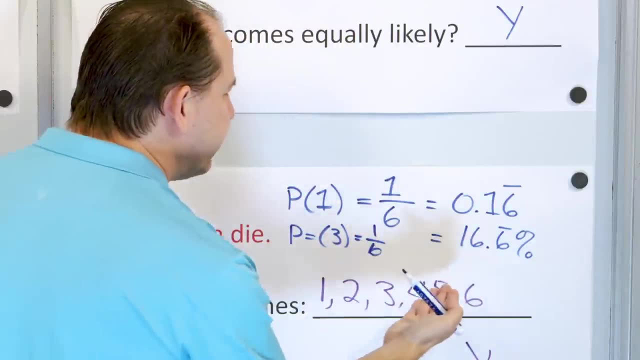 What's the probability of getting a four? It's also one sixth. What's the probability of getting a five? It's also one sixth. What's the probability of getting a six? It's also one sixth Because, again, for all of them, there's only one way in which you can get the number, and there's six outcomes. 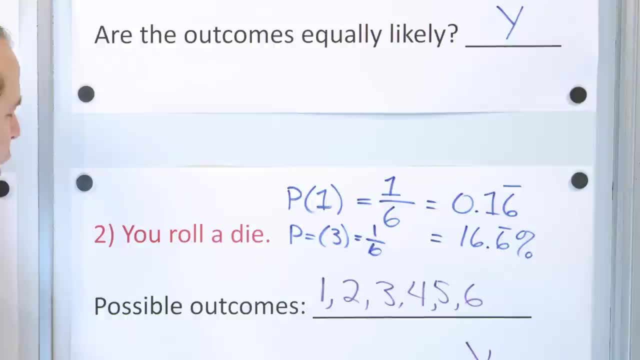 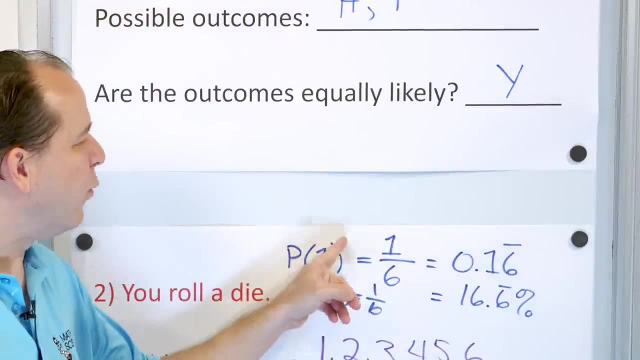 What's the probability of getting a two, One, sixth? So you see we answered. are the outcomes equally likely? Yes, But now we're proving mathematically that equally likely. because if you get the probability of rolling a one or a two, or a three or four or a five or 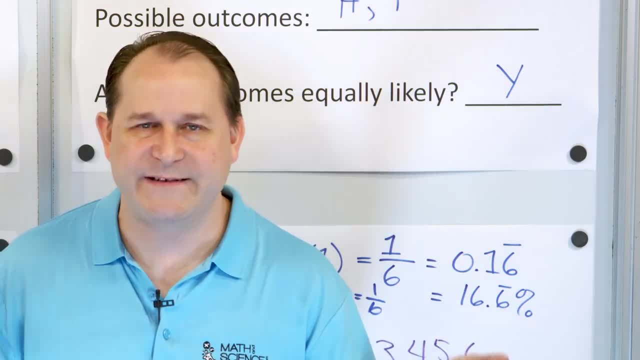 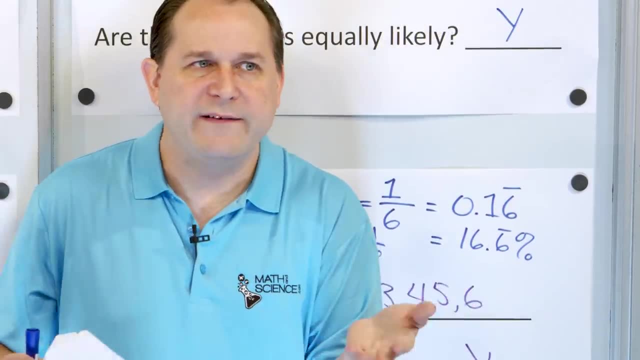 a six, all of the probabilities are the same. They're one sixth. That's why they're equally likely. So from an intuitive point of view, if all of the outcomes only occur once, it's equally likely. But if you can prove it mathematically, 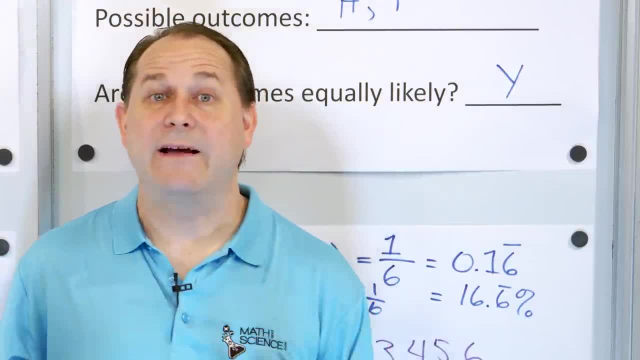 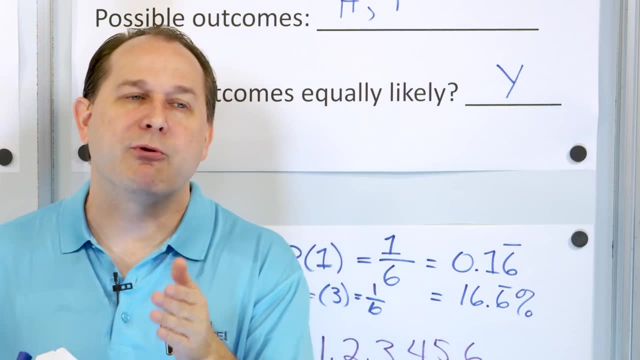 by calculating the probability of of doing that. Now let me ask you a question. The probability of getting a number one is one sixth. The probability of getting a number two is also one sixth. The probability of getting a number three is also one sixth. 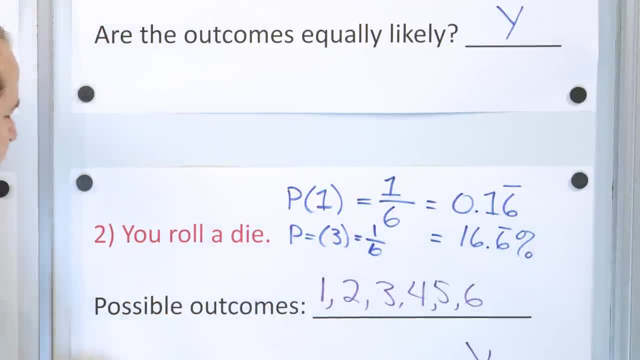 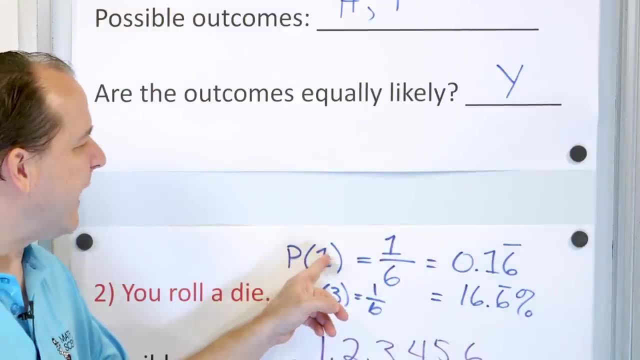 What's the probability of getting a two, One, sixth? So you see we answered. are the outcomes equally likely? Yes, But now we're proving mathematically that equally likely, because if you get the probability of rolling a one or a two or a three or a four or a five or a six, 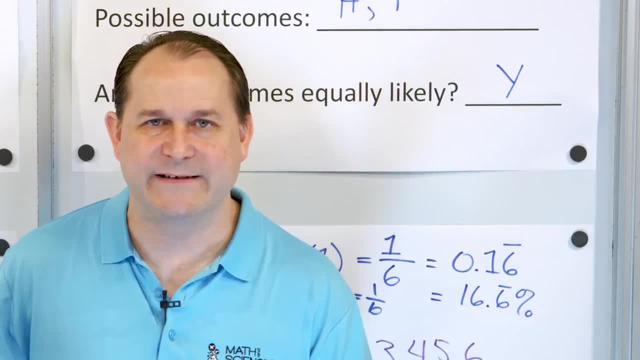 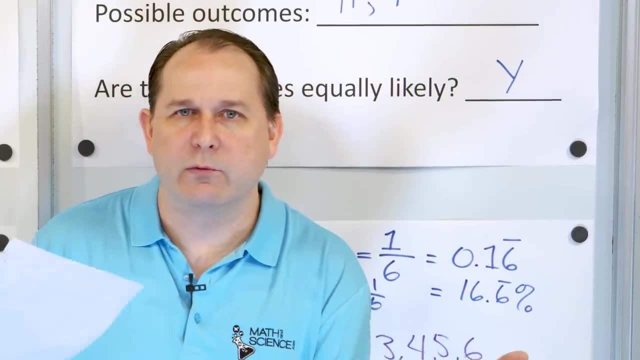 all of the probabilities are the same. They're one sixth. That's why they're equally likely. So from an intuitive point of view, if all of the outcomes only occur once, it's equally likely. But if you can prove it mathematically by calculating the probability of doing that, 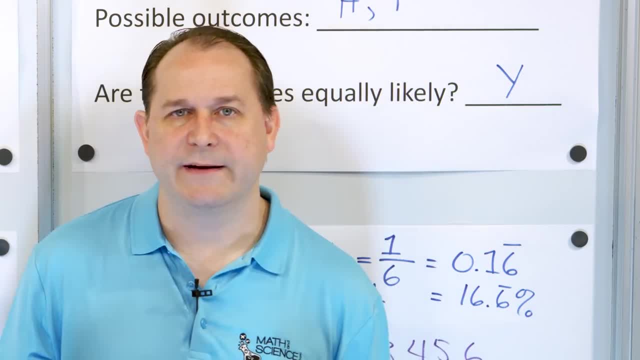 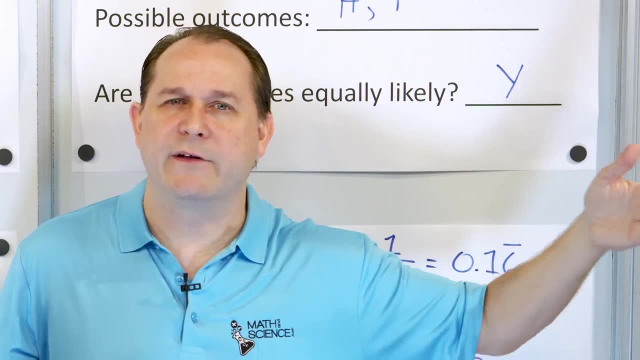 Now let me ask you a question. The probability of getting a number one is one sixth. The probability of getting a number two is also one sixth. The probability of getting a number three is also one sixth, And on and on down the line for all of the faces of the die. 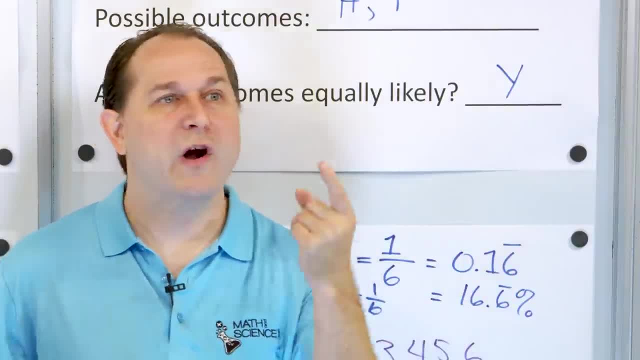 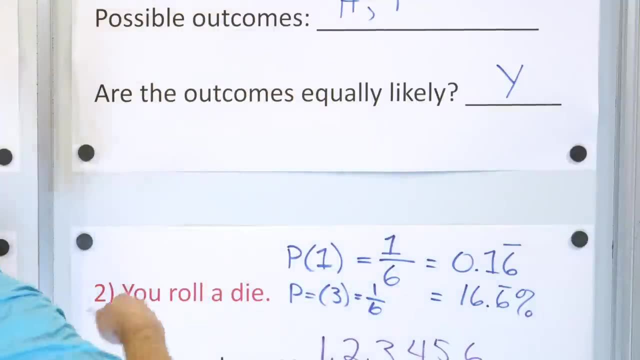 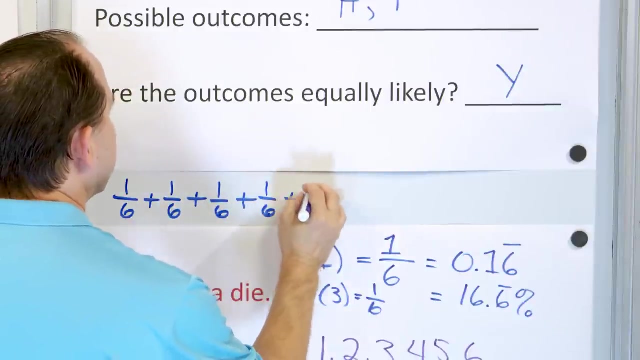 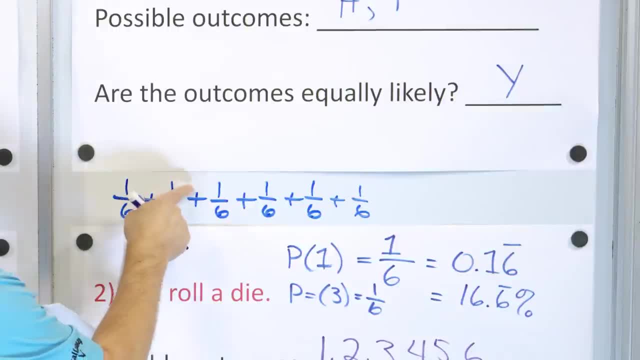 Well, this is the probability of rolling a one, the probability of rolling a two, the probability of rolling a three, the probability of rolling a four, the probability of rolling a five, the probability of rolling a six. We have a common denominator. 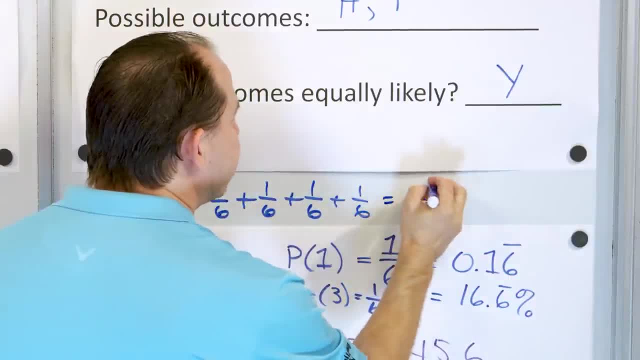 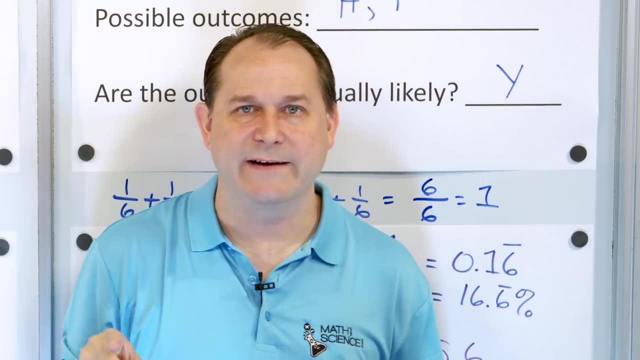 We keep it: one plus one plus one. add those together get six over six. Six over six is one. The probability of getting a one or a two or a three or a four or a five or a six is one. 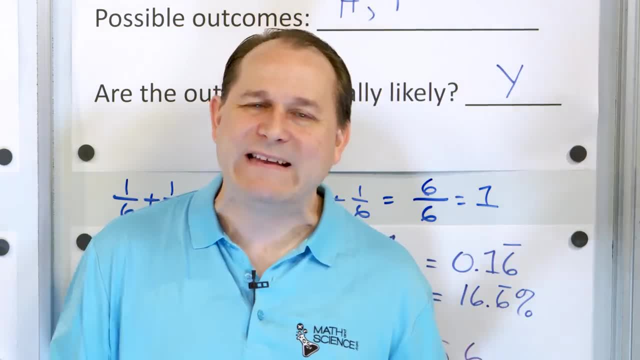 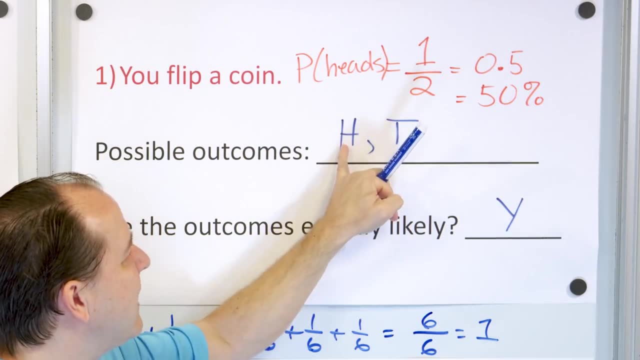 That means 100%. We're guaranteed to get one of these outcomes. when we take all the individual probabilities, they all have to add up to one And I've showed you that again up here: the probability of getting one half for this and one half for this. you add them, you get to one. 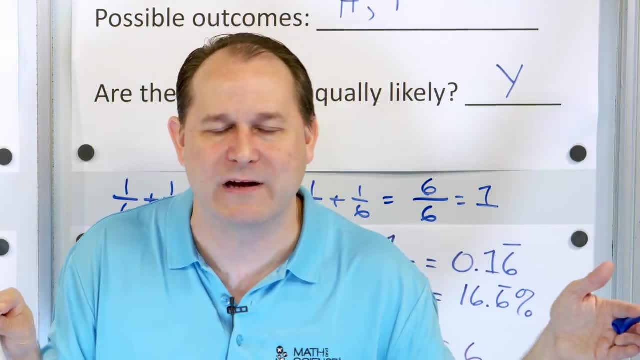 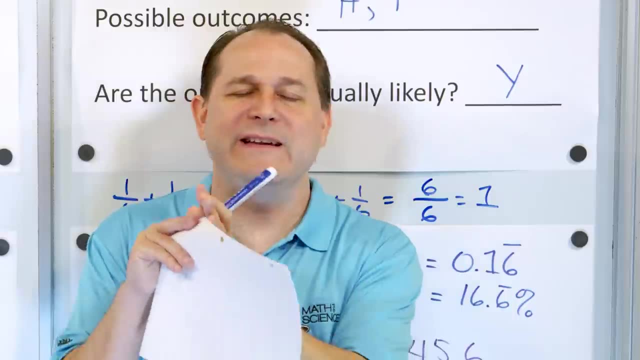 So when you look at probability, the probabilities of all the possible outcomes should always add up to one, because you're guaranteed to get one of those outcomes And so the probabilities have to add up to one. You see why I told you in the beginning. 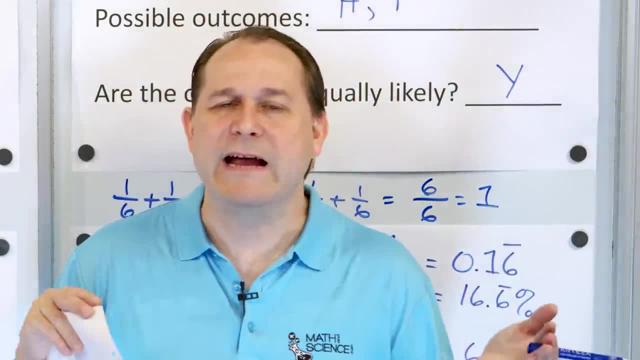 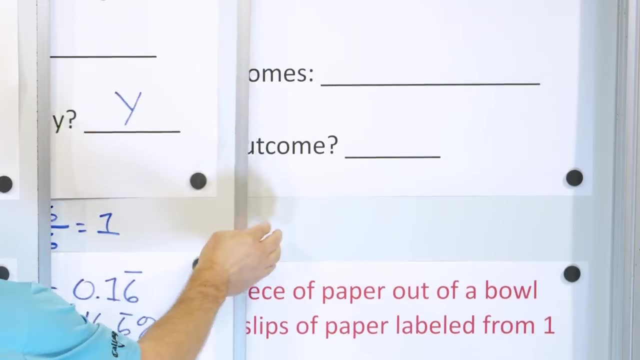 is that probability is just fractions. It's just literally an application of fractions, And I'm showing you that here. All right, let's go to something a little bit different. We've talked about flipping a coin. We've talked about rolling a die. 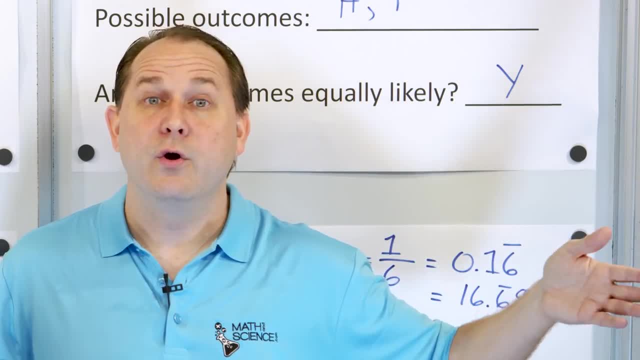 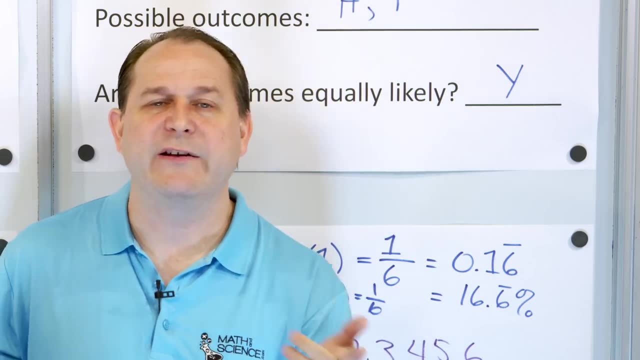 And on and on down the line for all of the faces of the die. So what's the probability of getting a number one or a number two, or a number three or a number four or a number five or a number six? We just add the probabilities. What is? we'll do it right here. 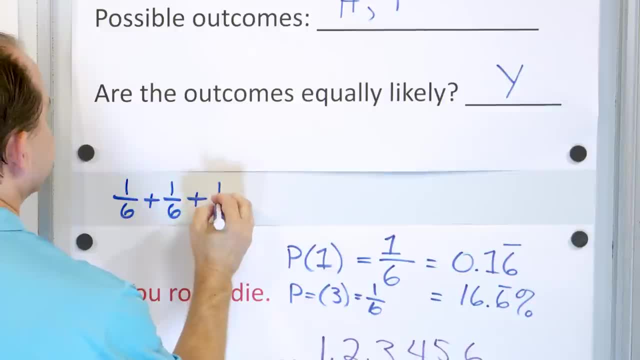 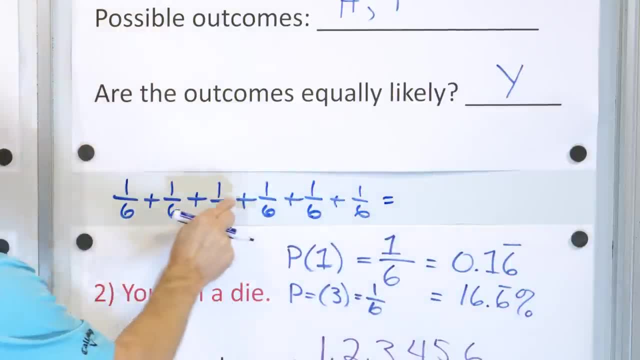 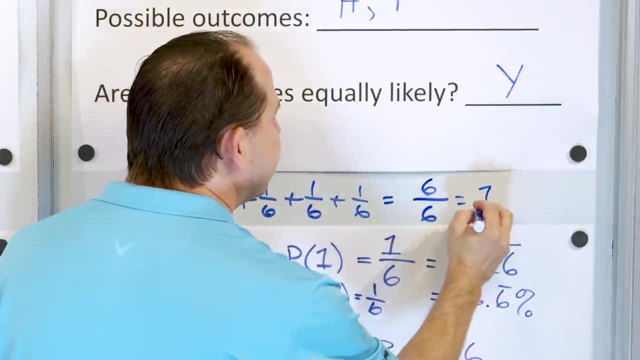 the probability of rolling a five. the probability of rolling a six. We have a common denominator. We keep it. one plus one plus one, add those together, get six over six. Six over six is one. The probability of getting a one or a two or a three. 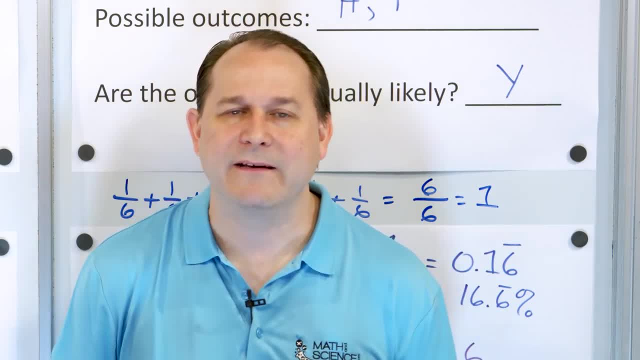 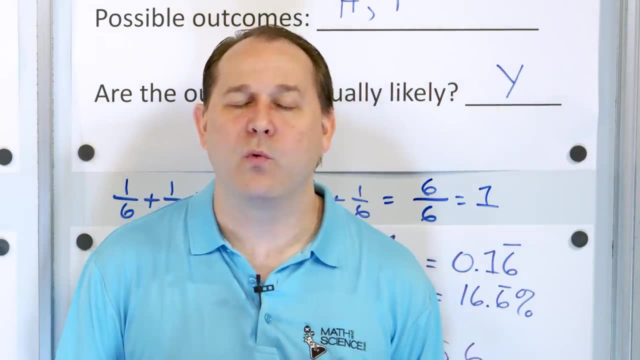 or a four or a five or a six is one. That means 100%. We're guaranteed to get one of these outcomes. when we take all the individual probabilities, they all have to add up to one, And I've showed you that again up here. 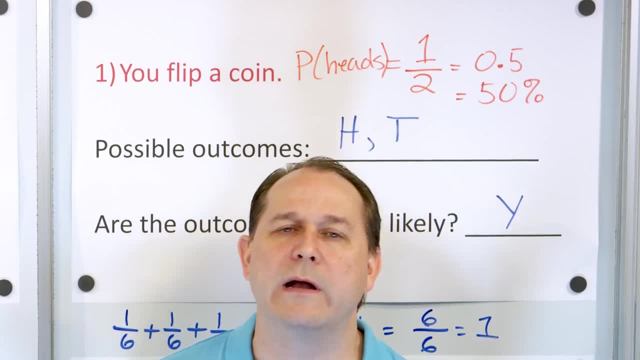 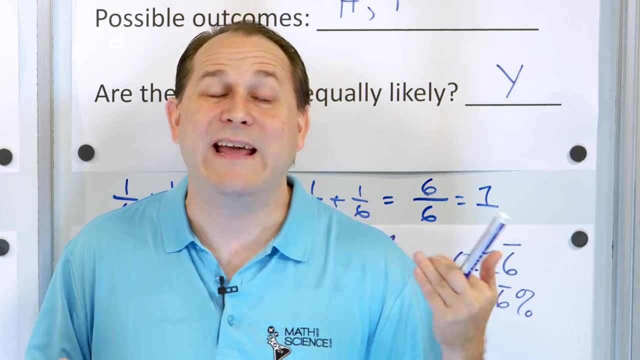 the probability of getting one half for this and one half for this. you add them, you get to one. So when you look at probability, the probabilities of all the possible outcomes should always add up to one, because you're guaranteed to get one of those outcomes. 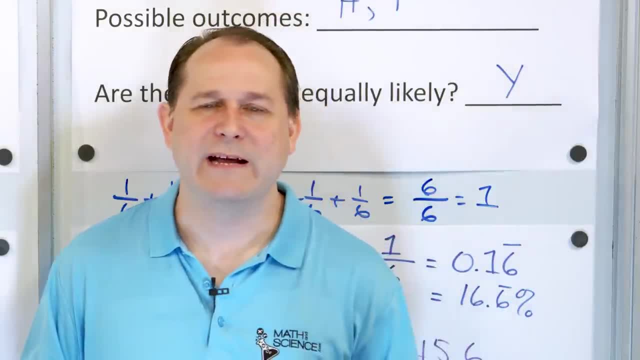 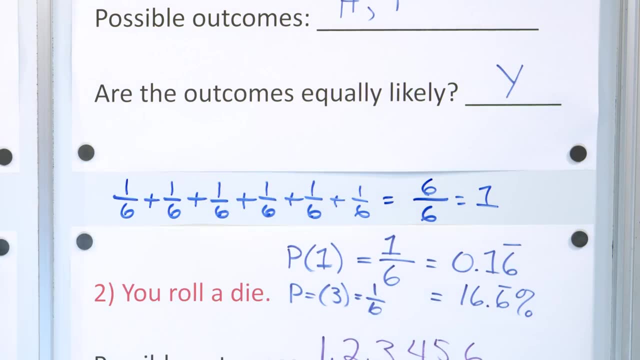 And so the probabilities have to add up to one. You see, why I told you in the beginning is that probability is just fractions, It's just literally an application of fractions, And I'm showing you that here. All right, let's go to something a little bit different. 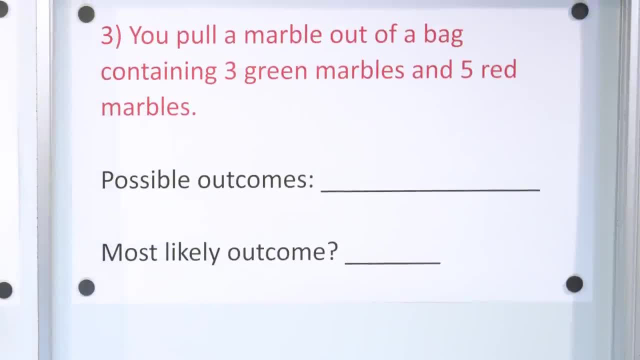 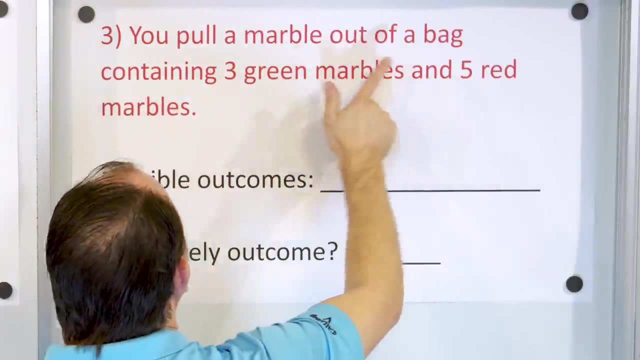 We've talked about flipping a coin. We've talked about rolling a die. Let's take a look at problem number three, something a little more complex. You pull a marble out of a bag containing three green marbles and five red marbles. 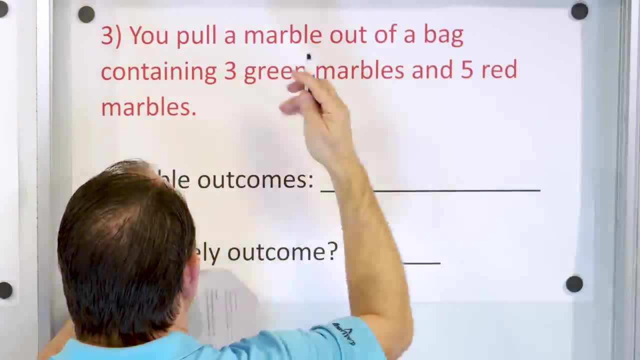 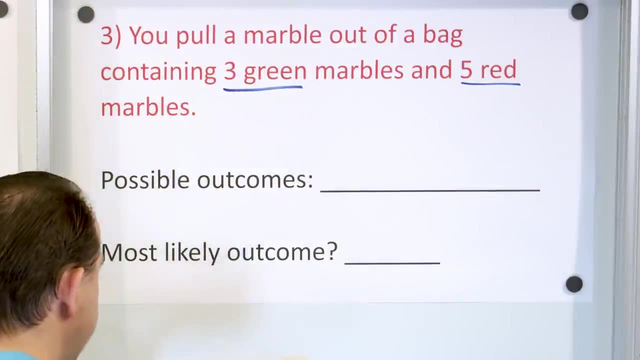 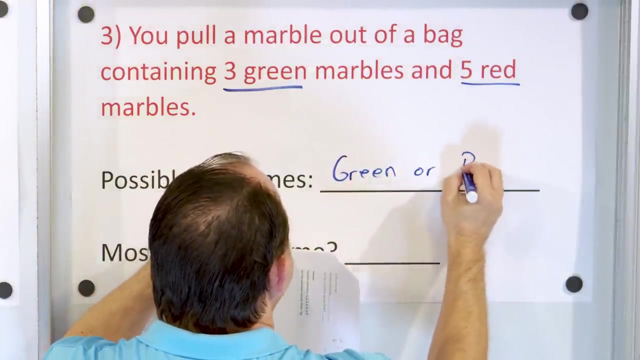 So you see, this bag has only three green marbles- underline this one- and five red marbles. all right, So what are the possible outcomes? If I pull just one marble out at random, I'm going to either get green or red, right? 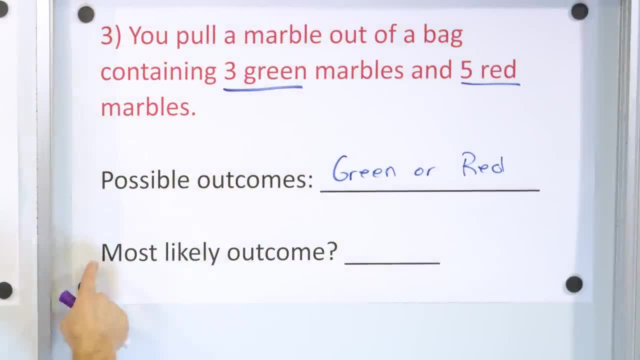 Green or red. That's the possible outcomes. So the question is: what is the most likely outcome? Well, you see, you might look at this and say, oh, it's green or red, they're equally likely, but we're hiding a little bit here. 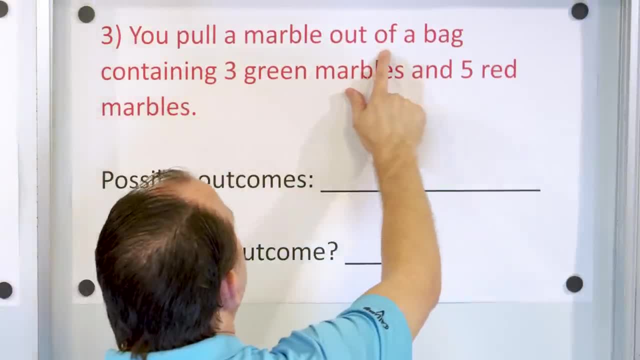 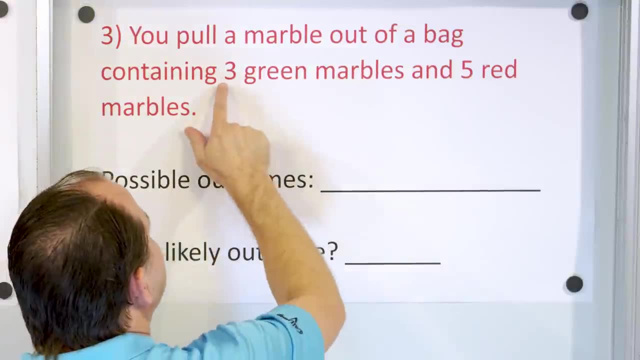 Let's take a look at problem number three, something a little more complex. You pull a marble out of a bag containing three green marbles and five red marbles. So you see, this bag has only three green marbles- underline this one and five red marbles. all right. 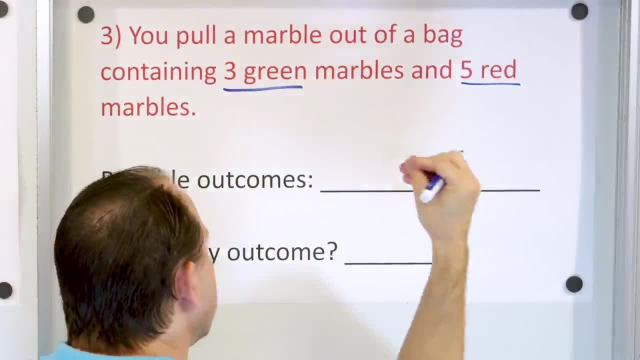 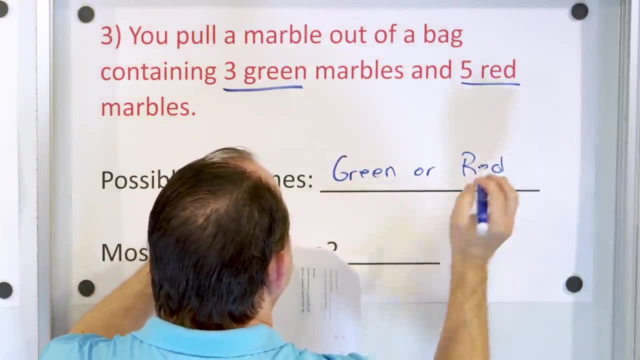 So what are the possible outcomes? If I pull just one marble out at random, I'm going to either get green or red, right Green or red. That's the possible outcomes. So the question is: what is the most likely outcome? 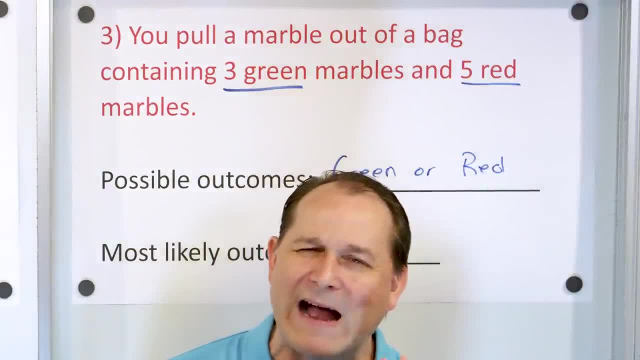 Well, you see, you might look at this and say, oh, it's green or red, they're equally likely. But we're hiding a little bit here because we said there's only three green marbles. So in reality there's only one marble that's green. 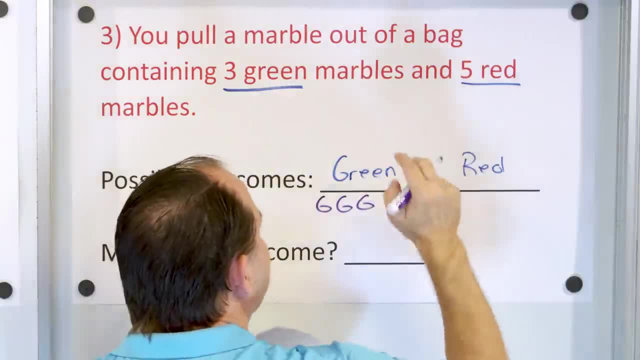 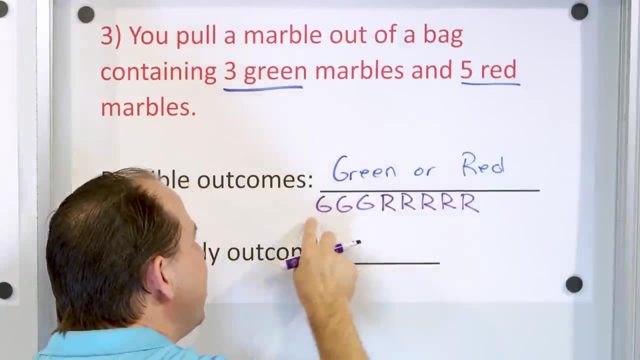 another marble that's green, another marble that's green in the bag, But red marbles. So we have red, another red, another red, another red and another red. When we write it all out and we see we have three green and five red. what do you think is more likely? Well, 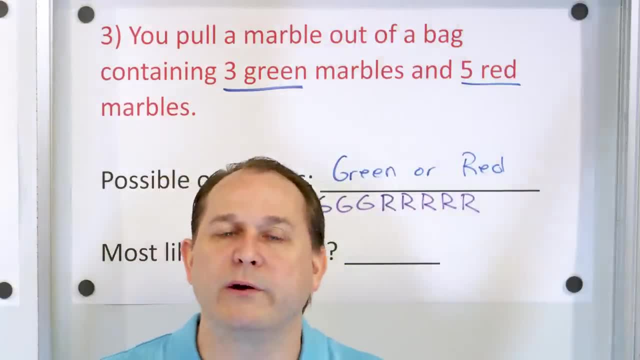 you have more red marbles On average, you're going to be pulling red marbles more often. So what is the most likely outcome? Red, A red marble is the more likely outcome. Now, what does that mean? It means that if I have a bag of marbles like this- some green and some red- 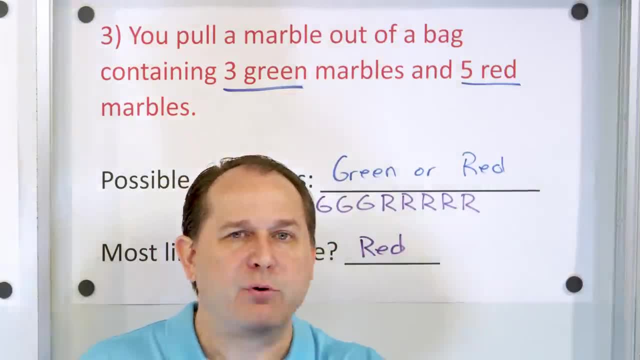 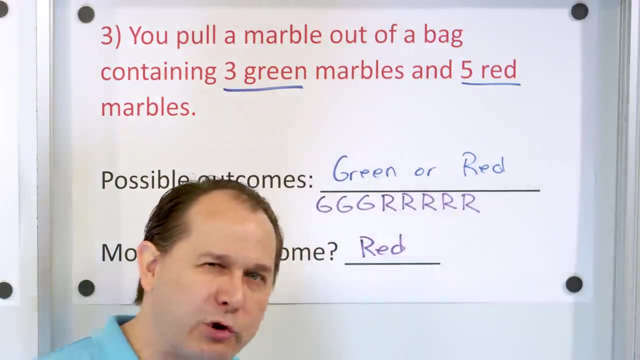 if I just pull one out, I could get either one. If I pull two out, maybe I still get two green marbles. Maybe I still get two green marbles. But if I do that experiment a thousand times- right, a large number of trials- then I'm going to expect over a thousand trials. that if I record. 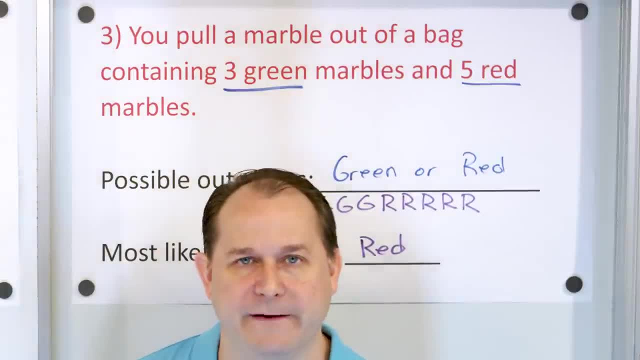 the results. it's going to be clear that I'm pulling red marbles more often. more often Because, as probability theory says, as I do the trial, more and more trials. if I make the experiment have a large number of trials, I'm going to expect more and more trials. 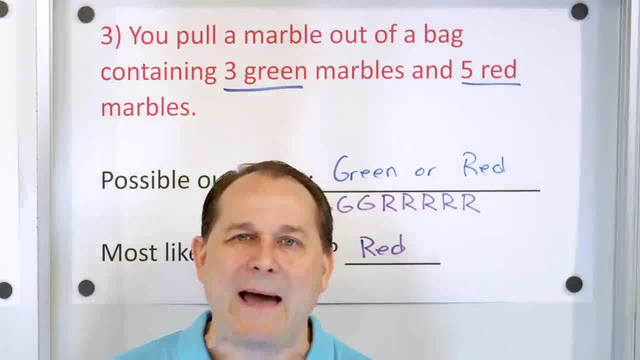 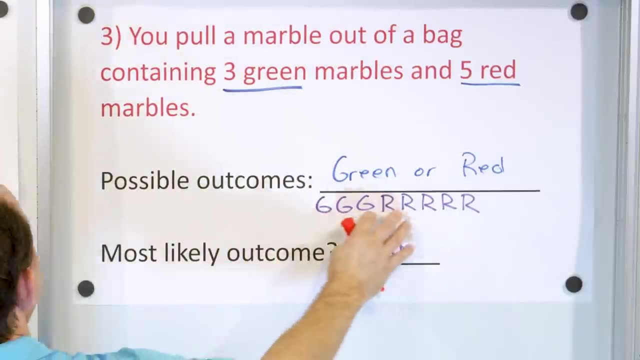 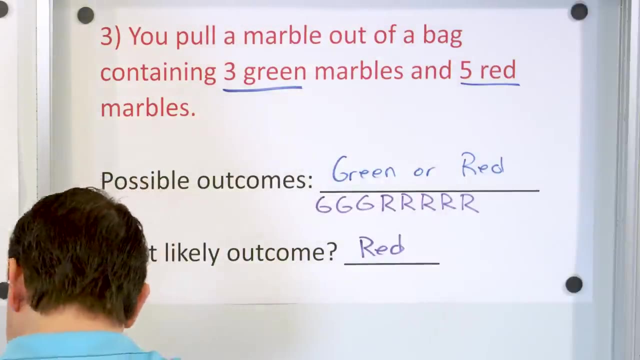 Then the observation I get is going to match when I calculate closer and closer and closer. And speaking of that, let's just take a minute to calculate something and see what we get. All right, Let's say that I'm going to calculate the probability of getting a green marble. 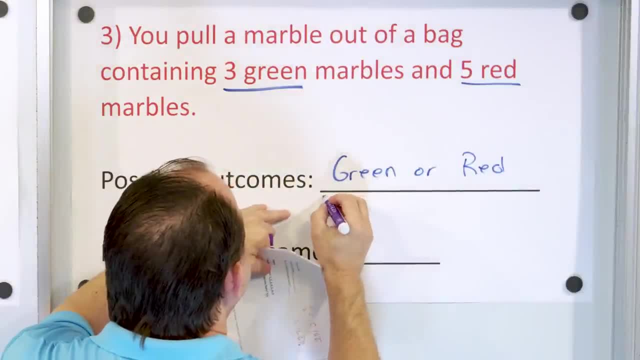 because we said there's only three green marbles. So in reality there's only one marble that's green, another marble that's green and another marble that's green in the bag. But we have five marbles in the bag, Five red marbles. 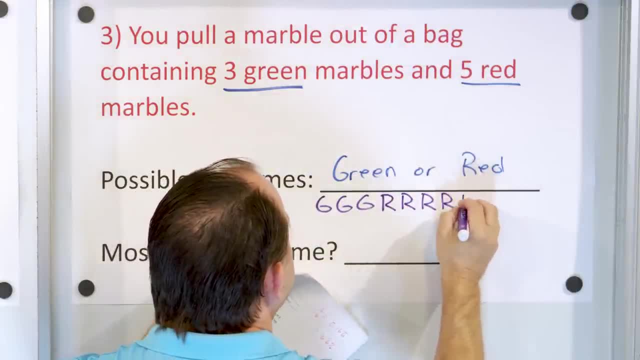 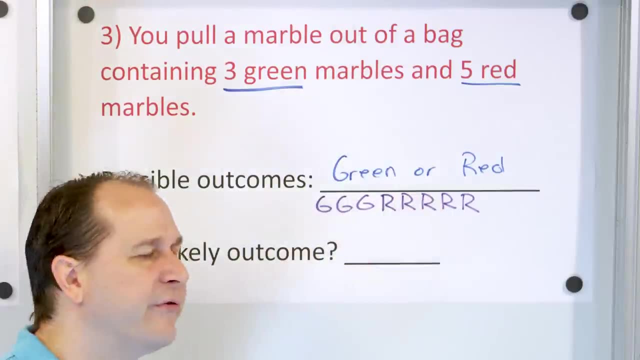 So we have red, another red, another red, another red and another red. When we write it all out and we see we have three green and five red, what do you think is more likely? Well, you have more red marbles. 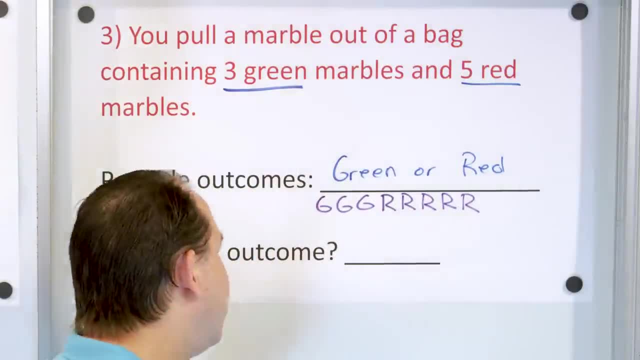 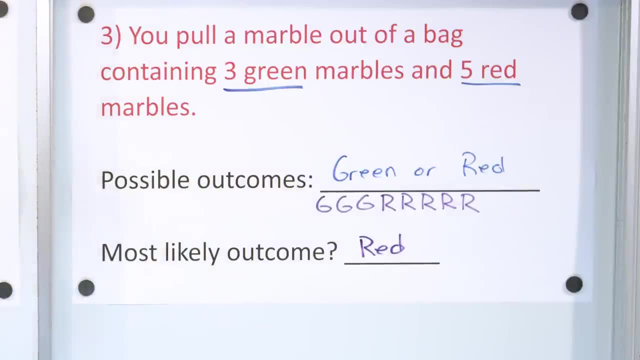 On average, you're going to be pulling red marbles more often. So what is the most likely outcome? Red, A red marble is the more likely outcome. Now, what does that mean? It means that if I have a bag of marbles like this, 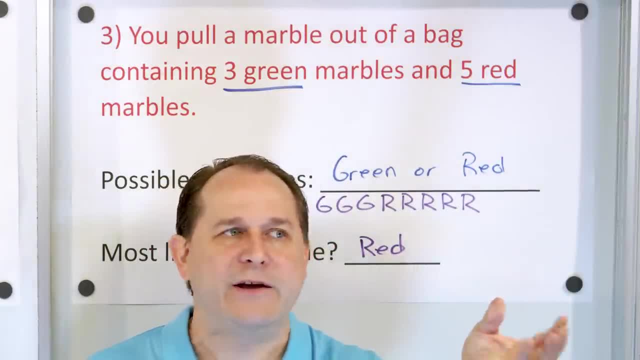 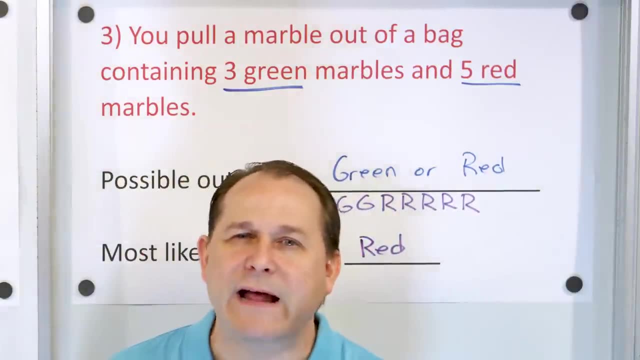 some green and some red. if I just pull one out, I could get either one. If I pull two out, maybe I still get two green marbles, Or maybe I still get two green marbles. But if I do that experiment a thousand times, 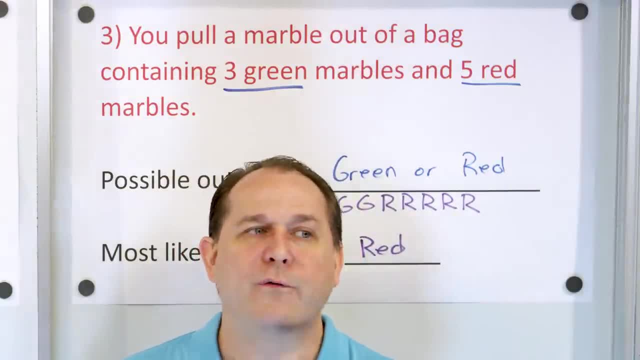 a large number of trials, then I'm going to expect over a thousand trials, that if I record the results, it's going to be clear that I'm pulling red marbles more often, More often, Because, as probability theory says, as I do the trial, more and more trials. 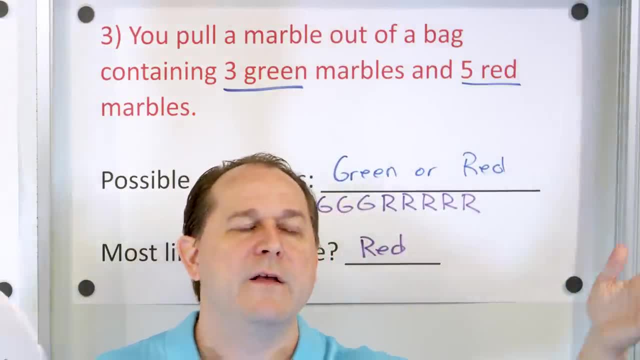 if I make the experiment have a large number of trials, then the observation I get is going to match when I calculate closer and closer and closer. And speaking of that, let's just take a minute to calculate something and see what we get. All right. 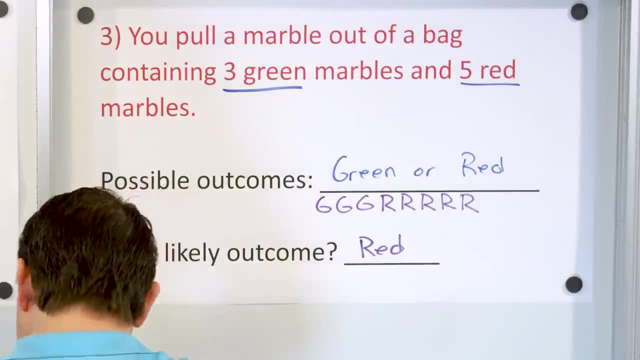 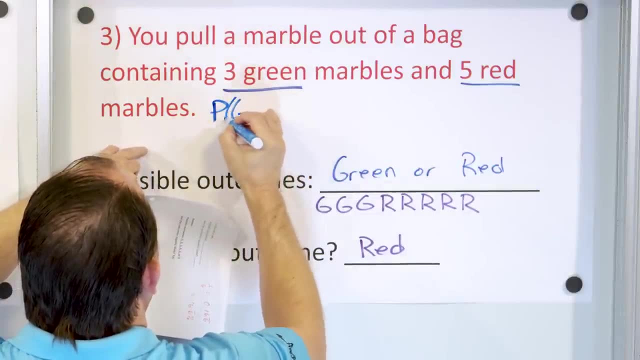 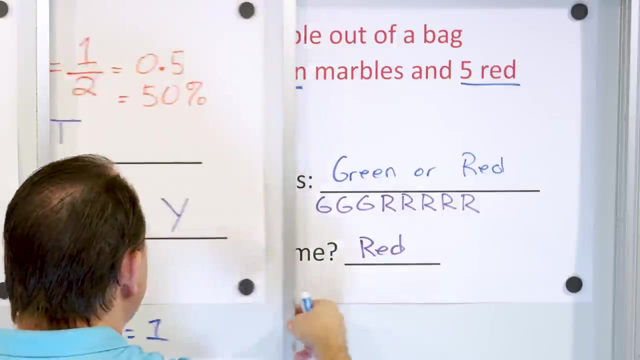 Let's say that I'm going to calculate the probability of getting a green marble. What is the probability of pulling one of these green marbles out? Well, how do we do it? before We said: well, we have to identify. how many ways can I get what I'm looking for? One head out of two possible. 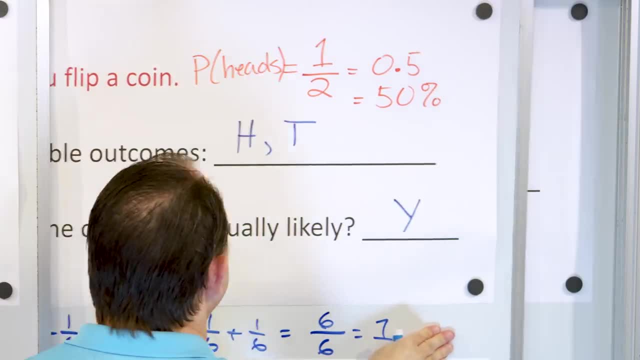 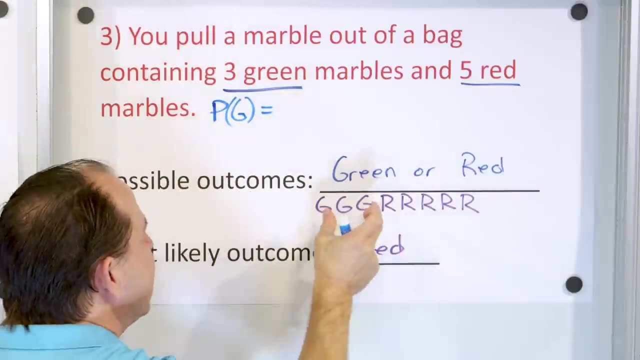 outcomes. So here we have to identify a similar sort of thing: How many ways can I get green? Well, you can't really just look at the outcomes. You have to look at how many marbles you actually have in there. I have three green marbles in there, right, But how many total marbles do I? 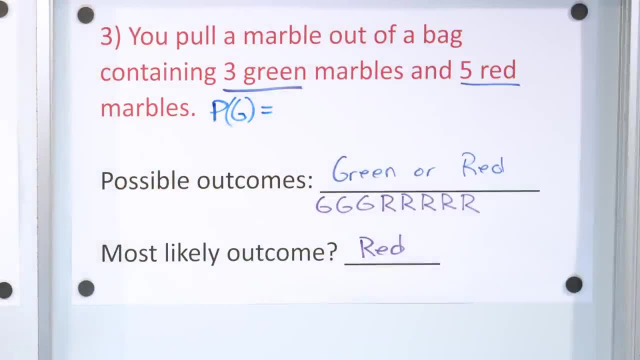 What is the probability of pulling one of these green marbles out? Well, how did we do it before? We said: oh, I'm going to get a green marble, I'm going to get a red marble, I'm going to get a. 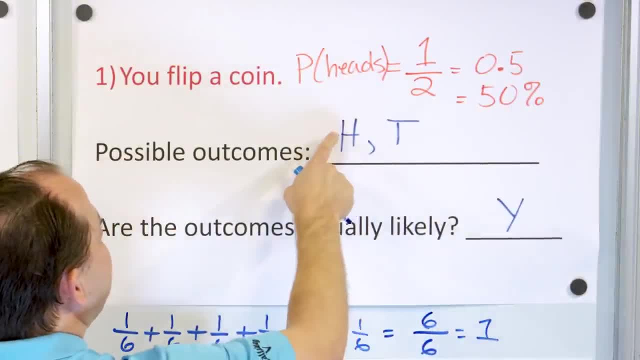 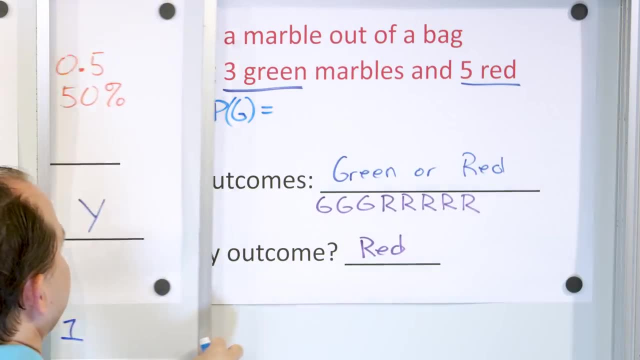 red marble. We said: well, we have to identify how many ways, how many ways can I get what I'm looking for One head out of two possible outcomes. So here we have to identify a similar sort of thing: How many ways can I get green? Well, you can't really just look at the outcomes You have. 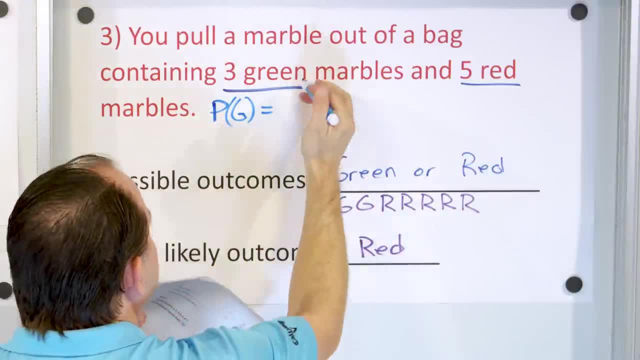 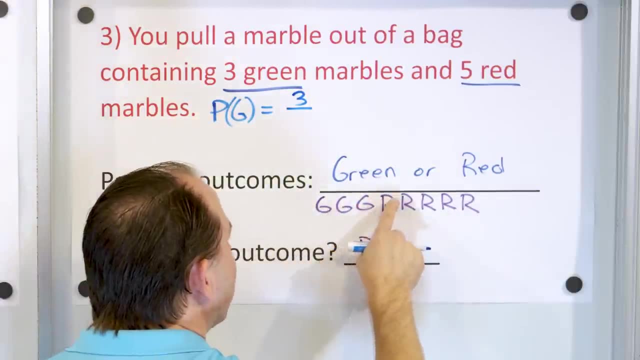 to look at how many marbles you actually have in there. I have three green marbles in there, Right, But how many total? how many total marbles do I really have? One, two, three, four, five, six, seven, eight? There's actually eight of those, All right. 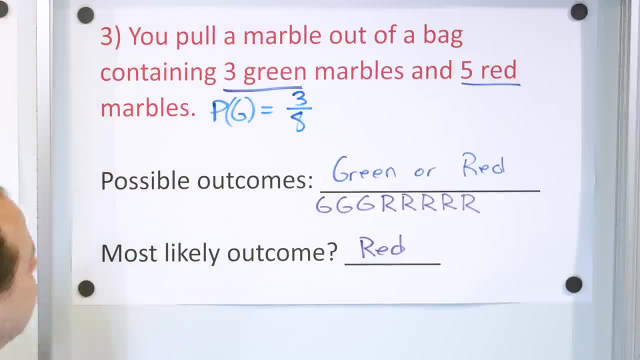 So the probability of getting a green marble is the fraction three eighths. Now consider that four eighths. four eighths would be one half, That's 50% of the time. Three eighths is less than that. So you know just from the probability that the probability of pulling a green marble 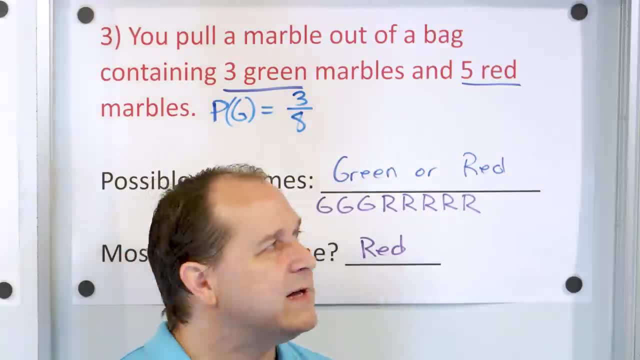 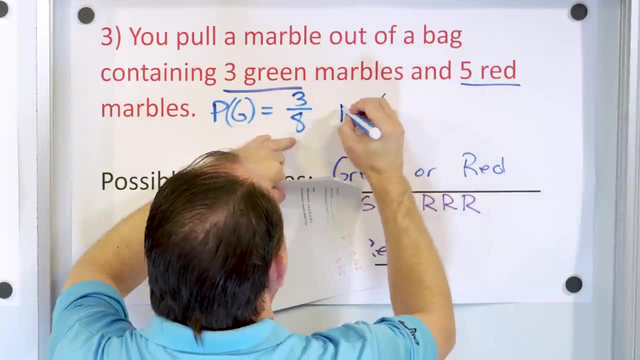 probability wise is less than 50%. Now let's go the extra mile here and find the probability of whoops. I kind of messed that up, Sorry about that. Let's find the probability of a red marble. Sorry about that. I can't really erase the probability of getting a red marble. 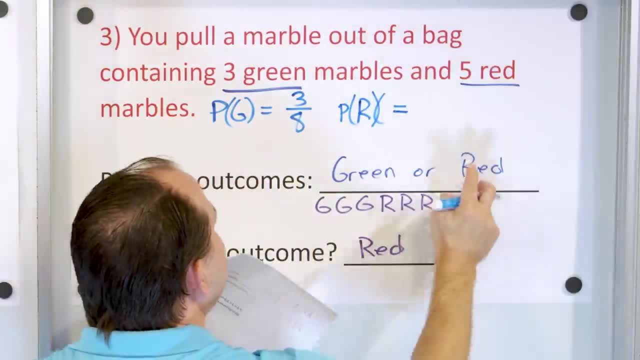 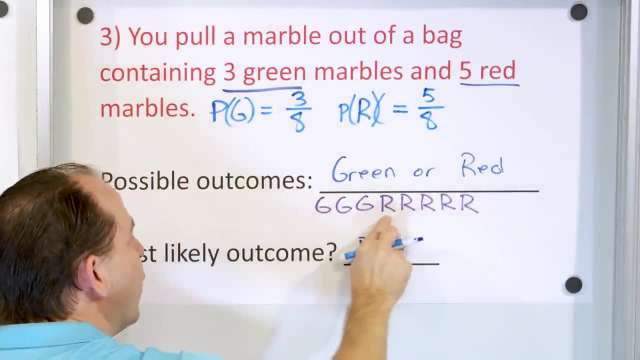 Same kind of thing. How many ways in which can I get red? I have actually five red marbles here, and how many all together? I have eight. So you see it's the same thing. It's how many ways can I get when I'm looking for in the outcome I'm trying to study, divided by how many total outcomes. 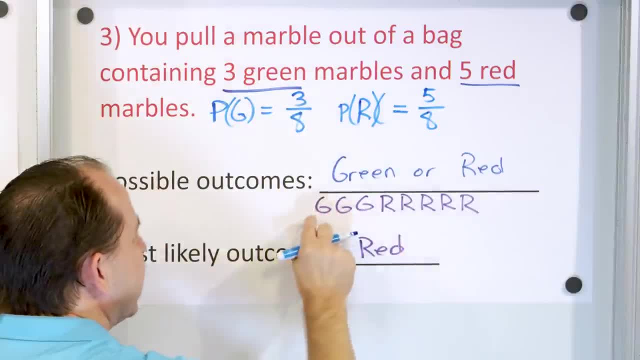 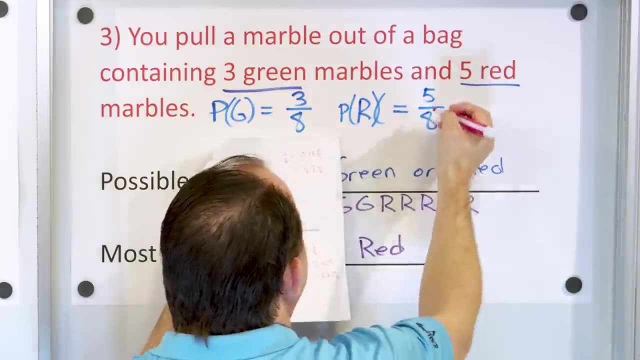 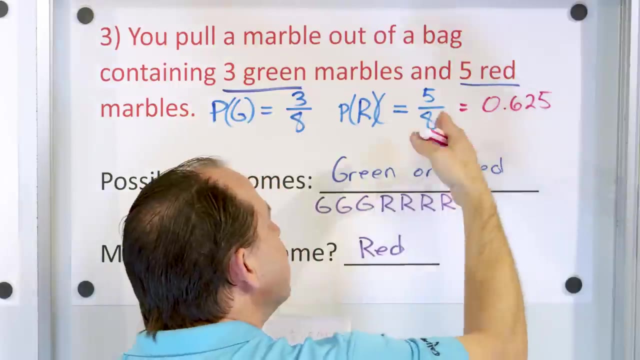 are there possible Five out of eight here? This one was three out of eight, So the probability is five eighths. Now, just for giggles, if you go back and count and take five divided by eight, you're going to get 0.625.. Notice again, this is higher than 0.5.. So it's. 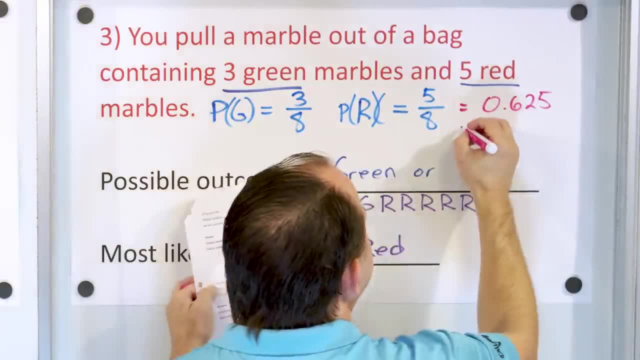 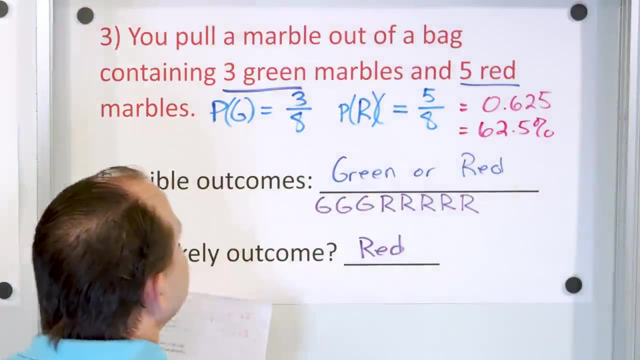 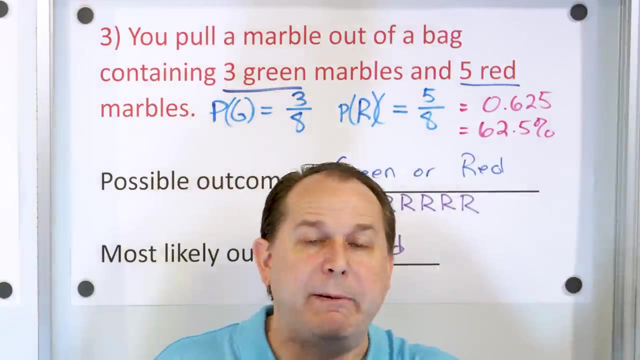 more than 50% of the time I expect to get a red marble And as a percentage, if I multiply by a hundred, this is moving the decimal 62.5%. So just from the numbers you can tell that the chances of getting a red marble are higher than 50%. So over the long haul I expect to be pulling. 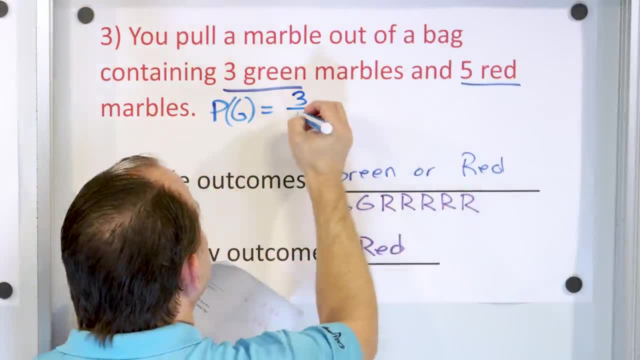 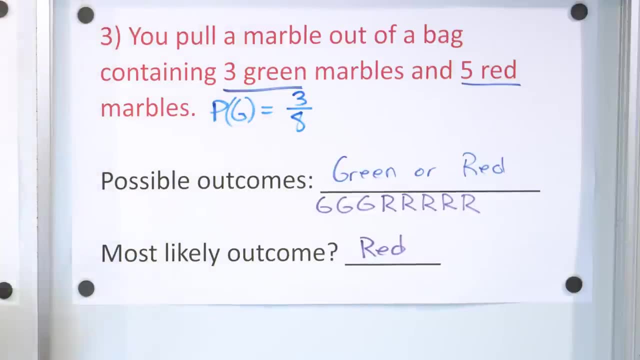 really have One, two, three, four, five, six, seven, eight. There's actually eight of those, all right. So the probability of getting a green marble is the fraction three-eighths. Now consider that four-eighths, four-eighths would be one-half, That's 50% of the time. 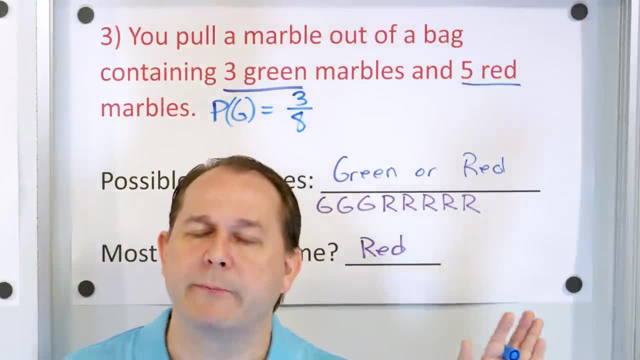 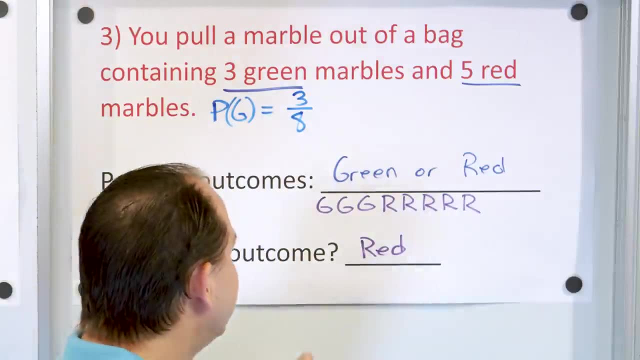 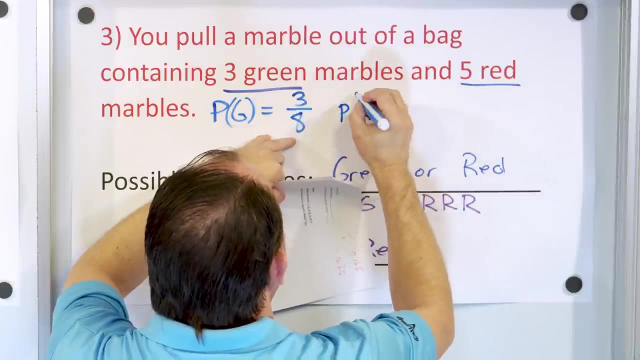 Three-eighths is less than that. So you know just from the probability that the probability of pulling a green marble probability-wise is less than 50%. Now let's go the extra mile here and find the probability of Whoops. I kind of messed that up, Sorry about that. Let's find the probability. 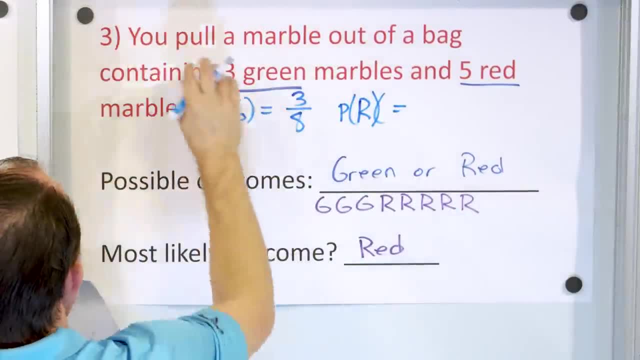 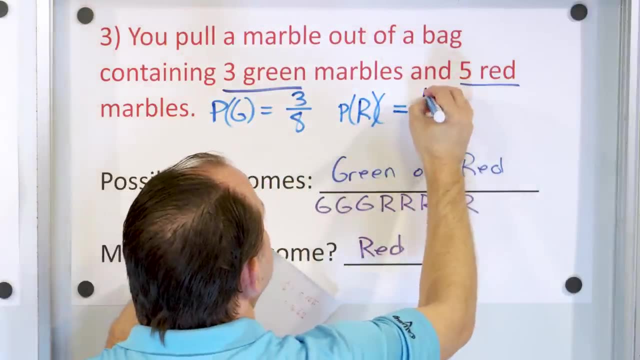 of a red marble. Sorry about that, I can't really erase The probability of getting a red marble. Same kind of thing. How many ways in which can I get red? I have actually five red marbles here, And how many? all together, I have eight. So you see, it's the same thing, It's. how many ways can. 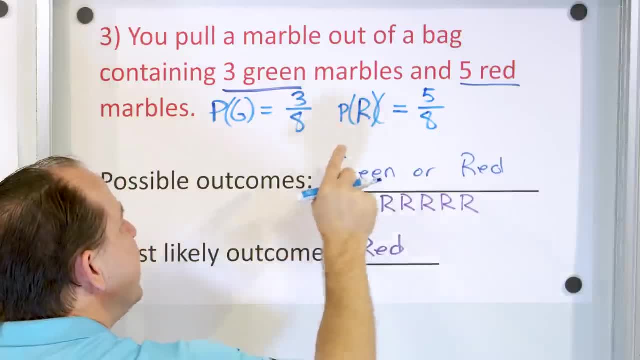 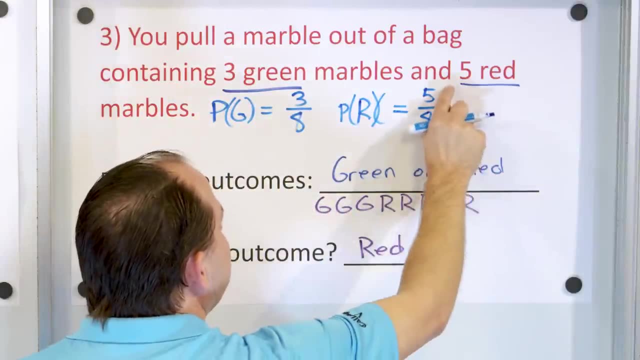 I get what I'm looking for in the outcome I'm trying to study. divided by how many total outcomes are there possible? Five out of eight here. This one was three out of eight. The probability is five-eighths. Now, just for giggles. if you go back and take five divided by 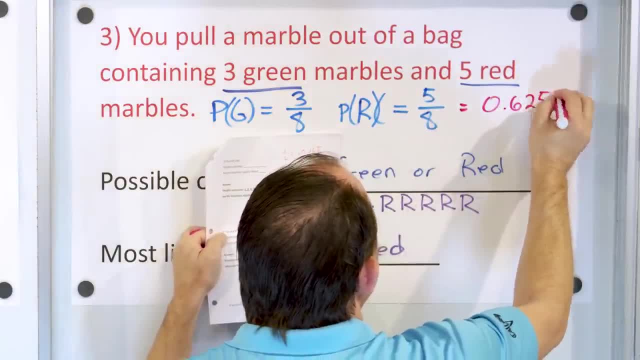 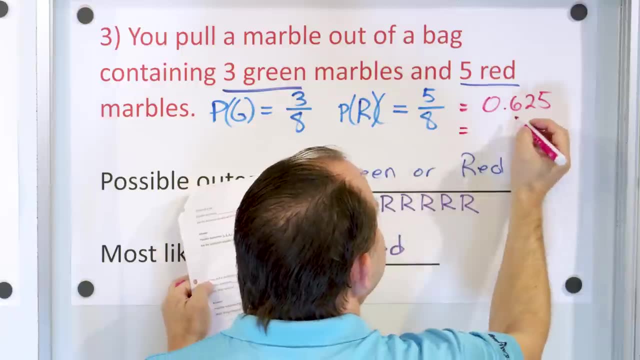 eight, you're going to get 0.625.. Notice again: this is higher than 0.5.. So it's more than 50% of the time I expect to get a red marble And as a percentage, if I multiply by 100,. 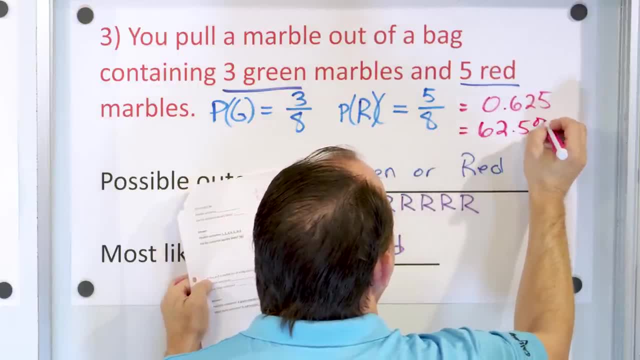 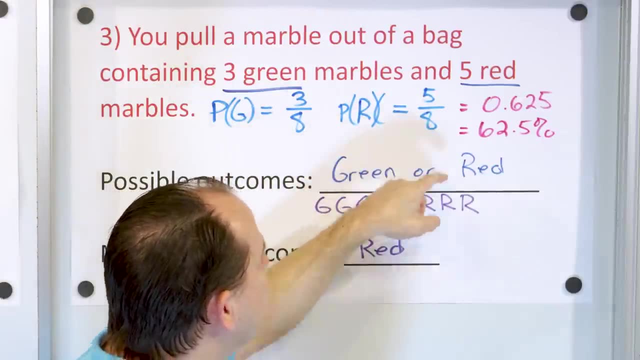 this is moving the decimal 62.5%. So just from the numbers you can tell that the chances of getting a red marble are higher than 50%. So over the long haul you're going to get a red marble. I expect to be pulling more red marbles than green marbles. And one last thing. 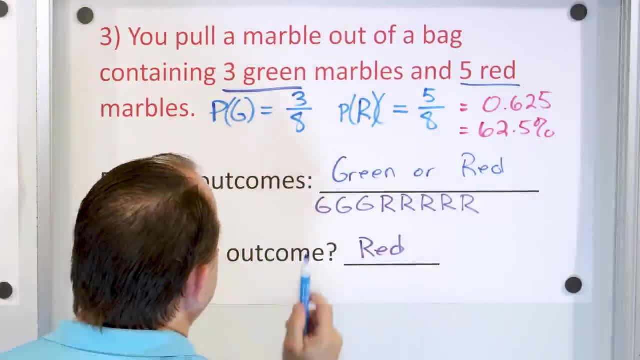 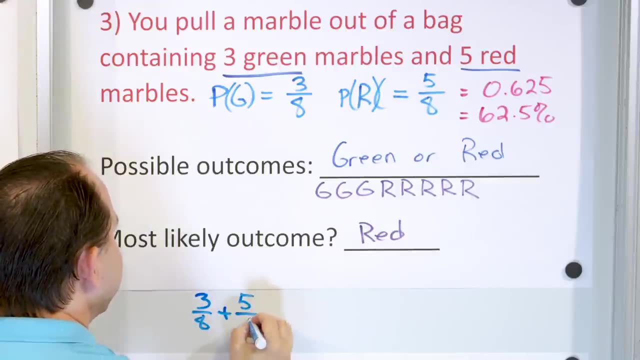 what is the probability of a green or a red marble? Well, that's going to be three-eighths, the probability of a green plus the probability of a marble that's red, five-eighths. You can add the probabilities And what do I get? Three plus five is eight. The denominator is eight. 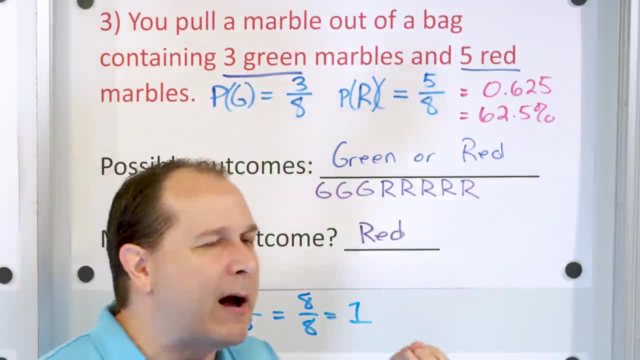 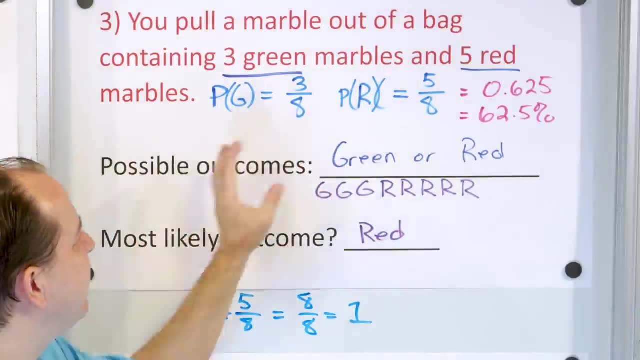 And I get an answer of one. What does that mean? It means that what is the probability of getting a green or a red is one. because the probability of getting a green or a red is one, The probabilities have to add to one The probabilities of all the outcomes, that are. 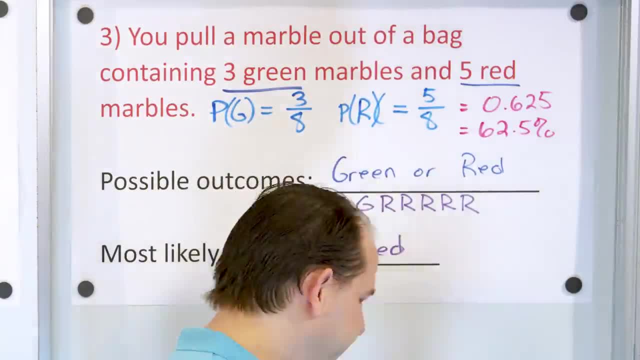 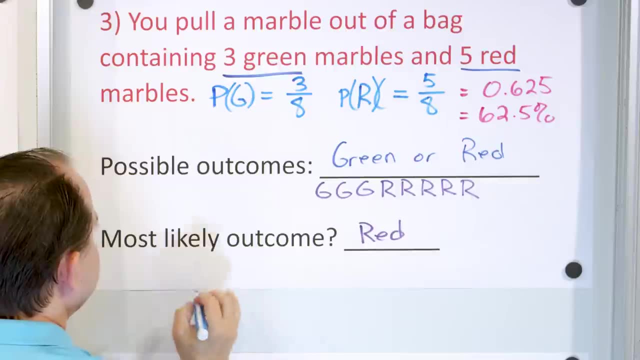 more red marbles than green marbles. And one last thing: the probability of a green or a red marble. Well, that's going to be three eighths, The probability of a green, plus the probability of a marble that's red, five eighths, You can add. 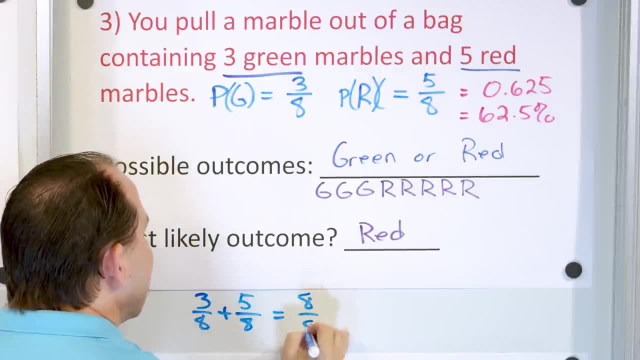 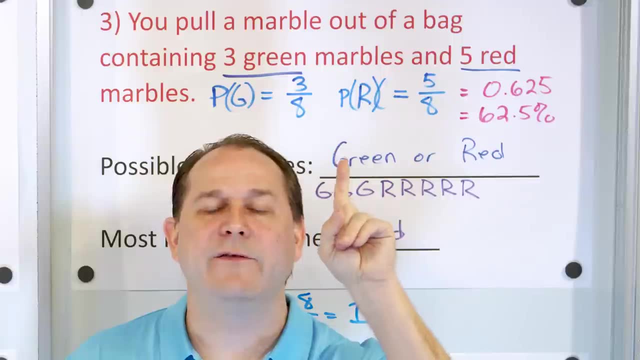 the probabilities. And what do I get? Three plus five is eight, The denominator is eight And I get an answer of one. What does that mean? It means that what is the probability of getting a green or a red is one, because the probabilities have to add to one The probabilities of all the. 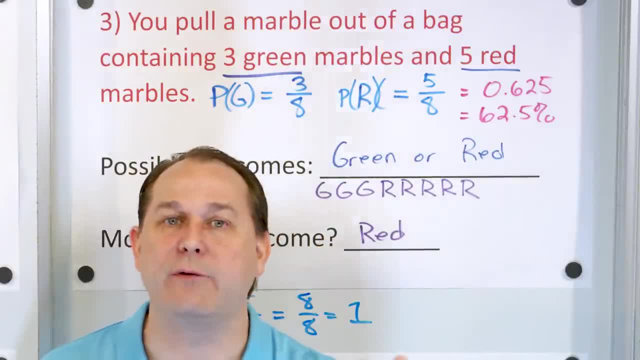 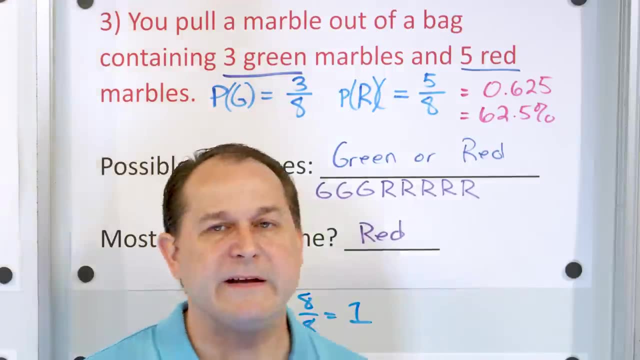 outcomes that are possible have to add to one because I'm guaranteed to get either a red or a green marble. The probability over here for the- I don't want to crunch my paper up- The probability over there of getting the heads or tails also added to one, and the probability of the dye also. all of the 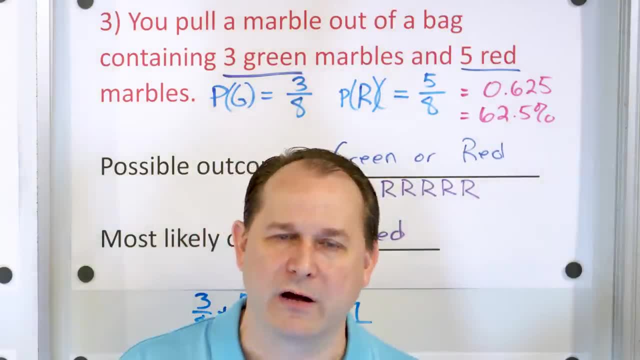 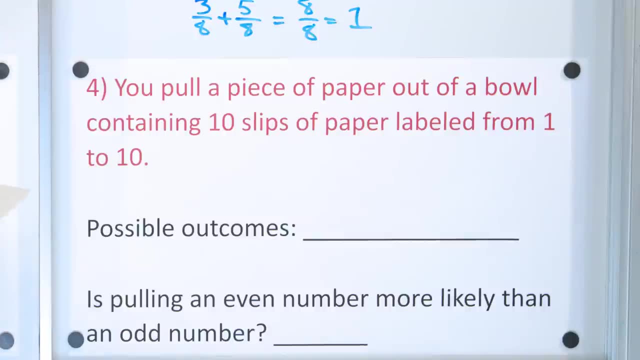 outcomes always added to one, So the probabilities of all outcomes that are possible in the experiment have to add to one. All right, let's go over here to number four. All right, You pull a piece of paper out of a bowl containing 10 slips of paper labeled from one to 10.. 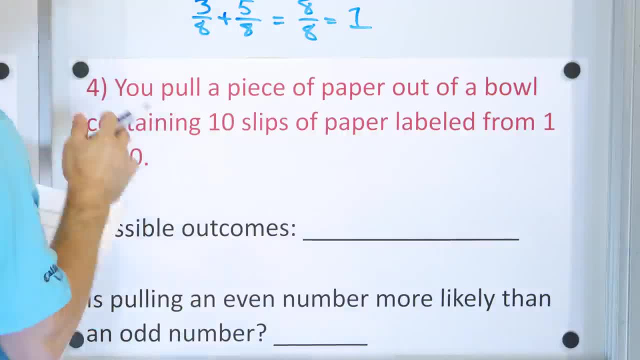 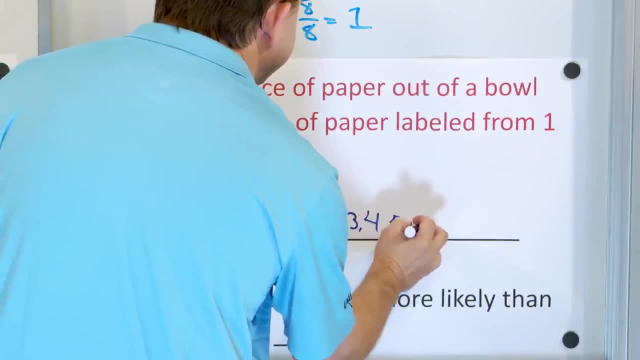 So there are 10 slips of paper. Each one is labeled 1 to 10.. What are the possible outcomes? Well, I can get a 1, or a 2, or a 3, or a 4, or a 5, or a 6, or a 7, or an 8, or a 9, or a 10.. 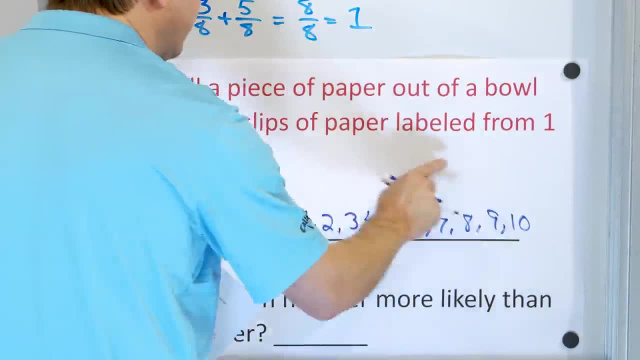 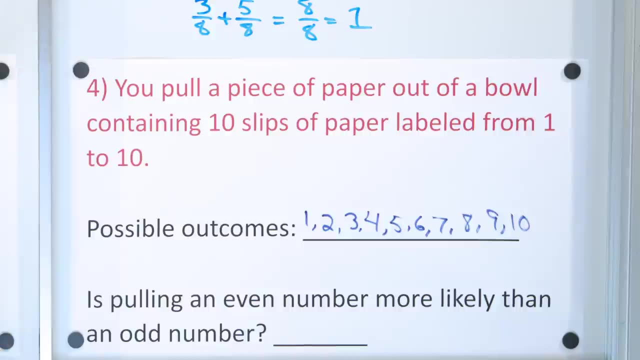 Why? Because it says I have 10 slips of paper. I have 10 numbers here and each paper is labeled 1 to 10.. So I have 10 pieces of paper. Each paper has a different number on it. Is pulling an even number more likely than an odd number. 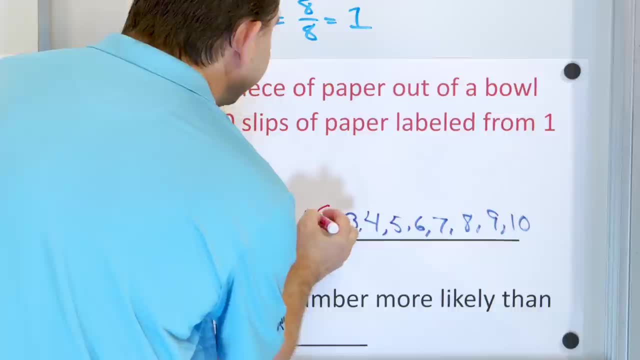 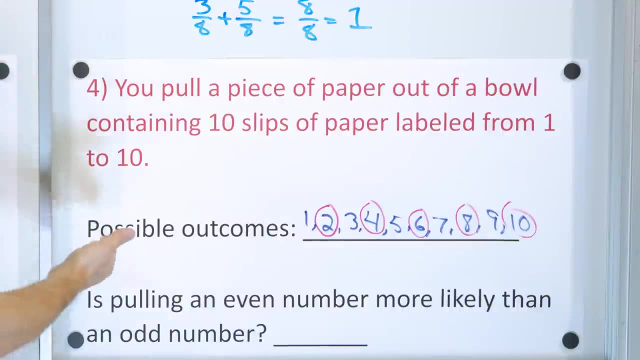 Well, let's talk about the even numbers. Here is an even number: 2, 4, that's even 6, 8, 10.. So you have to look at what the problem is. asking you Pulling an even number, is it more likely or not? 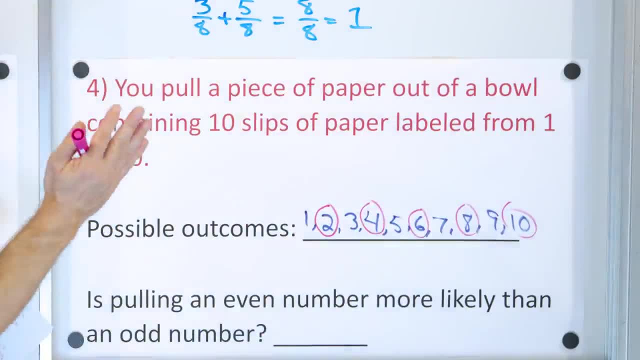 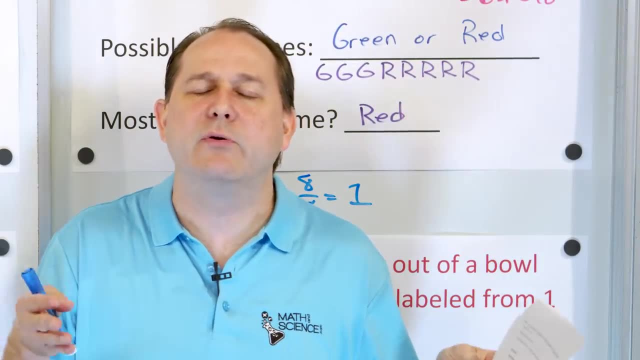 Well, I have 1,, 2,, 3,, 4, 5 even numbers, but I also have 1,, 2,, 3,, 4, 5 odd numbers. Because I have the same number of even numbers as odd numbers, then I'm equally likely to get even or odd. 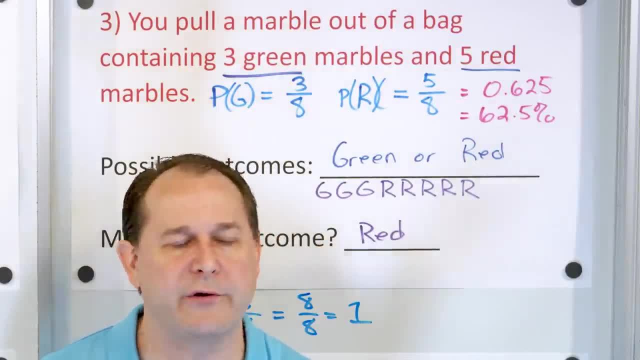 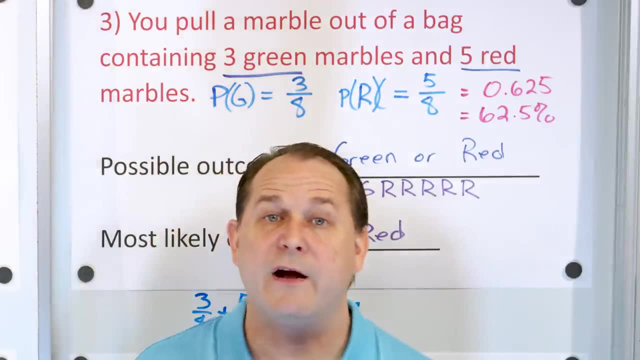 possible have to add to one, because I'm guaranteed to get either a red or a green marble. The probability over here for the- I don't want to crunch my paper up- the probability over there of getting the heads or tails also added to one, And the probability of the die also. all of the 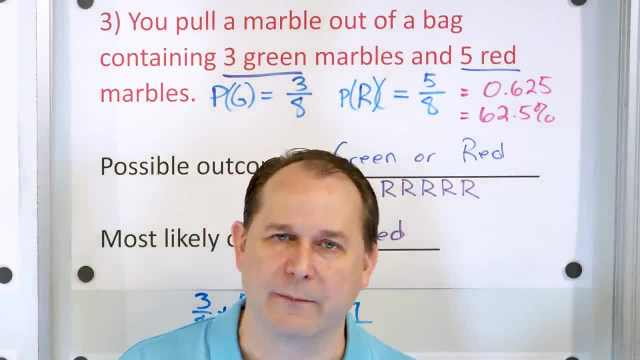 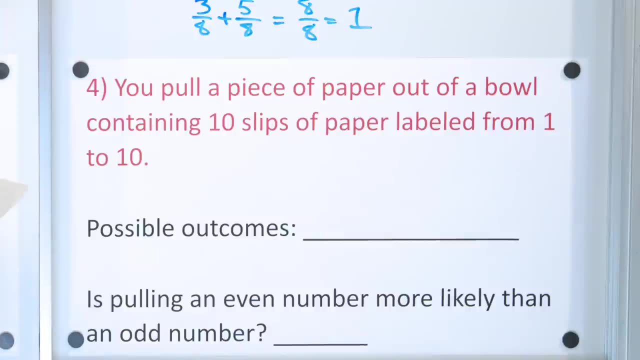 outcomes always added to one, So the probabilities of all outcomes that are possible in the experiment have to add to one. All right, let's go over here to number four. All right, you pull a piece of paper out of a bowl containing ten slips of paper labeled from one to ten. 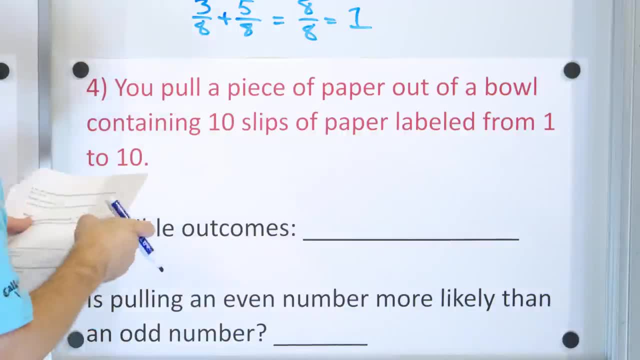 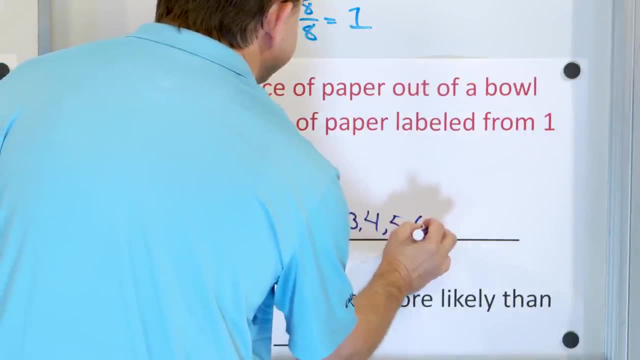 So there are ten slips of paper. Each one is labeled one to ten. What are the possible outcomes? Well, I can get a one or a two, or a three or a four or a five or a six or a seven or an eight or a nine or a ten. 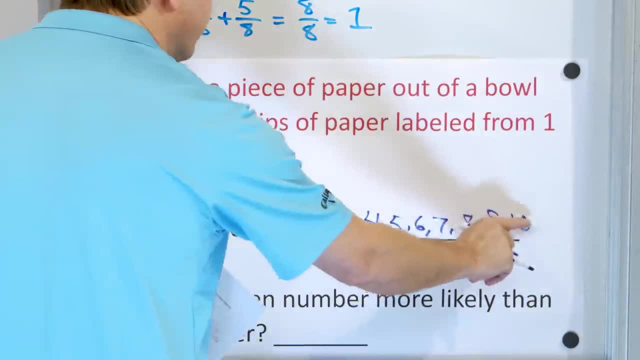 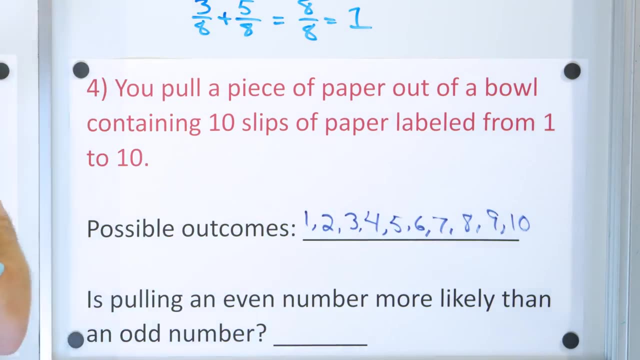 Why? Because it says I have ten slips of paper. I have ten numbers here and each paper is labeled one to ten. So I have ten pieces of paper. Each paper has a different number on it. Is pulling an even number more likely than an odd number? 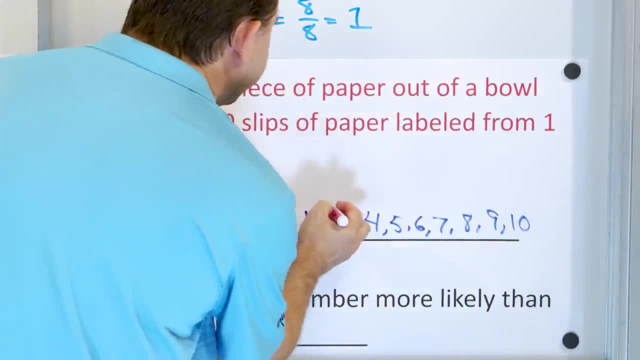 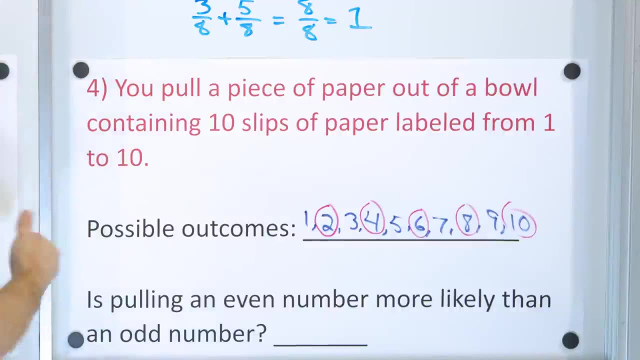 Well, let's talk about the even numbers. Okay, here is an even number: Two, four, that's even. Six, eight, ten. So you have to look at what the problem is. asking you Pulling an even number: is it more likely or not? 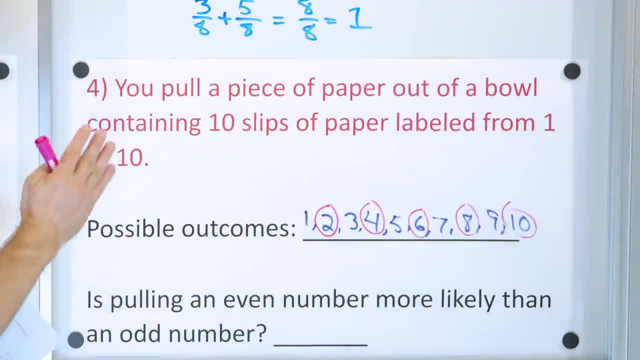 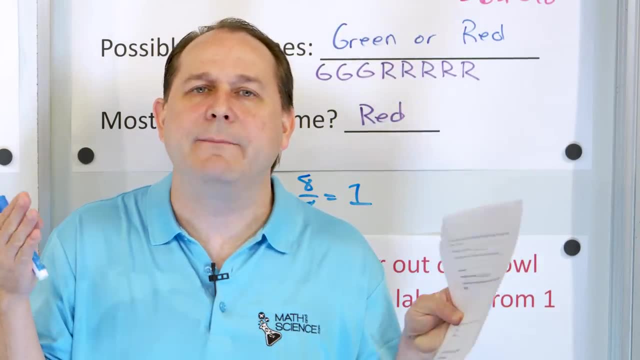 Well, I have one, two, three, four, five even numbers, but I also have one, two, three, four, five odd numbers. Because I have the same number of even numbers as odd numbers, then I'm equally likely to get even or odd. 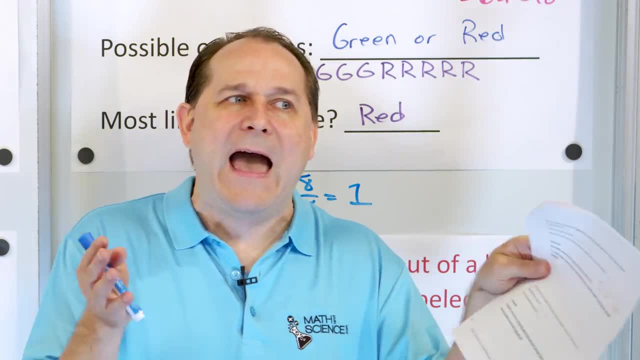 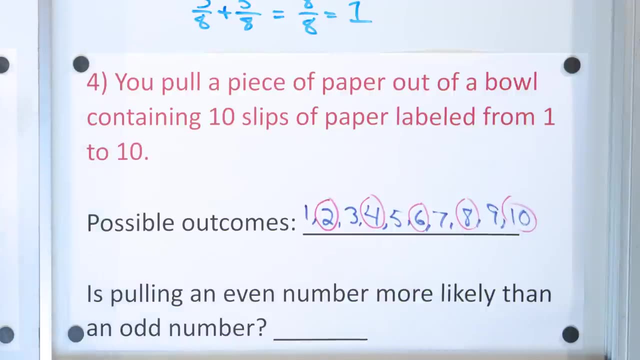 Because in the bag, yes, there's a bunch of numbers, but half of them are even and half of them are odd. So I expect that is pulling an even number more likely than an odd number. No, They're equally likely, And let's talk about that for a second: equally likely. 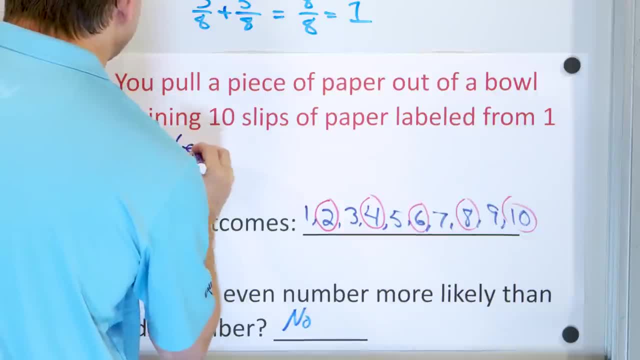 Let's figure out what the probability of pulling out an even number actually is. You know we're going to do these problems a lot later, but let's just kind of do it now. It's not so hard. The probability of getting an even is the number of ways in which I can get an even. 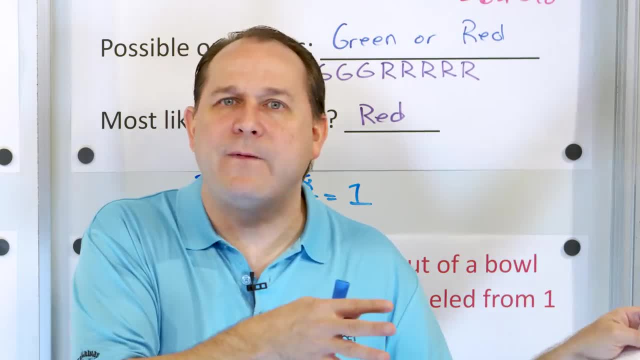 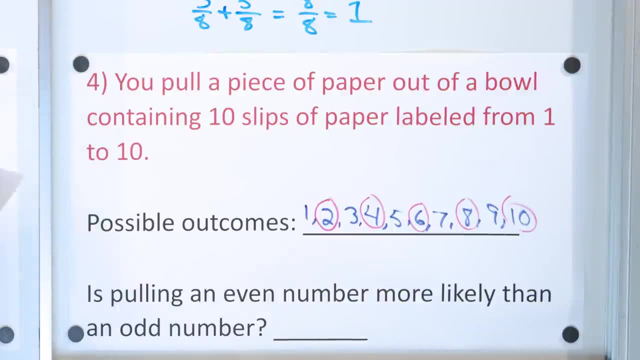 Because in the bag, yes, there's a bunch of numbers, but half of them are even and half of them are odd. So I expect that is pulling an even number more likely than an odd number. No, They're equally likely, And let's talk about that for a second: equally likely. 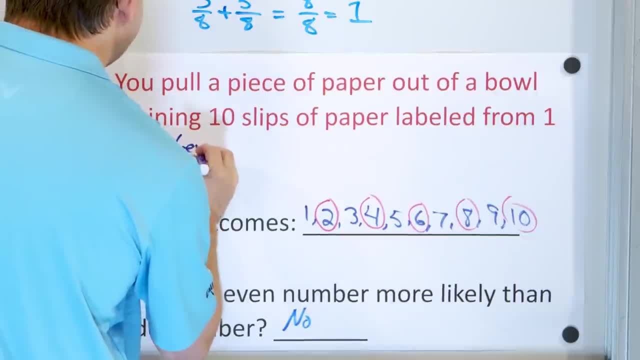 Let's figure out what the probability of pulling out an even number actually is. You know we're going to do these problems a lot later, but let's just kind of do it now. It's not so hard. The probability of getting an even is: 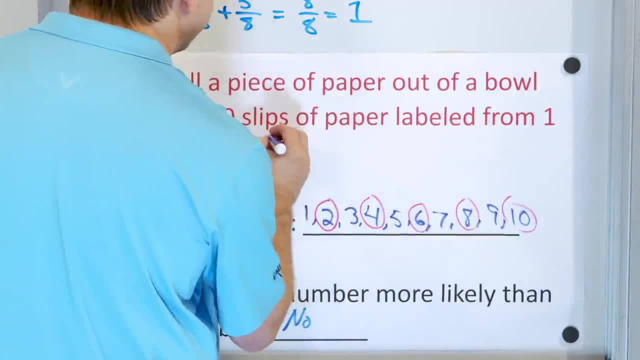 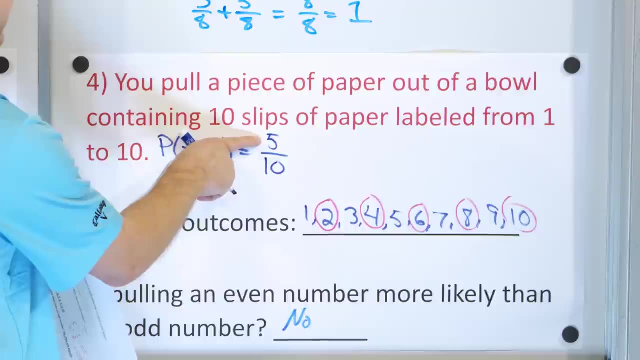 The number of ways in which I can get an even. there's 5 even numbers here divided by the total number of outcomes. There's actually 10 outcomes here. So I can get my even number 5 ways, but there's actually 10 pieces of paper in there, 5 out of 10.. 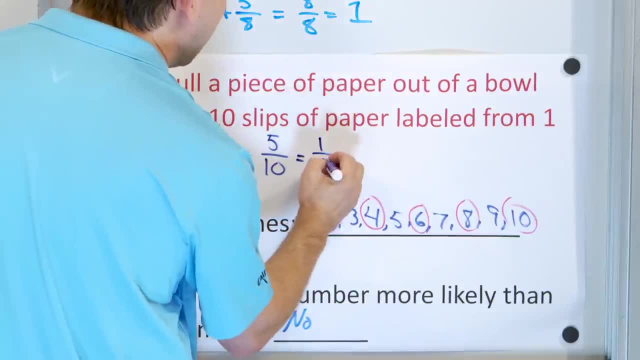 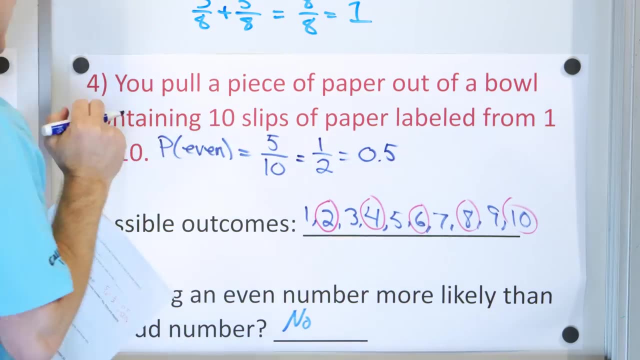 And when you divide by 5, divide by 5, divide by 5, that's the same as 1 half, which is 0.5.. Right, So the probability of getting an even is 0.5, which is half of the time. 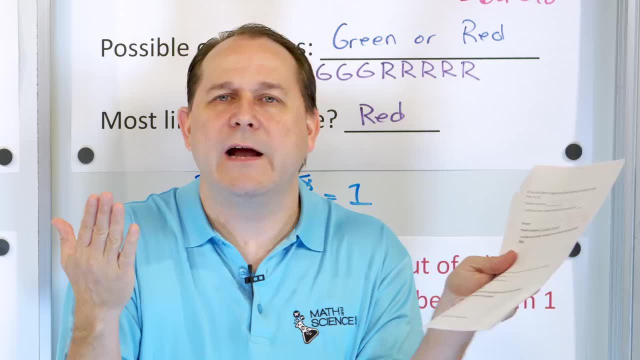 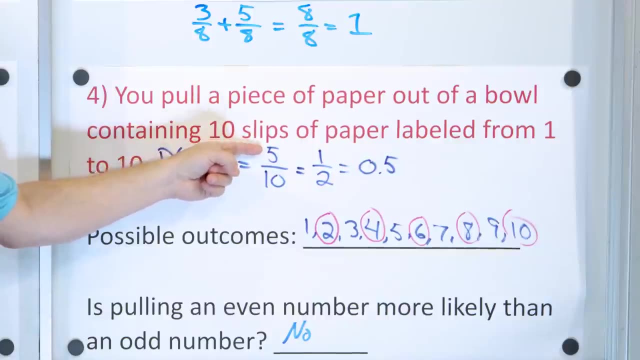 It's exactly what we knew. Because we have 5 even and 5 odd, you know, half the time we should get even or odd. This is proving it with a probability. I can get an even number 5 ways, but there's a total of 10 papers. 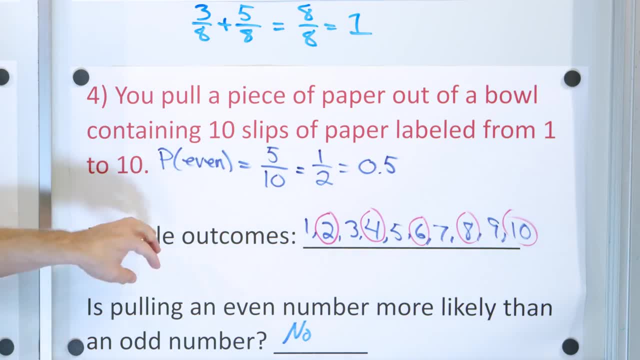 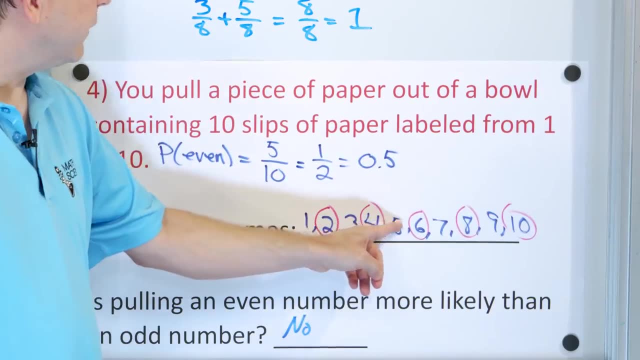 and that means the probability of pulling it is 1 half, which is the same as 0.5. Now here's the next question: What is the probability of drawing an odd number? Well, how many odd numbers are there? 1,, 2,, 3,, 4, 5.. 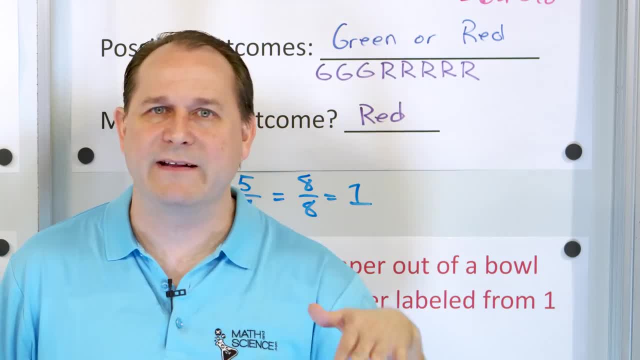 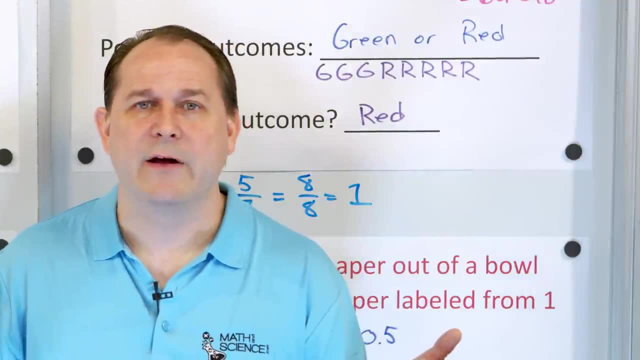 Again 5, but there's still 10 total numbers, So again 5 out of 10.. So the probability of odd is also 1 half And the probability of even is also 1 half, And when you add all the possible outcome probabilities you should get 1.. 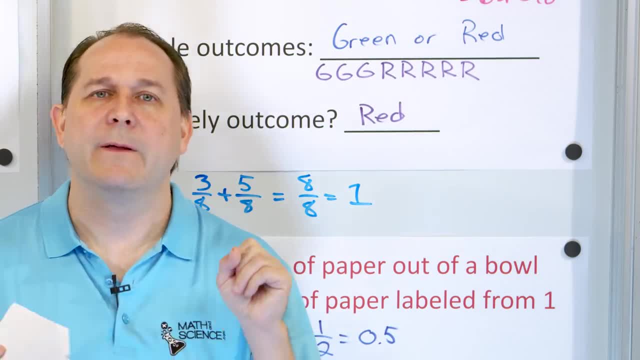 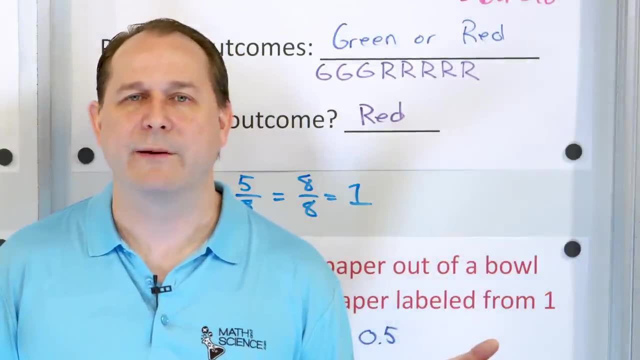 1 half plus 1 half is 1.. In every one of these examples, the probability, when we calculate all the probabilities that we can do and we add them all together, all the ways in which the outcomes can happen, they always have to add to 1, and that is shown here as well. 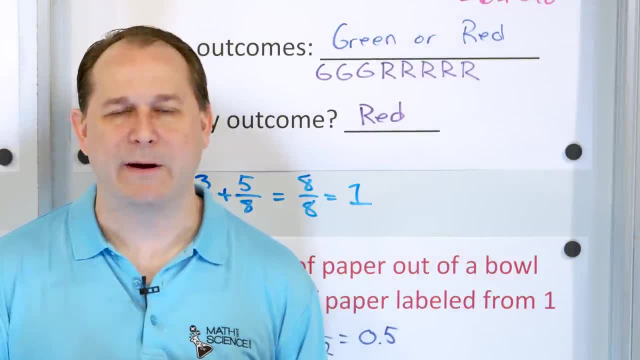 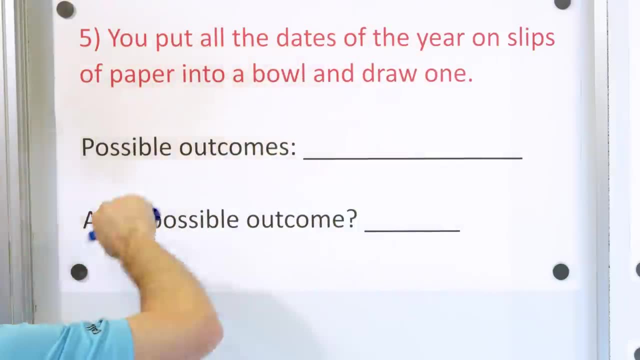 I have one more. Let me take these down and we'll conquer the last one and wrap up this lesson. All right, Here's our very last problem. It says: Draw all of the dates of the year on slips of paper into a bowl and draw 1.. 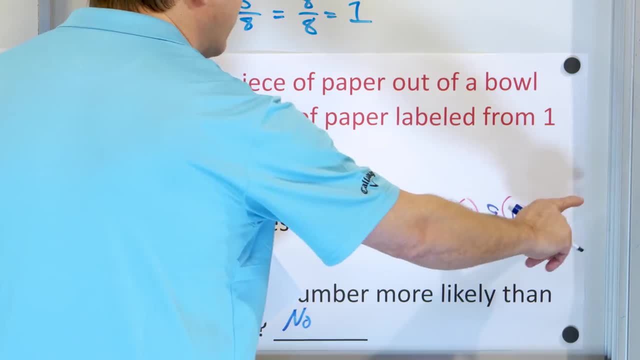 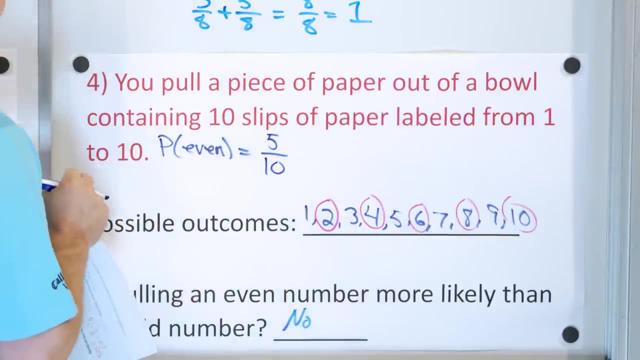 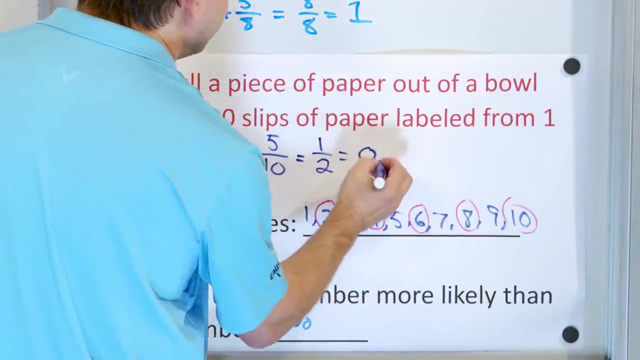 there's five even numbers here divided by the total number of outcomes. There's actually ten outcomes here, So I can get my even number five ways, but there's actually ten pieces of paper in there, five out of ten, And when you divide by five, divide by five, divide by five, that's the same as one half, which is 0.5. 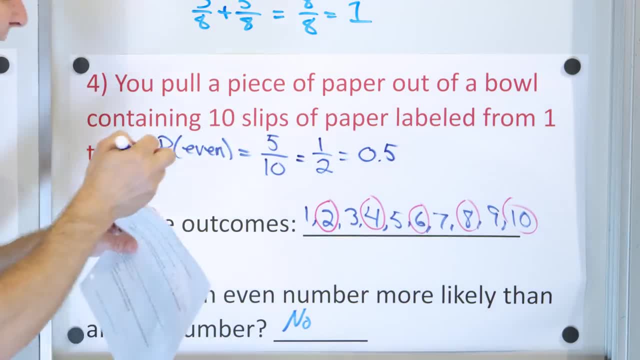 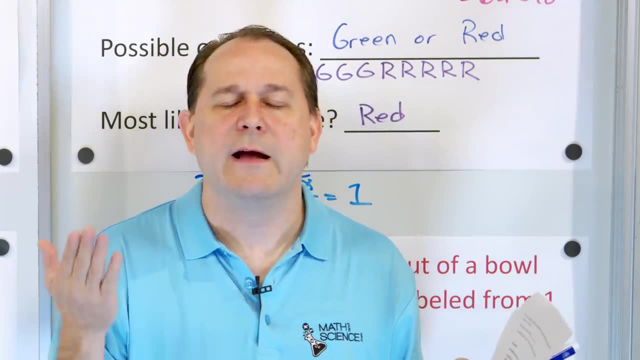 So the probability of getting an even is 0.5, which is half of the time. It's exactly what we knew, because we have five even and five odd. You know half the time we should get even or odd. This is proving it with a probability. 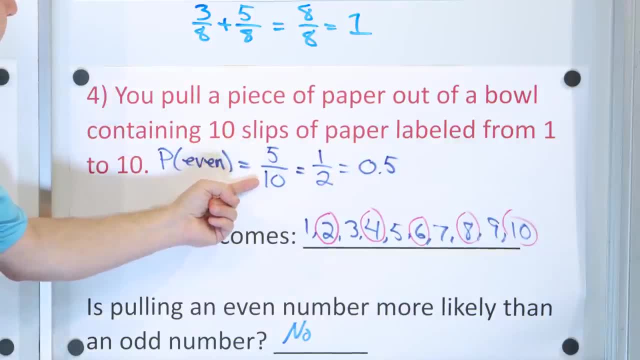 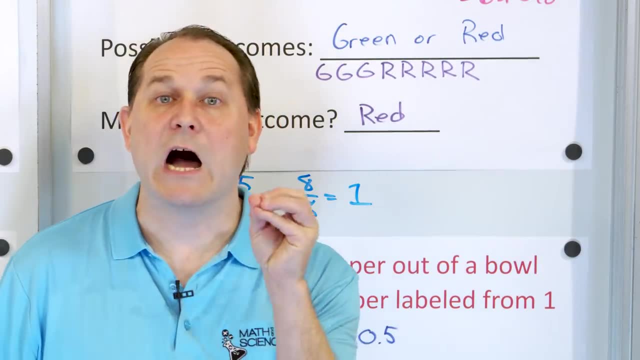 I can get an even number five ways, but there's a total of ten papers and that means the probability of pulling it is one half, which is the same as 0.5.. Now here's the next question: What is the probability of drawing an odd number? 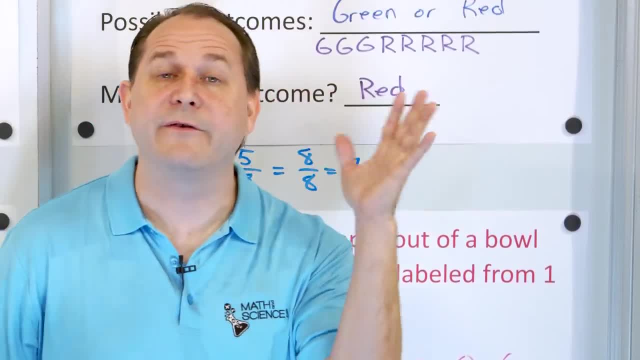 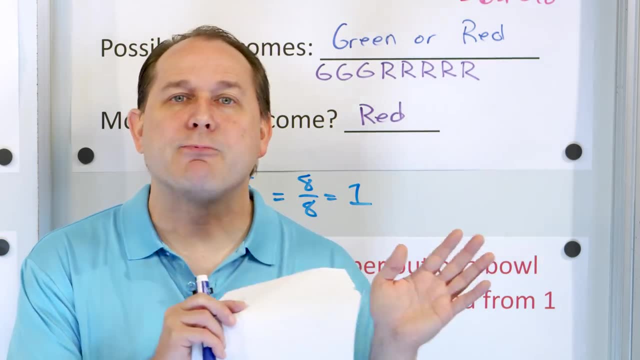 Well, how many odd numbers are there? One, two, three, four, five, Again five, but there's still ten total numbers. So again five out of ten. So the probability of odd is also one half, and the probability of even is also one half. 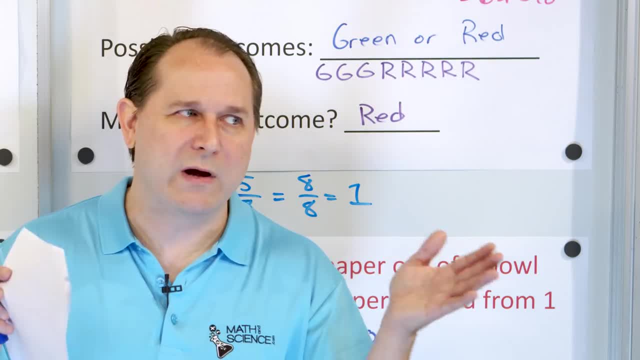 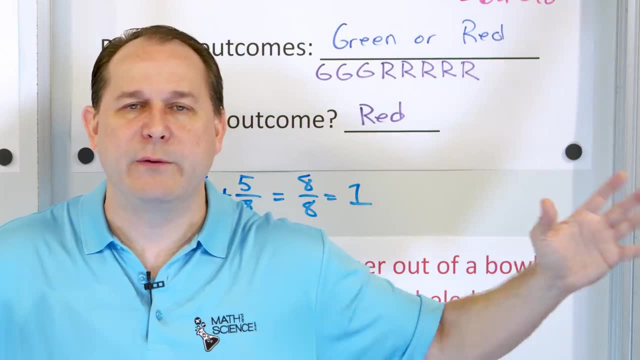 And when you add all the possible outcome probabilities you should get one. One half plus one half is one In every one of these examples, the probability, when we calculate all the probabilities that we can do and we add them all together, all the ways in which the outcomes can happen. 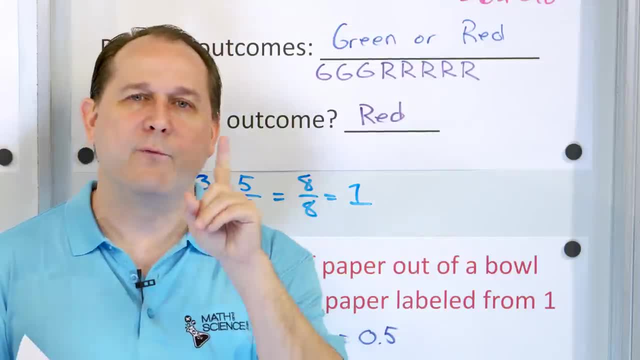 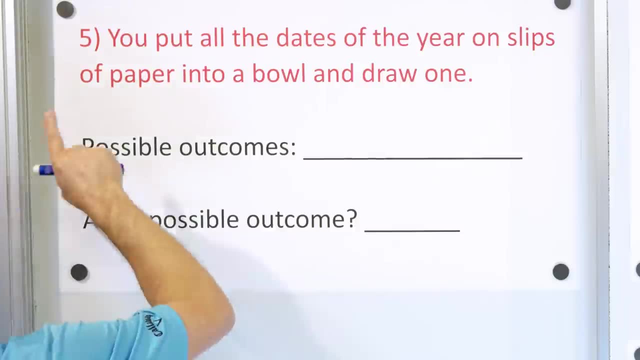 they always have to add to one, and that is shown here as well. I have one more. Let me take these down and we'll conquer the last one and wrap up this lesson. All right, Here's our very last problem. It says you put all of the dates of the year on slips of paper into a bowl and draw one. 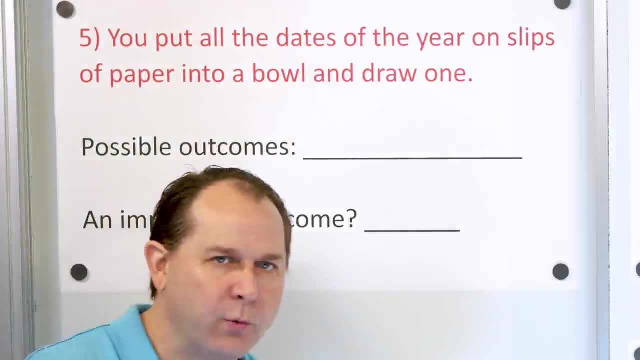 So what are the possible outcomes? You know I have January 1,, January 2,, January 3, all the days of the year, all the way through December 31 in there. So the possible outcomes is- I'm just going to put all dates- 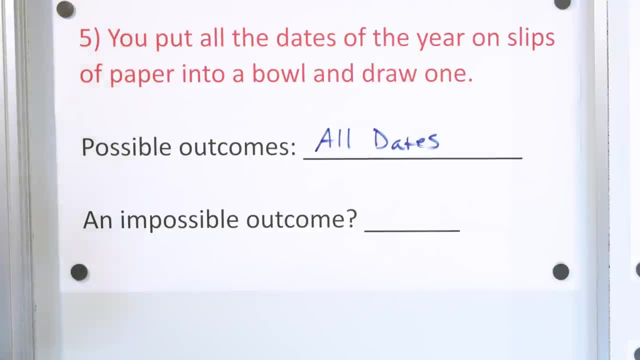 So there's 365 pieces of paper in general in that bowl right. And give me an example of an impossible outcome. Well, of course, January 1, I could pull it out. January 2, I could pull that out. 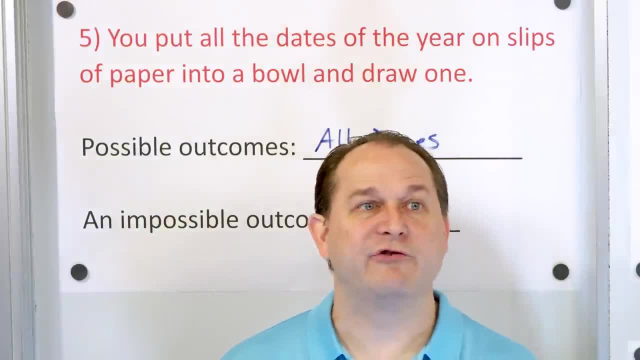 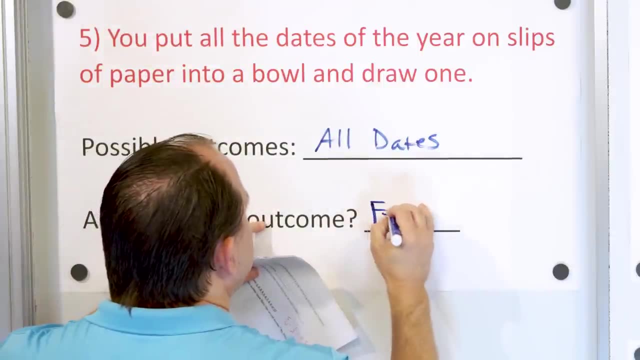 January 3,? I could pull that out. Give me an example of an impossible date. How about July 35? There is no July 35. That's an impossible outcome. Or you could say something like February 30. That never happens either. 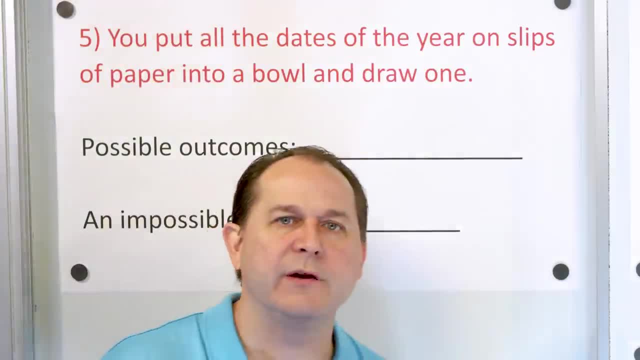 So what are the possible outcomes? You know I have January 1,, January 2,, January 3, all the days of the year, all the way through December 31 in there. So the possible outcomes is- I'm just going to put all dates- 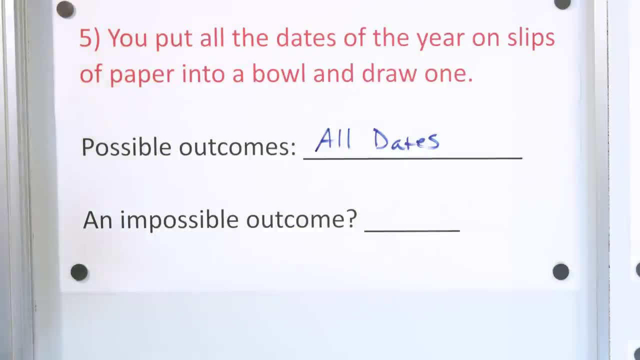 So there's 365 pieces of paper in general in that bowl right. And give me an example of an impossible outcome. Well, of course, January 1, I could pull it out. January 2, I could pull that out. 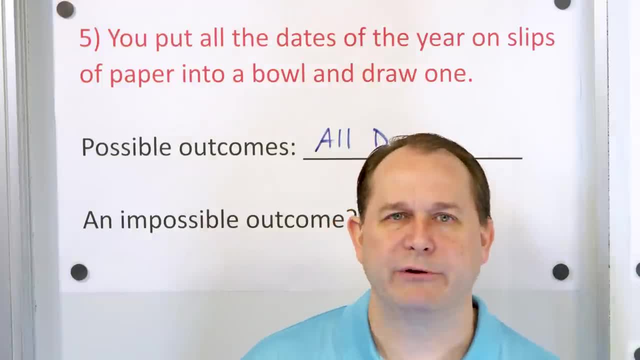 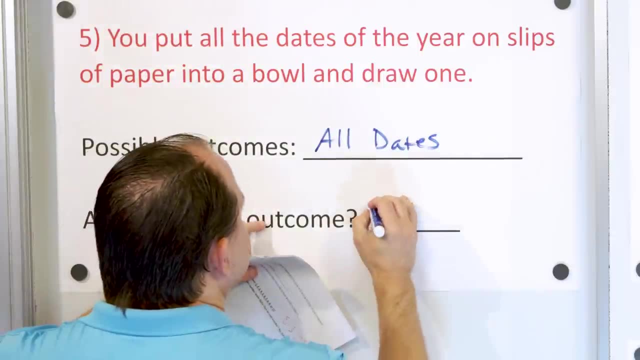 January 3,? I could pull that out. Give me an example of an impossible date. How about July 35? There is no July 35. That's an impossible outcome. Or you could say something like February 30. That never happens either. 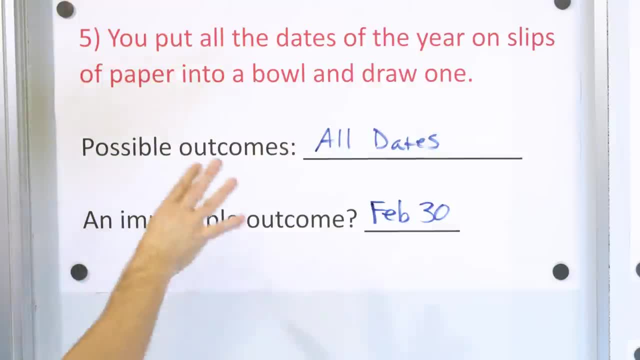 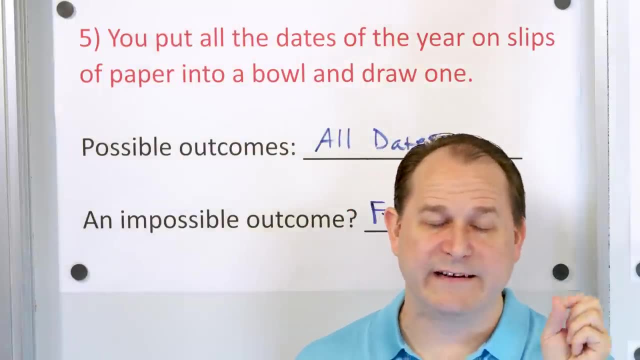 So that's an impossible outcome. So here we didn't calculate anything, But still understanding the possible outcomes and an example of an impossible outcome is important too For rolling the dice. a six-sided dice, a die. an impossible outcome might be getting a number 8.. 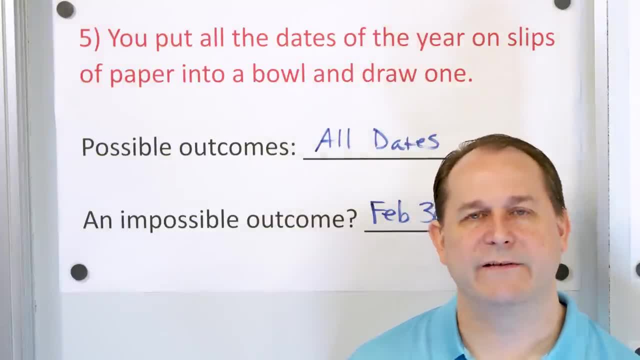 You can't get an 8 on a six-sided die. That's impossible as well. So here we've conquered quite a bit. The main thrust of this lesson actually isn't to calculate probabilities. We're going to do a lot of that later. 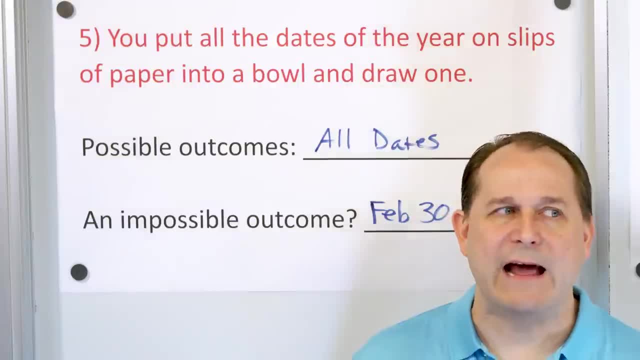 But I just couldn't resist helping you and showing you how to do that, as we're learning these basic ideas, because I think it's very intuitive for us to understand how to do it. The main thrust is understanding what a trial is, what an experiment is. how do you look at the number of outcomes? 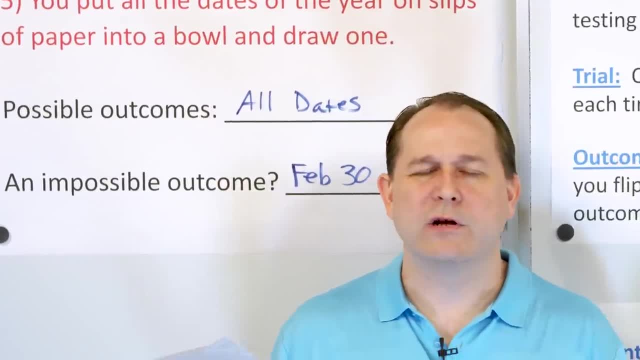 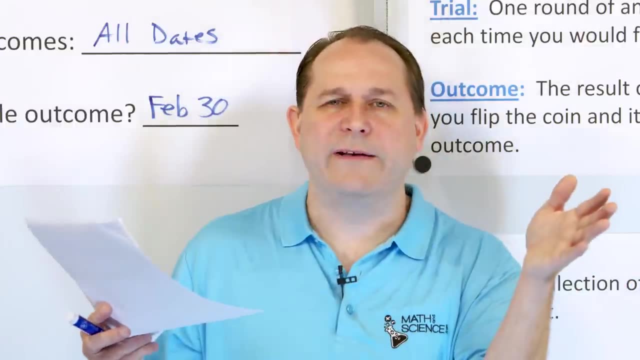 and to get a feel for is it equally or not equally likely to get the outcomes? And, basically, if the number of ways in which you can get an outcome, if you have a certain number of ways in which something can happen and they all can happen, the same number of ways, 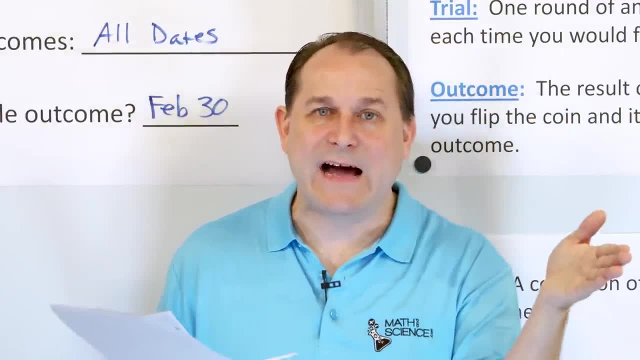 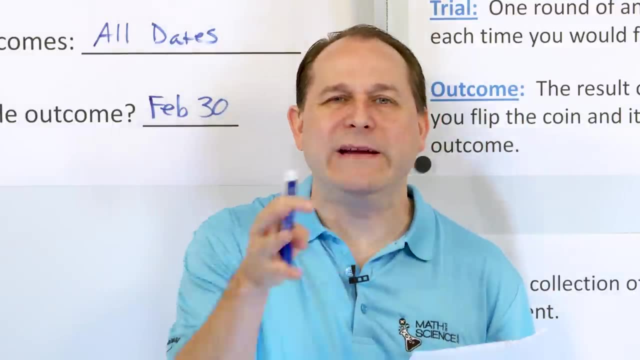 like heads or tails, there's only one head and one tail. On a six-sided die there's six numbers, But each number only happens once. Then you have equally likely outcomes. But if you change the die and you make it where, like, three sides have the same number, 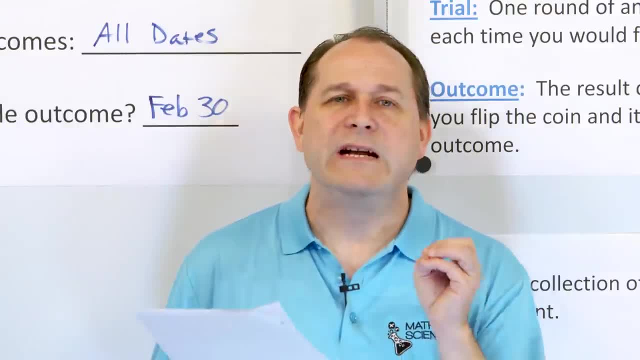 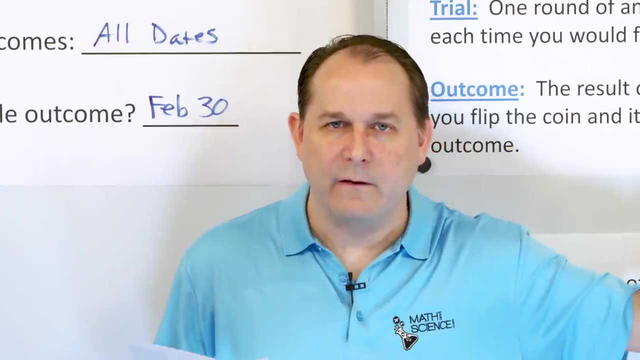 well then, things are not equally likely anymore, But in all cases, I also showed you to calculate that probability. you look at: how many ways can you get what you're looking for, like heads divided by as a fraction, how many total outcomes possible are there? 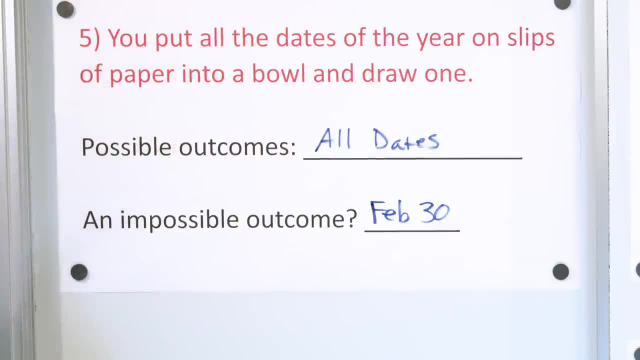 So that's an impossible outcome. So here we didn't calculate anything, But still understanding the possible outcomes and an example of an impossible outcome is important too For rolling the dice. a six-sided dice, a die. an impossible outcome might be getting a number eight coming out. 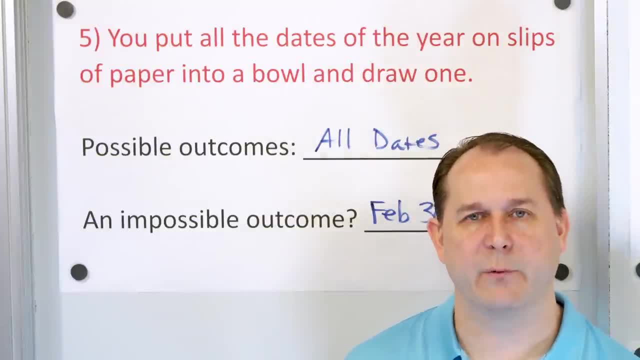 You can't get an eight on a six-sided die. That's impossible as well. So here we've conquered quite a bit. The main thrust of this lesson actually isn't to calculate probabilities. We're going to do a lot of that later. 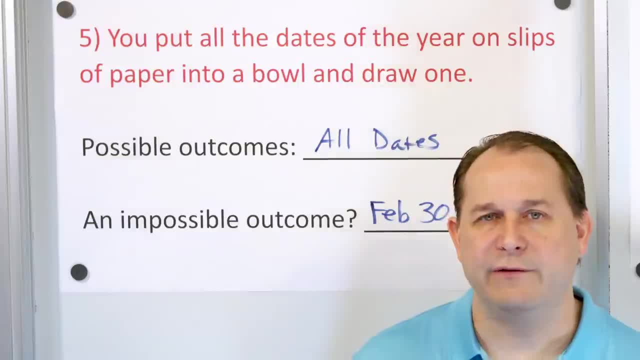 But I just couldn't resist helping you and showing you how to do that, as we're learning these basic ideas, because I think it's very intuitive for us to understand how to do it. The main thrust is understanding what a trial is, what an experiment is. 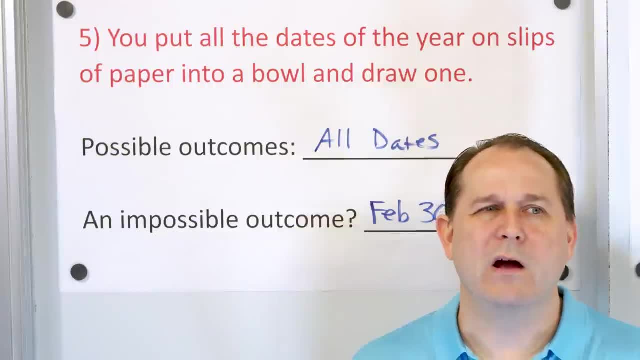 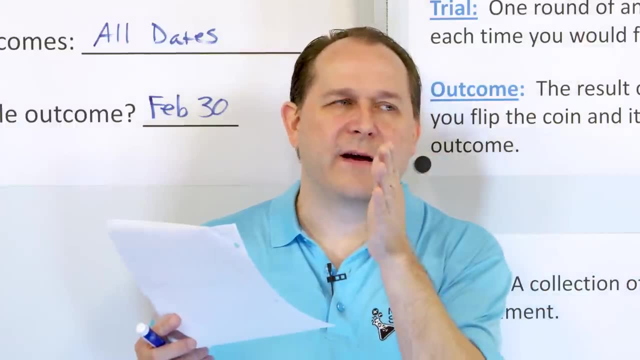 How do you look at the number of outcomes and to get a feel for, is it equally or not equally likely to get the outcomes And, basically, if the number of ways in which you can get an outcome, if you have a certain number of ways in which something can happen and they all can happen, the same number of ways? 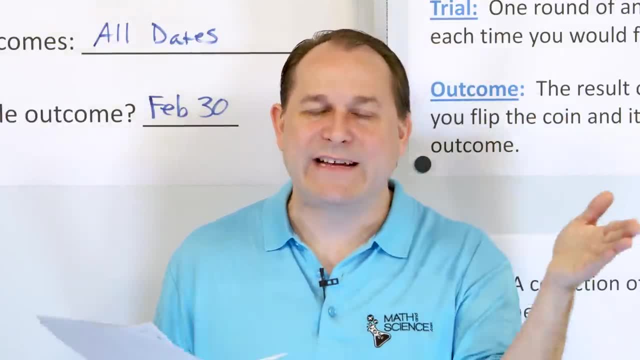 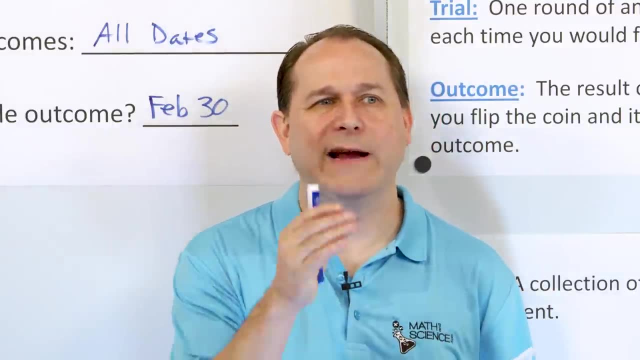 like heads or tails, there's only one heads and one tail. On a six-sided die there's six numbers, But each number only happens once. Then you have equally likely outcomes. But if you change the die and you make it where, like, three sides have the same number, 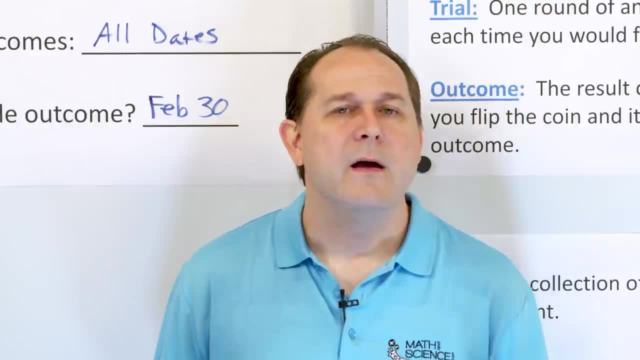 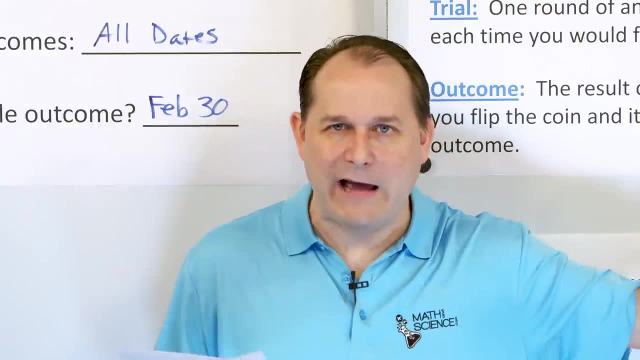 well then, things are not equally likely anymore, But in all cases, I also showed you to calculate that probability. you look at: how many ways can you get what you're looking for, like heads divided by as a fraction, how many total outcomes possible are there? 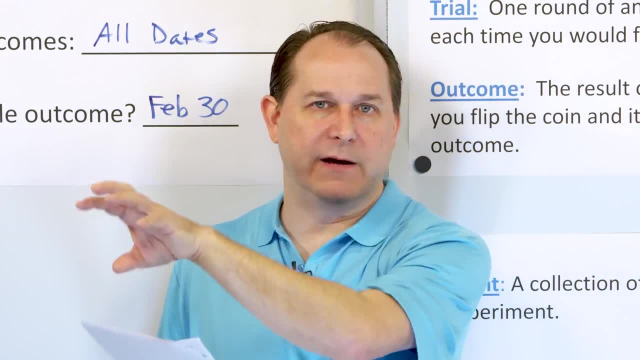 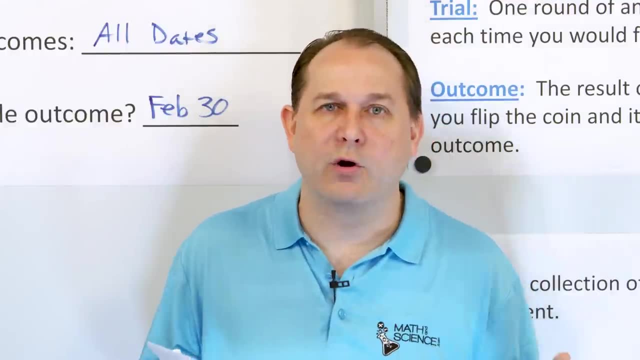 And when you look at the probability of all the different outcomes, all the different things that can happen, when you add all those up, you should always get one, because then you know that when you do an experiment or a trial, you're going to definitely get one of those outcomes. 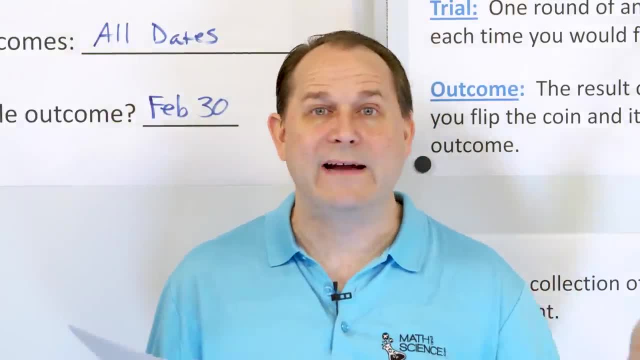 So when you add the probabilities, it's just like adding fractions. They should always be equal. They should always add up to one. Okay, a lot of stuff in there. Let's wrap this up. Go through it. Make sure you understand. 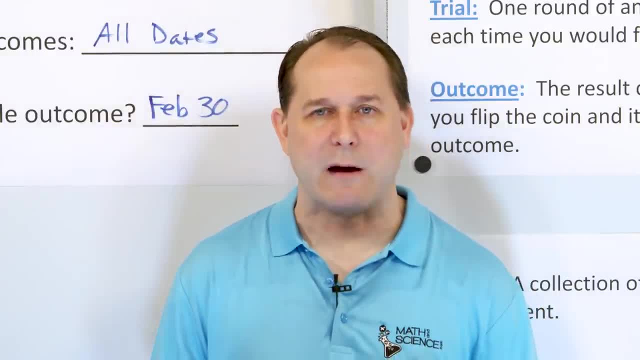 Go on to part two. We'll continue considering some other scenarios to understand probability.